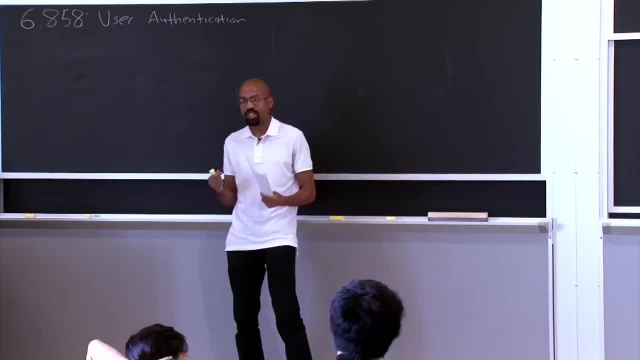 In particular, the paper that was assigned for today's class addresses sort of an existential question in the security community: Is there anything better than passwords for authentication? So at a high level it seems like passwords are a terrible idea, So they have very low entropy. It's very easy for attackers to guess them. Also, the security questions that we use to recover from lost passwords often have even lower entropy than the passwords themselves, which also seems like a problem. Even worse, users typically will use the same password across a lot of different sites. 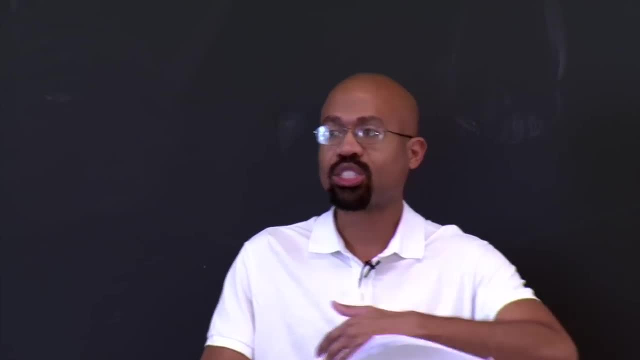 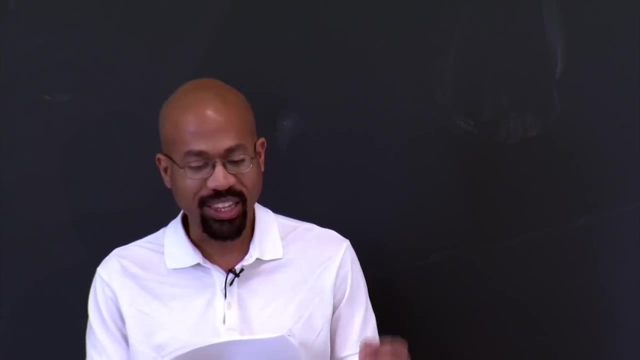 So that means that the vulnerability in one password, if it's easy to guess, could expose a user's activity across a wide range of sites. So, as the paper for today's class states- I love this quote- The continued domination of passwords over all other methods of end user authentication. 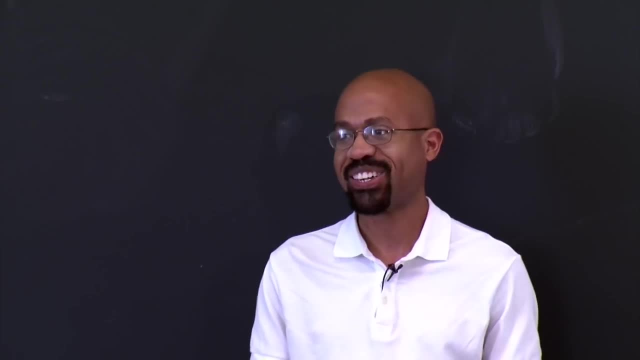 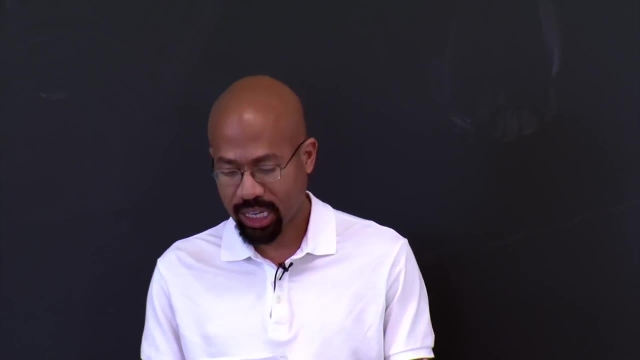 is a major embarrassment for security researchers. So the community is just seething out there. They want some better alternative, But it's not clear if there actually is an authentication scheme that actually totally dominates passwords. that's more usable, that's more deployable. 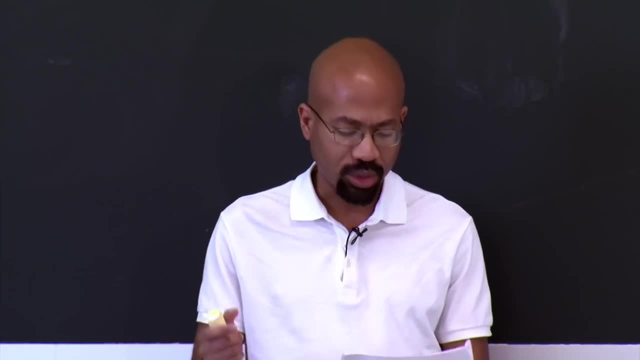 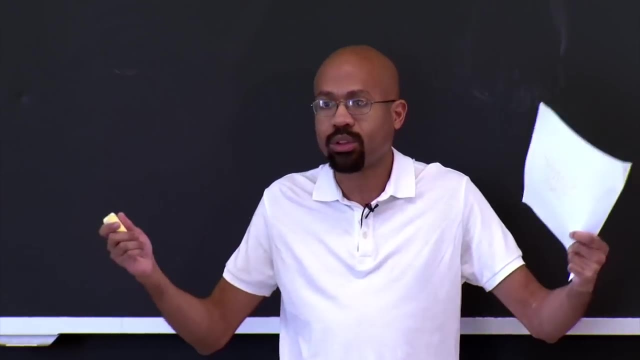 that's more secure. So in today's lecture we're basically going to do three things. First of all, we're going to look and we're going to see how current password schemes work. Then we're going to talk about the desire of all properties at a high level. 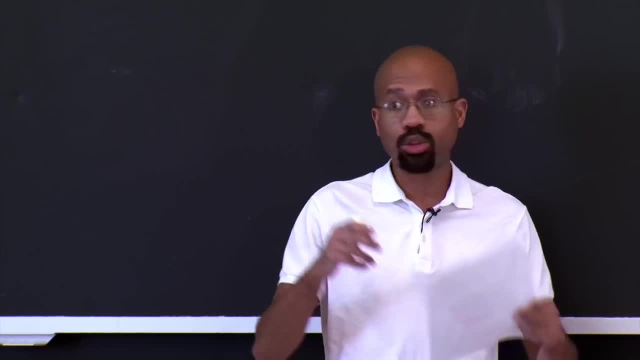 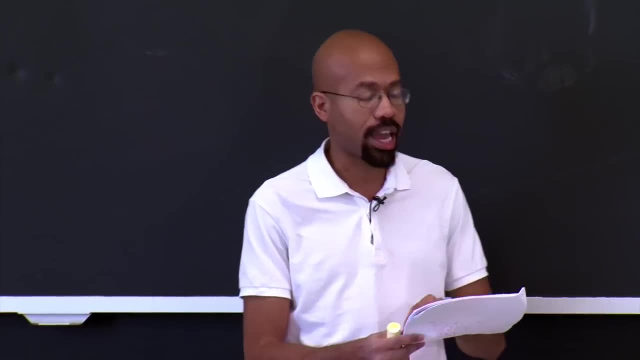 for any authentication scheme, And then we're finally going to look at what the paper gives us in terms of metrics for authenticating authentication schemes And we're going to see how some of these other authentication schemes actually compare to passwords. So, at a high level, what is a password? 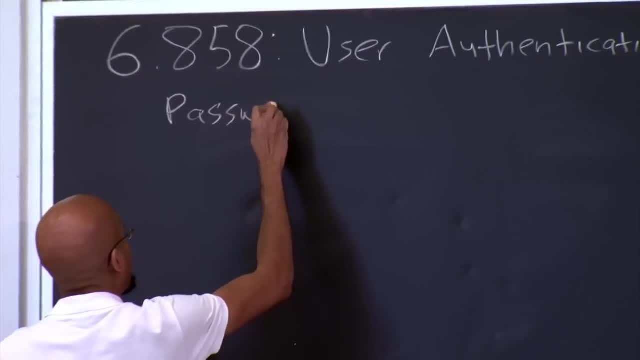 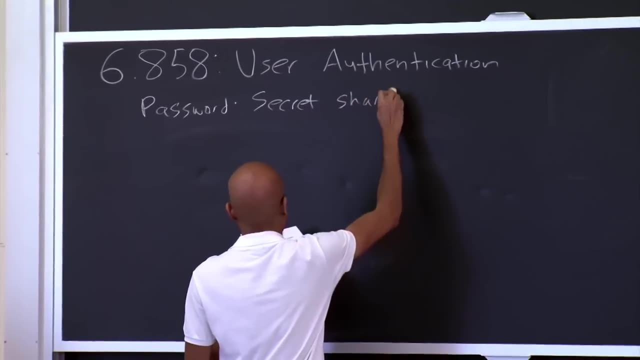 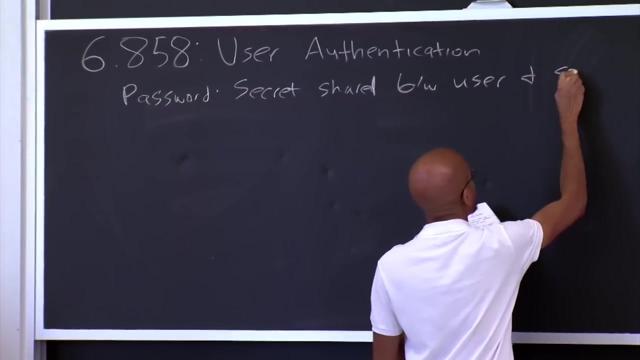 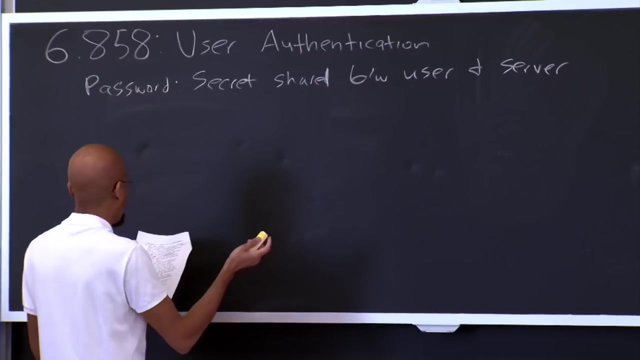 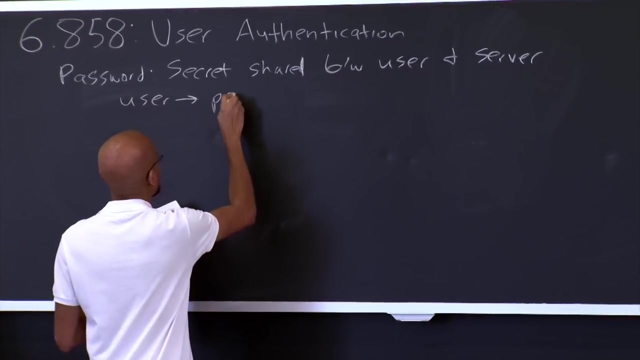 So a password is a secret that is shared between a user and a server. So the naive implementation of a password scheme is to basically just have a table on the server side that essentially just maps user names to passwords. That's the simplest way you can imagine implementing. 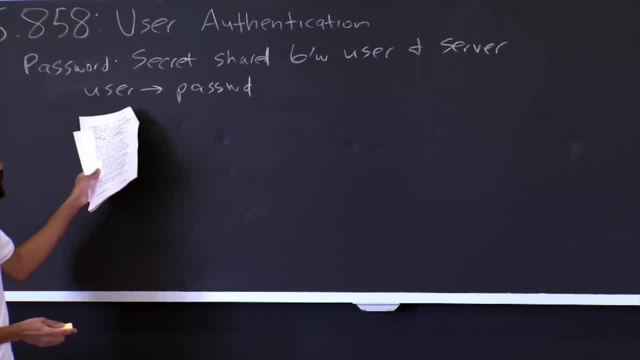 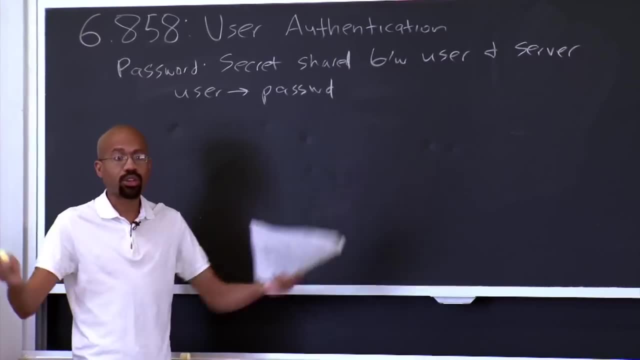 one of these authentication schemes. User passes in their user name and their password. The server does a look up. in this table compares the password that the client supplied. what's in here? If everything's good, the user's authenticated. So clearly the problem with this is: 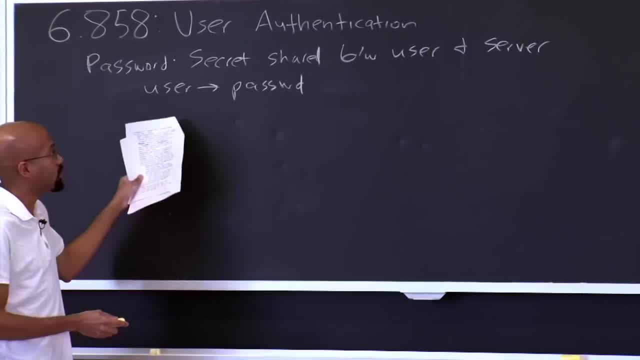 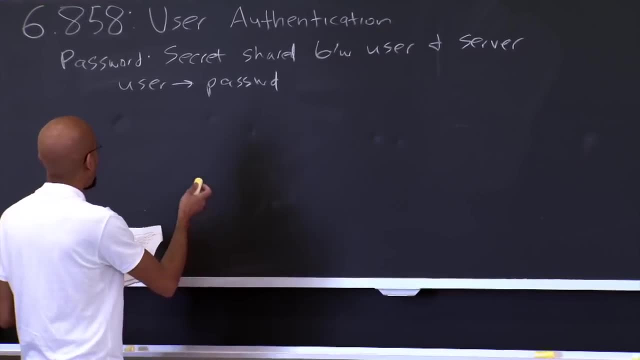 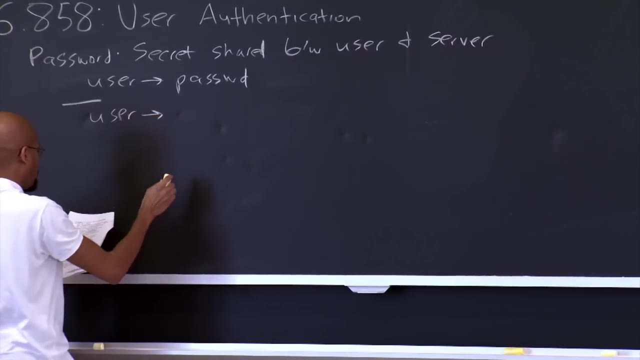 that if the attacker compromises the server, then it can just look at this table and then get all the user's passwords in the clear. So that's clearly a bad thing. So perhaps an improved solution is to have the server store table that looks like this: 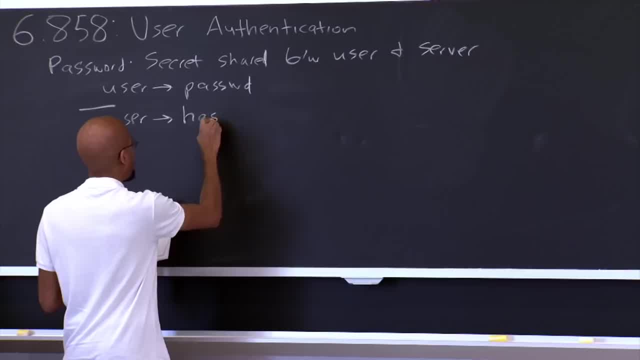 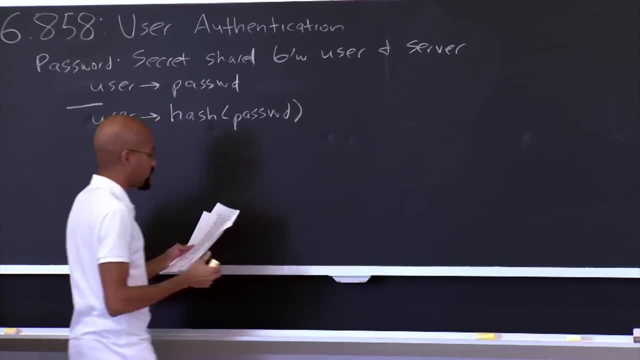 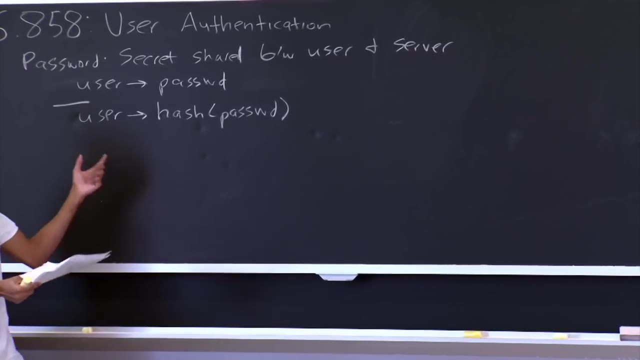 So once again it maps the user name, but now it actually maps to the server, So it's a hash of the password. So the user client is going to supply their clear text password to the server. The server will then take that clear text password hash it. 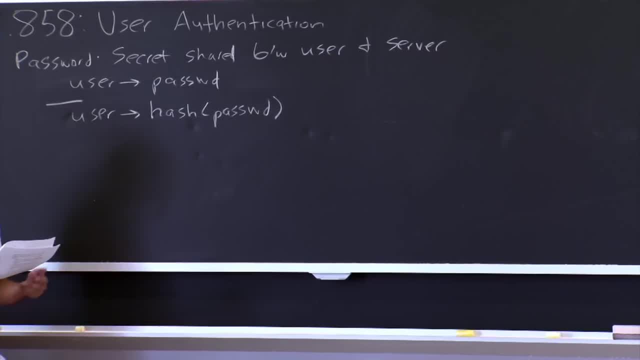 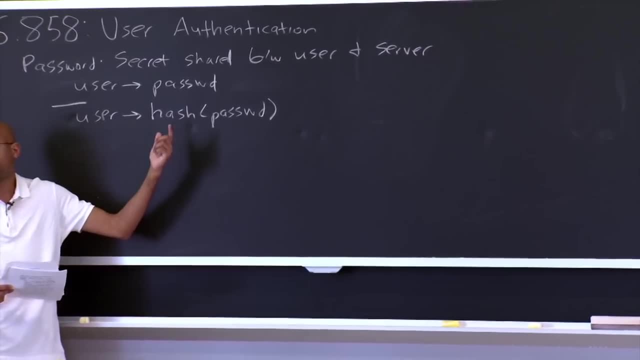 do a look up in the table and once again see if the user is who he or she says that they are. So the advantage of this scheme is that by design these hash functions are difficult to invert. So if this table is lost, it's leaked somehow. 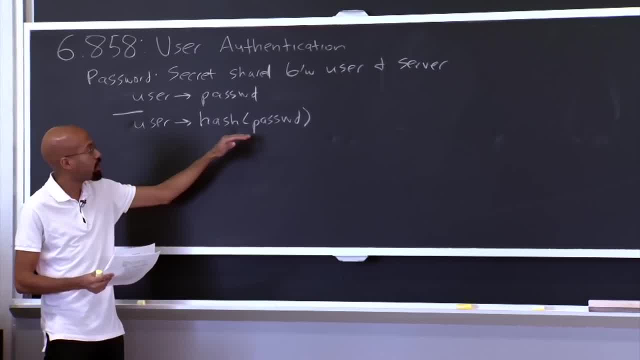 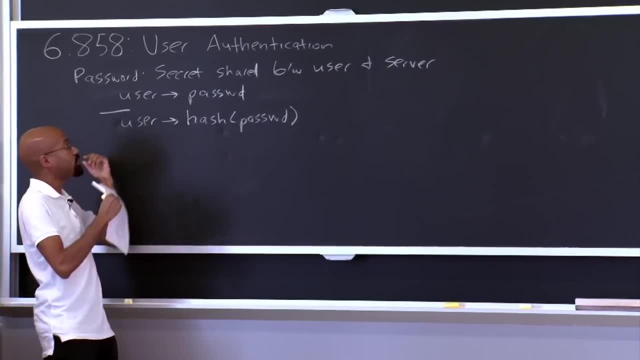 or the attacker compromises the server And the attacker can look at these things here, but it's difficult for the attacker to say, OK, this string of random alphanumeric characters here. here's the pre-image that was used as the input of the hash function. 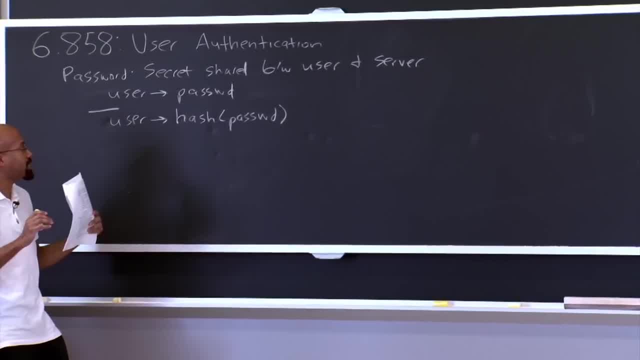 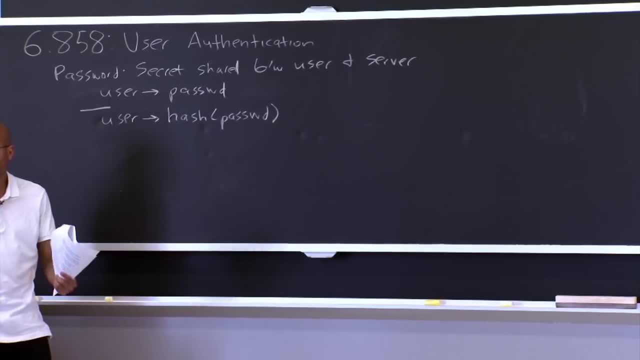 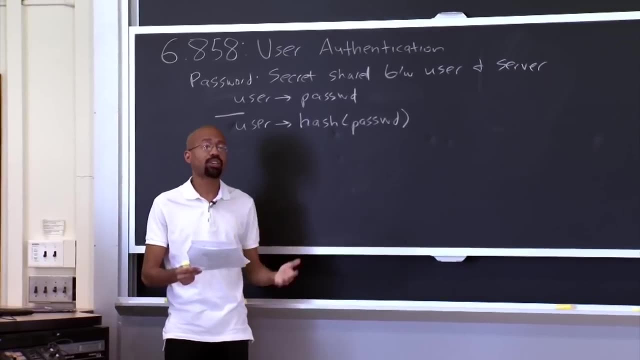 to generate that value there. So that, at least, is the nice thing about these hashes in theory. Now, in practice, attackers don't actually have to launch brute force attacks to figure out what the pre-image is for these hash values. OK, So attackers can actually take advantage of the fact. 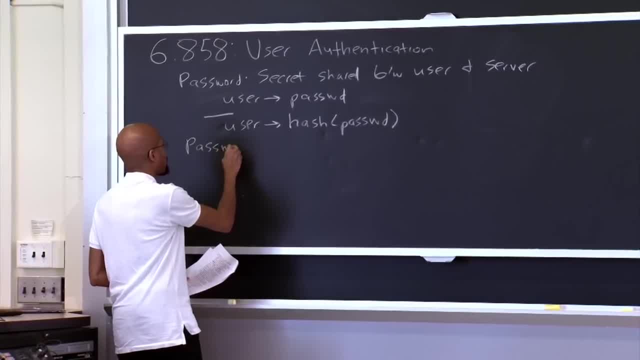 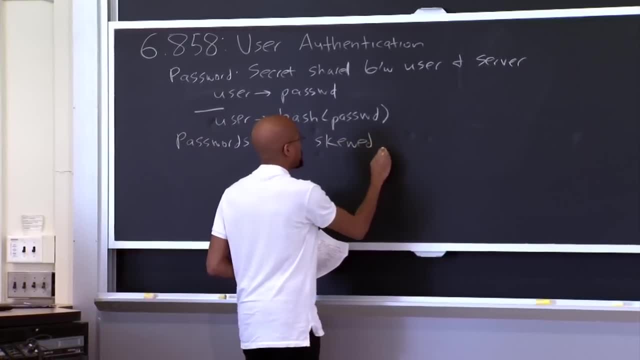 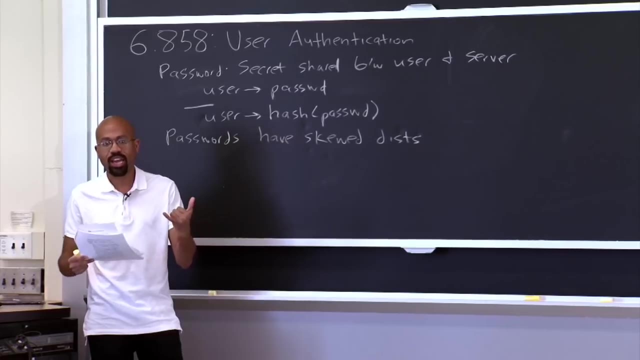 that passwords in practice have skewed distributions, And by skewed distributions I mean that let's say that we knew that all passwords are 20 characters long. It's not like users actually pick passwords that sort of exist in all places in that space of 20. 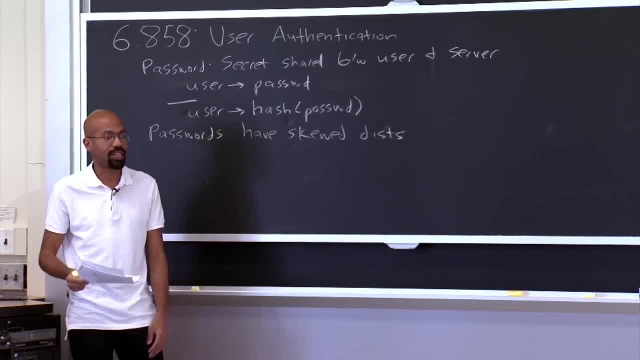 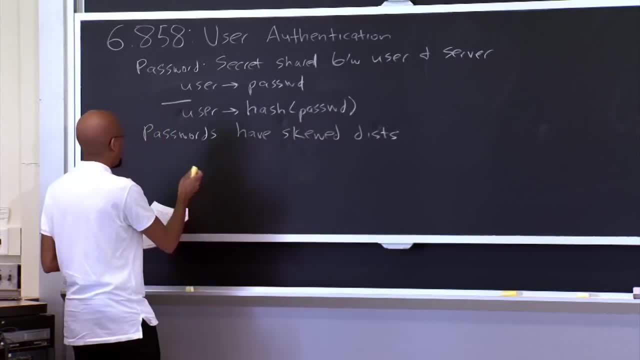 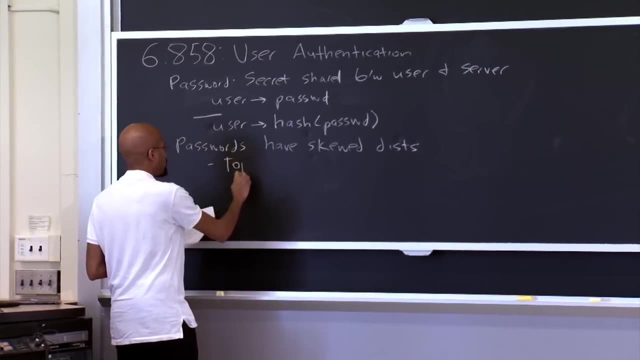 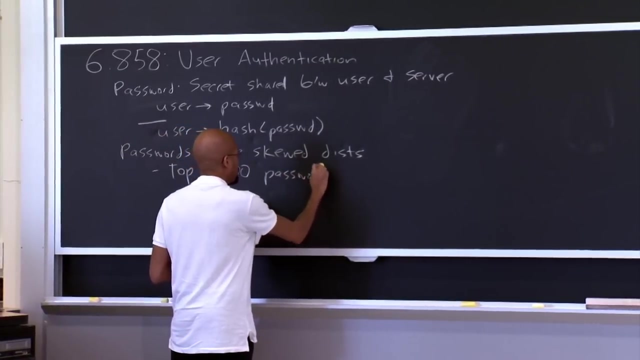 possible characters. In practice, people pick passwords like 123, or Todd or things like this, And so, in fact, there's been these empirical studies of how passwords work, And a lot of times these studies find things like: the top 5,000 passwords cover about 20%. 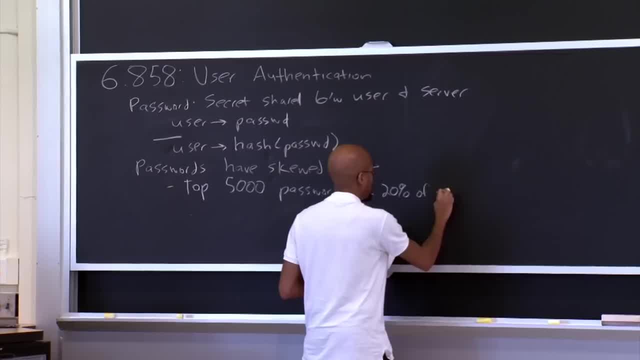 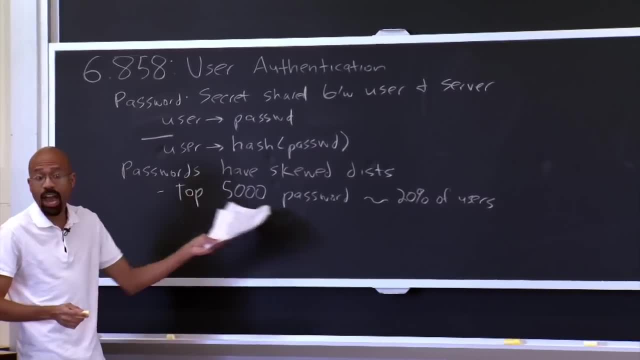 of users. So what that means, in other words, is that if the attacker, if the attacker has a database of those 5,000 passwords, then the attacker can just hash those And then when the attacker looks at this stolen password table, 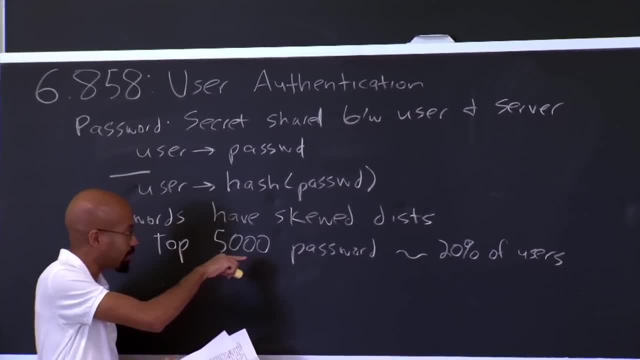 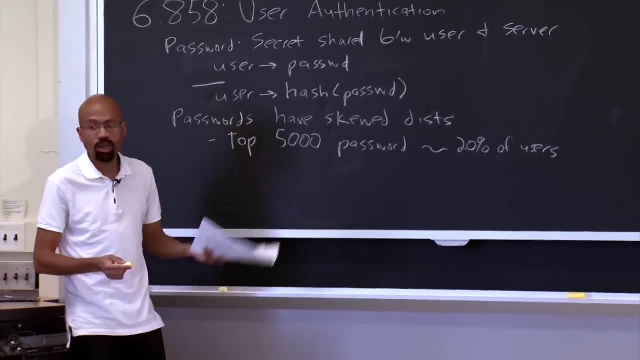 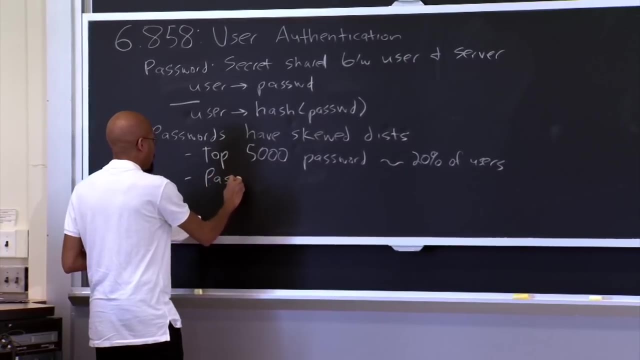 can just see if any of those things that come from this 5,000 large list match over here, And so, empirically speaking, the attacker will be able to recover about 20% of passwords that way, And so folks at Yahoo found that passwords have roughly. 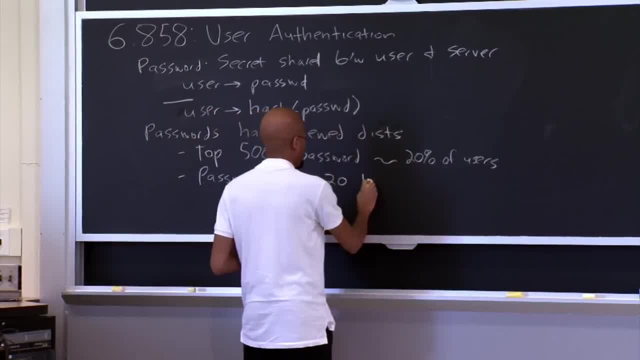 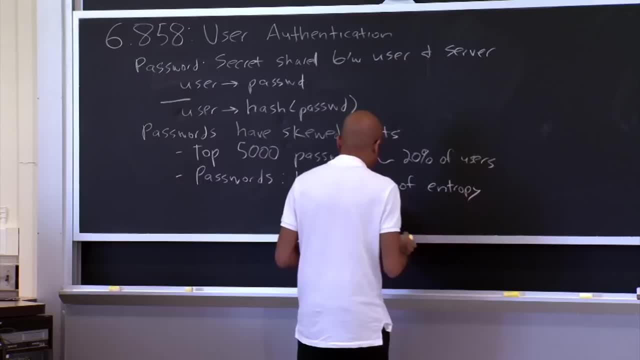 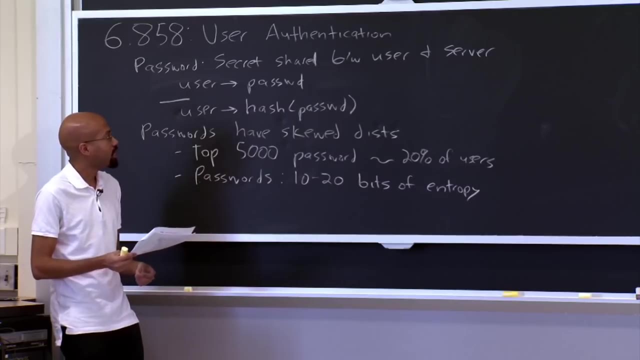 10 to 20 bits of entropy, 10 to 20 bits of randomness in them, And that's actually not that big. So, for example, if you think about what might this hash function here be? So maybe it's something like SHA, something like this. 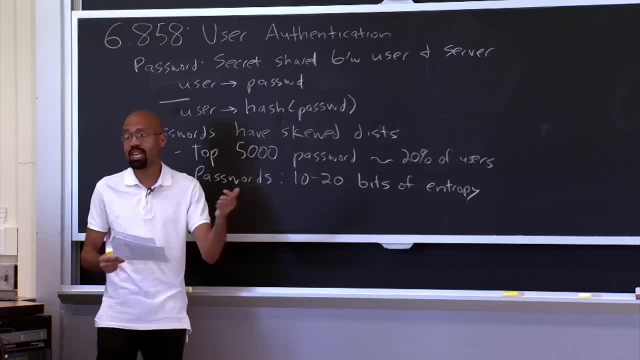 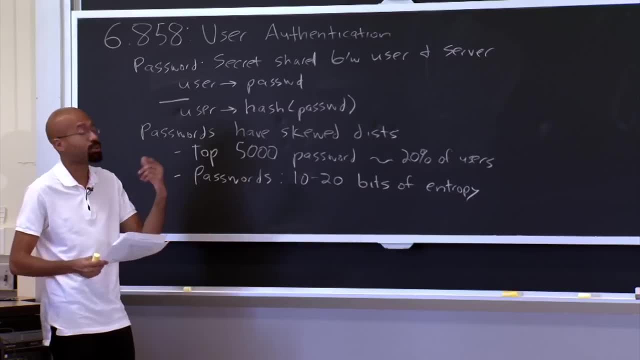 So modern machines can actually calculate millions of these hashes every second. So the fact that hash functions, by design, are supposed to be easy to calculate, supposed to be fast to calculate, combined with this fact that they're these skewed password distributions, means that, in principle, this scheme here 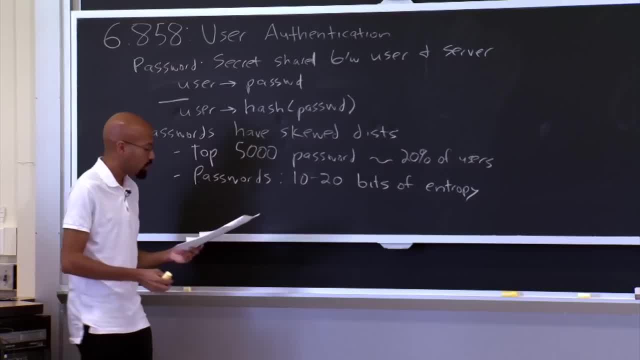 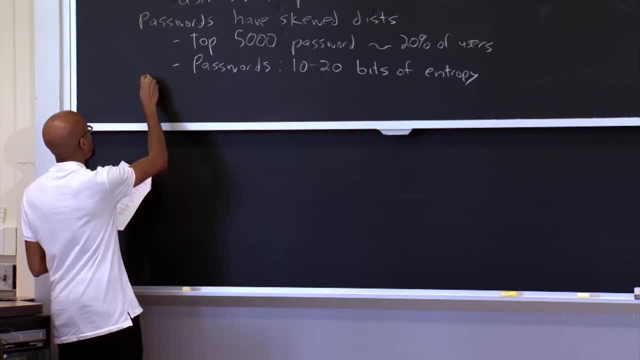 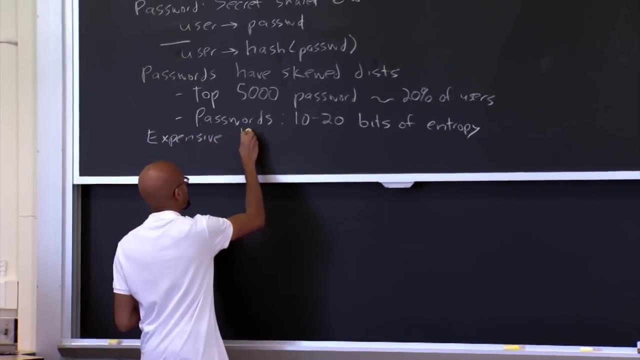 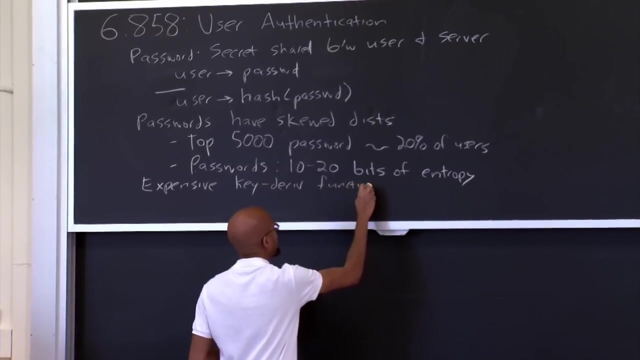 is not as secure as it might seem. So one thing you can imagine to try to make life more difficult on the attacker is you could imagine that you use an expensive key derivation function, And so by key derivation function I just mean This thing up here. 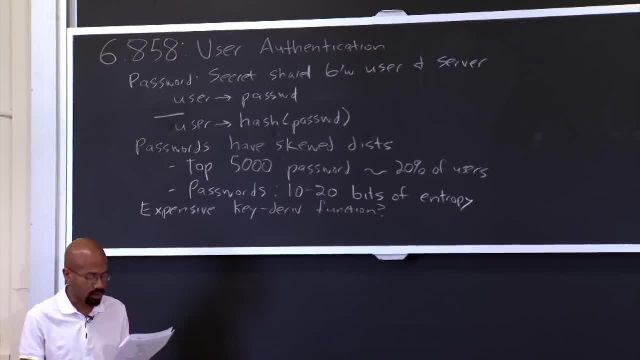 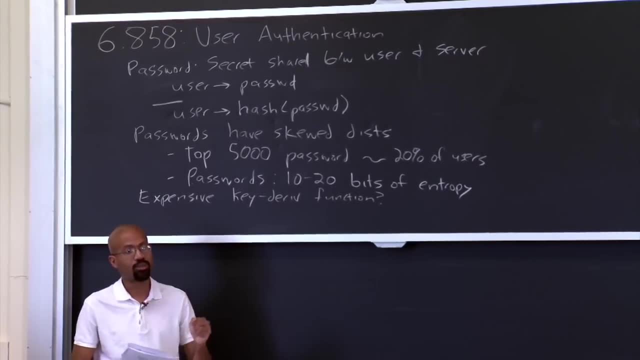 This thing that's taking the password as an input and then generating something that's stored on the server. And so what's nice about these key derivation functions is that they actually have sort of tunable cost, So you can basically turn this knob and make that function run slower or faster. 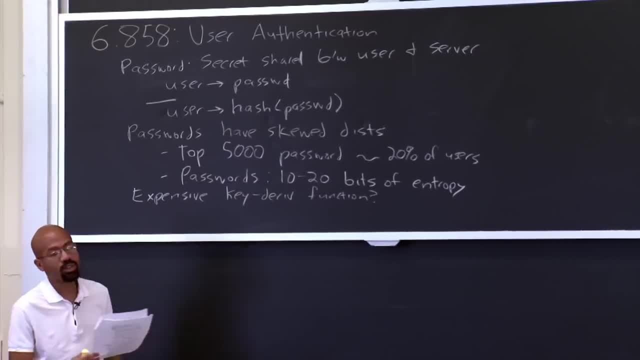 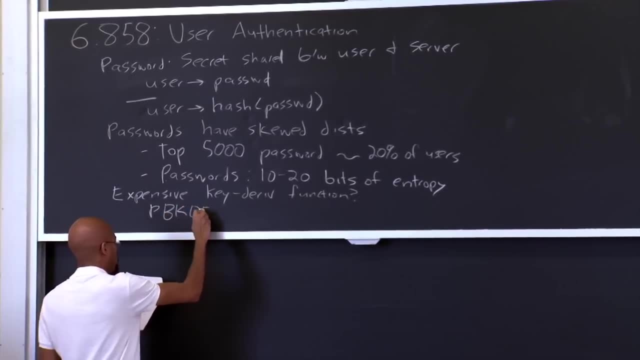 depending on what you want, And so the idea here is that let's say that you're going to use a key derivation function. So some of these examples are like PB, KDF2.. Or maybe bcrypt. You can look these up using the miracle of the internet. 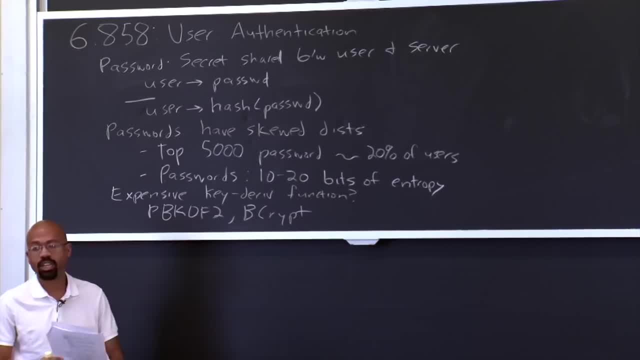 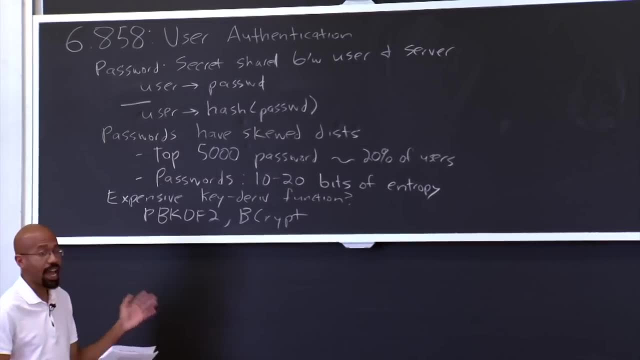 if you care to know more about them. But the base idea is: let's imagine that one of these key derivation functions took a second to calculate as opposed to a few milliseconds. That actually makes the attacker's job much more difficult, Because then when the attacker is trying to, let's say, 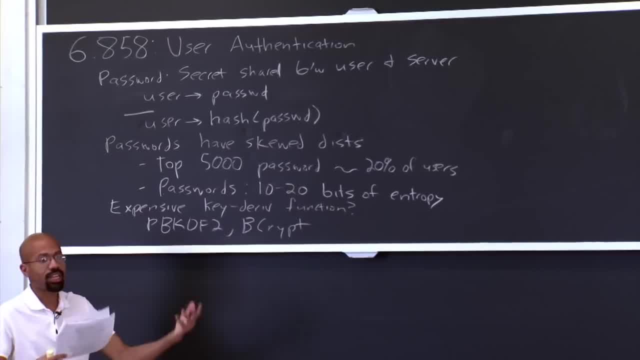 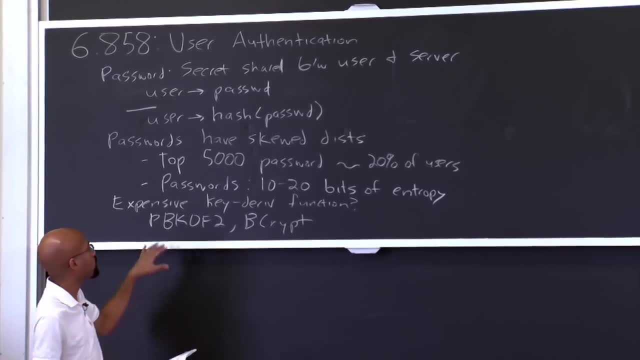 generate values for these 5,000 topmost passwords. it's going to take the attacker much longer to do that, So does that all make sense? how these things work? Pretty straightforward, And so, internally, these key derivation functions often operate by repeatedly calling a hash. 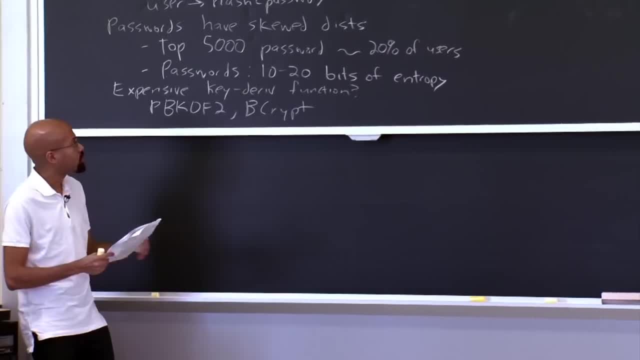 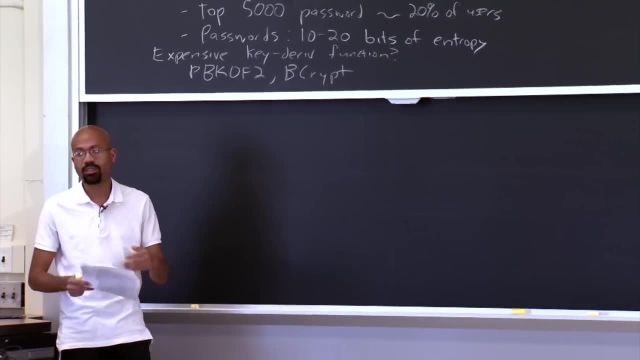 multiple, multiple times. So that's all pretty straightforward. So you might say: well, does this solve the problem? So can we just use these expensive key derivation functions and be done with it? So this is a security class, Of course, the answer is no. 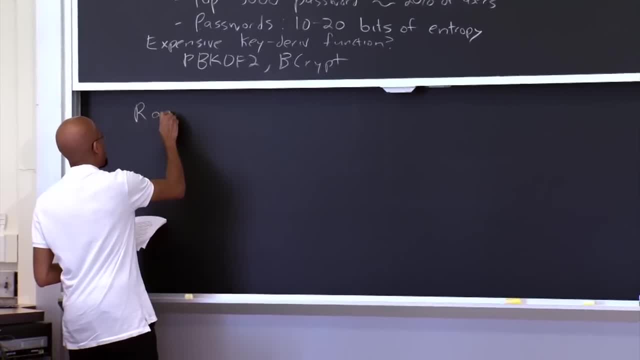 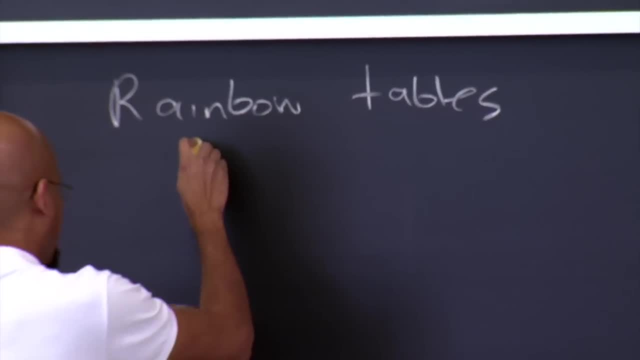 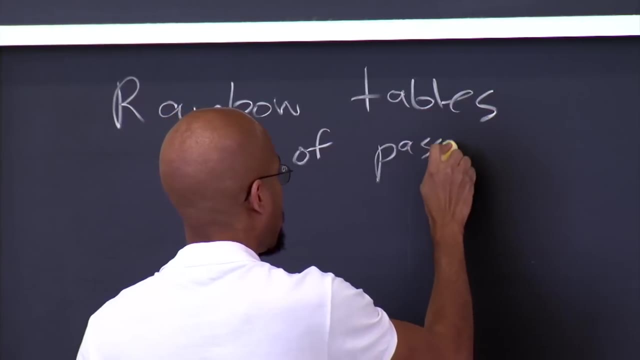 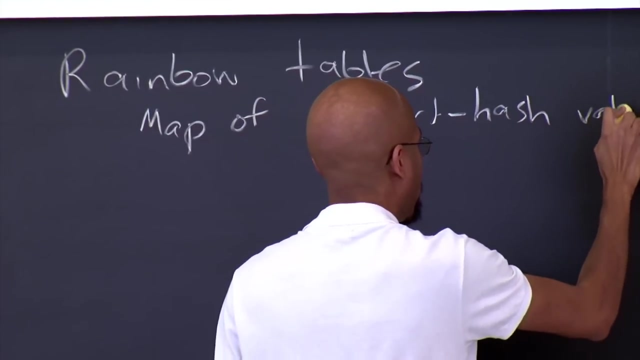 So one problem is that the adversary can build something called rainbow tables, And so a rainbow table is basically just a map of password to hash values, And so the insight here is that, even if the system is using one of these expensive key derivation functions, 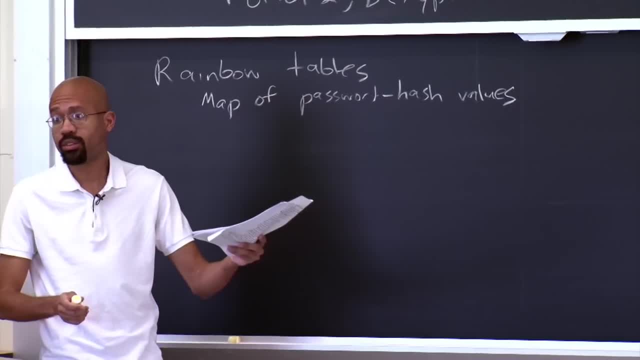 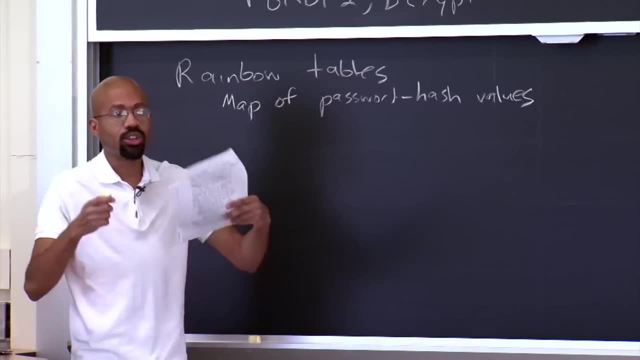 the attacker can calculate one of these tables once. It might be a little bit painful because each key derivation function invocation is slow, But the attacker can build this table once and then use that to crack all subsequent systems. the attacker can break into that. use that same key derivation. 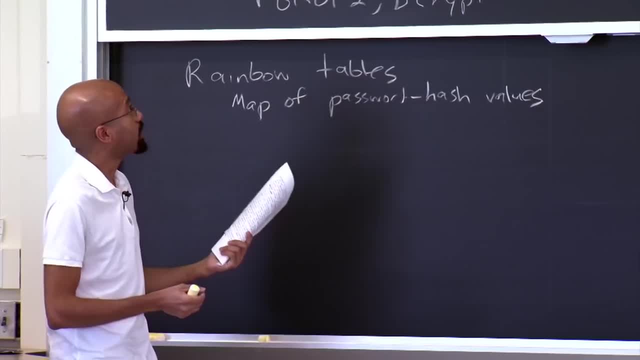 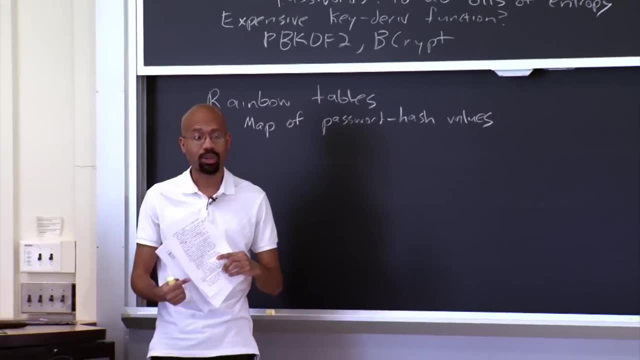 function. So that's how rainbow tables work And, once again, to maximize the cost benefit of building this rainbow table, the attacker can take advantage of these skewed password distributions like we see up here. So the attacker might only need to build a rainbow table for some small set of all possible passwords. 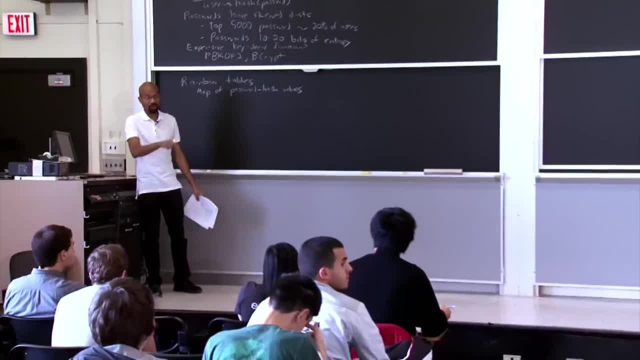 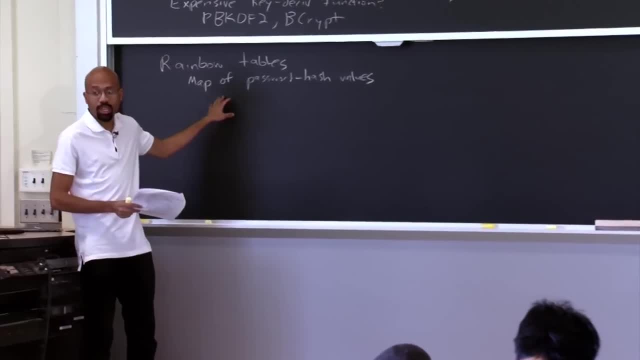 So salting makes this much more difficult. Yeah, that's right. So we're going to get to salting, I believe, in a couple seconds. That's right. So, but at a high level, if you don't use salting rainbow tables actually. 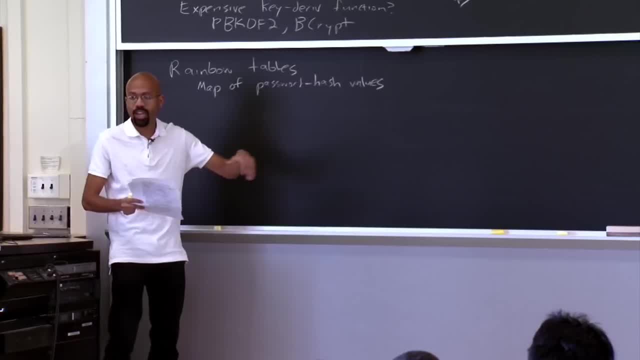 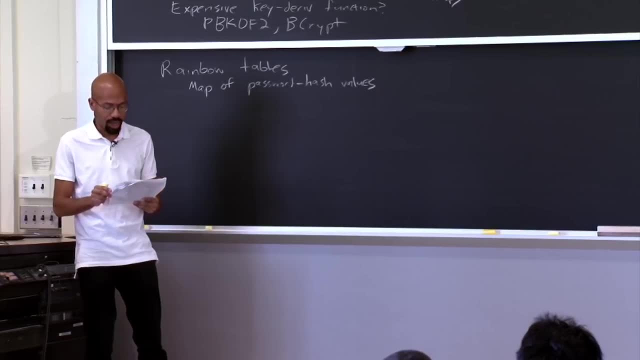 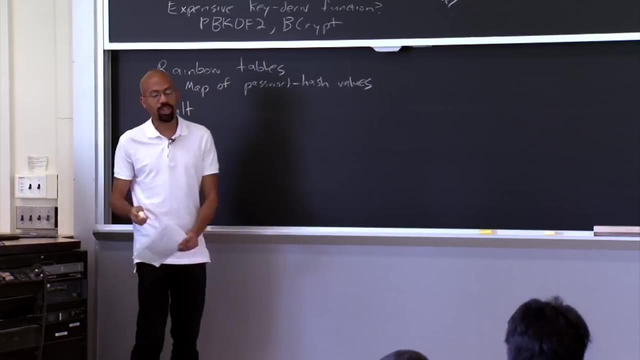 allow the attacker to spend some effort offline, calculate this table and then amortize the cost of calculating that table over, breaking many different password databases, And so the next thing that we can think about to improve things is salting. I swear that guy was not a plant. 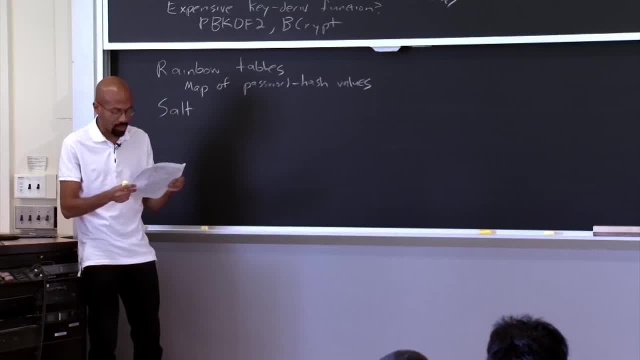 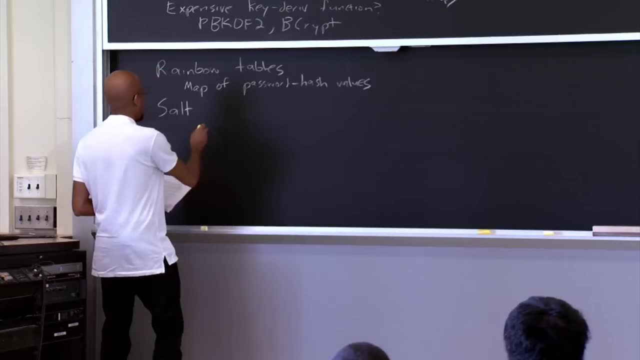 I'll give you your $20 after class. So how does salting work? So the basic idea is that you just want to input some additional randomness into the way that the password is generated. So basically, you want to take this hash function. 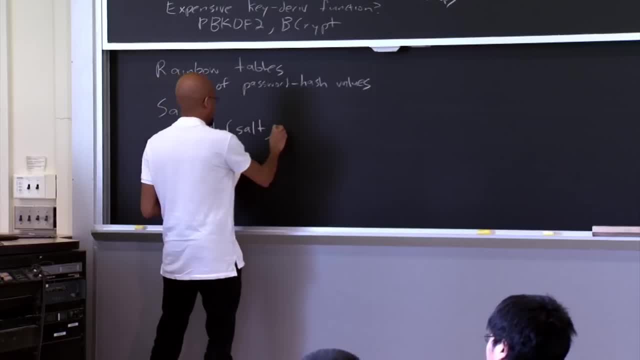 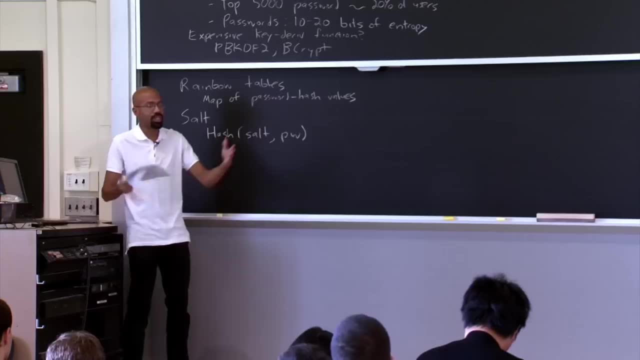 and you want to put some salt in there, which I'll explain in a second, and then the password, And this is the thing that you store on the server side in the table. So what is this salt? I mean, just think of it as just a string. 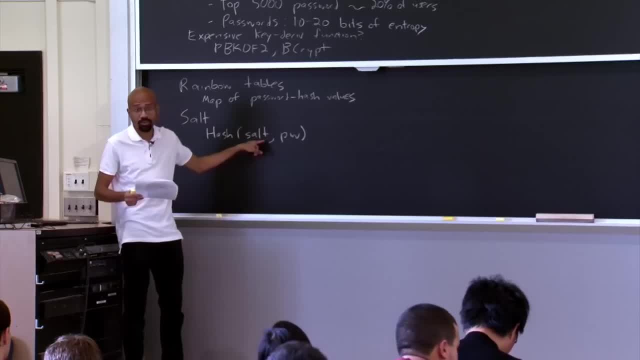 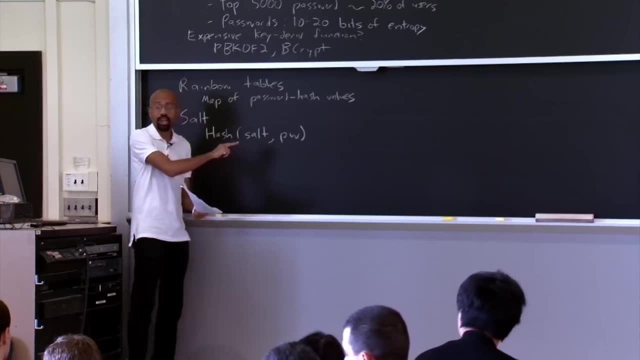 a long string that's provided as sort of the first part of this hash function. So why is it better to use this scheme And note that the salt Is actually stored in the clear text on the server side? So you might be thinking, OK, well. 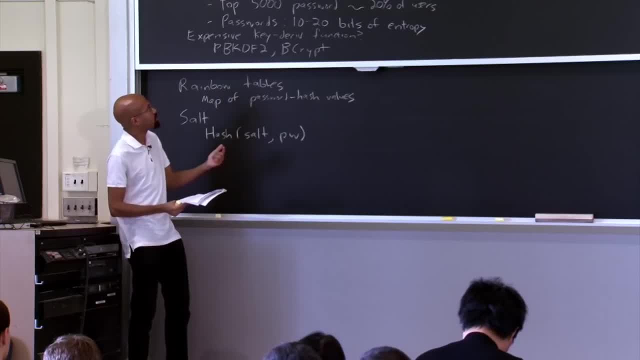 if that salt is stored on the clear text on the server side, it seems like the server can both steal the table that maps usernames to passwords, and the attacker can also steal the salt. So why is that useful? Because you pick the top most common password. 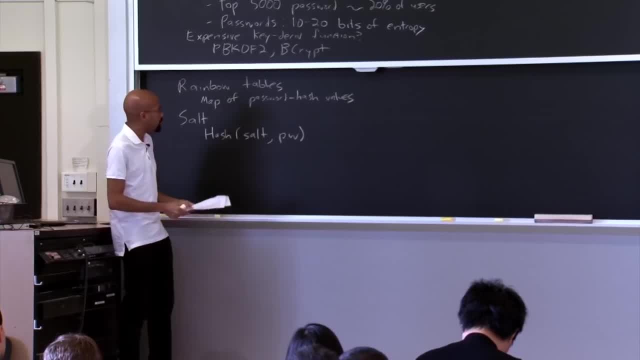 and you can't just use it once and find any user. That's exactly right. So basically, what this does is this prevents the attacker from building a single rainbow table and then using that rainbow table against all instances of that hash function, And so you can basically think of this: 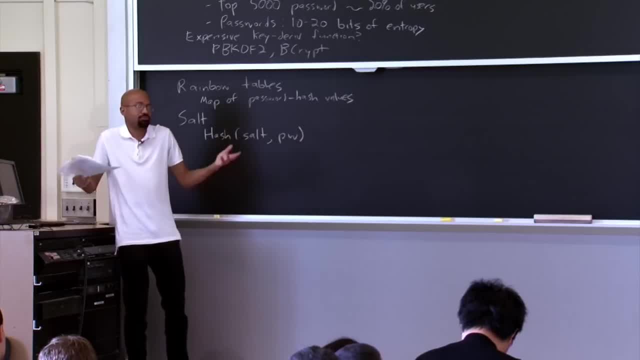 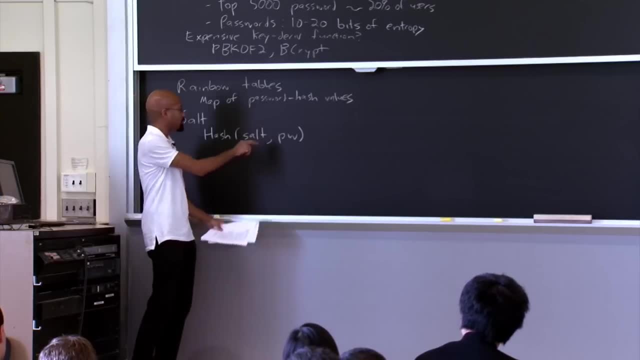 as sort of unique-ifying passwords, even if they're the same, basically. So this is what a lot of systems do in practice. They use this notion of a salt here, And so the best practices for this. so you want to choose a salt that's long. 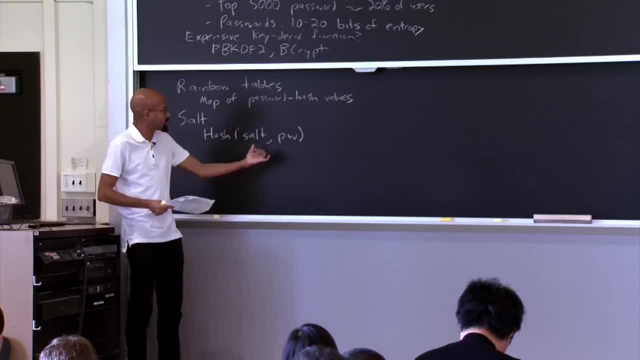 Because you can essentially think of the salt as adding more bits to this sort of pseudo password. So more bits is always better. And the other thing you want to do too is that whenever the user changes his or her password, you typically want to change that salt too. So one reason for that is, let's say, the users are lazy and they want to pick the same password multiple times. Changing the salt will ensure that the thing that's stored in the password database will actually be different, even if that password's the same. 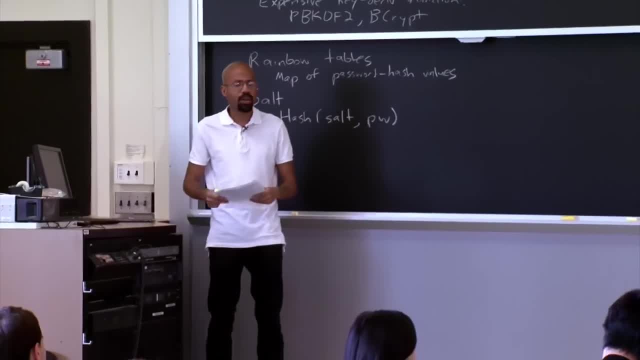 I think there was a question somewhere: Why is it called salt? I'm actually not sure why it's called salt. That's a good question. I'm sure there's some answer to this, though It's like: why are cookies called cookies? 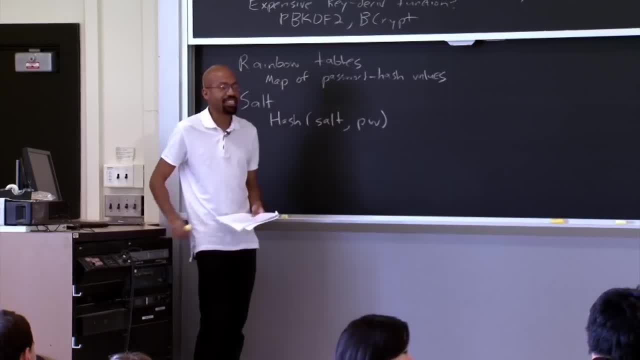 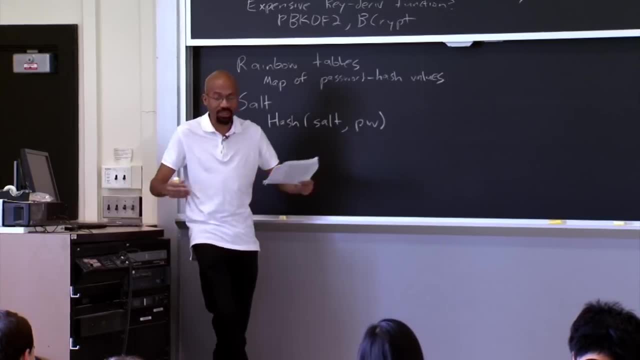 The internet will know, But I actually don't know. It does add some taste to the hash. The hash is interesting. If something is salt, you know. There we go. I'm glad that we're getting this on film because I feel this is how we're going. 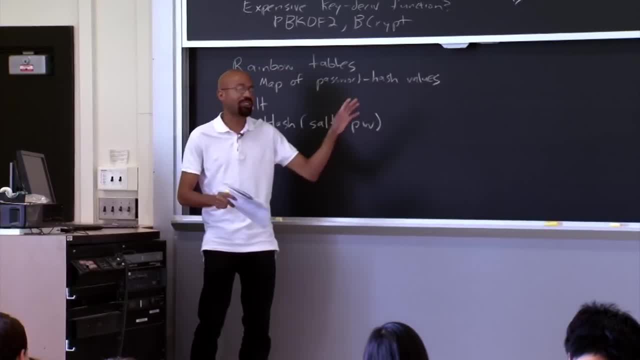 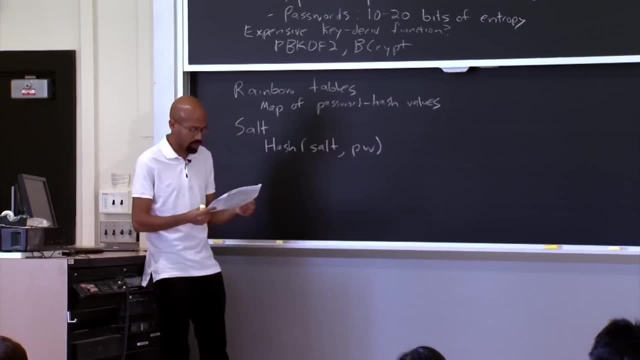 to get our Turing awards. That's right. So yeah, I'm sure there's some answer out on the internet, So I'll look that up later. But does that all basically make sense? OK, so these approaches are fairly straightforward. All right, so what I've assumed so far. 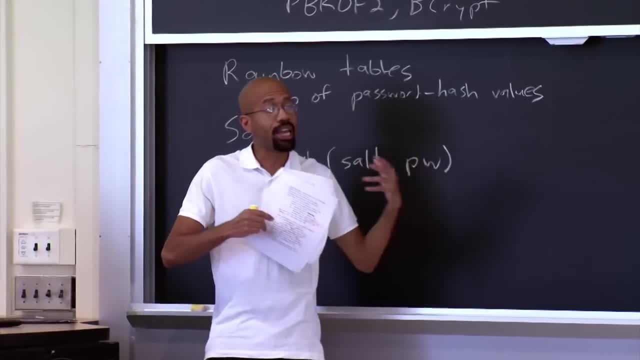 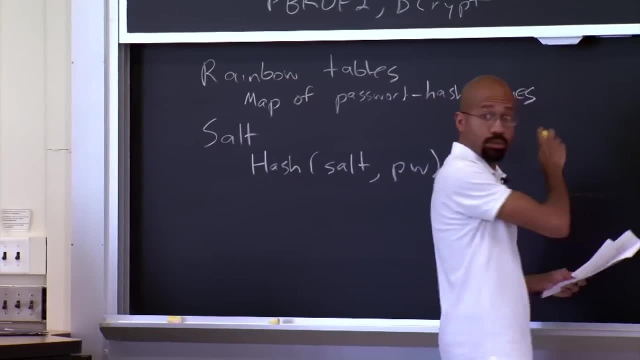 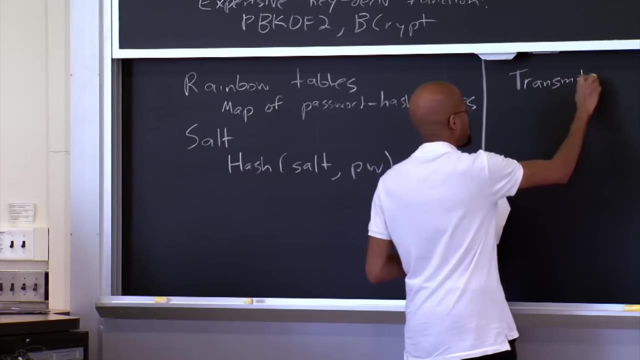 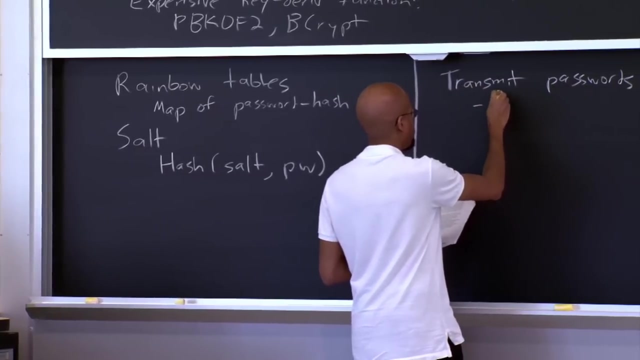 is that somehow the client is transmitting the password to the server, But I haven't actually specified how that transition's actually going to take place. So any questions? No, OK, so yeah, how do we transmit these passwords? So the first idea you might have would be: well, 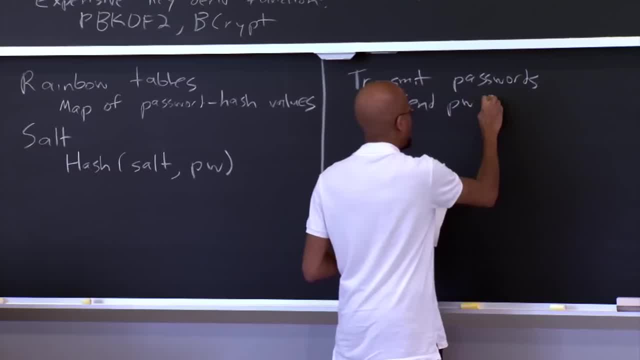 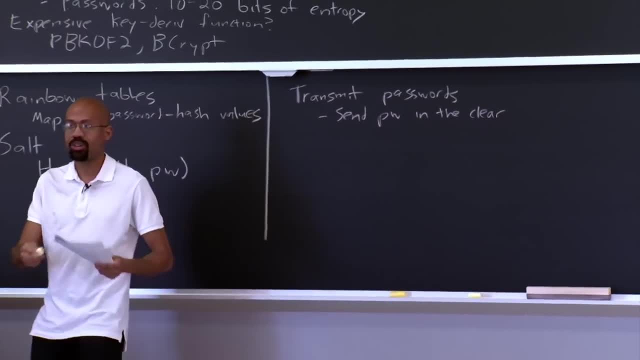 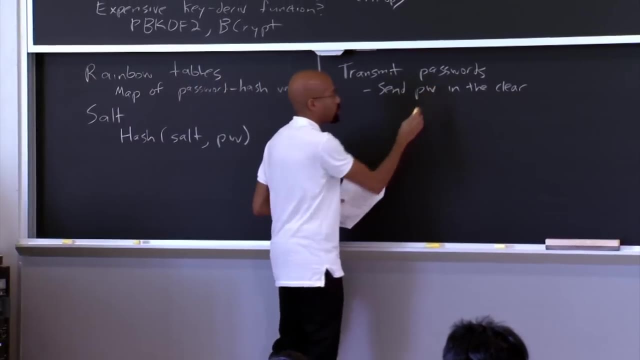 we'll just send the password in the clear over the network. This is clearly cartoonishly bad, because then there could be a network attacker who's basically snooping And seeing the traffic that you're sending and that snooper can just take that password right off. 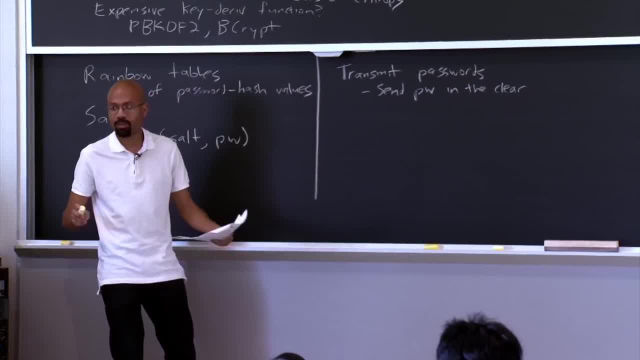 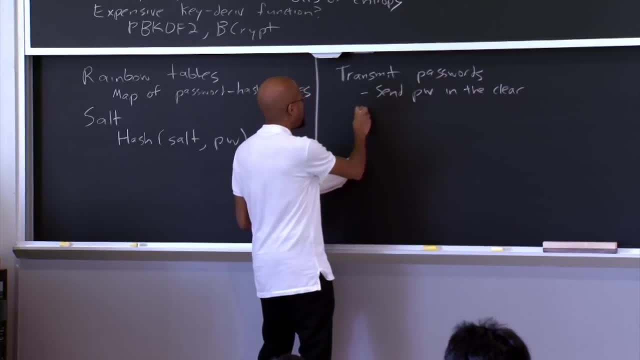 the wire and then impersonate you. OK, so we always start with the straw man before I show you other straw men which, of course, are also fatally flawed. So first thing you think about is sending the password in the clear. Another thing you might think, which? 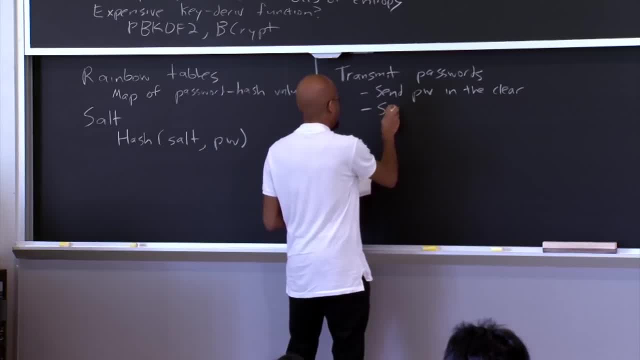 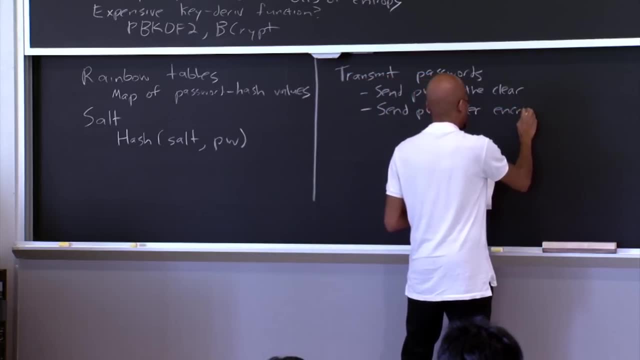 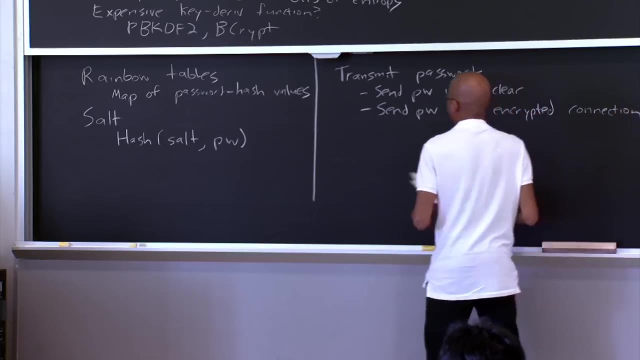 would be a little bit better perhaps, is: perhaps we send the password over an encrypted connection And so we use some type of cryptography here. Maybe there's some secret key or something like that, And that's what we use to transform the password before we. 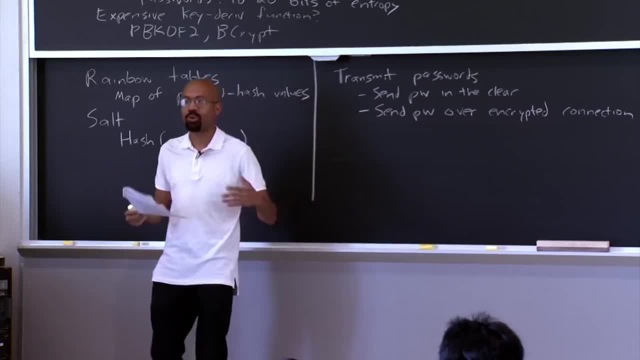 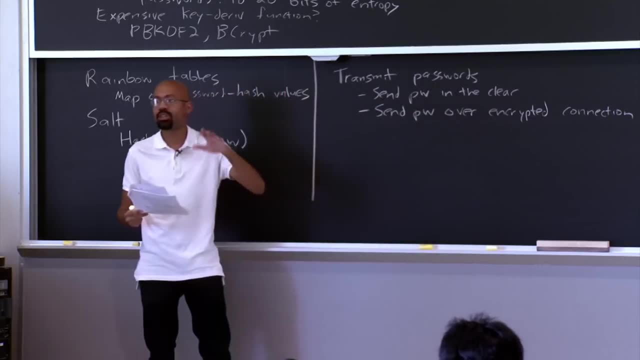 send it over the connection. So at a high level, encryption always seems to make things better trademark. But the problem is that unless you think carefully about how you're using things like encryption and hashing, you may not be getting the security benefits that you think you're getting. 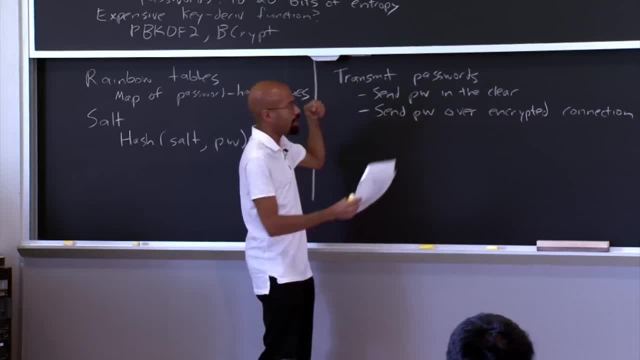 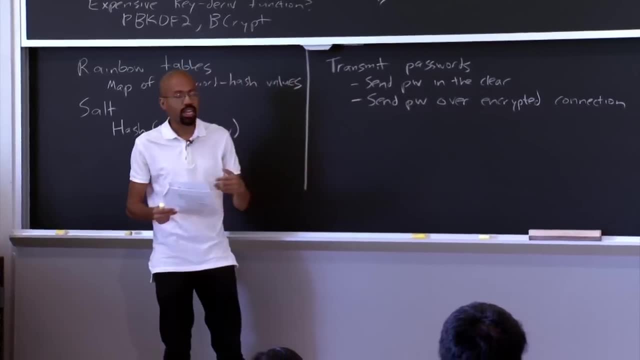 Because, for example, what if there is someone who's sitting between you, the client, and the server, this proverbial man-in-the-middle attacker, right, who's actually snooping on your traffic and pretending to be the server, If, when you send encrypted data, you haven't actually authenticated the other end, then you could still be opening up yourself to problems, Because if the client just, let's say, picks some random key, sends it to some entity on the other side, who may or may not be the server, 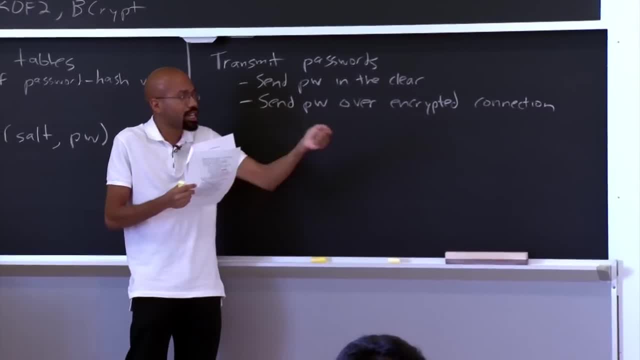 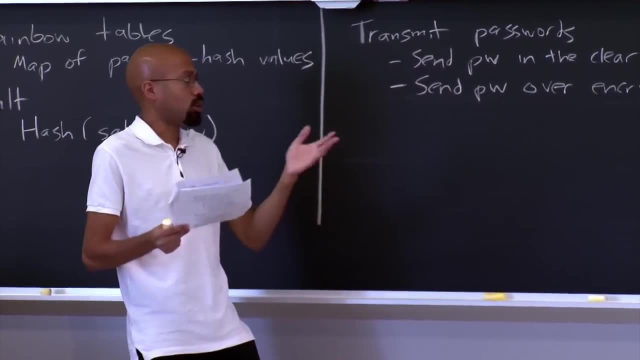 if it's not the server. your encryption didn't really buy you anything. You're sending something to some person who will then be able to get all your secrets, And so, similarly, People might think: oh well, what if I don't send the raw password? 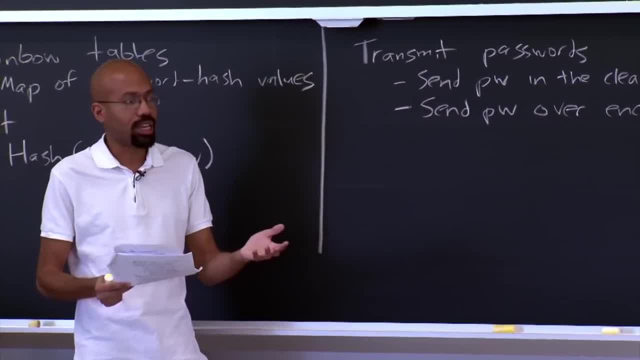 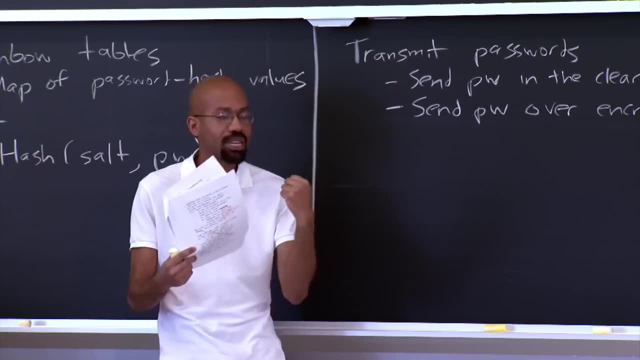 but I send a hash of the password instead. That actually doesn't give you anything in and of itself either, Because whether you send the password or the hash of the password- I mean the hash of the password- has the same sort of semantic power. 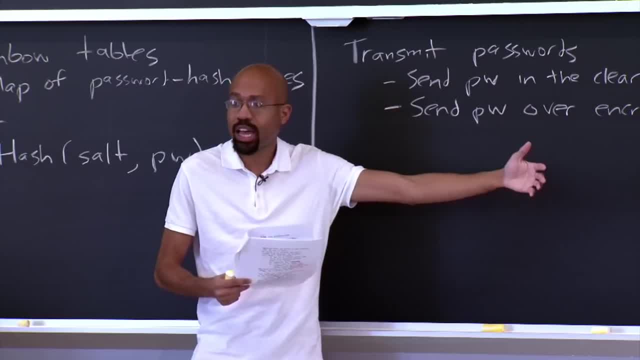 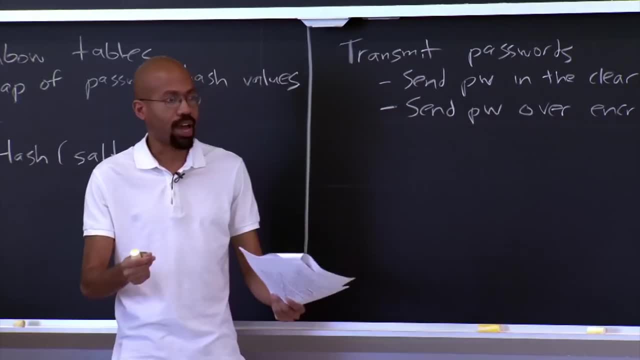 as the original password itself. right, if you haven't authenticated the other side, if you haven't authenticated the server, or things like this. So the basic point with this discussion here is just to sort of stress the fact that just adding encryption or just adding hashing, 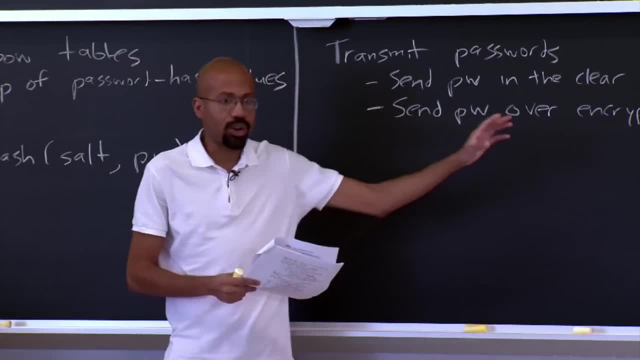 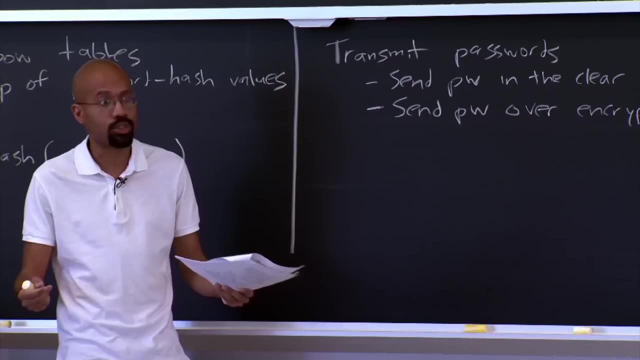 doesn't necessarily give you any additional power, right? If the client can't authenticate who he or she is sending the password to, then the client could be mistakenly divulging that password to someone that they don't intend to divulge it to. OK. 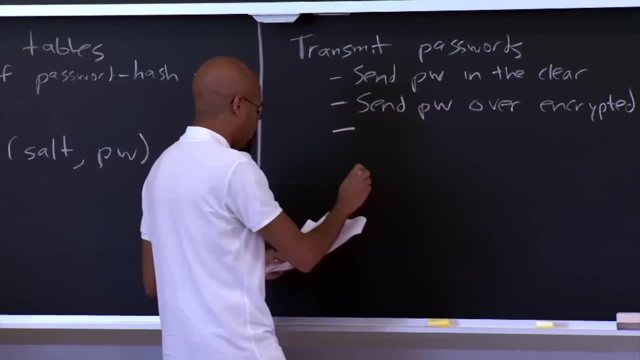 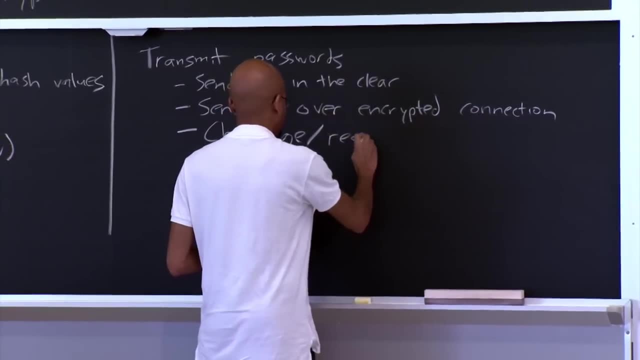 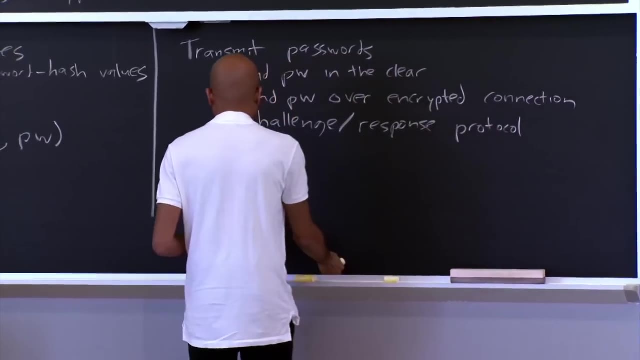 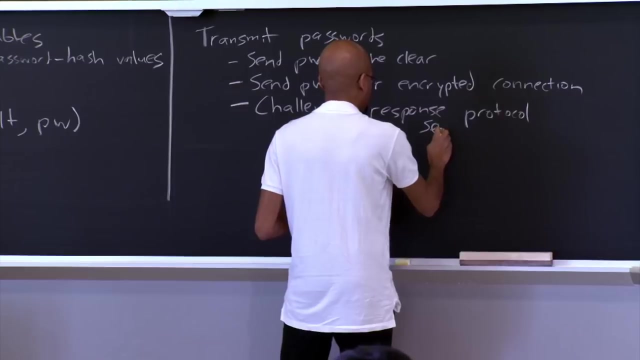 So perhaps a better idea than these two is to use what they call a challenge response protocol. And here's an example of a very simple challenge response protocol. So let's say we've got a server, We've got the client here, And then we've got the server over here. 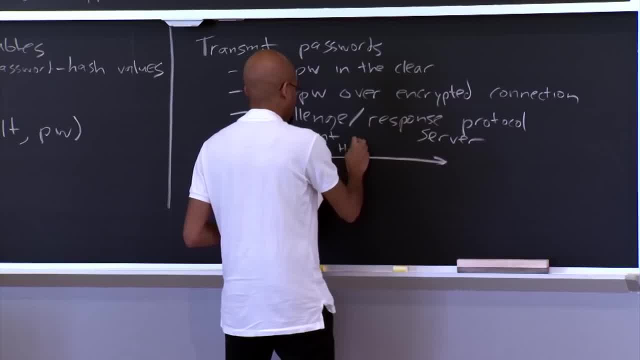 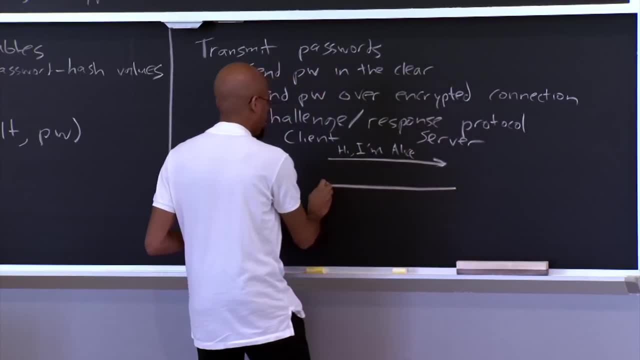 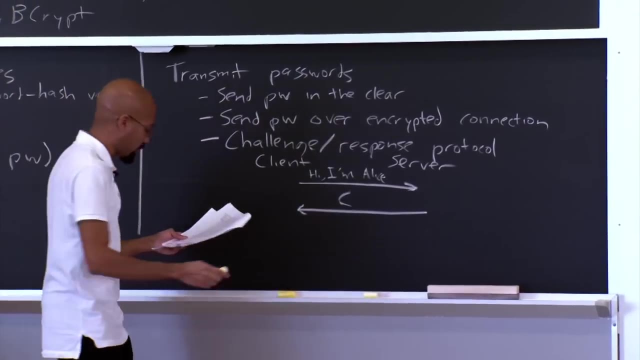 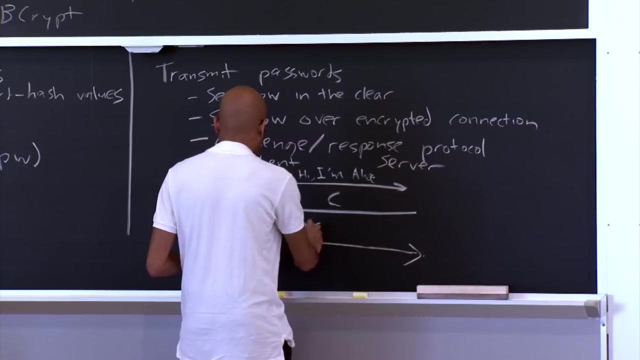 So the client says hi, I'm Alice. And then the server responds with some challenge C right, Some quantity that the server got to pick, And then the client is going to respond. And then the client is going to respond with the hash of that server-sent challenge. 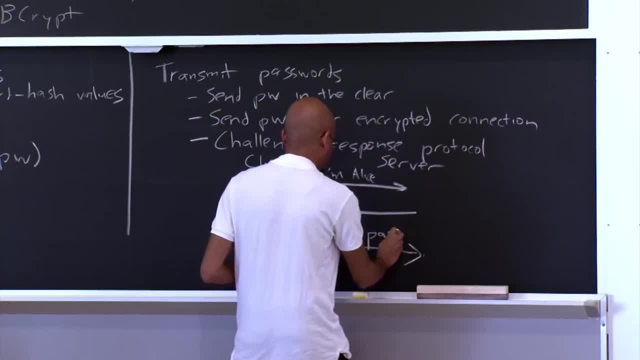 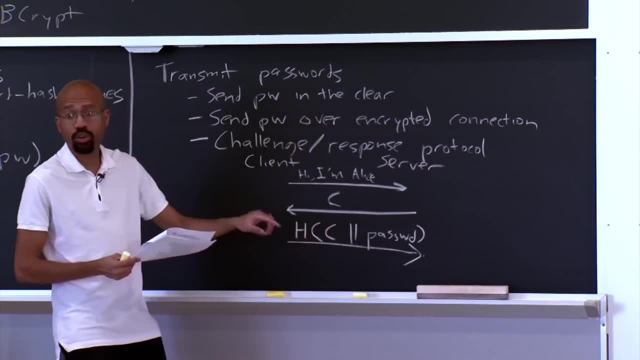 And then you can concatenate that with the password, right? So at this point the server can take this quantity. The server knows the challenge that it sent right, And presumably the server knows the password. So the server can sort of recompute this quantity. 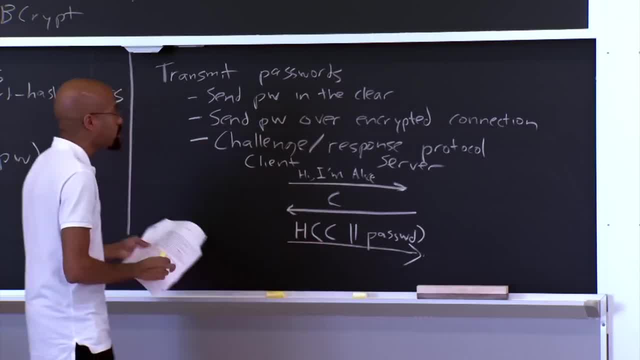 and see if it actually matches what the user sent right. So what's nice about this protocol is that if we ignore man-in-the-middle attacks for a second, the server is now confident that the user is actually Alice, Because only Alice would know this password here. 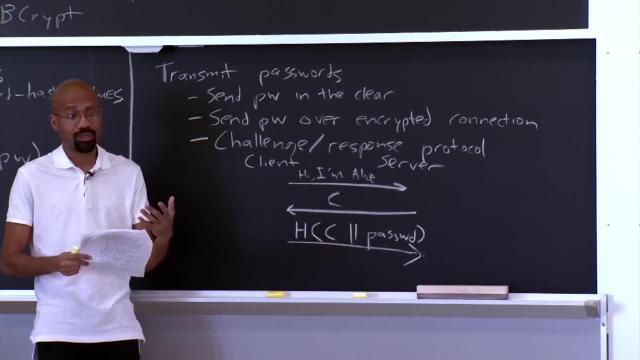 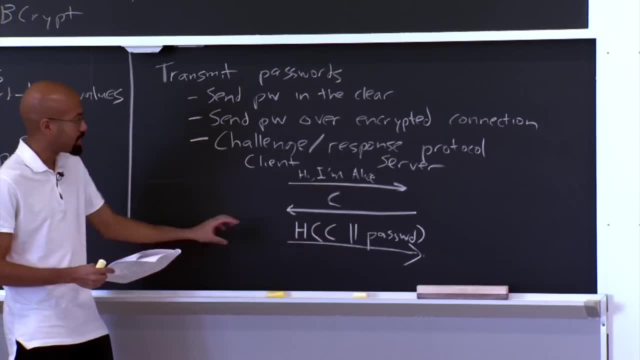 And what's nice about this is that if the server is actually the attacker, right? So in other words, if Alice sent this thing to someone who's not the person that she's trying to authenticate to, then the attacker still doesn't know the password, right? 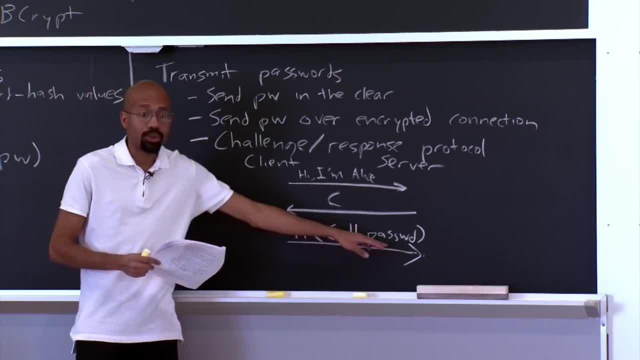 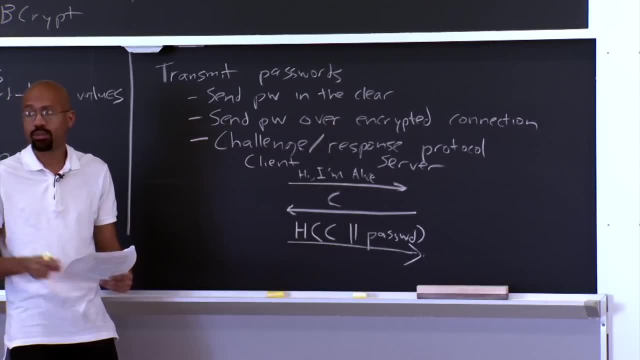 Because the attacker got to choose C. but the attacker doesn't know what this is, And so, basically, for the attacker to figure out what the password is, the attacker would have to be able to once again sort of invert these hash functions right. 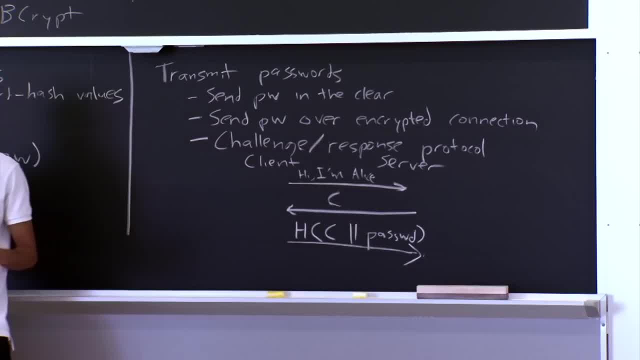 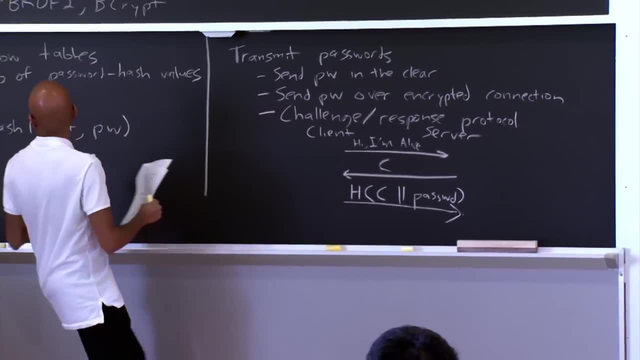 You have a question. I'm just curious: How come you don't make the client do the hashing? How come you don't have a script and make it do pd, pdk, df2, hashing Also, if you're still using the server. 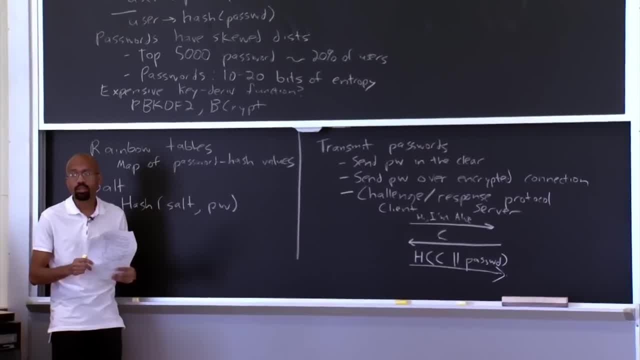 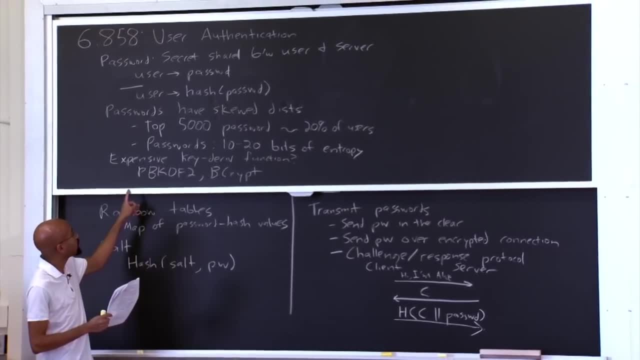 And also, that way the server definitely doesn't know what the password is. So it's an extra perk that you gain. So let's see. So your proposed scheme is that the client side is going to call this thing. Yeah, So instead of sending the password, 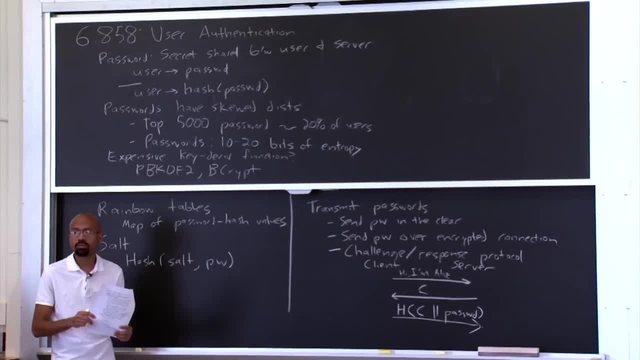 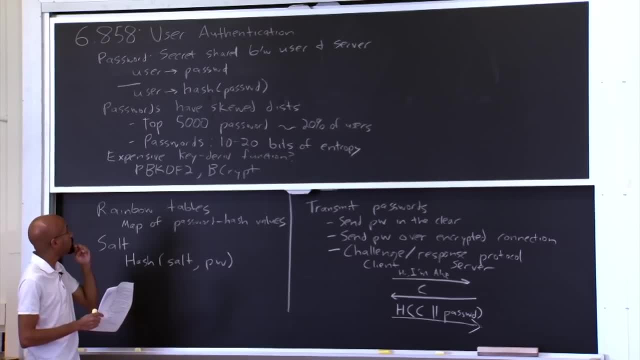 and then having the server hash the password to check it. you'll just- the client will just send the hash password. The client will just send the hash password. So one thing you want to keep in mind is that you typically well. so there's a couple of reasons. 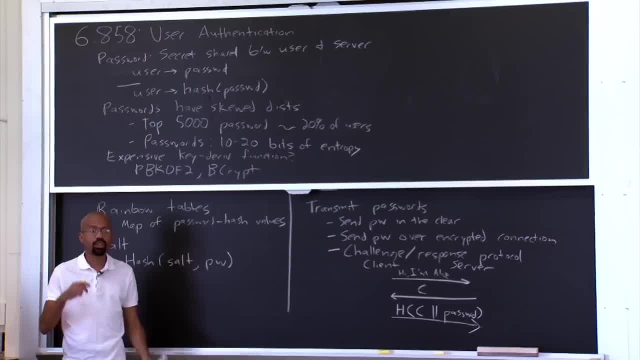 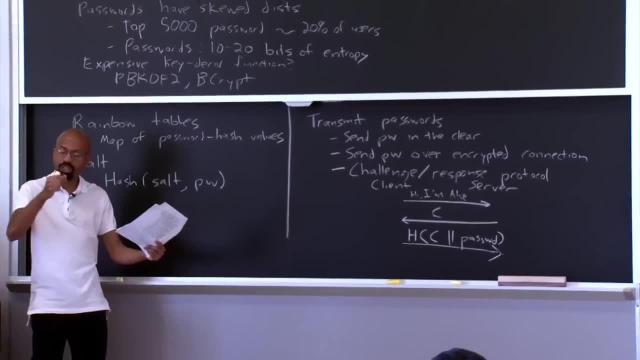 So one reason- as we'll discuss later- is that there's going to be these things called anti-hammering defenses. right, Anti-hammering defenses are designed to prevent sort of like a bad client from continually asking: is this the password? 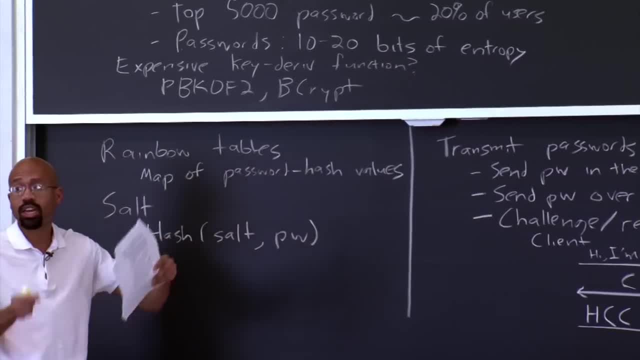 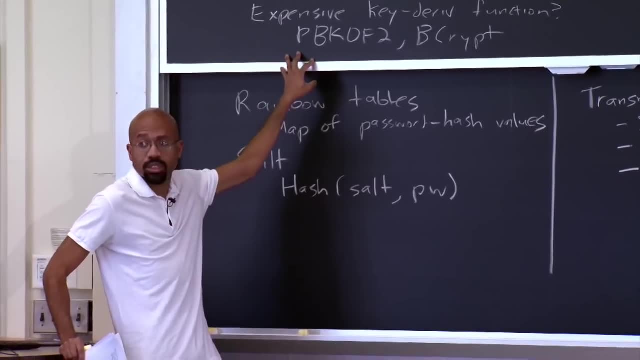 is this the password? is this the password? Sometimes, as a result, it's easier for things to be done on the server side as on the client side, But suffice it to say that you can in fact do the hashing on the client side using JavaScript. 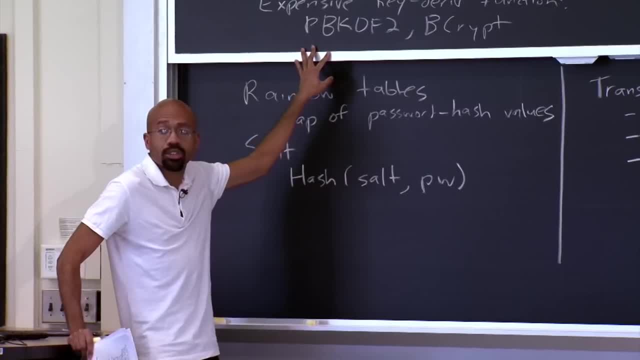 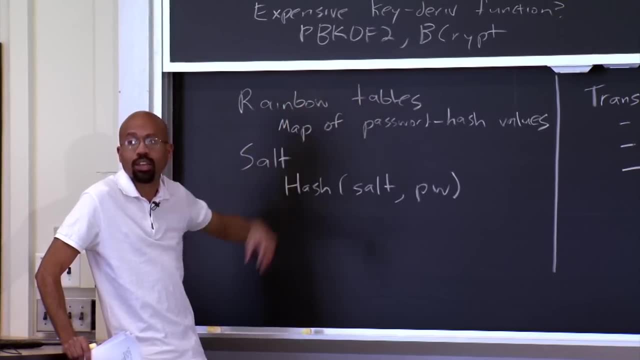 or something like this. But the basic idea is that somehow you have to have the computational expense be very, very large, Because that's going to prevent the attacker from just guessing sort of what the password is quickly. Do you have another question? Well, I just wanted to point out: 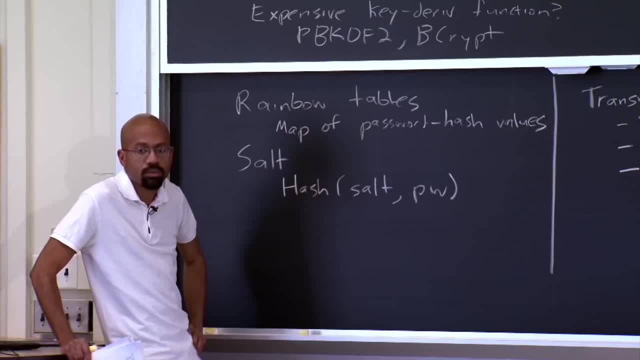 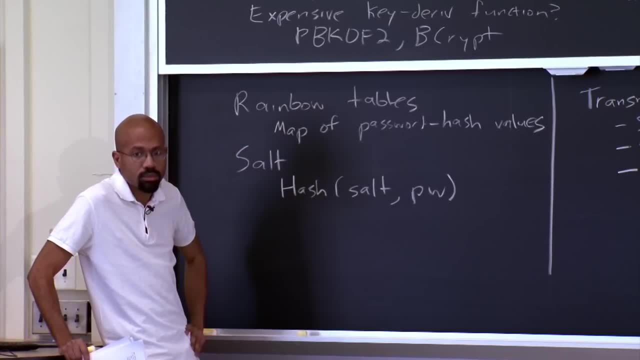 that if the client does the hashing, then it is. if you're not doing hashing Because your password is the hashing, So that's true, right? So if someone gets the sort of table from the server of all the usernames and hashings, 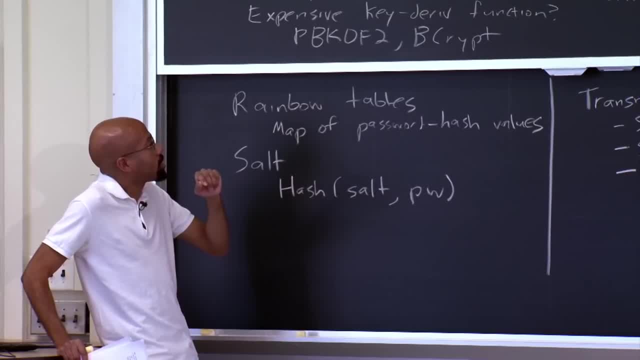 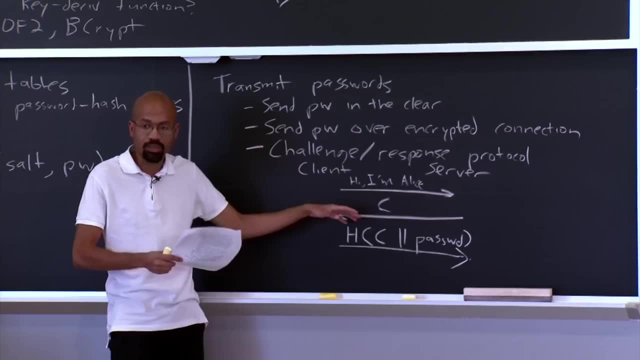 they can log in. That's right. That's right. Yeah, It gets a little bit subtle sometimes depending on who can pick, for example, these challenge values. right, Because if clients and servers can pick challenge values, sometimes that makes it more or less difficult for the client. 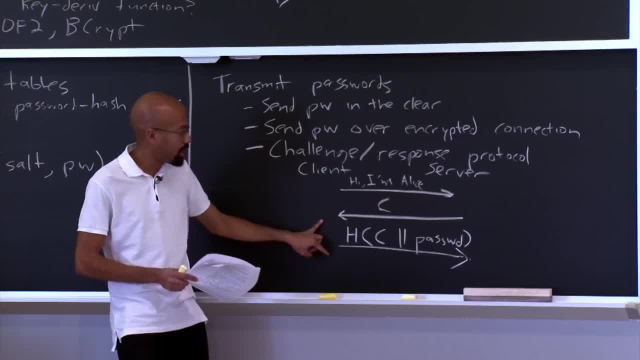 to launch those types of attacks. So, for example, like one problem with this protocol here is that basically the client doesn't get to inject any hash, It doesn't get any randomness into this. So you can imagine that we can make this protocol more. 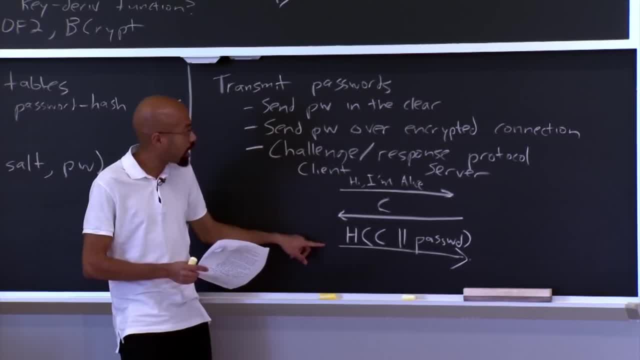 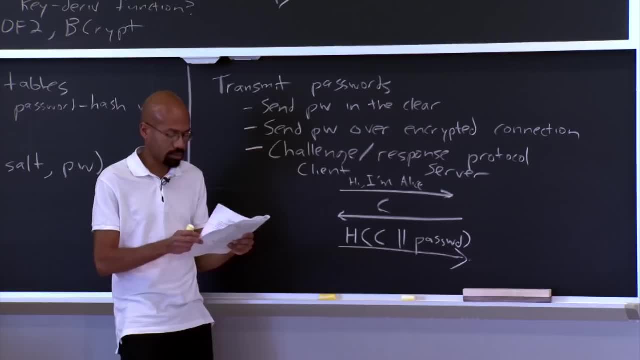 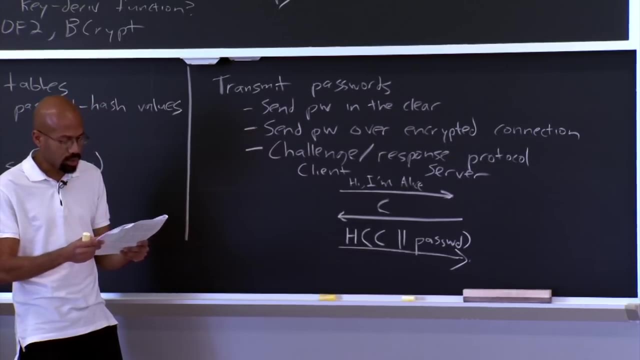 difficult for the server to invert if the client actually got to choose some challenge. that was put in here. So you have a server-side challenge versus a client-side challenge. But you're right about that. Any other questions? OK, So this segues into the discussion we were just having. 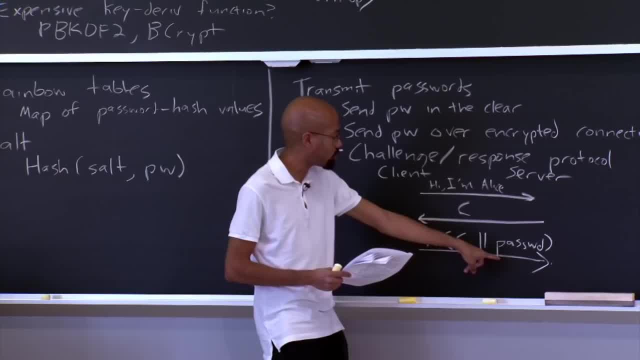 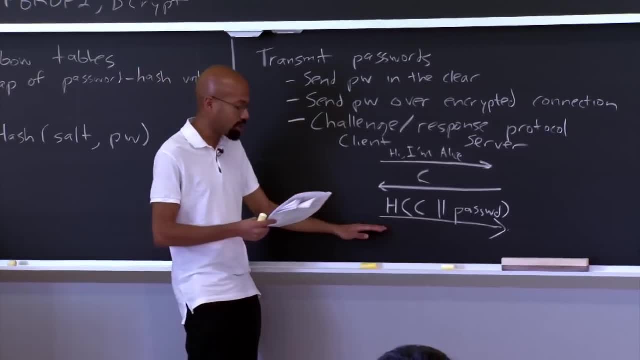 So even though to break this there is, the server would have to invert this hash, the attacker could still try to do one of these brute force attacks. So one way that we can prevent the server from doing these brute force attacks is to choose one of these expensive hash functions. 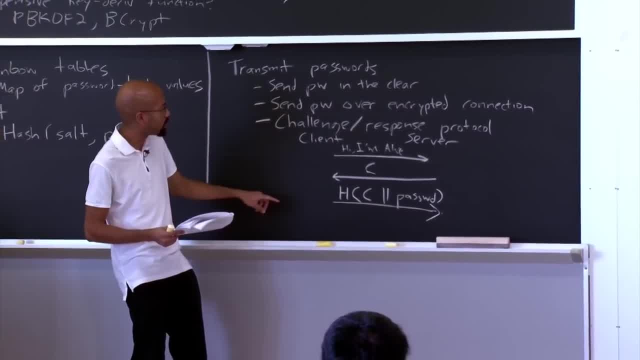 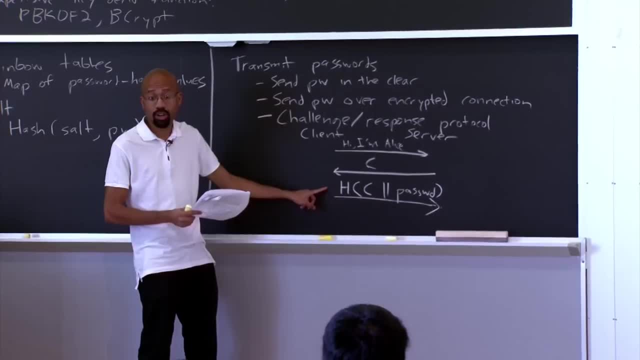 kind of like we were discussing before. Another thing, as we just discussed, is that you could actually allow the client to, for example, choose its own client-chosen challenge over here, And so that essentially would act as a client-chosen salt. 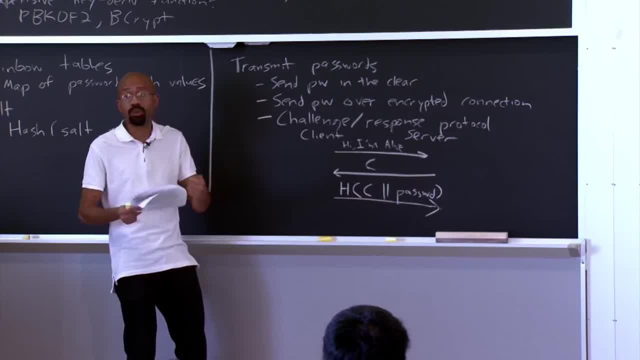 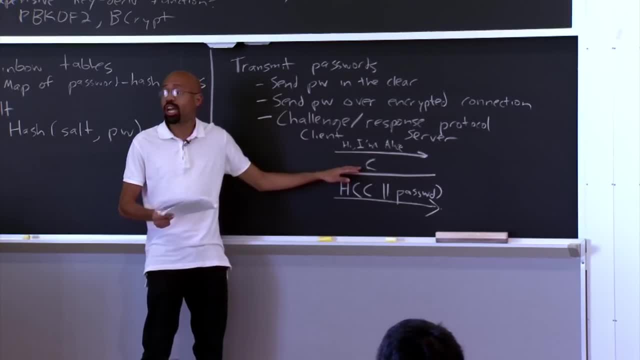 So that would essentially make it more difficult for the hacker to do things like build up a range of rainbow table, Because- note that if the server is the attacker here, the server always can pick the same challenge value again and again and again, allowing to build up a rainbow table. 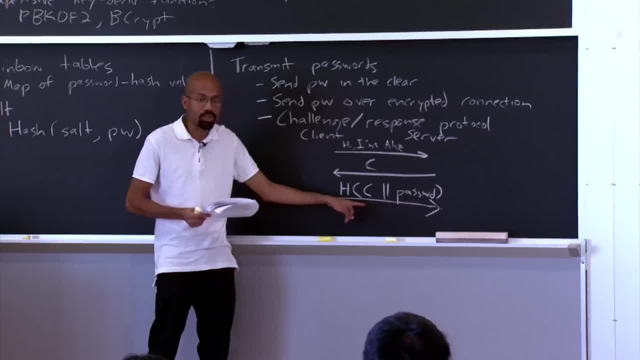 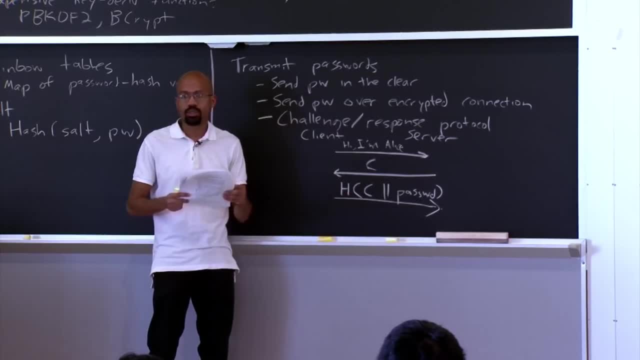 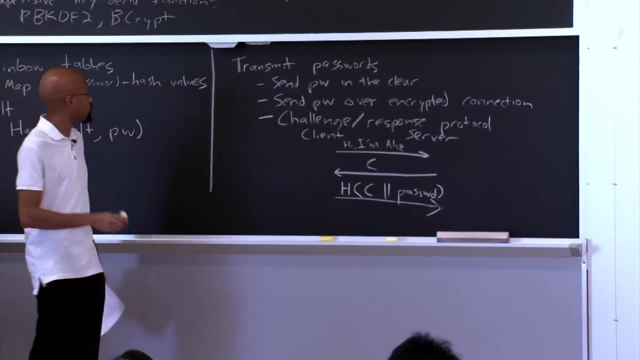 But if, when the client responded back, the client also included some salt, some client-chosen challenge that it included, then that would prevent the attacker from building one of those rainbow tables. So does that all make sense, OK, So yeah, so one thing that I mentioned. 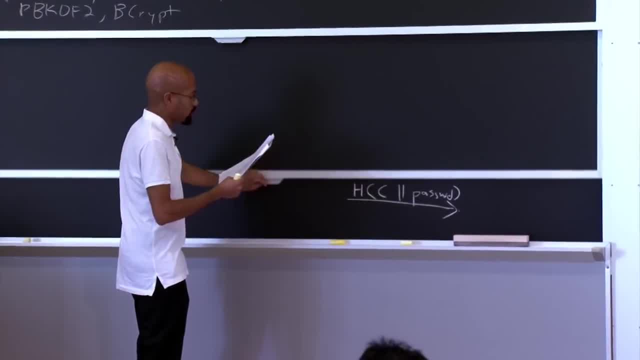 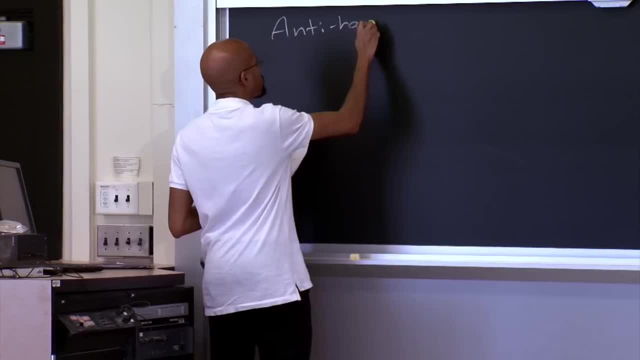 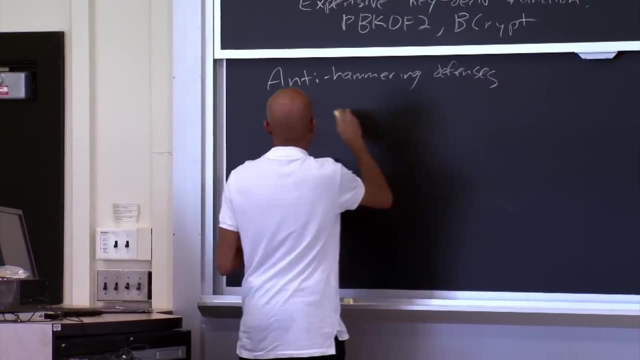 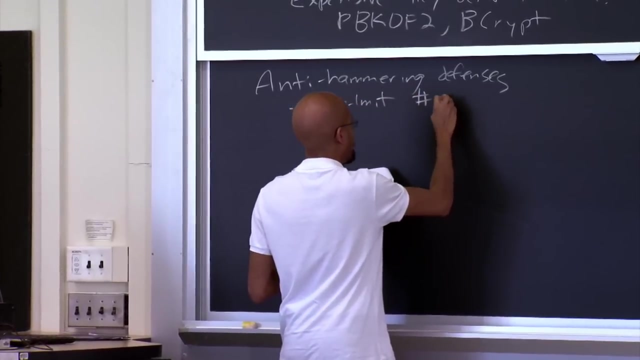 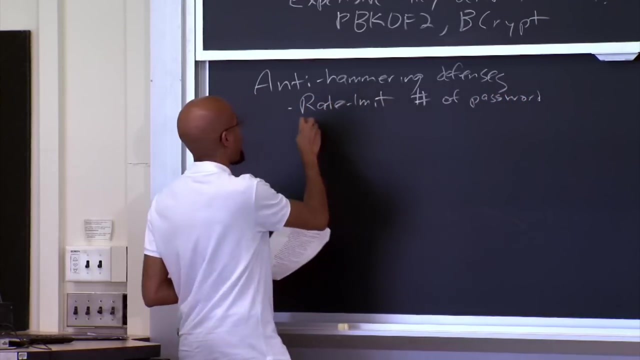 is that might be useful to do is implementing these anti-hammer defenses, And so anti-hammering defenses are basically designed to rate, limit the number of password guesses that say Sort of a bad client can issue. Because the idea here is that if you've got some client who's trying to launch one of these root-force guesses against a password, you don't want that client to be able to sit there in a tight loop and just say: is this the password? 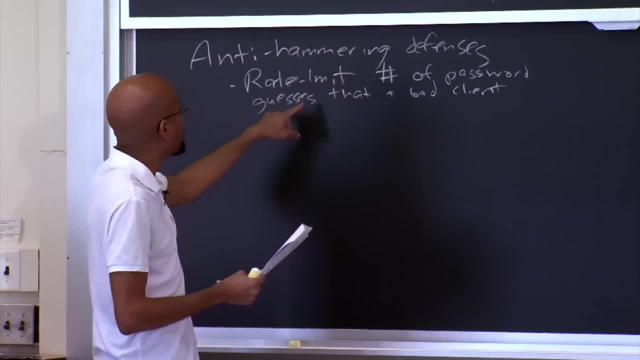 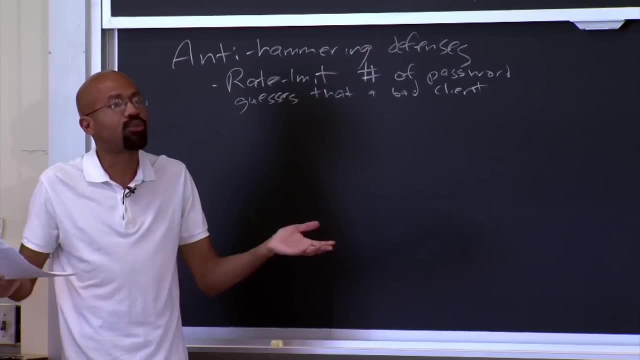 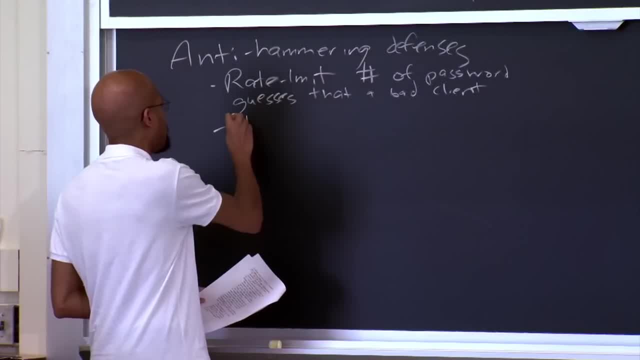 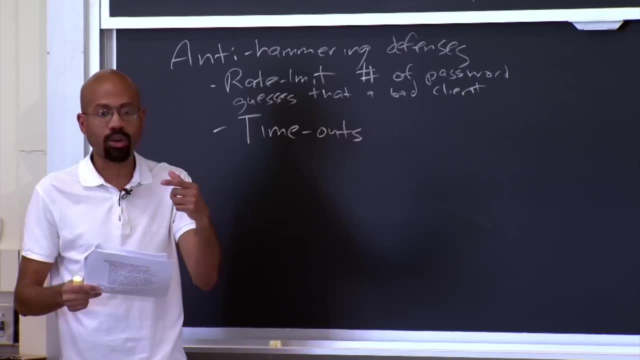 from any particular client. You could also imagine implementing timeouts here, So maybe the client can issue a bunch of password requests in a row, but then, after, let's say, 10 of them are wrong, the server says: OK, you've got to hold on. 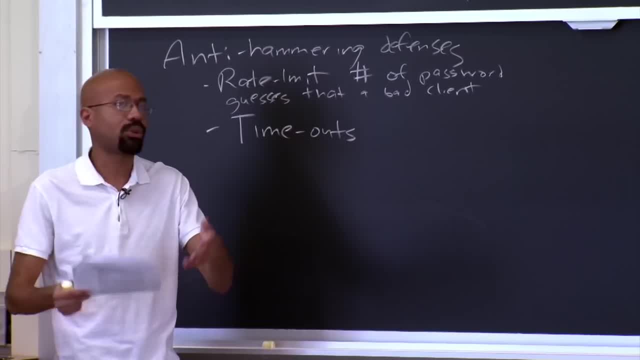 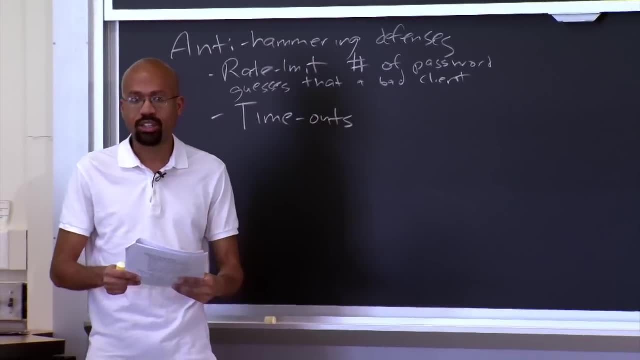 I will not accept any more requests from you for, let's say, 10 seconds, something like that. And so both of these things are designed to prevent against brute force attacks, And so, for example, some smart cards have these types of defenses. 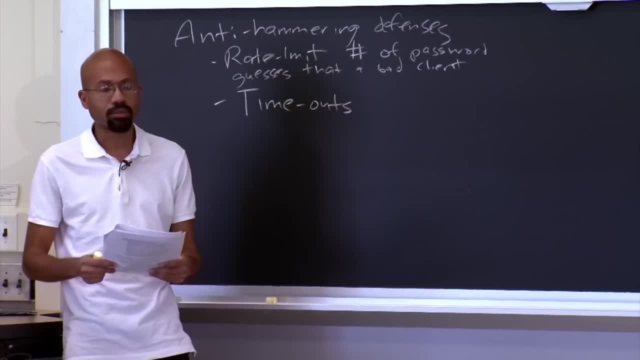 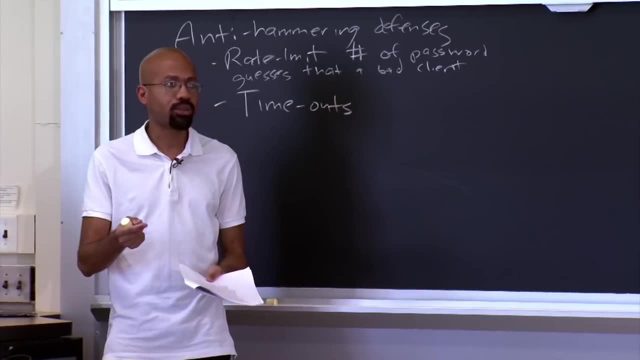 Some TPMs have these kinds of defenses to basically stop against this brute force attack. So why is it important to use these anti-hammering defenses? Well, one reason why it's important is, as we've discussed, these passwords have so little entropy. 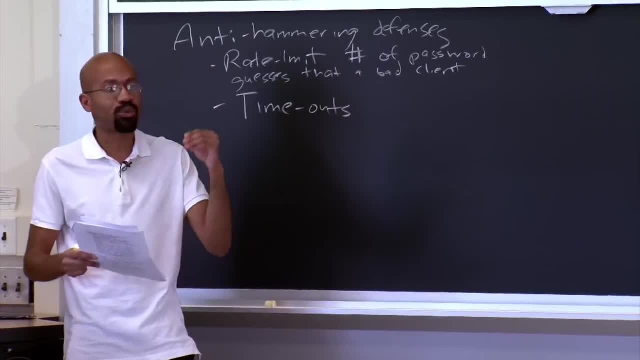 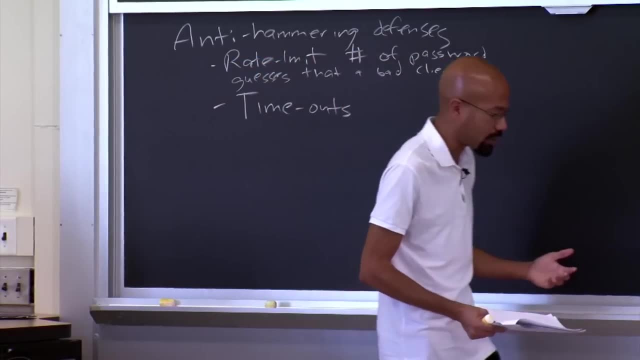 So, because passwords typically have so little entropy, it's really important to prevent the attacker from just trying to cycle through that low entropy space very, very quickly. So, as you may be aware, a lot of websites have these formatting constraints that they've 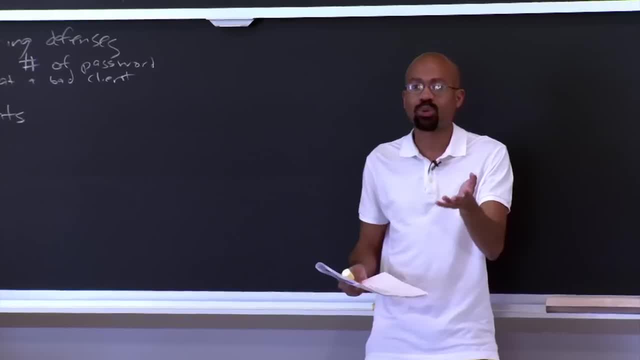 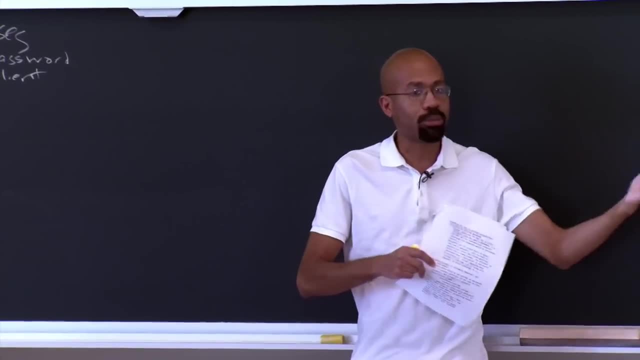 And they push upon you for your passwords. They'll say things like: oh, your password must have an unprincipled character, But it must have a punctuation. It must have a mixture of numbers and letters. You must have uppercase and lowercase stuff. 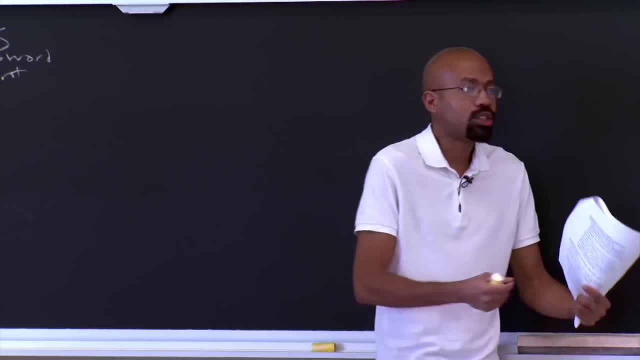 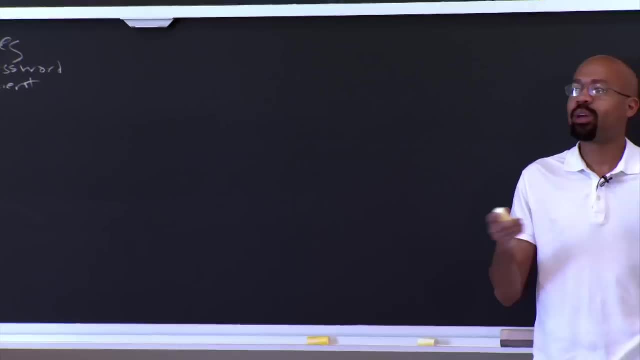 so on and so forth, And so what those constraints are trying to get you to do is they're trying to get you to expand the entropy of the password, But what's problematic, though, is that it's not really these formatting constraints that we 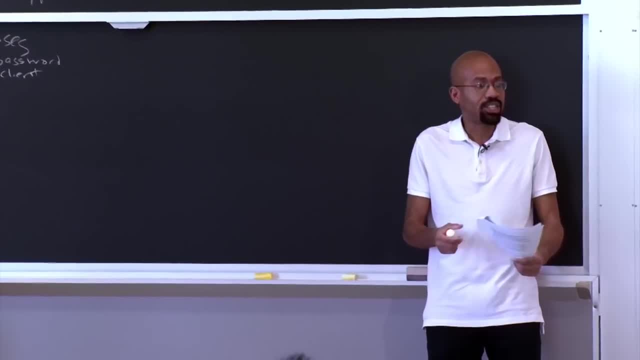 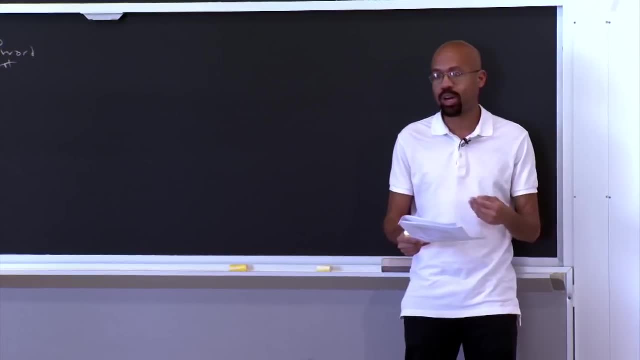 should be caring about, It's the actual entropy of the password itself. So, as it turns out, even if people are given these constraints- like you have to use punctuation characters and stuff like that- the entropy of the resulting passwords is often quite low. So, for example, people often put punctuation at the beginning or the end because they don't want to be troubled to remember: do I have a dollar sign in the middle of something? And so, as it turns out, these formatting requirements oftentimes don't make dictionary attacks much harder. 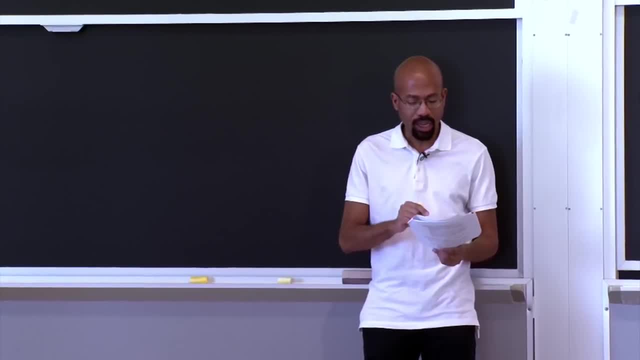 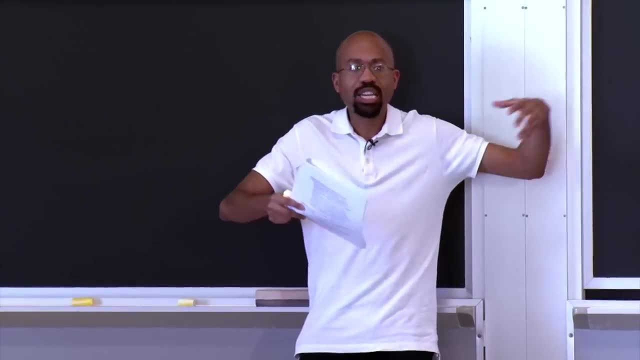 for a sophisticated adversary. The reason is because, basically, the dictionary attacker can leverage these observations, These observations about how people pick passwords, even in the presence of constraints. So, for example, if the attacker knows that people typically put punctuation at the beginning or the end, just 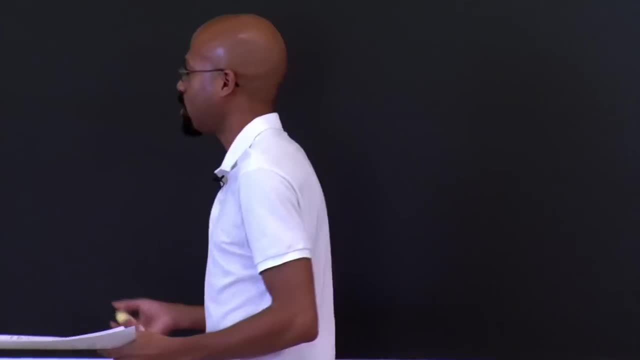 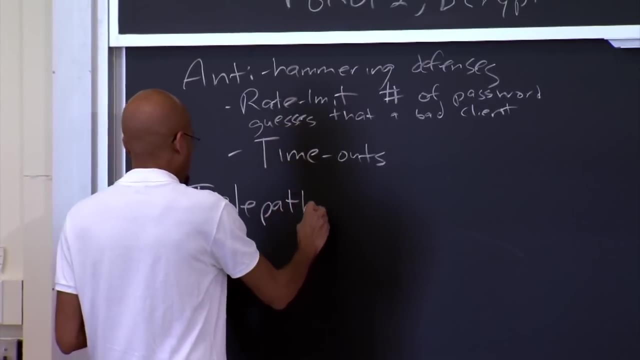 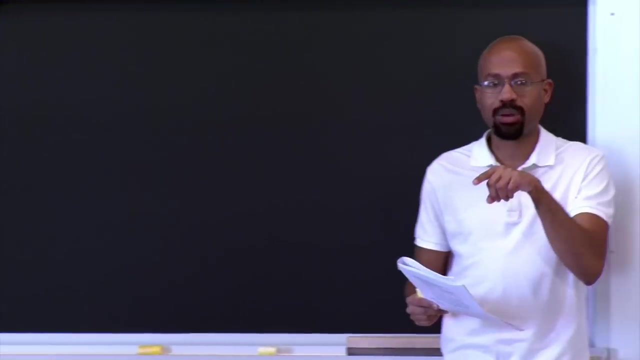 incorporate that into your dictionary attack, And so there's actually a really interesting website you can go to. that's called telepathwords, And so what's neat about this site is that it has a little text box. You can type a character into that text box. 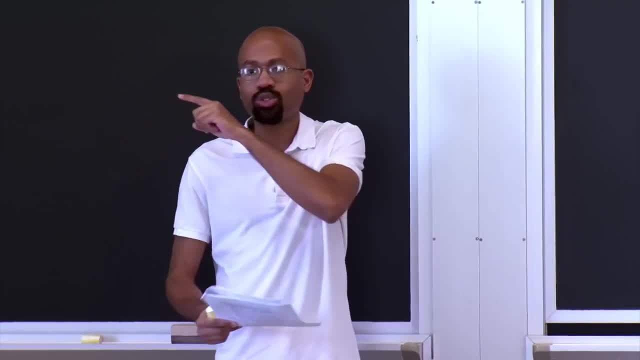 You know you're pretending that you're entering in a password And telepathwords will try to guess what your next character is right, And so as you type additional characters, it'll have a little drop down box which says: 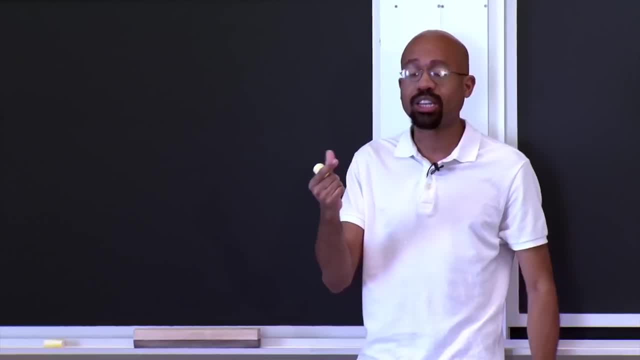 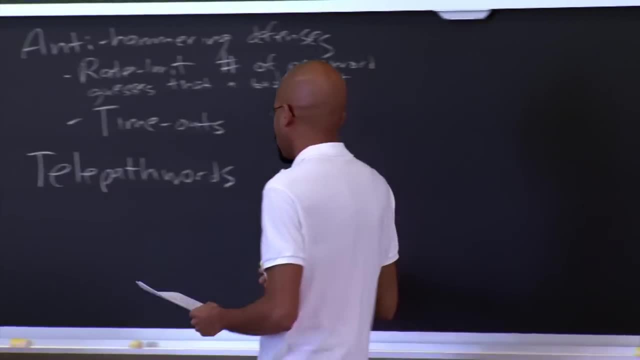 where are you going to put this? Where are you going to put this? And it'll give you a little blurb that says: here's why I think that you were going to enter this next password. So how does telepathwords work? So it basically has a bunch of databases, right? It has a database of common passwords. It also has a list of popular phrases And it has a list of common phrases And it has a list of common phrases And it has a list of common phrases. 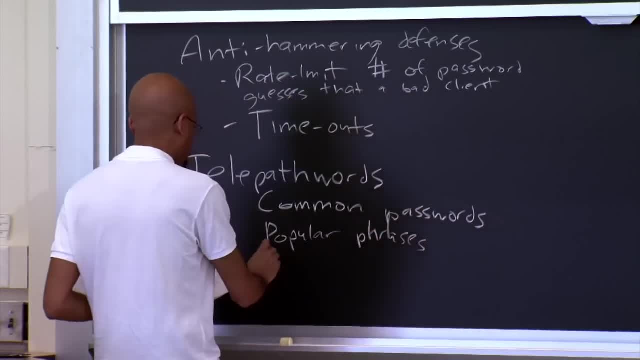 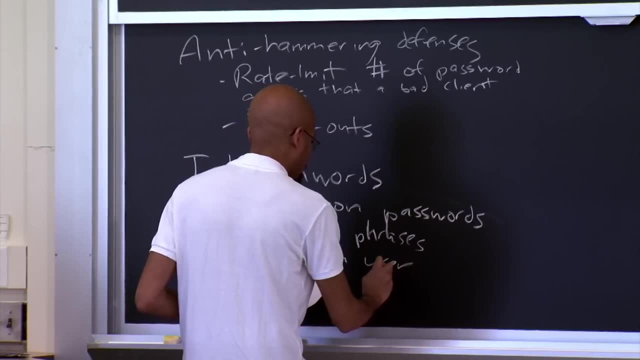 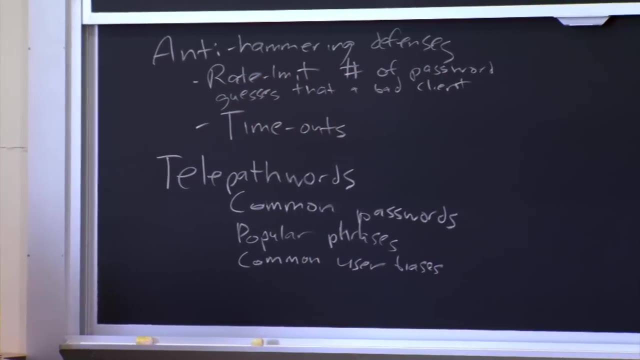 That it's taken from websites And it also has this set of heuristics which describe common user biases in picking passwords. So, for example, one funny bias is that people will often like, when they're forced with these constraints, to say: you must use punctuation, and stuff like that. 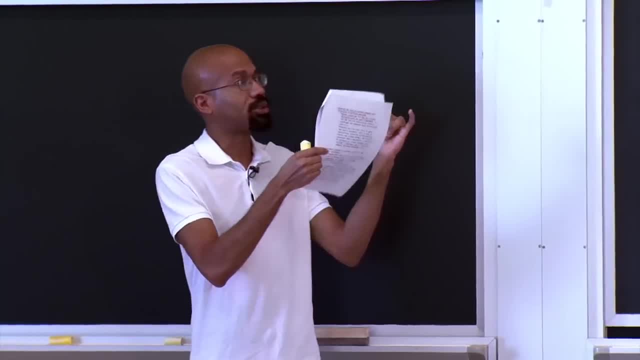 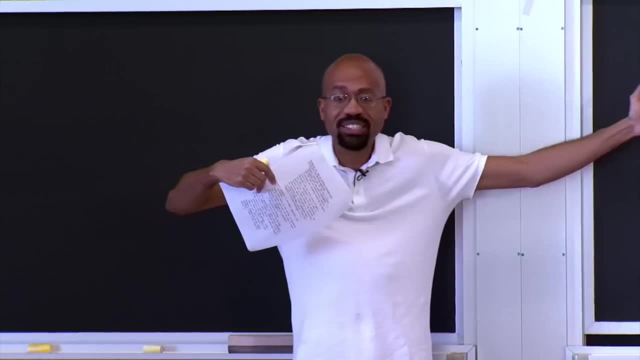 a lot of times they will. when they're picking characters for the password, they'll use keys that are adjacent to each other, So in other words, they'll be very small edit distance in physical space with respect to edit distance sort of in the actual password itself. 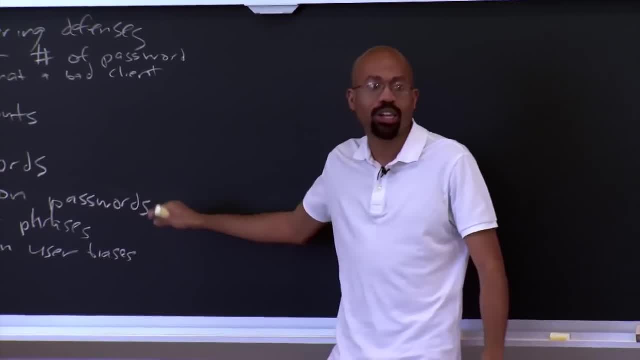 So what telepathwords does is it has this big database here. So when you type in things, it's running these models And it's saying, statistically speaking, here's the most likely thing that you're going to type next. It's almost like autocomplete for passwords. 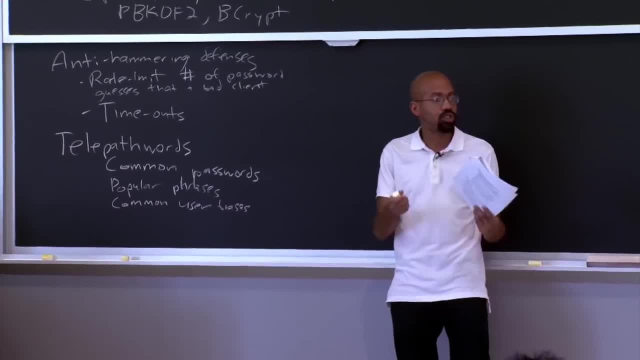 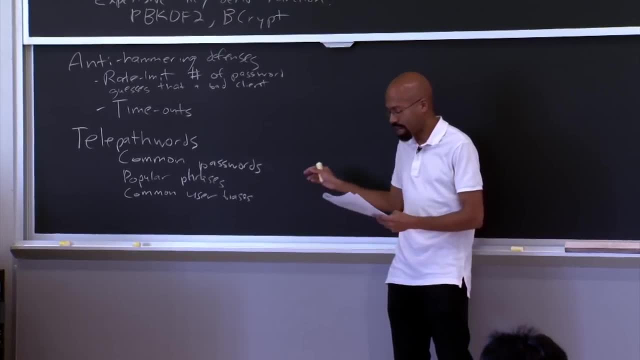 And so what's funny is that this shows once again that if you have these constraints, they actually don't protect you that much, if there are still these underlying sort of a priori distributions of things that the attacker can leverage. I think there was a question. Oh yeah. So it seems like if an attacker is too sophisticated, if they could try guessing like, do users pass it through a bunch of IP addresses and things, And it only would sort of prevent hammering in this case, if you just need to have like a global rate limit on password. 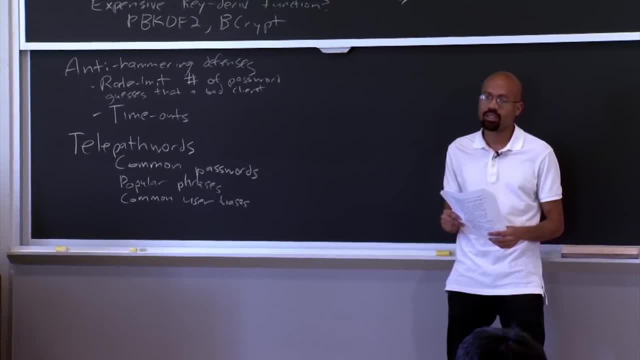 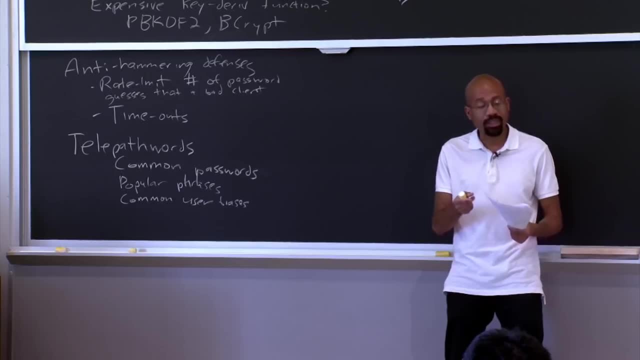 for two users. Yeah, You can have like this issue of like a DOS possibility, users and whatnot. So how do you like balance? Yeah, it's very tricky. Now, that's a good point. So anti-hammering, I mean, basically it's. 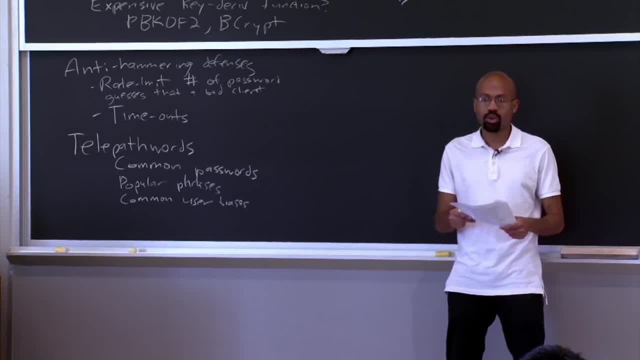 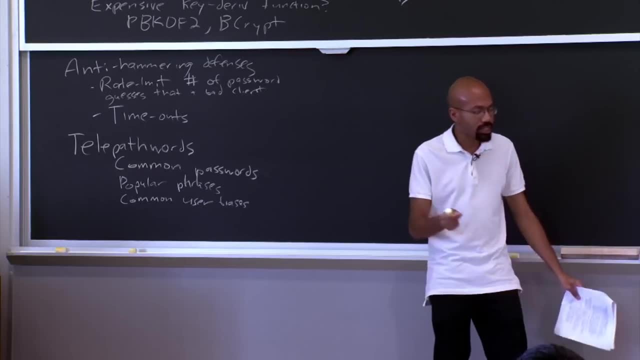 down to what's the scope of the attack that you're trying to prevent, right? So if you're concerned about sort of distributed attackers and sort of a network system, it does become very, very subtle, And suffice it to say that the notion of anti-hammering 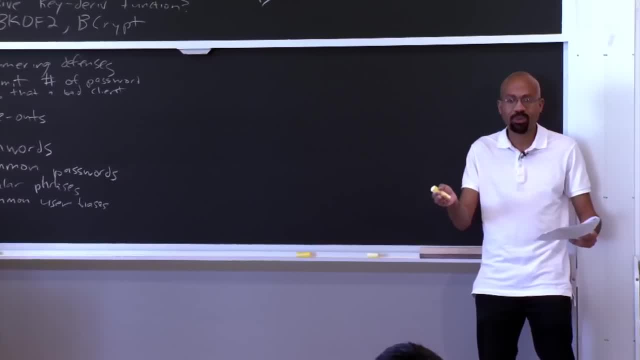 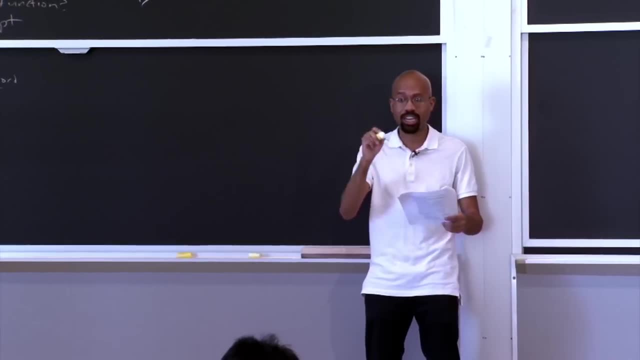 and distributed systems and also the notion of things like, let's say, click fraud, for example. so, in other words, how does someone who's running an advertising campaign online determine if someone's actually clicking the link? and I should actually be paying someone for those clicks. 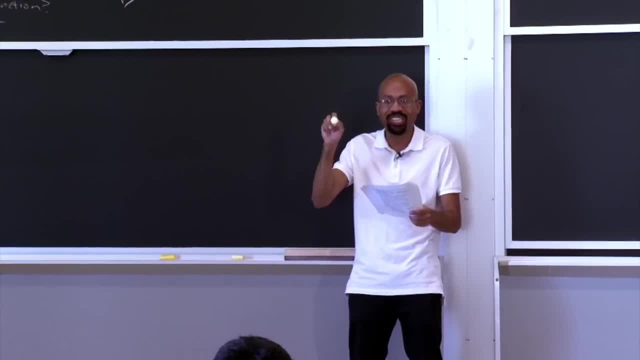 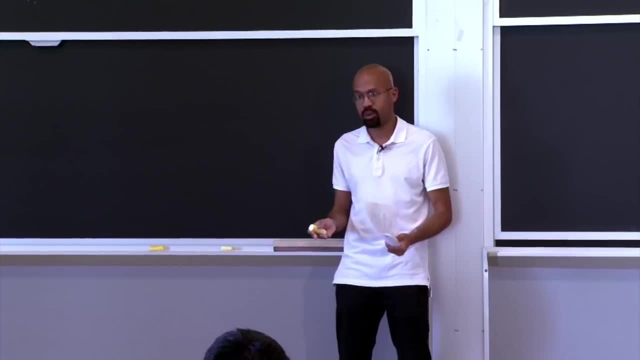 versus. this is just some spammer who's got some bot that's just sitting there clicking on stuff, right? So suffice it to say there's a lot of distributed heuristics that try to solve those problems, And in many cases it's not a science, it's an art. 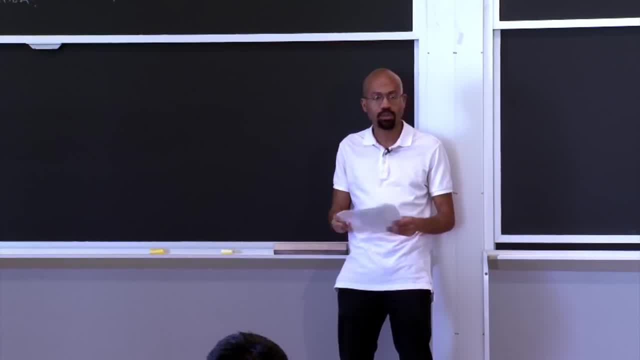 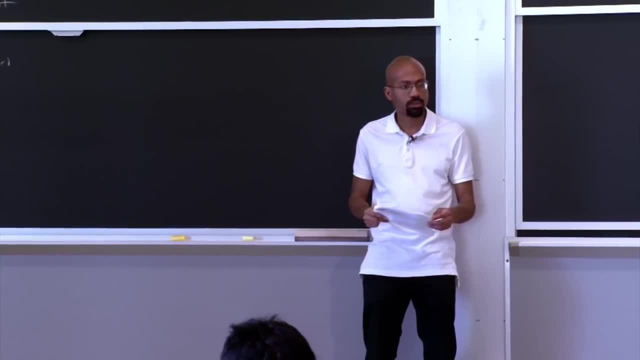 But you're exactly correct that in a distributed setting, things get much more difficult. All right, so does this all make sense? Yeah, What about the cryptographic anti-hammering defenses? Most of the time, you end up sending a hash on the line. 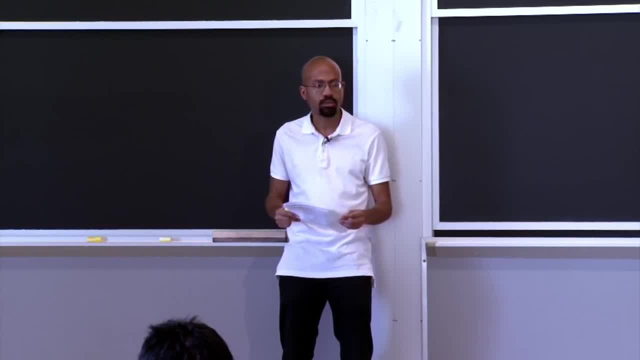 and this hash is pretty high rate and what you get out of it is exactly what you need. You get either the password or the hashable password. So is there? I know there are protocols like SRP or there are some zero knowledge protocols. 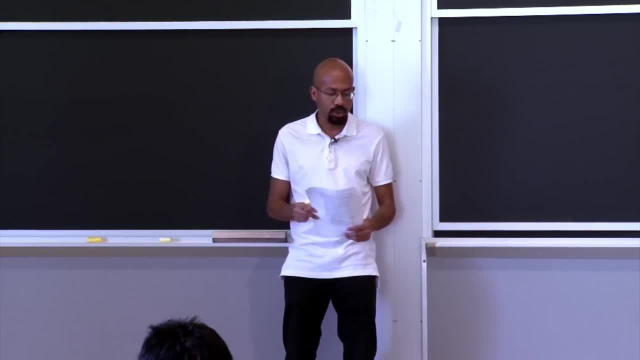 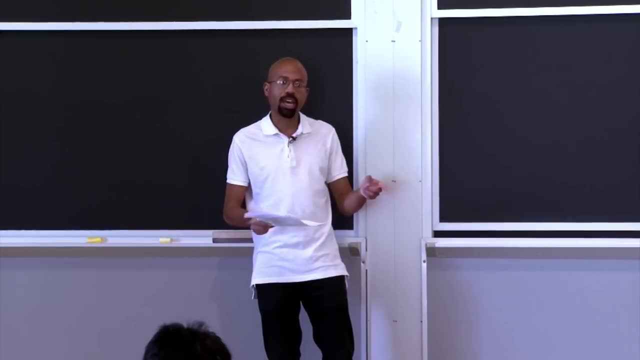 Yeah, so they do. Those things are. so, yeah, those protocols provide some stronger cryptographic guarantees. A lot of times they are not backwards compatible with current systems, which is why, in practice, you don't see them used a lot. But yeah, so there are some protocols, for example, 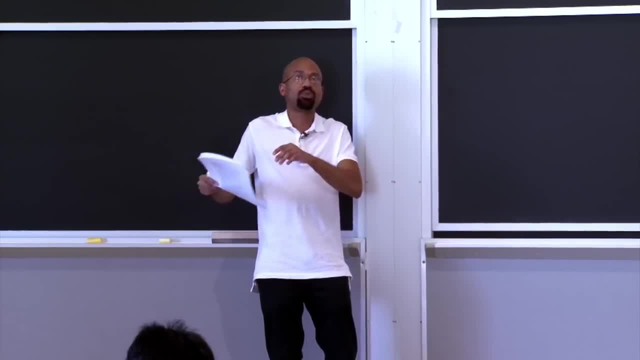 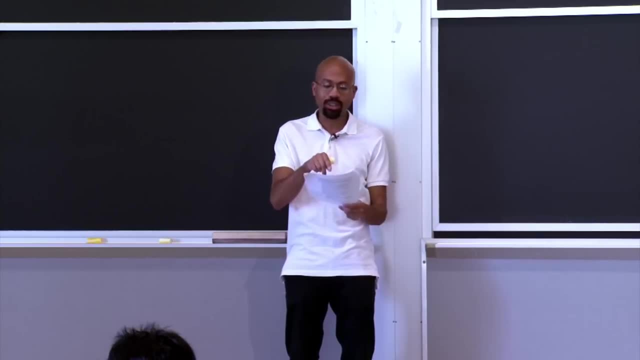 that prevent, that allow the server to not have sort of any notion of the password at all. right, So there's some zero knowledge, Yeah, There's some zero knowledge type thing or whatever. So those things do work in practice. But one of the things that this paper says: 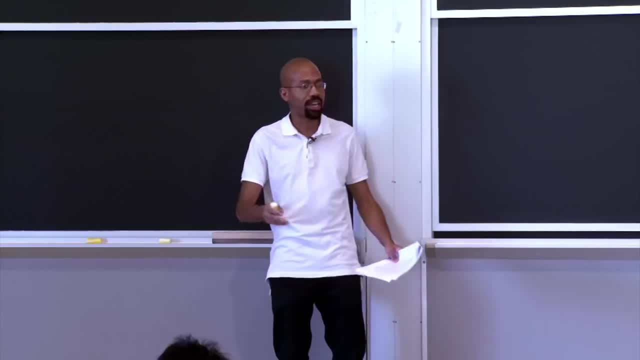 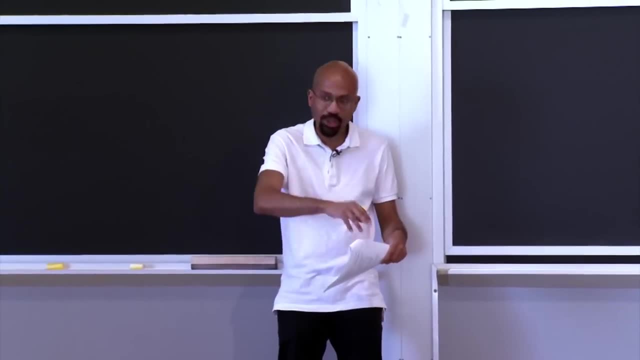 is very interesting is that they basically go through all these authentication schemes and they say, OK, here's passwords, Yeah, they kind of suck. Here's some other things that are actually much stronger on the security axis, but then they all fail on deployability or usability. 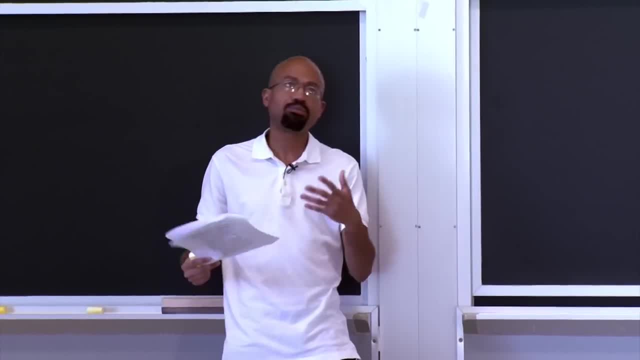 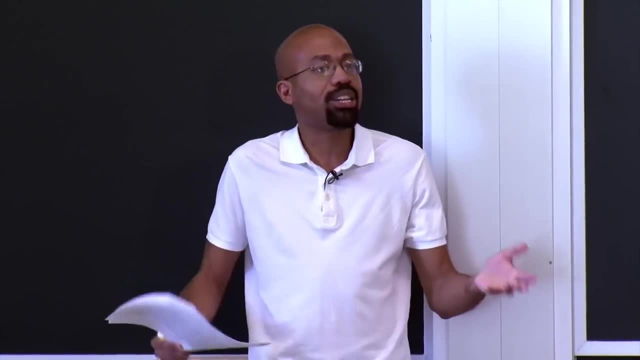 or things like that. And so that's sort of one of the interesting and slightly sad outcomes of this paper: that maybe, even though we have all these sort of much stronger from the security perspective protocols, we can't deploy them for some usability reason or some sort. 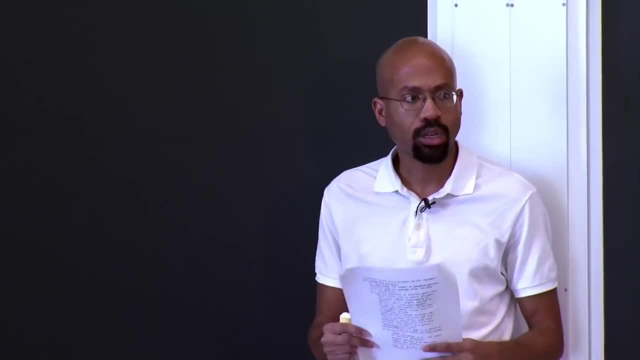 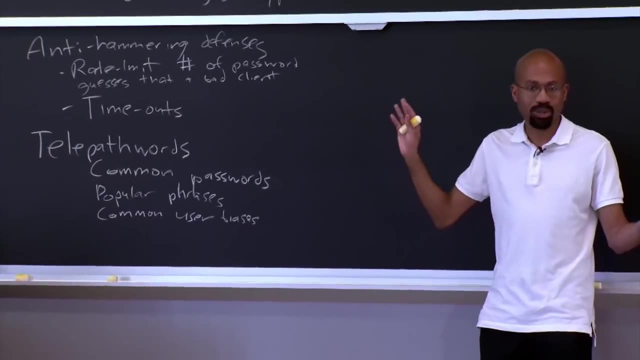 of technical reason. OK, so yeah, so that's just a fun site to go to right. And so they claim that they don't store your passwords. so you can take them at their word if you want to. But it is very interesting to just sit down and think. 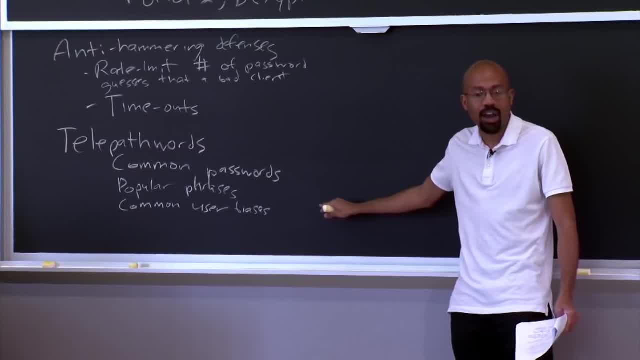 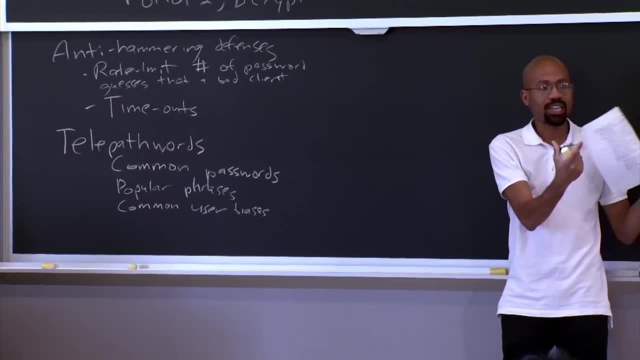 like what password would I generate And then type into this and see how accurate it is in guessing what the next thing will be right? And it even covers things like the popular heuristic, like: take a popular phrase that has multiple words and then only take the first letter of each word. 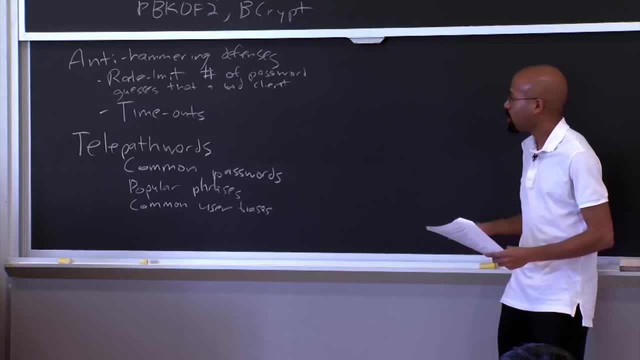 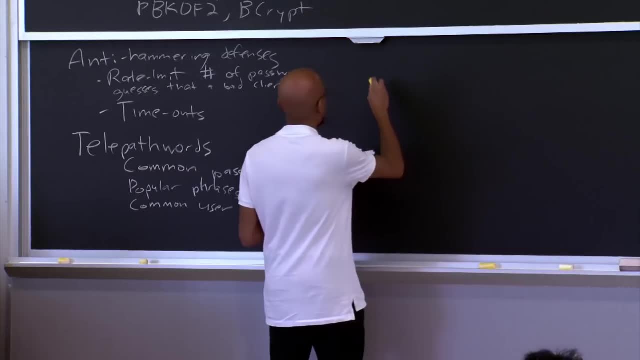 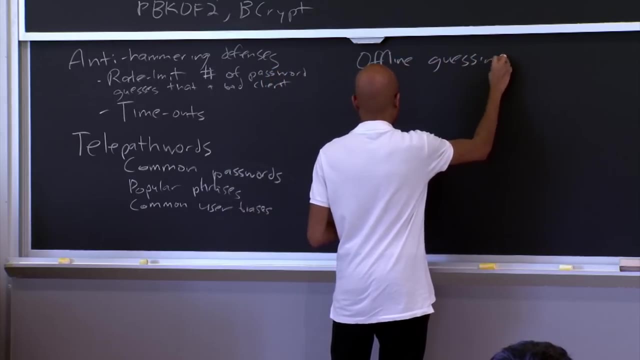 So this thing is very, very good, Very, very scary too. OK, so that's telepath words, And so one thing that is also interesting to think about is: in your password scheme, is it vulnerable to offline guessing right? 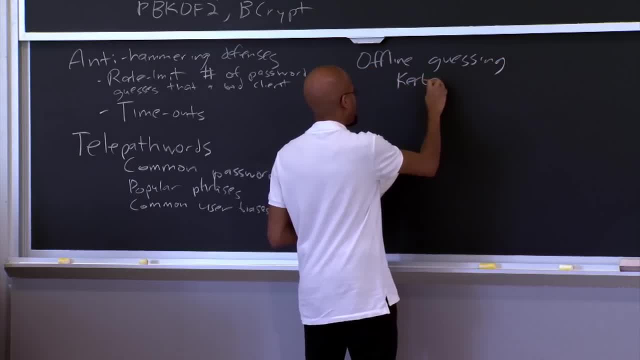 So this was a problem that Kerberos v4 had and then also v5, without this thing they call. 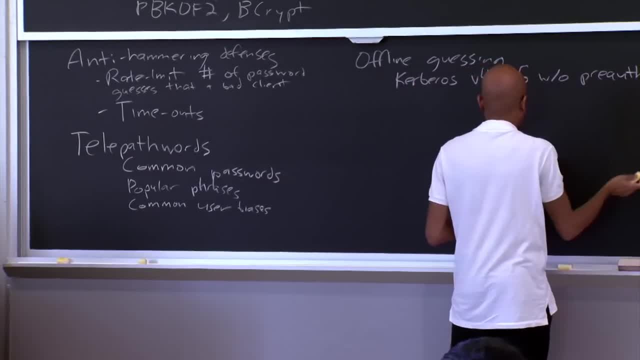 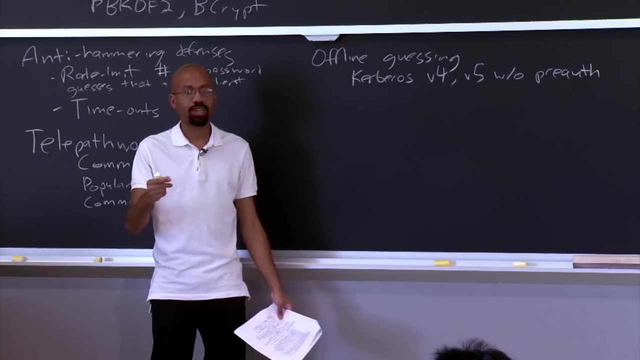 So the basic idea was that in these versions of Kerberos anyone could ask the KDC for a ticket that would be encrypted with the user's password. So basically, the KDC did not authenticate requests. 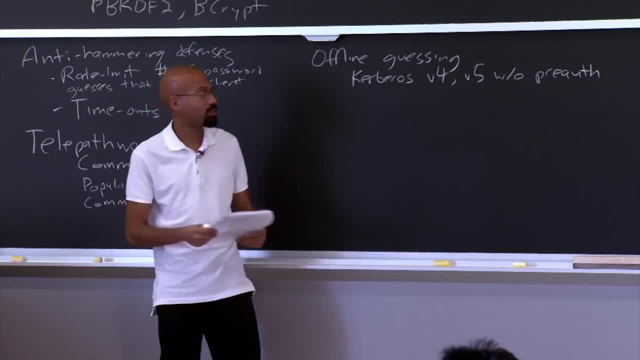 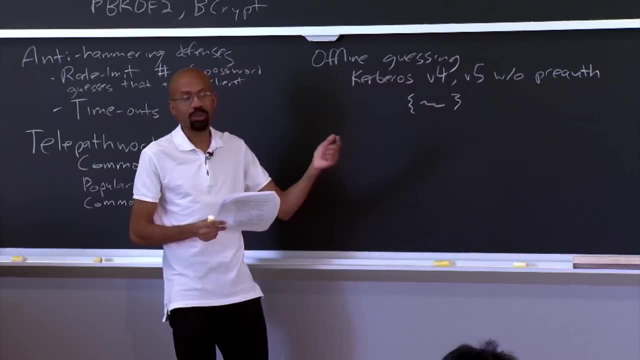 that were coming from a client. Now, the thing that the KDC would return was, in fact, there were some set of bits here that the KDC would return. I'm sure you don't want to think about this ugly set of cryptographic anymore. 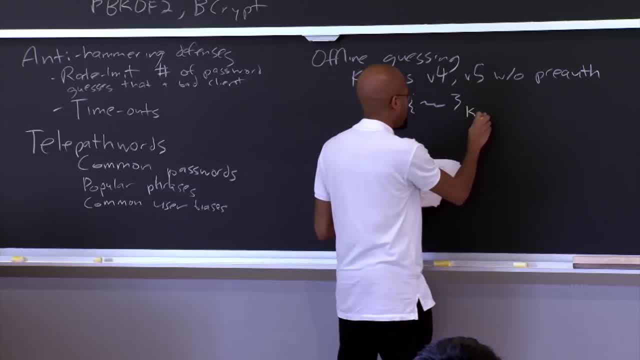 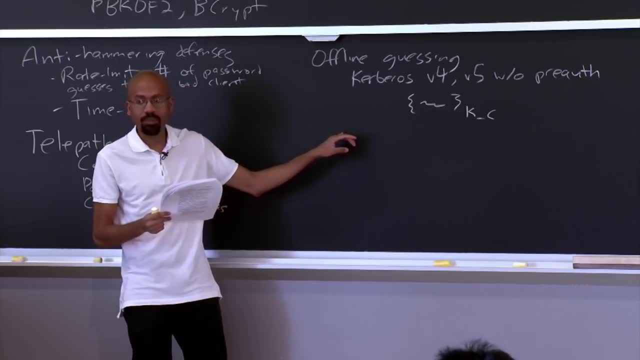 But suffice it to say the KDC would return this stuff that was encrypted with the key of the client. That's what will come back to the client side. So the problem with this is that because the server did not check who it was sending this encrypted set of things to, 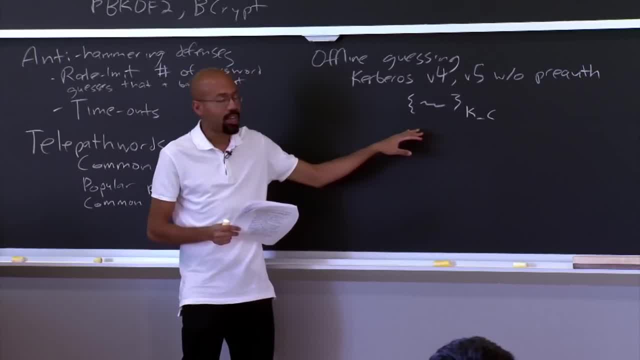 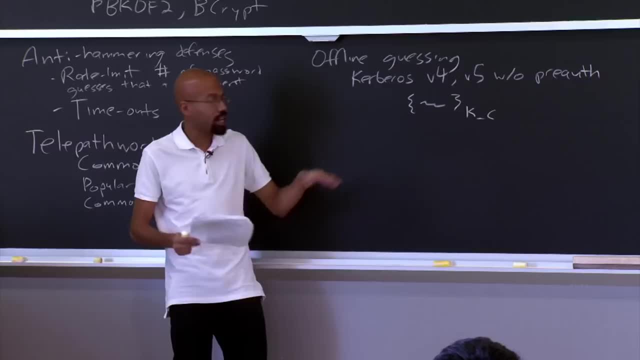 the attacker can basically get this thing here and then try to just guess what KC is. Just guess that KC is some value. try to decrypt this, see if it looks reasonable. If not, try to guess another KC. decrypt this, see if it looks reasonable. 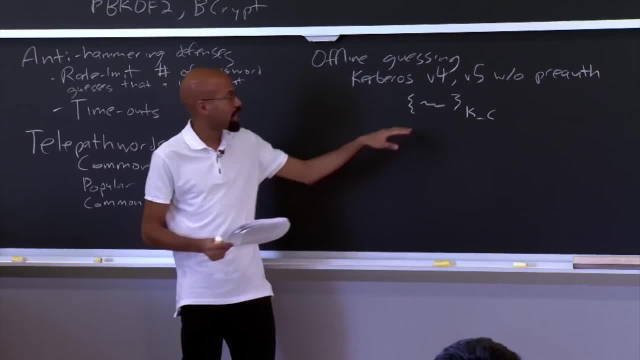 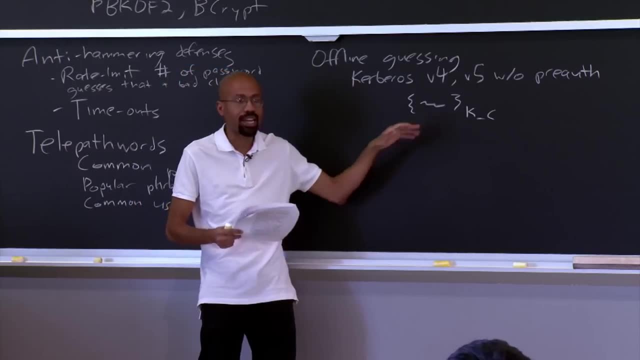 And the reason why the attacker can launch this type of attack is that this thing here, this TGT, actually has a known format. So it has things in here like timestamps and it has things in here like various length fields would have to be sort of internally consistent. 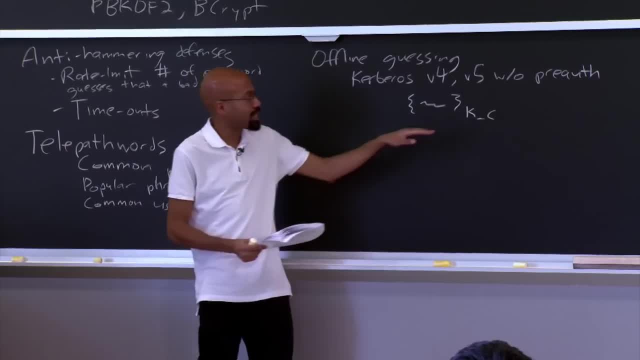 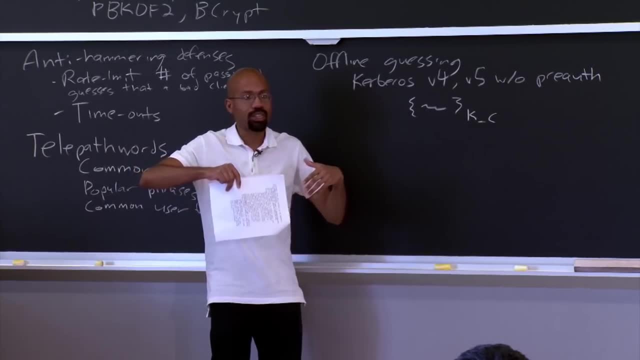 And so that basically helps the attacker. Because if the attacker guesses a KC, gets this thing here, a decrypted thing, and the internal fields don't check out. the attacker knows that It picked the wrong KC, So they can go on and pick another KC. 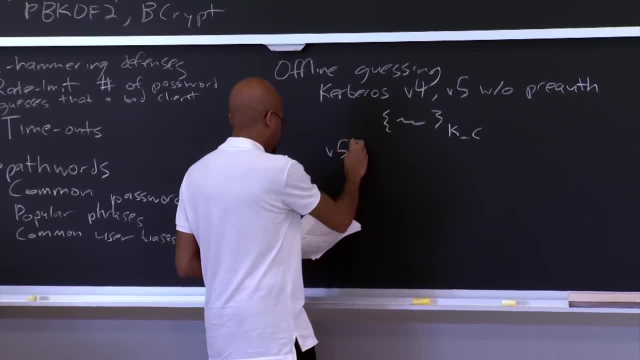 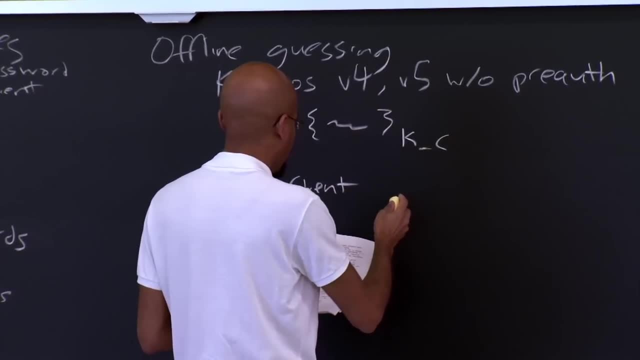 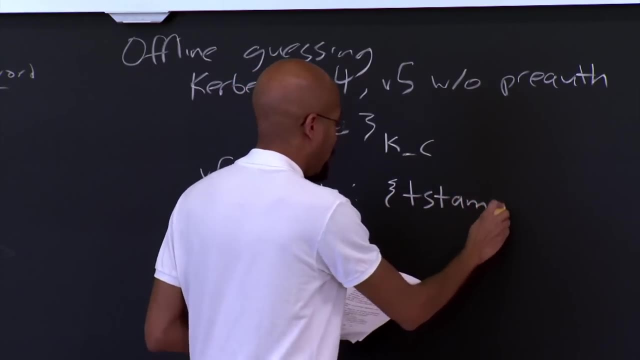 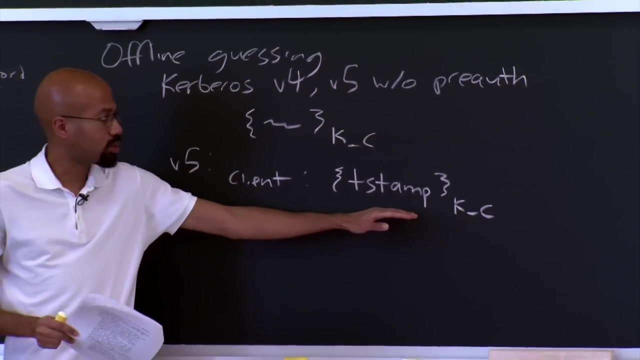 And so in Kerberos V5, basically the client has to send in this thing that it sends over to the KDC. it basically sends a timestamp And then this timestamp is going to be encrypted with KC. So this is sent to the server and the server looks at this. 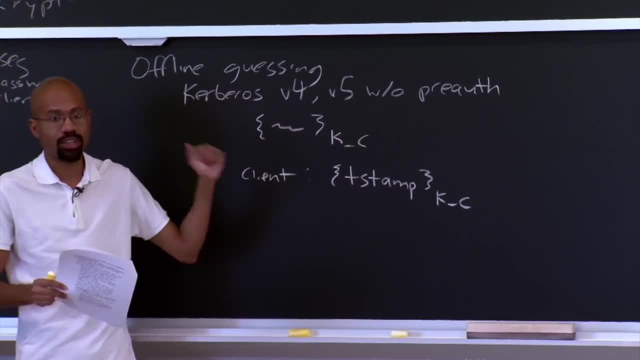 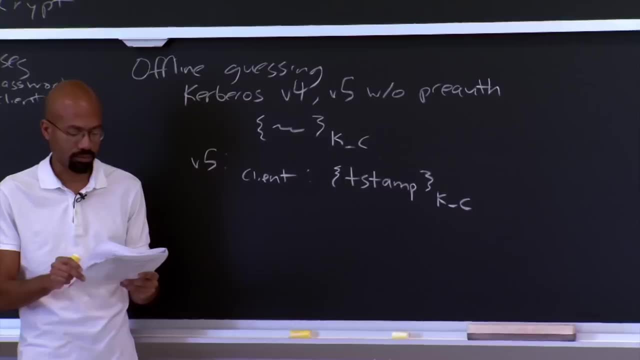 and validates, And then it's going to do that before it will send something back to the client, And so that gets rid of this problem that any random client can show up and just ask for this thing here. All right, So is the timestamp included in the message? 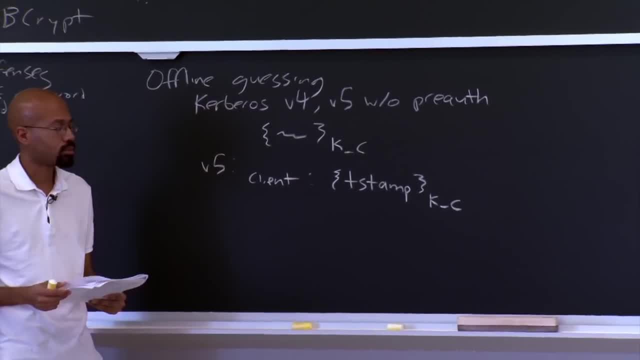 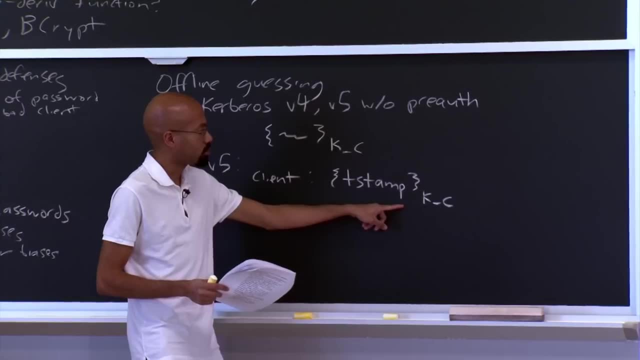 So can't the attacker just get this message and reinforce it? Let's see here. So can't the attacker get this message here? Yeah, the encryption. So you're worried that the attacker might try to spoof this, For example? No, 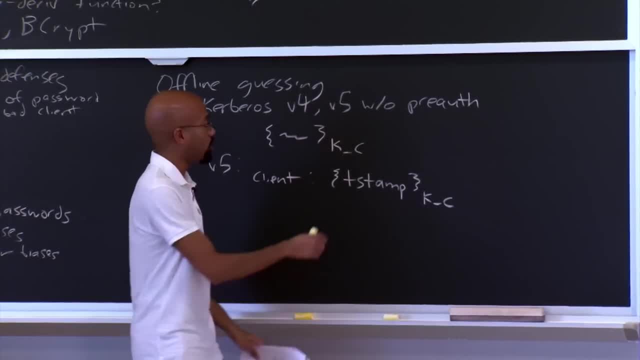 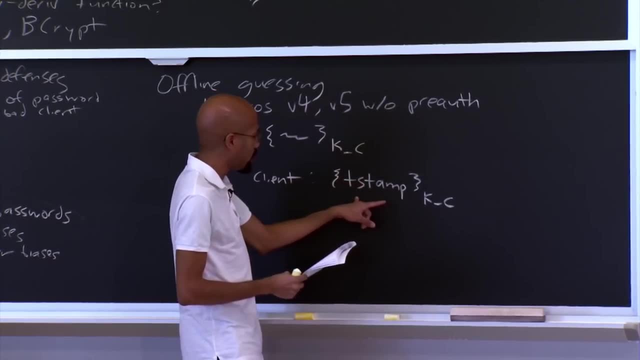 I just spoofed for set and get KCM. Ah, OK, So in other words, you're worried someone could observe this, Right, The attacker could observe it, Right, right. So I believe that this is put inside an encrypted thing, that 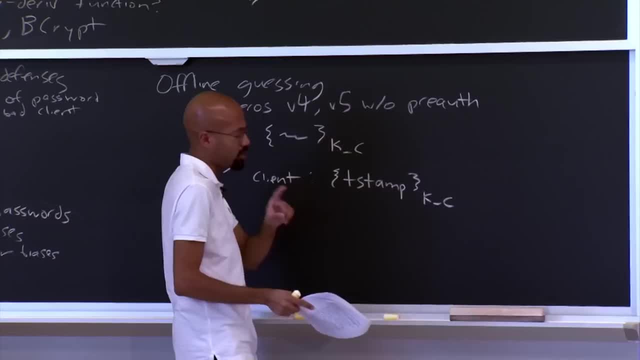 belongs to the server, that the key belongs to the server, I think. to prevent that attack I have to check the protocol, so don't quote me on that. But you're correct that if it's not, for example, And if the attacker, for example, 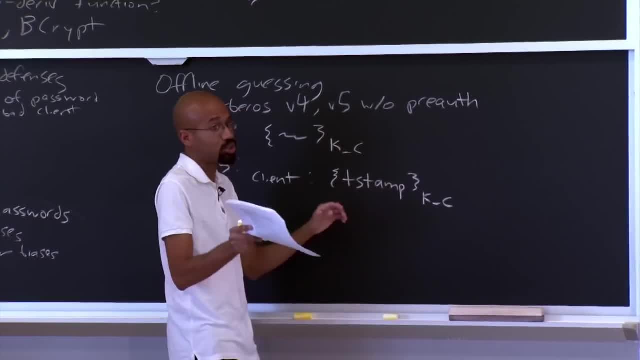 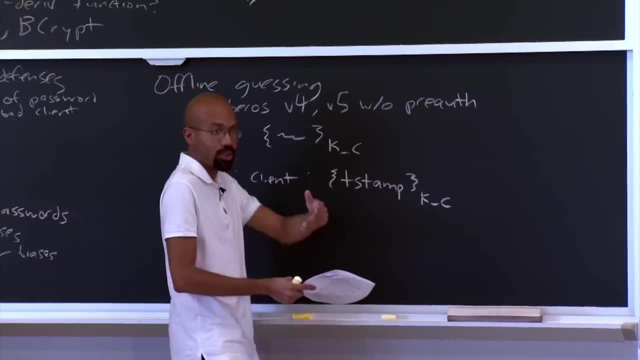 knew something about what the current time is roughly. that actually is super useful, Because then the attacker can guess: oh, the timestamp should be roughly between here and here, right, And if it sees this in the clear it can do the exact same attack that we had up here. 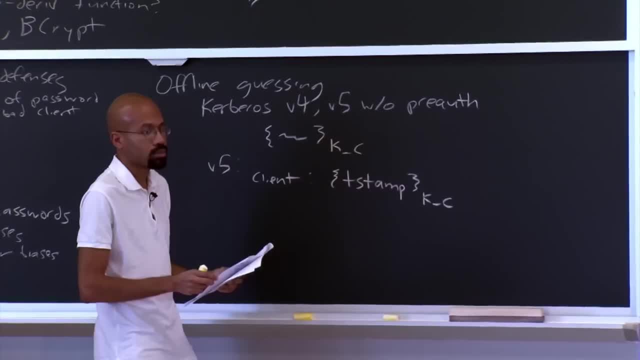 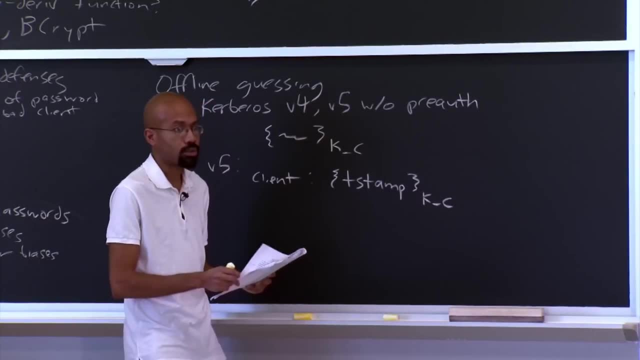 It's a little better, because the attacker has to be in the middle to still see stuff, That's true. Well, yeah, that's right. I mean the attacker has to be on the network somewhere sniffing stuff, That's right. 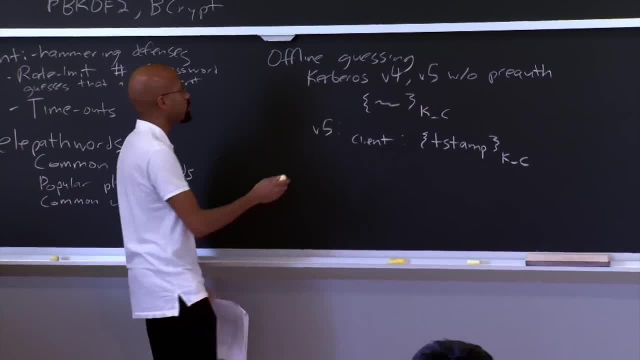 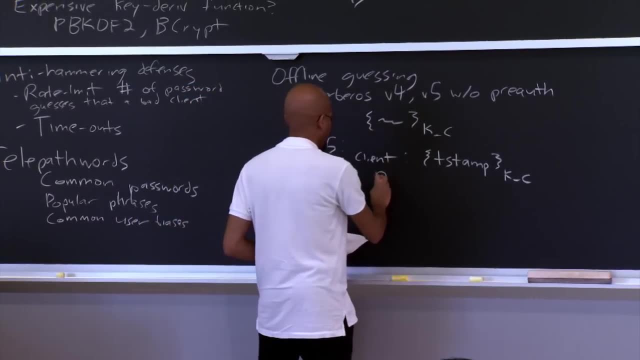 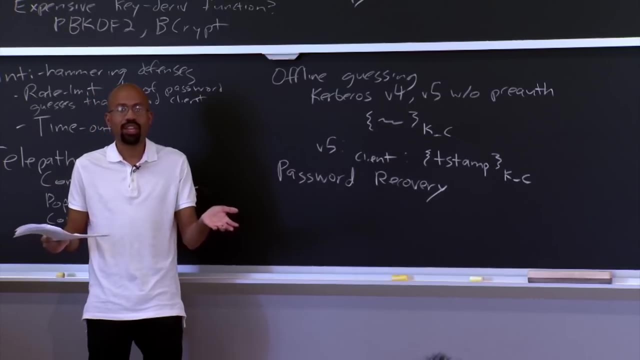 All right, so that's offline guessing. So another thing that's important to think about is sort of password recovery. So this is the idea that you lose your password and then somehow you have to go to the service and you have to ask for another password. 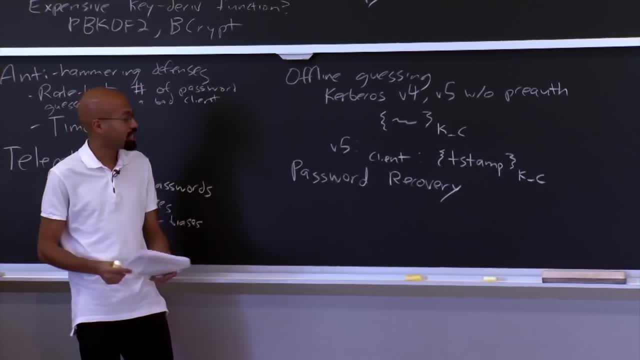 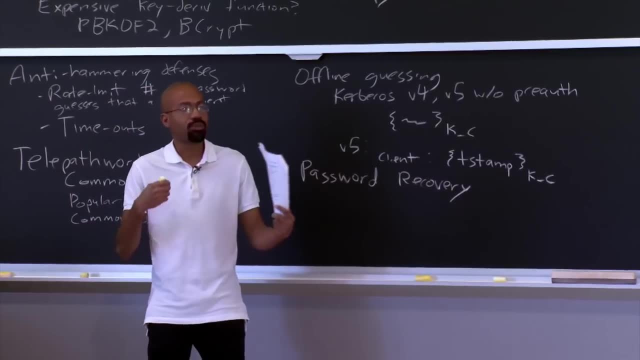 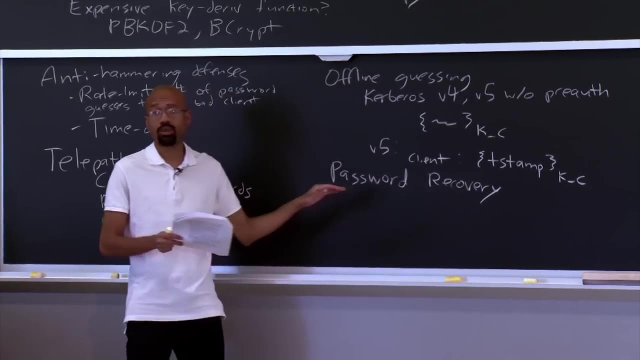 But before you get that password, you have to prove that you are you in some way. So how does that work? How do you do password recovery? So what's interesting is that people oftentimes focus on the entropy of the password itself, But the problem is that if the password recovery questions 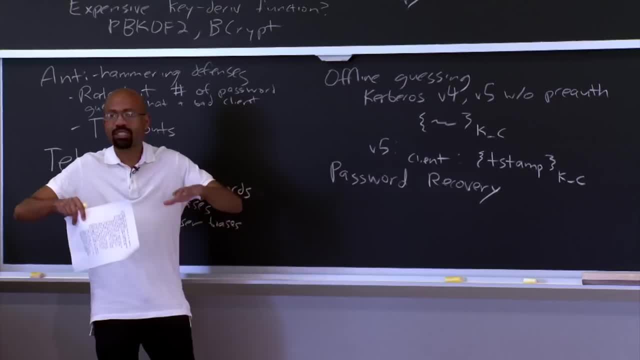 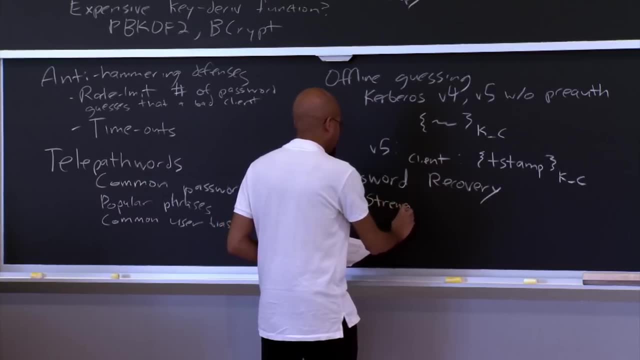 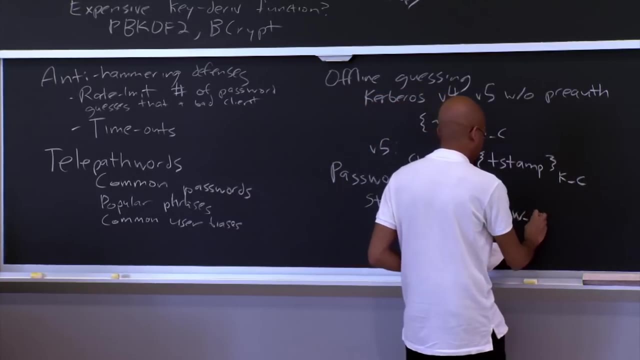 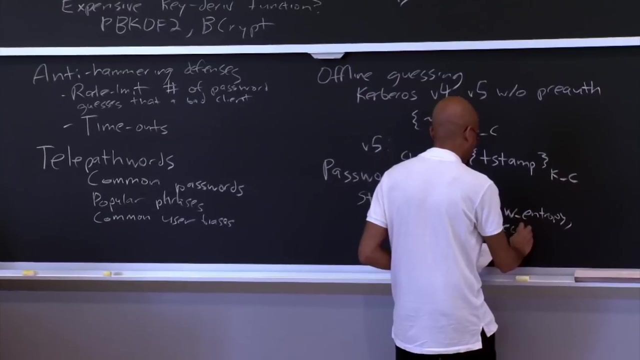 or the password recovery scheme has low entropy that actually affects the entropy of the overall authentication scheme. So in other words, the strength of the overall scheme is basically equal to the minimum of the password entropy and the recovery question entropy. And so you see this actually play out. in a lot of real world scenarios. There's a lot of famous cases, like the Sarah Palin case, where basically someone was able to recover her password fraudulently because her recovery questions were things that any random person could find, by looking at her Wikipedia article, for example. 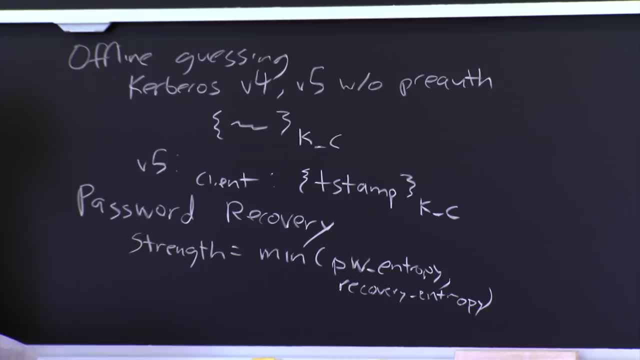 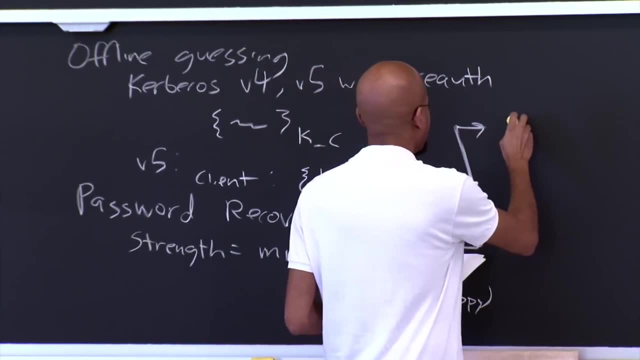 find out where she went to high school and things like that. And so oftentimes these password recovery questions are not very good, And they're not very good because of a couple of reasons. So sometimes these things just have very low entropy. 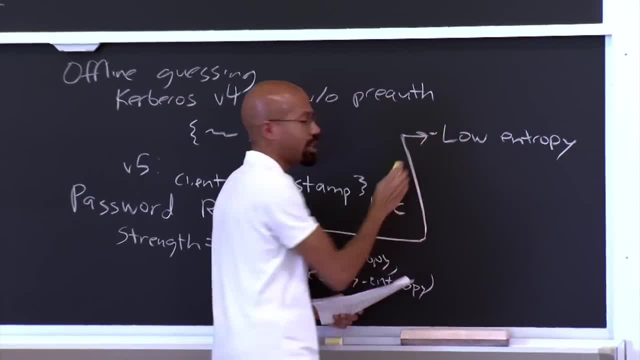 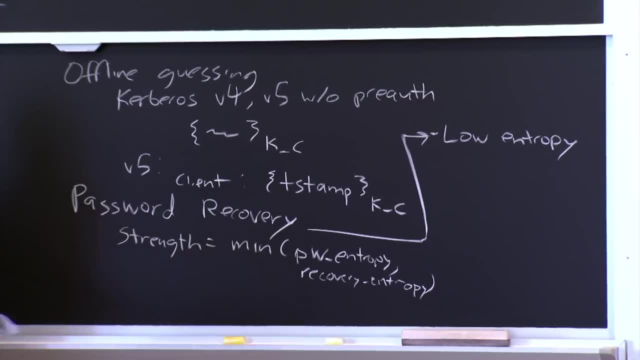 Right. So if you have a password recovery question that is something like what's your favorite color, the most popular answers are going to be blue and red. Nobody's going to say off-white, fuchsia, magenta. So some of these recovery questions just intrinsically. 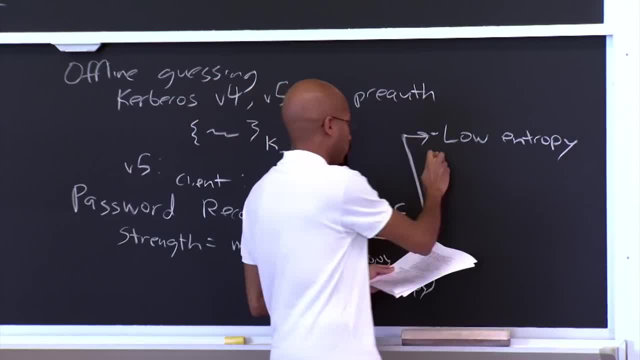 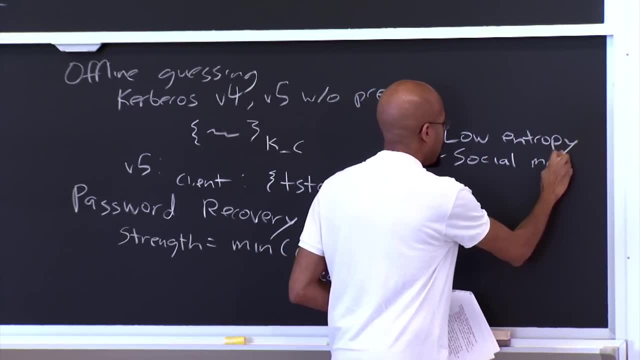 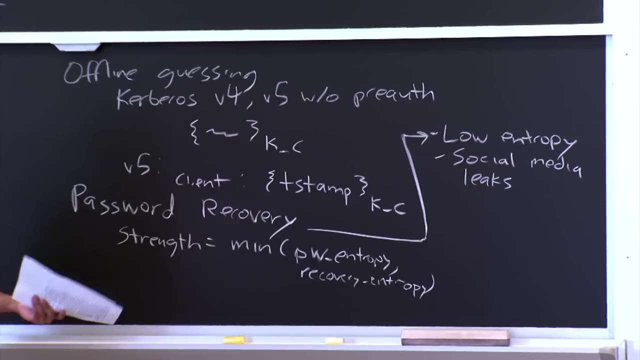 are just very difficult to provide a lot of entropy for. The other problem is that sometimes these recovery questions can be leaked via social media. So, for example, if one of the recovery questions is what's your favorite movie, So maybe the space there is a little bit bigger. 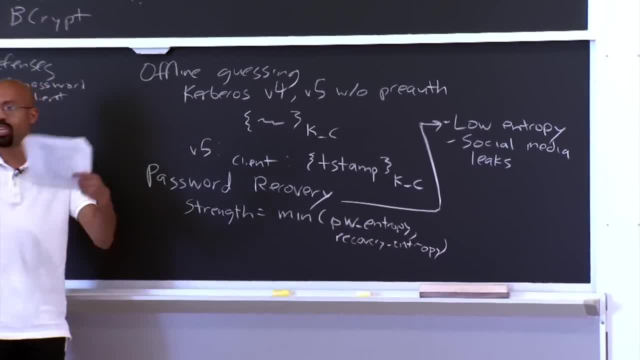 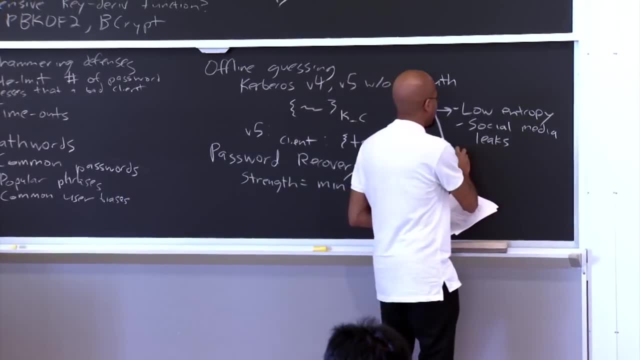 But if, intrinsically, I can go look at, let's say, your IMDB profile or your Facebook profile and figure out- oh hey, you literally told me that's your favorite movie- this isn't super useful either. And another problem: this is actually sort of the funniest. 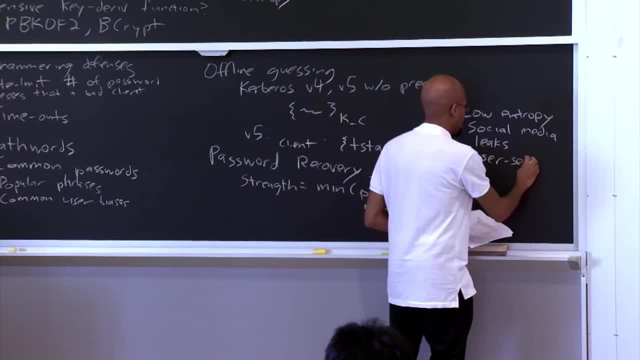 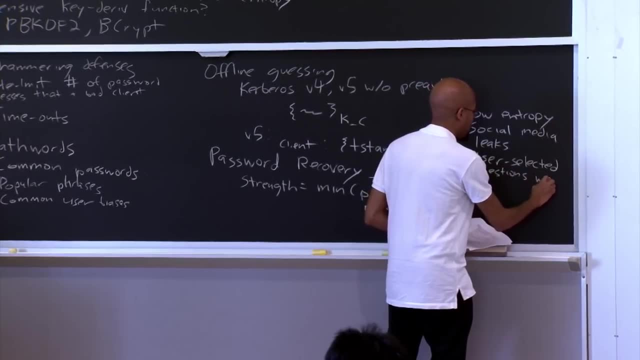 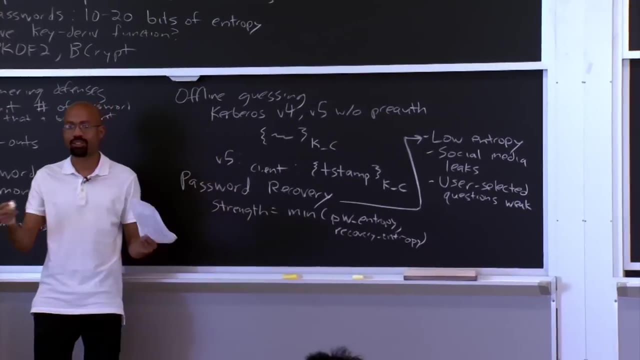 one is that the user-selected recovery questions are often super weak. So, for example, people have done a survey of what some of these questions, And sometimes users themselves, will set recovery questions that are things like: what is 2 plus 3?? 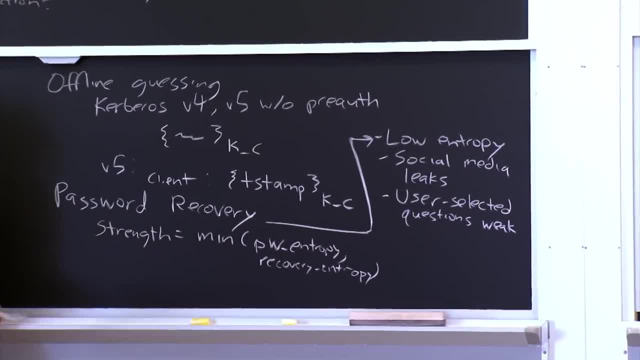 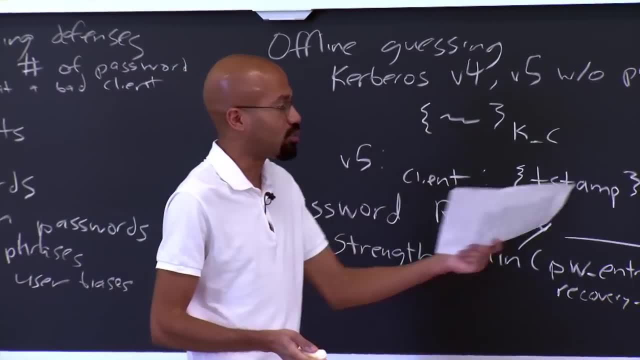 And so at the time the user's thinking this is a big hassle and they're going to have to use this. But trivially, most humans who pass the Turing test can answer that question successfully and then therefore get the user's password back. So both Microsoft and Google have a system for recovering passwords that doesn't use any recovery password for recovery questions. It's basically like you enter a password and you enter in your name and maybe the subject of some emails that you've sent and a small amount. 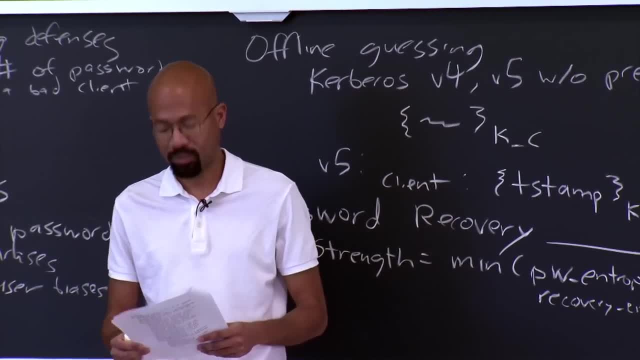 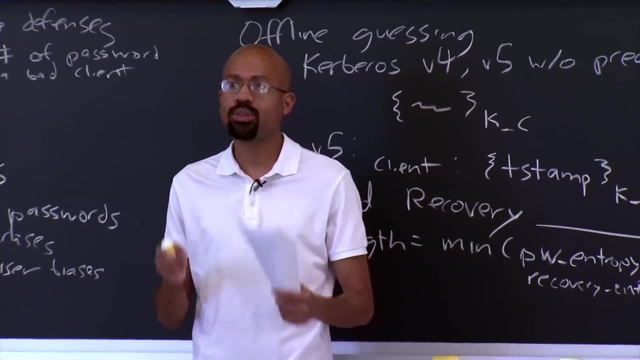 of additional information Based on that. in some cases they can, you know. So security, that kind of stuff then. So I don't know of any formal study like that. Those things are actually a lot better. So I actually know this because I. 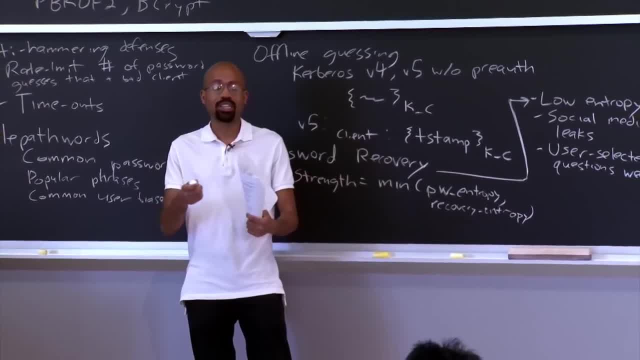 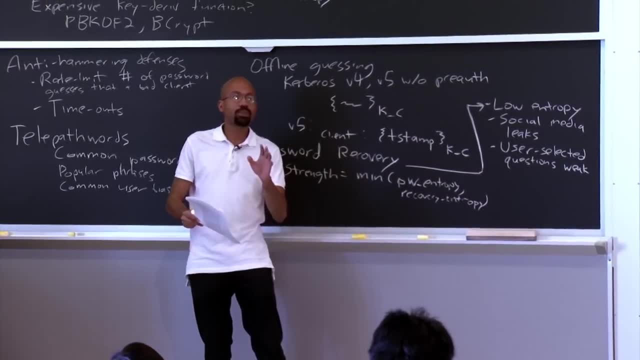 was trying to help a friend go through this process, So she basically lost control of her Gmail account and she was trying to prove that this was her account. And so, yeah, they would ask you things like, roughly speaking, when did you open this account? 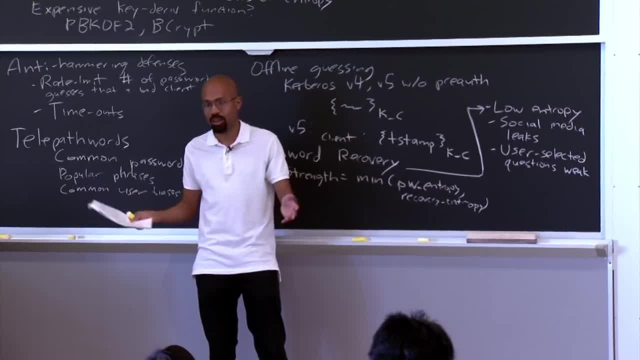 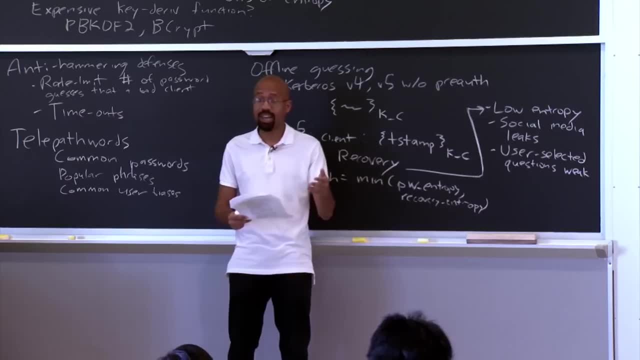 Roughly speaking, before you lost control of this account to Hezbollah or whatever, who are some of the people that you talk to And things like that, And it's actually a pretty laborious process, right, But what ends up happening is that you're exactly correct. 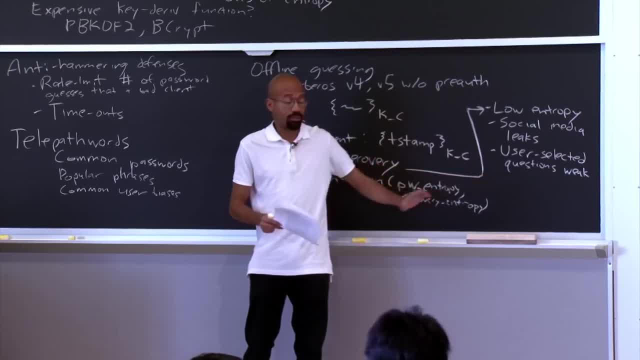 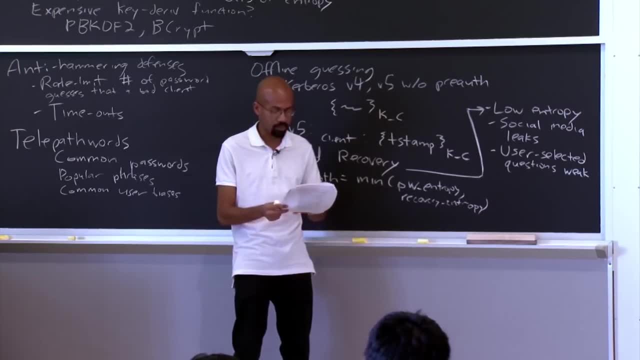 It ends up being much more powerful than this stuff, right, And so I don't know of any formal studies of that, but it does seem, at least intuitively, to be much stronger than these types of things. All right, any other questions? 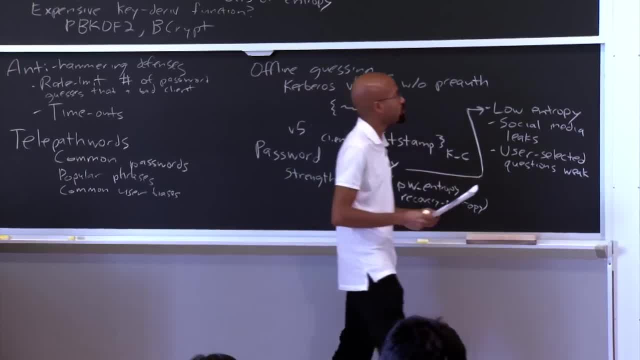 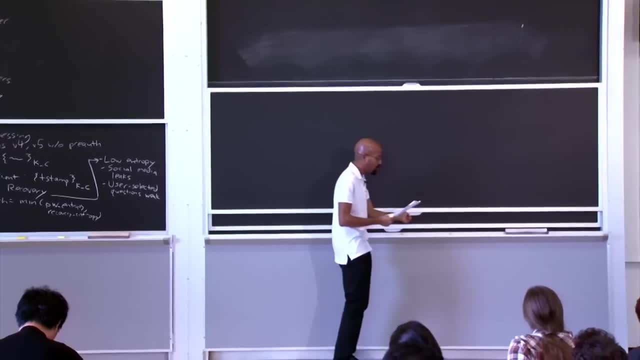 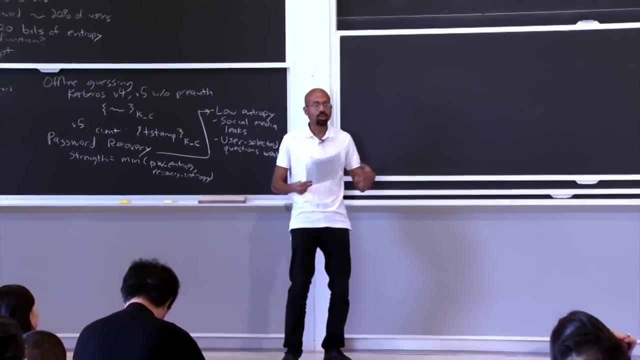 OK, so now we can get to the paper for today. So in the reading for today, the authors basically propose a bunch of factors that can be used to evaluate these authentication schemes, And what's really cool about this paper, I think, is that it basically tries to say: look, 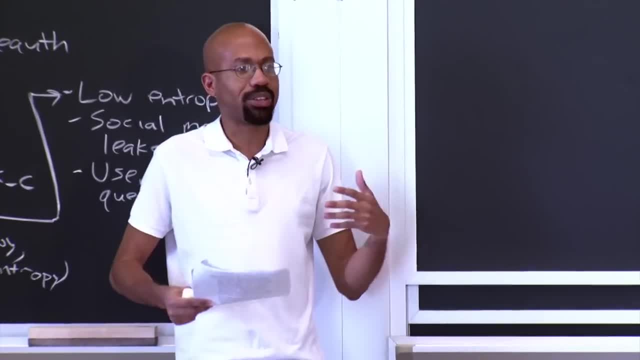 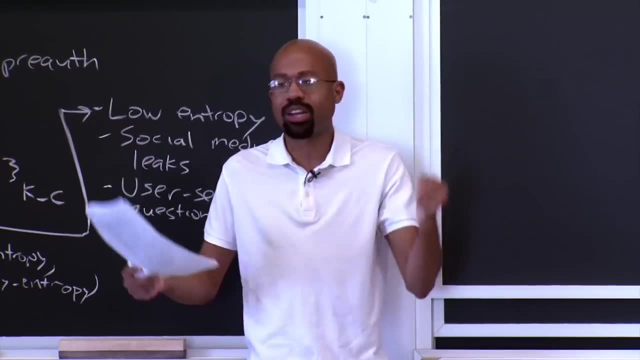 a lot of us in the security community are sitting there fighting just based on aesthetic principles. Like: we should pick this because I just like the way that the curly braces look in the proof. We should pick this because it just uses a lot of math mode, right. 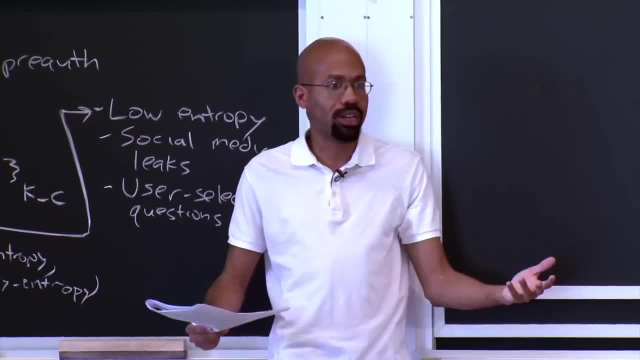 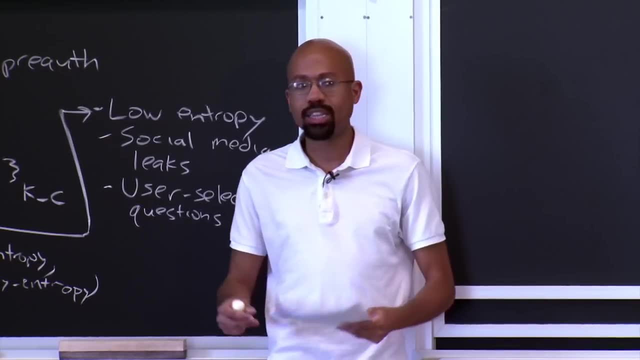 And so what they say is: well, look, why don't we try to establish some type of criteria? Maybe some of the criteria are a little bit subjective, But let's just try to have this taxonomy of ways to evaluate these authentication schemes. 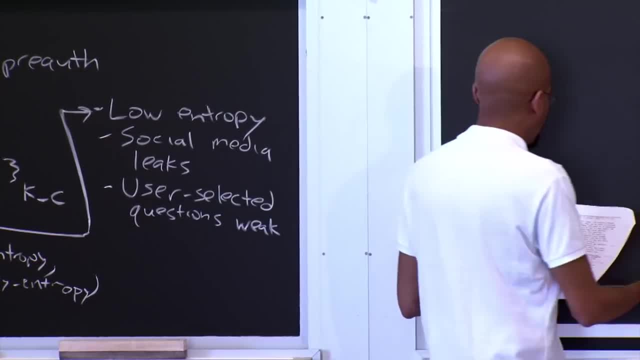 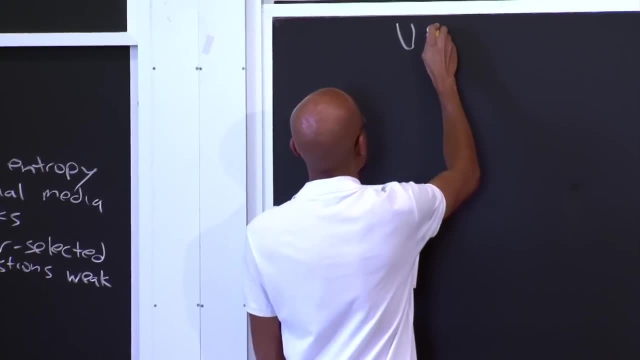 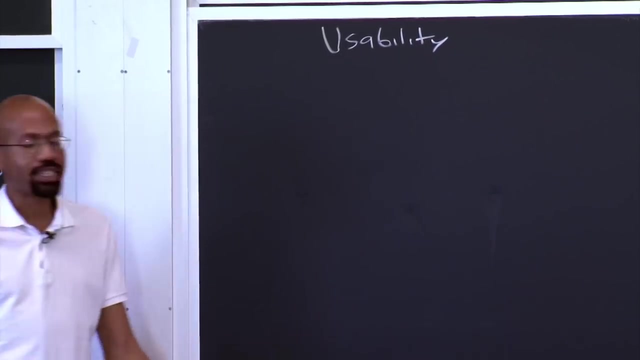 Then let's just see how these various schemes stack up, And so the authors basically propose three high level metrics for evaluating these schemes. So the first metric is usability, And so the base idea here is how easy is it for users to interact with this authentication. 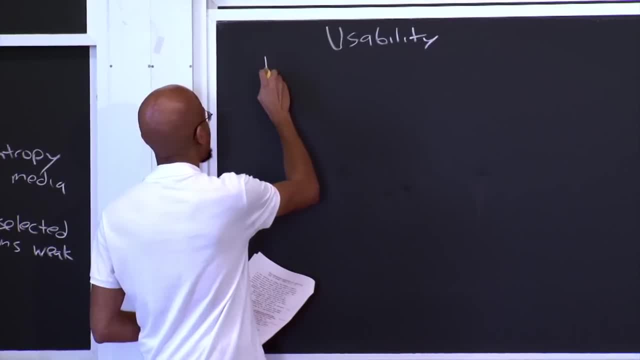 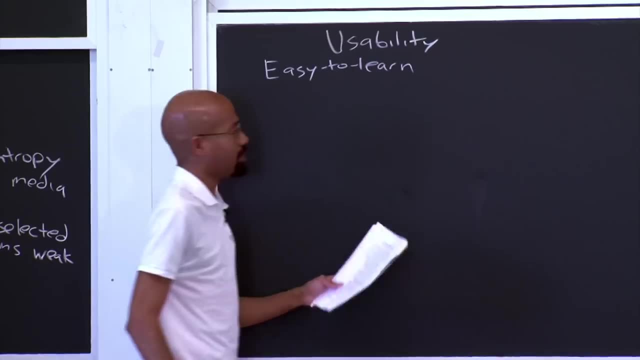 scheme. So they define a couple interesting properties. So, for example, is it easy to learn? This basically just means: is this scheme easy to learn? So some of these categories are pretty straightforward. Some of them actually involve a little bit of subtlety. 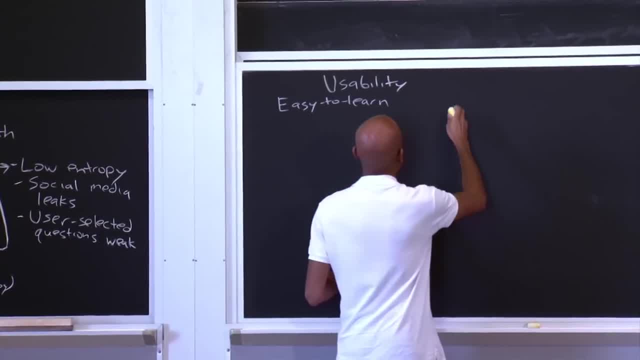 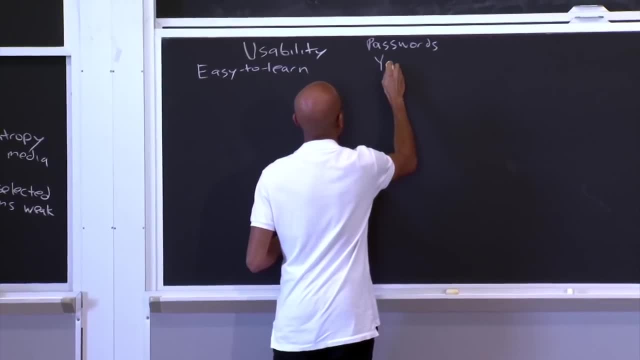 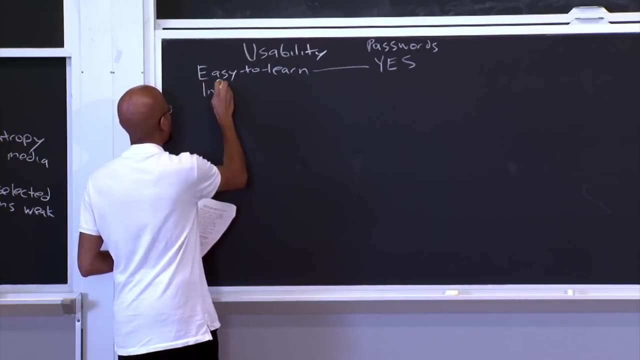 But this one makes a lot of sense And so if we look at passwords, passwords sort of pass this test Right, Because everybody is used to using passwords, So we'll say they're easy to learn. Another category is infrequent errors. 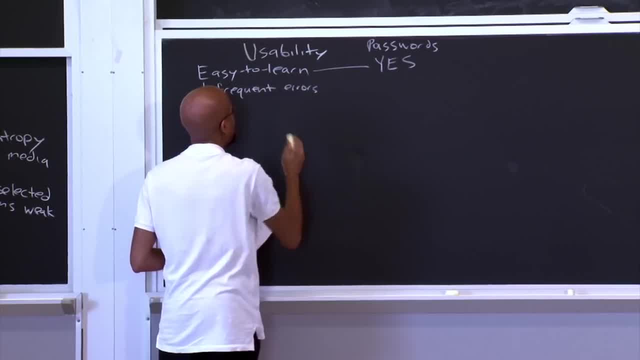 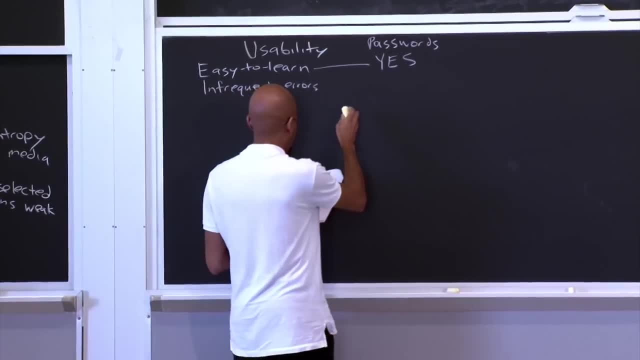 So that means, when you are trying to authenticate to the system, if you are the actual user in question, is it the case that you can often authenticate yourself without generating errors? And so here the authors say quasi-yes, Yes, Yes. 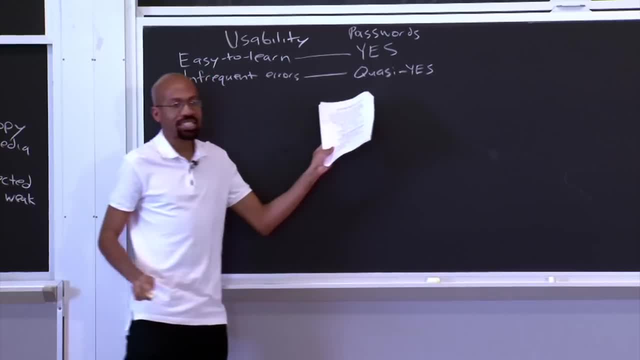 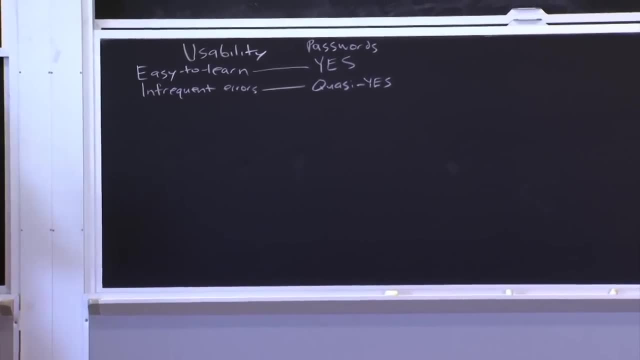 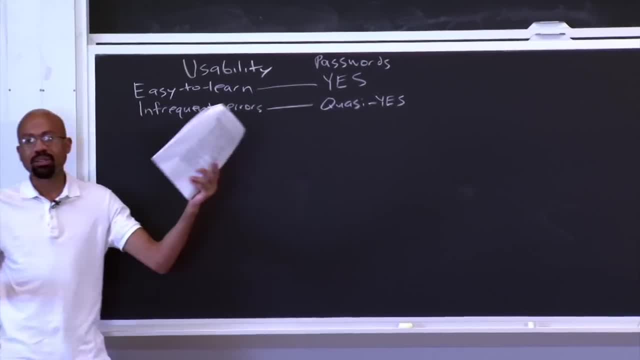 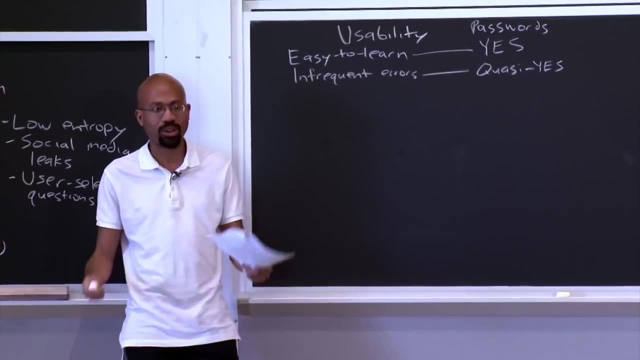 things like this. So the reason why they say quasi-yes is because in general, you can authenticate a password successfully. But we've all been in that place where it's like 3 AM We're trying to log into our email server. 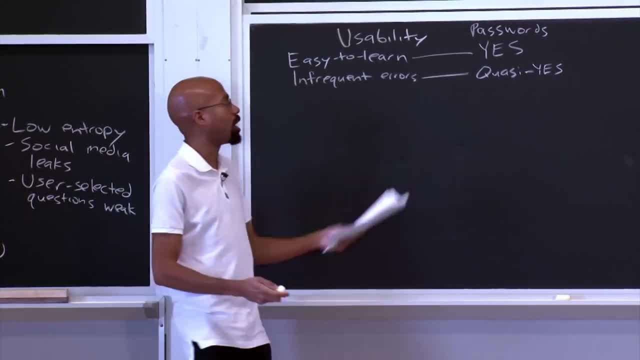 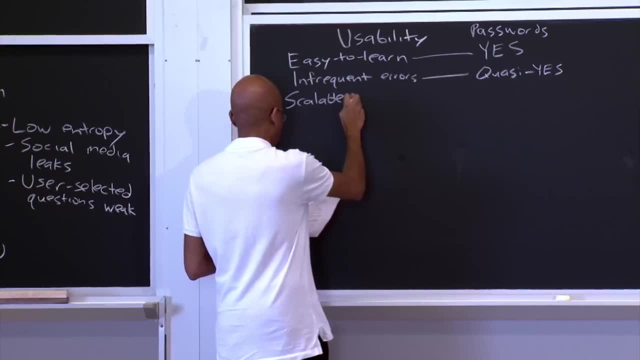 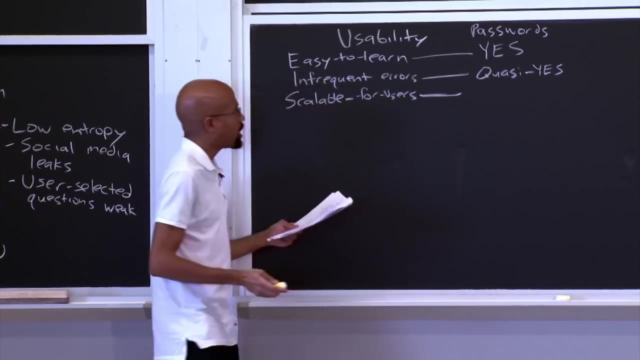 Our mind's not in the right place And we enter in a bunch of errors a bunch of times. So they say quasi-yes for this. Another category is Scalable for users, And so the basic idea here is if the user has a bunch of different services. 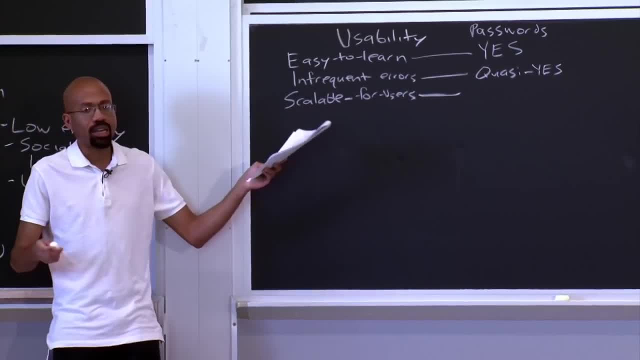 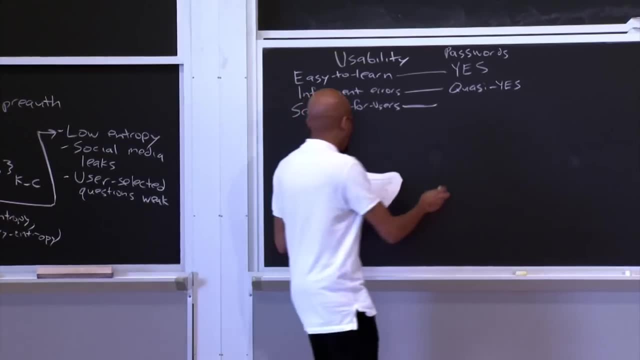 that he or she wants to authenticate to. does this scheme sort of scale? well, Does the user have to remember some new thing for each one of these schemes? And so for here, the authors say no, Because in practice it's very difficult. 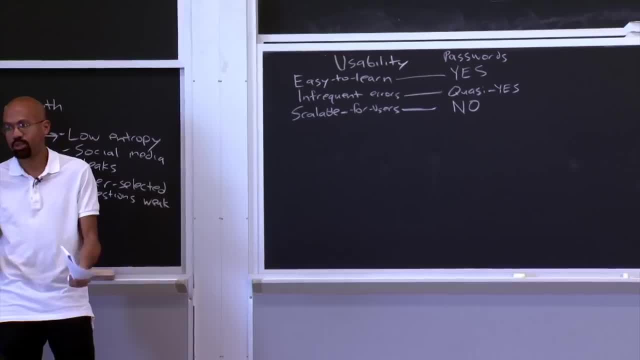 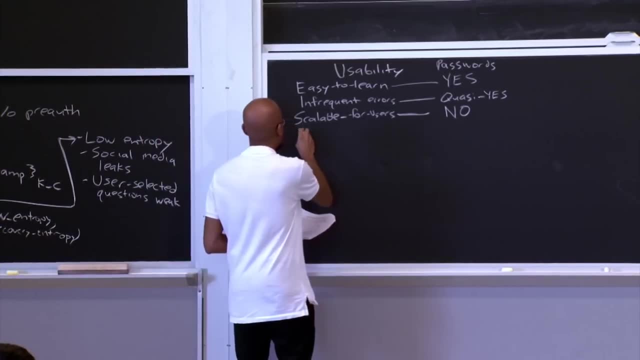 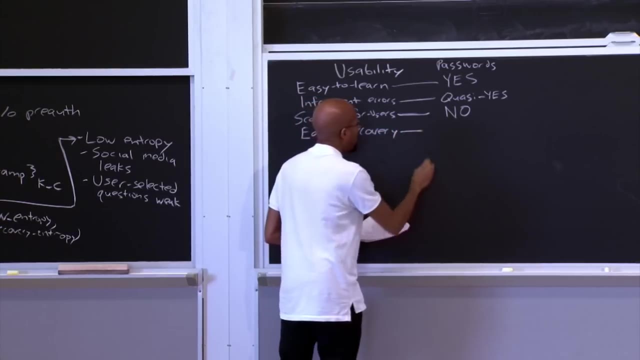 It's difficult for users to remember a separate password for every single site that they go to. This is one reason, actually, why people reuse their passwords often, So another usability property is easy recovery. So what happens if you lose your authentication token, In this case, your password? 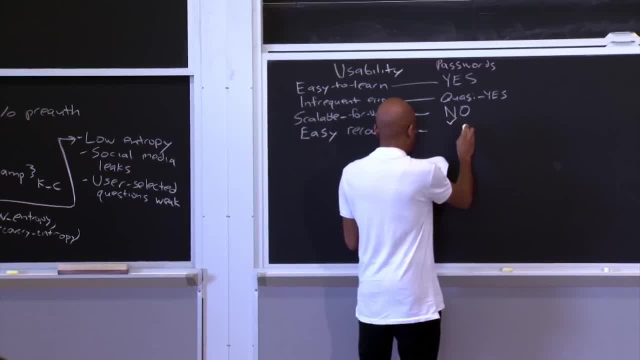 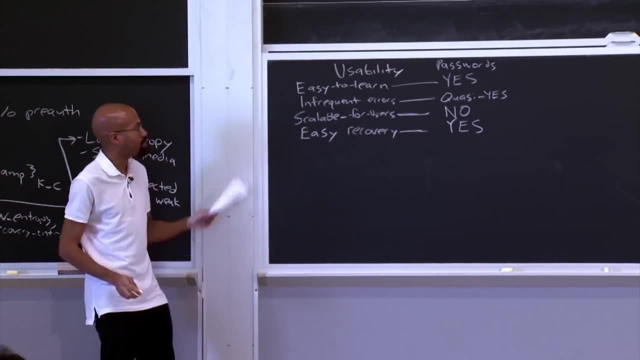 Is it easy to reset, And in this case, the answer for passwords is yes, And in fact they are probably not OK. OK, So that's probably too easy to reset, as we just discussed a couple of minutes ago. So that's a yes. 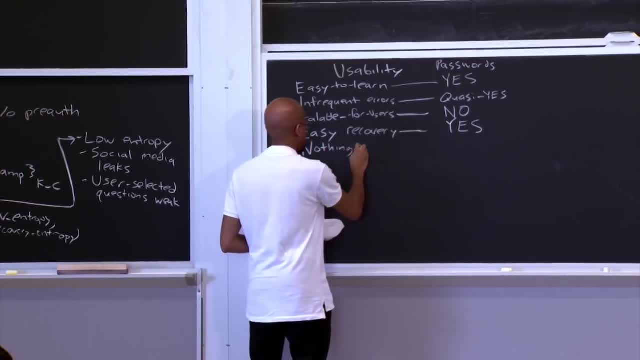 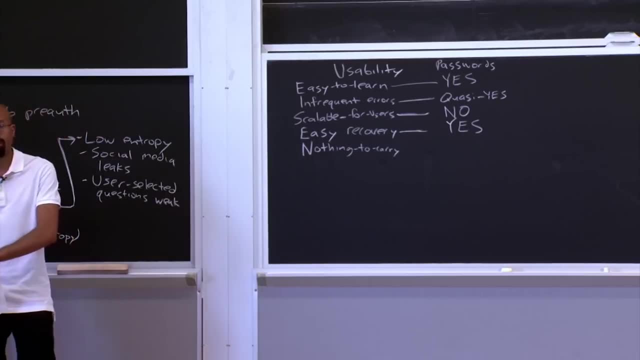 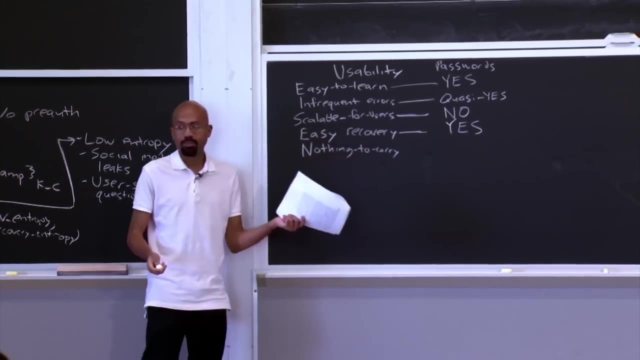 And so another interesting one is nothing to carry. So a lot of the more baroque authentication protocols require that you run some smartphone app or you have some security token or a smart card or things like that. So that's a burden right. 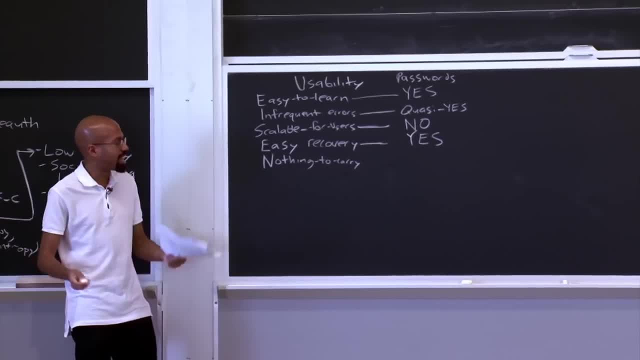 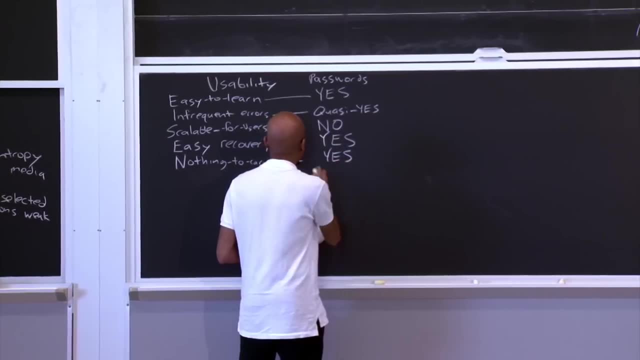 Maybe not with a smartphone so much, but having to carry around one of these other gadgets is probably a pain, And so this is actually one nice feature of passwords: you basically only have to carry around your brain, which presumably you should have at all moments. 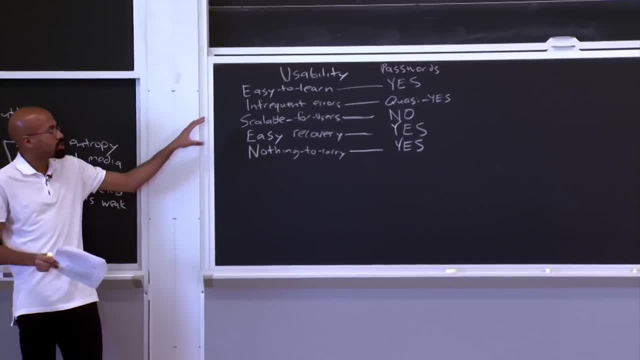 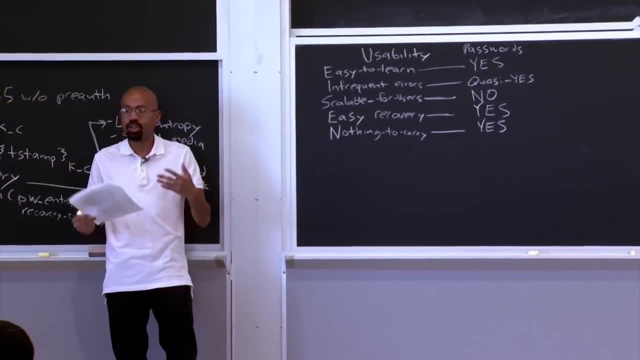 So that's basically what usability looks like, And it's just very interesting at a high level that a lot of times these sort of factors are given a little bit of a short shrift in the security community. when people are evaluating new schemes They say, oh, this thing uses like a million bits. 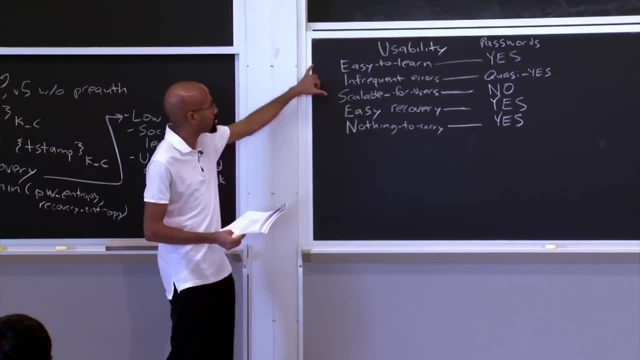 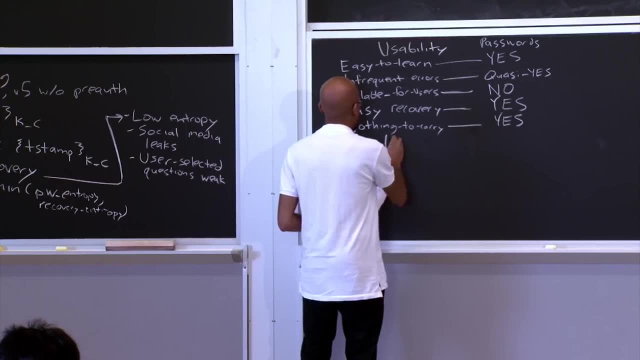 of entropy and it can only be broken by the Death Star or whatever. But then people don't necessarily remember. oh, these are actually very important factors too. So the next sort of high level category that the authors use to evaluate authentication schemes is deployability. 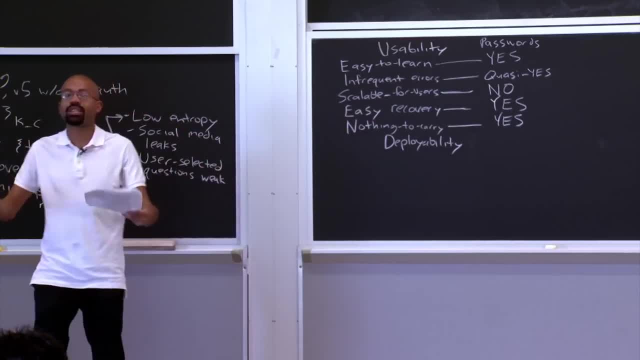 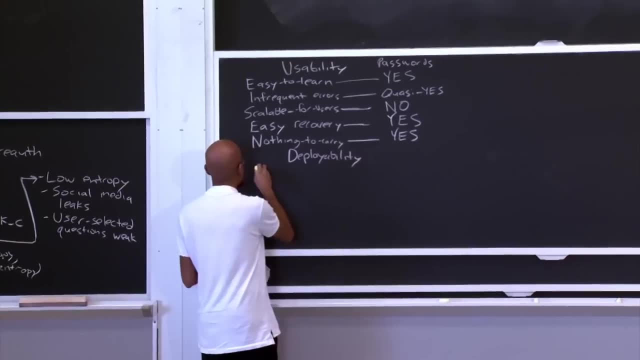 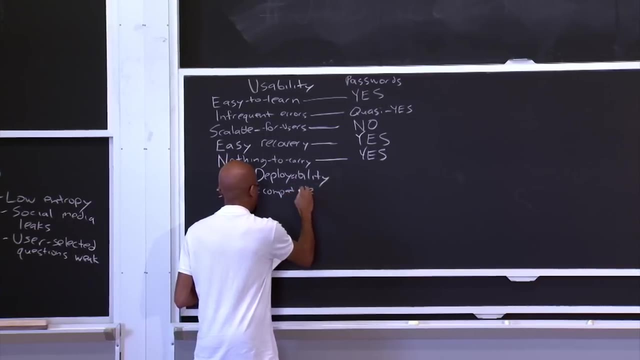 So the base idea here is: how easy is it to incorporate this system into current web services? So one thing they look at, for example, is: is it server? Is it server-compatible? And this basically means: can I easily integrate this scheme with today's servers which? 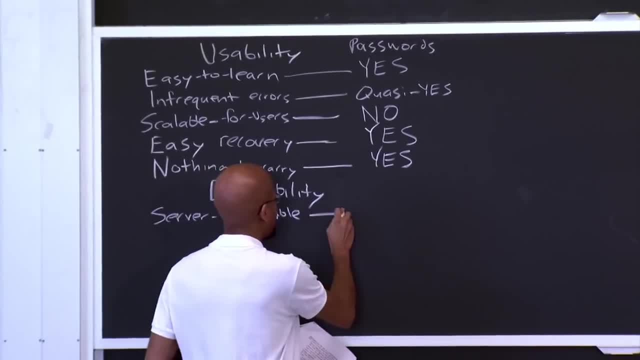 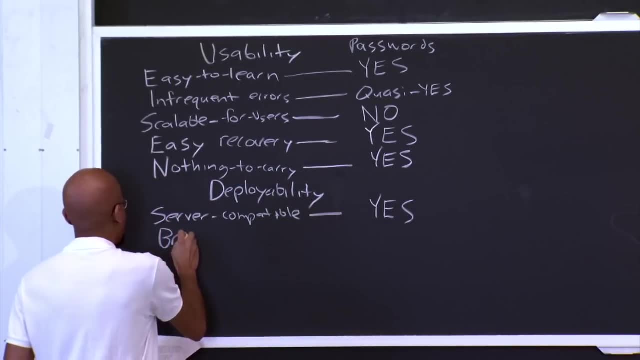 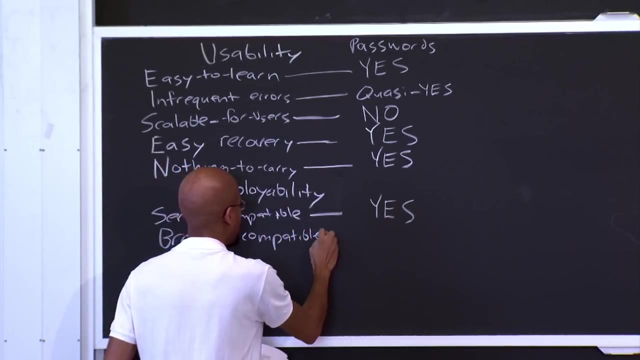 are based around sort of text-based passwords, And so, since success here is defined with respect to passwords, passwords succeed. So another metric is browser compatibility, Similar type of thing. can I use this scheme with current off-the-shelf browsers Without having to install a plug-in? something like that. 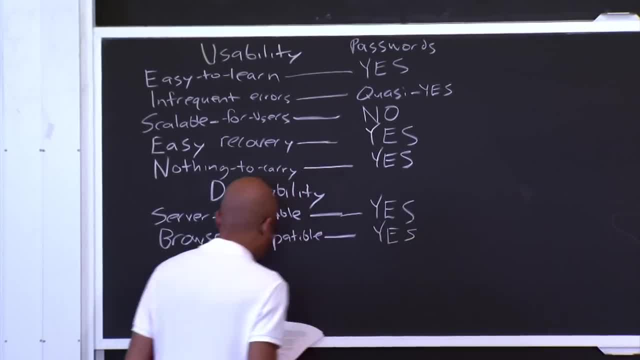 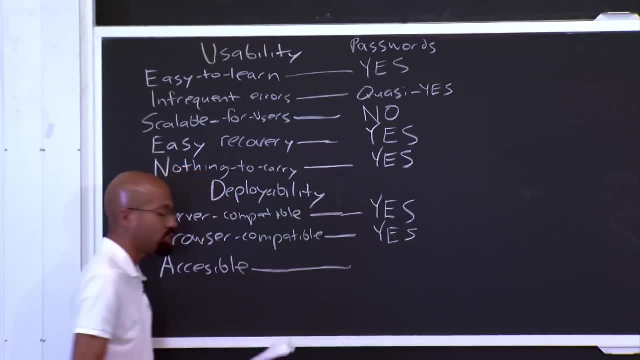 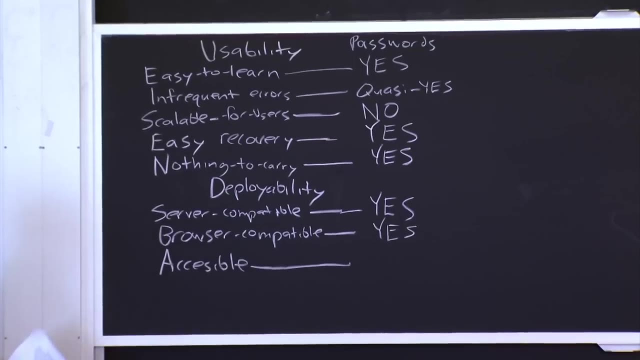 Once again, passwords win by default. And another interesting one is accessibility. So can people who can use passwords now but maybe have some type of physical disability. maybe they're blind or they can't hear well, they can't gesture well, or things like that. 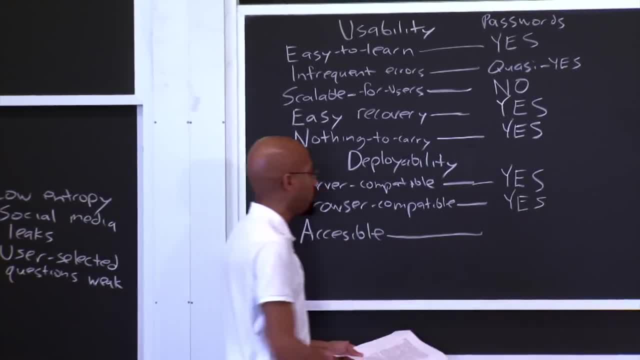 can they actually use this scheme, And this is actually pretty important. So once again, the authors say, oh well, I'm not going to do this, And they say, yes, It's a little bit weird, because it's not. 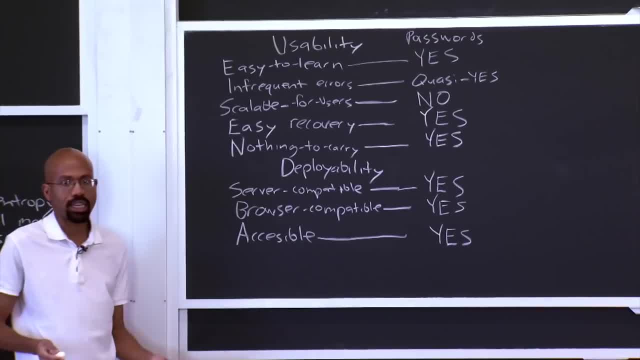 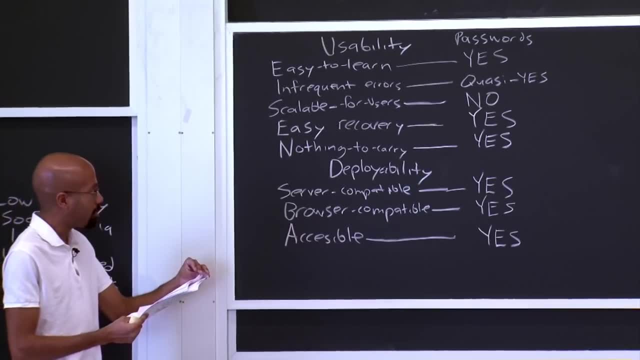 clear that all people with all disabilities can use passwords, but they say yes here, So yeah. so these are sort of three interesting things to think about with respect to deployability, And the reason why this deployability category is so important is because it's very difficult to get anyone 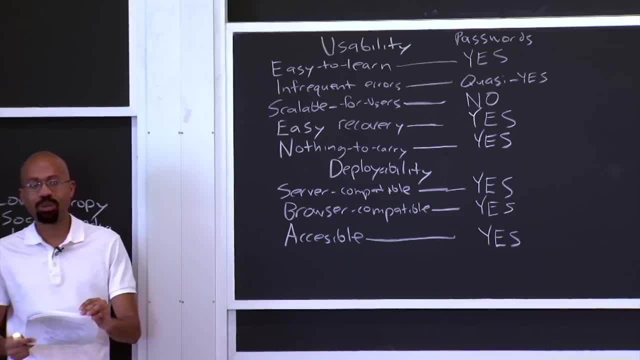 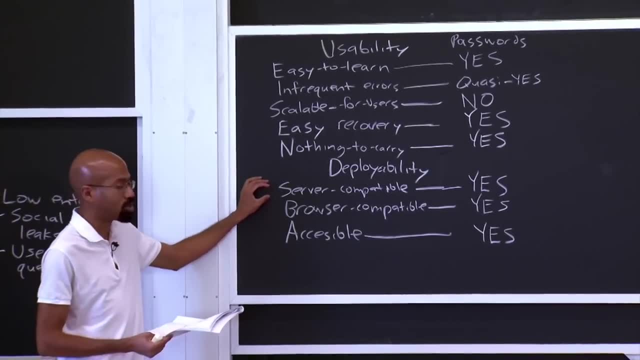 to upgrade anything ever really. I mean, people don't even want to reboot their machines to get a new OS update installed. So it's very difficult, if the scheme requires reasonable changes on the server, to sort of get people on the server to actually do different stuff. 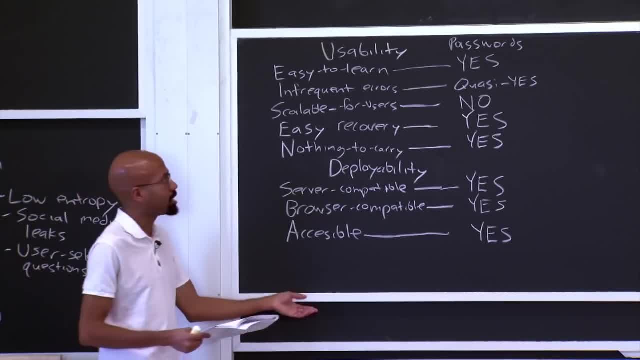 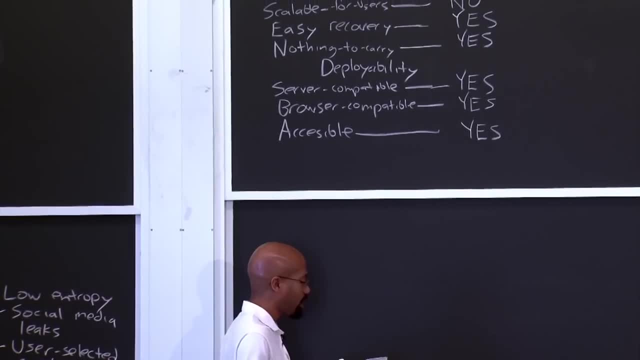 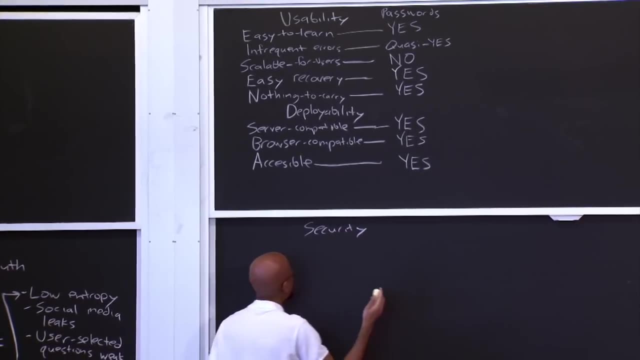 This gets back to your question: why don't we use these better things? Because deployability in many cases is super, super important to people. All right, so then the final category that people look at is security. So what kinds of attacks can this scheme prevent? 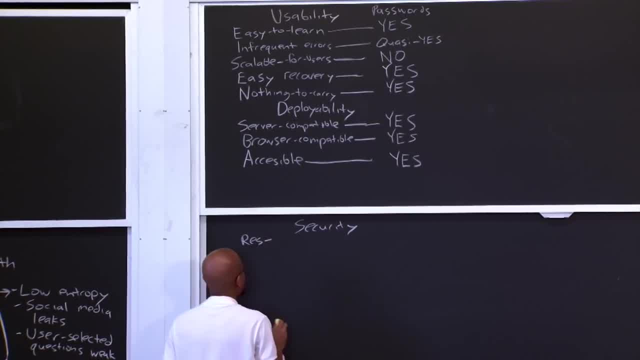 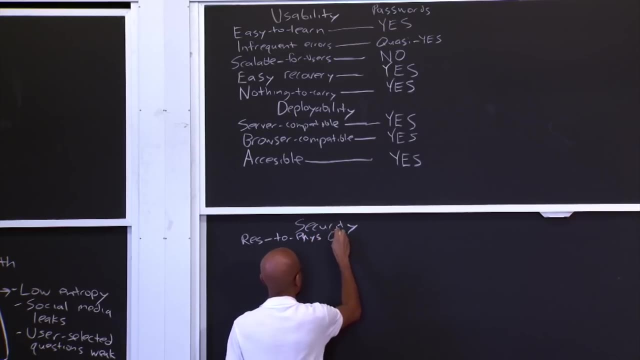 So a lot of these security properties are sort of resilient to foo, right. So I'll just sort of shorten that with res. So is the scheme resilient to physical observation, right? So the idea here is that an attacker cannot impersonate a user after observing them authenticate a few times. 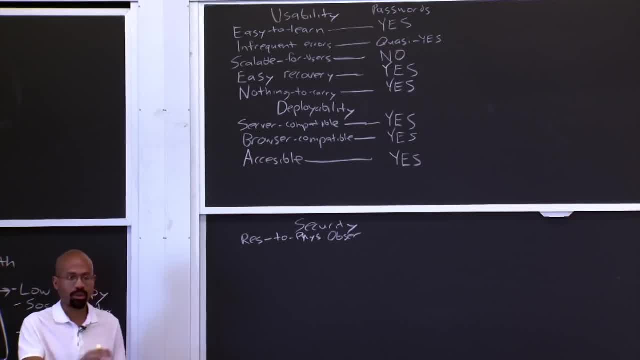 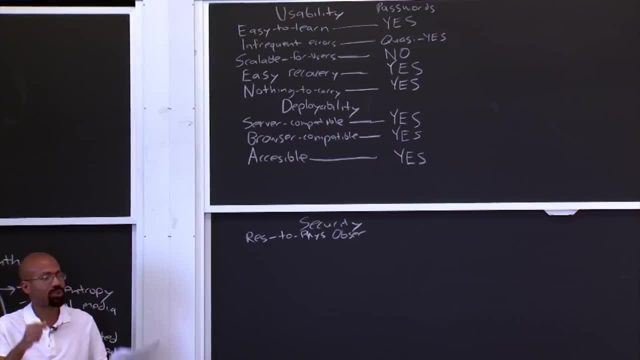 So imagine that you had a shoulder surfer. So you're somewhere in a computer lab. Someone's looking over your shoulder seeing what you type in Right. Imagine someone's videotaping you- Maybe someone's got a microphone They're listening to, sort of like the acoustic signature. 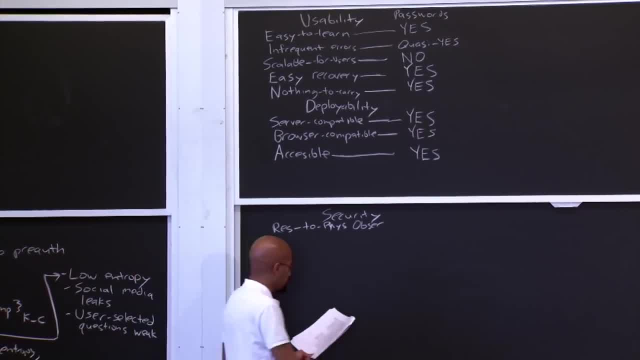 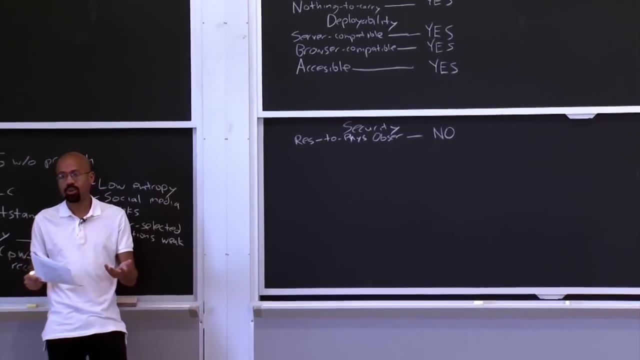 of your keyboard and trying to extract things from that, so on and so forth. So the authors say that passwords actually fail this test And that's because if someone can videotape you typing in things, they can pretty easily figure out what letters you typed. 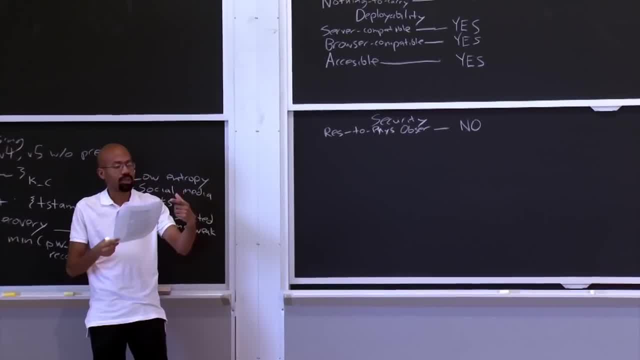 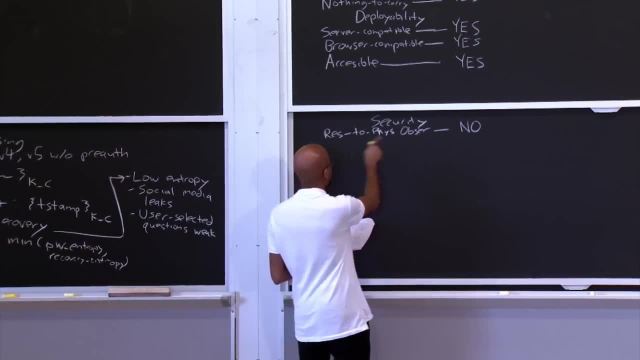 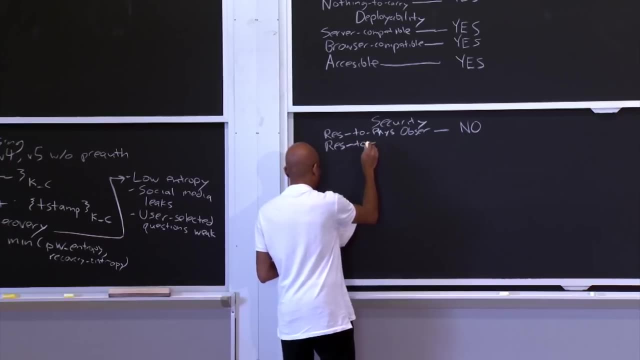 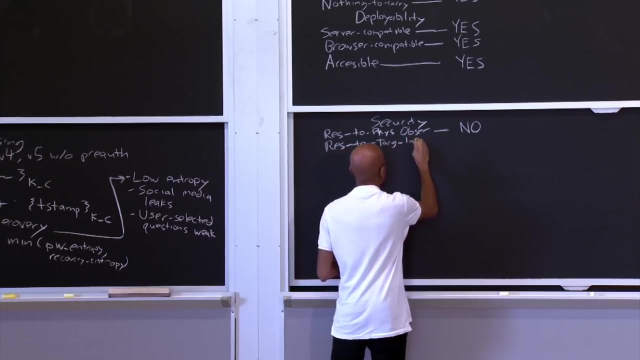 Or there's actually these attacks where you can actually listen to the acoustic fingerprint of a keyboard and detect what was typed based on what sounds that you hear. So passwords are not resistant to physical observation, So another property is resistant to targeted impersonation, And so the basic idea here is that is it? 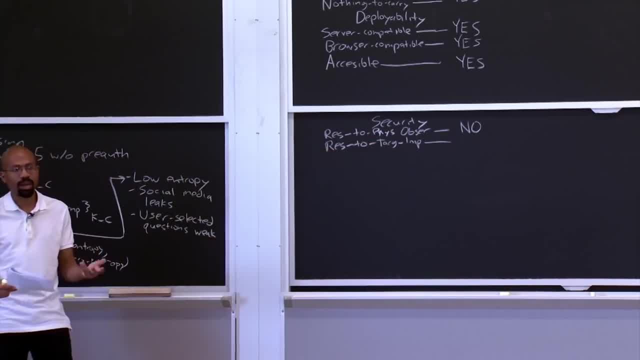 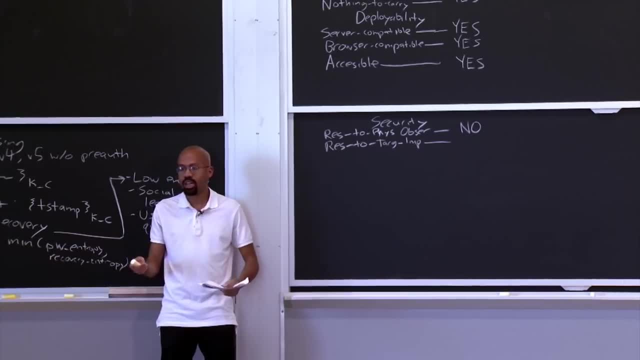 possible for someone who knows you- a friend, an acquaintance, a spouse, a loved one, a family member, whatever- to impersonate you using their knowledge of who you are and what you do. Right, So could your friend try to pretend to be you easily. 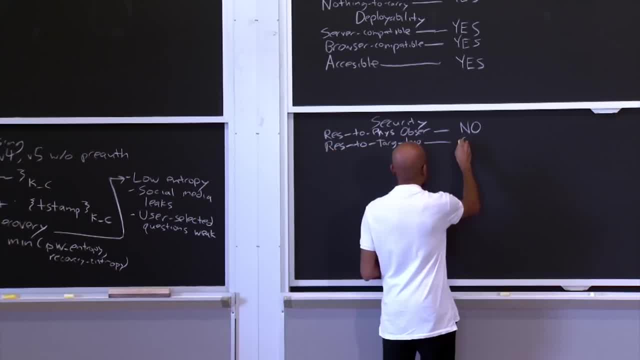 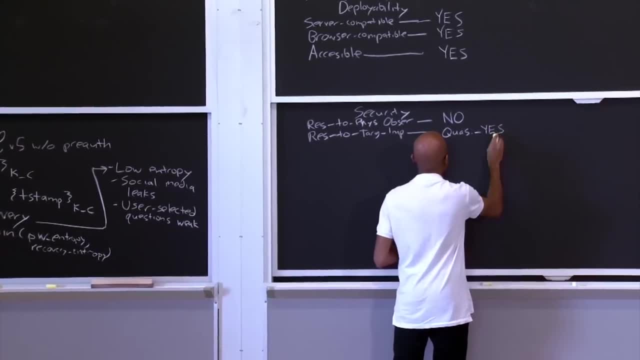 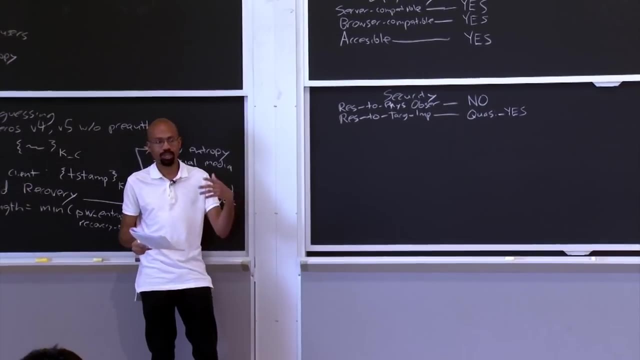 in this particular scheme. So here the authors basically have another one of these quasi yeses. And they say quasi yes because they're not aware of any studies which show that if you know a person, you're more likely to be able to guess their password. 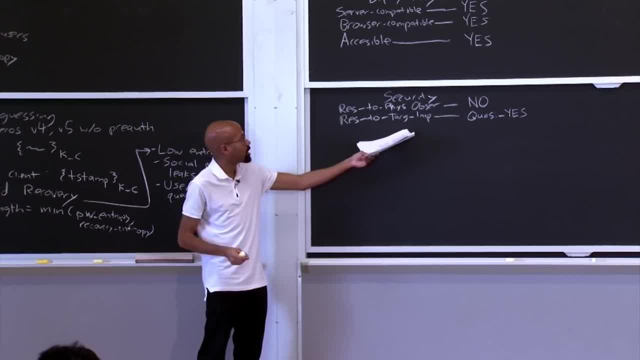 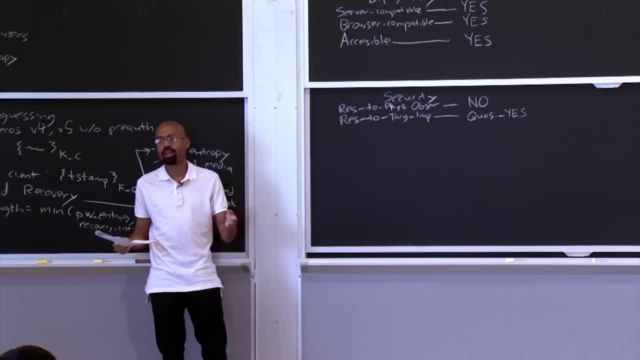 So they say quasi yes for that, And so note that resistance is targeted, It's targeted impersonation. This is where most security backup questions fail miserably, because if someone knows something about you quite easily, they can sort of guess your security. 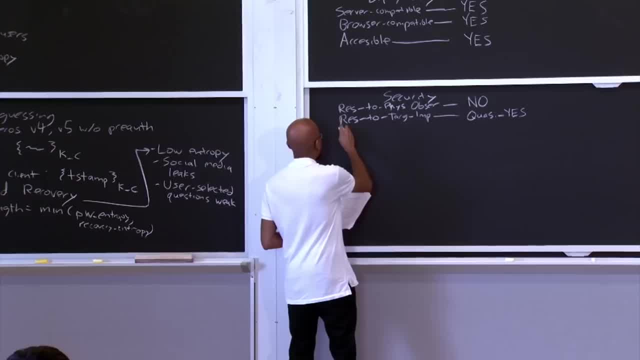 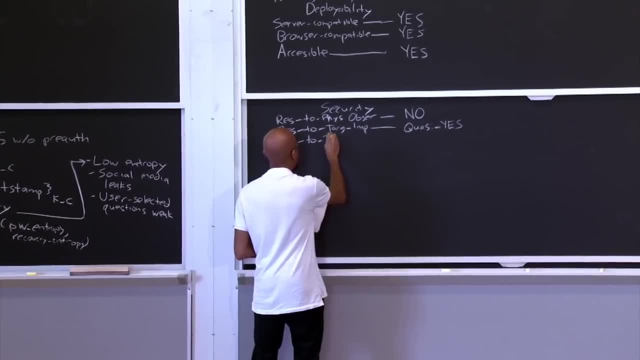 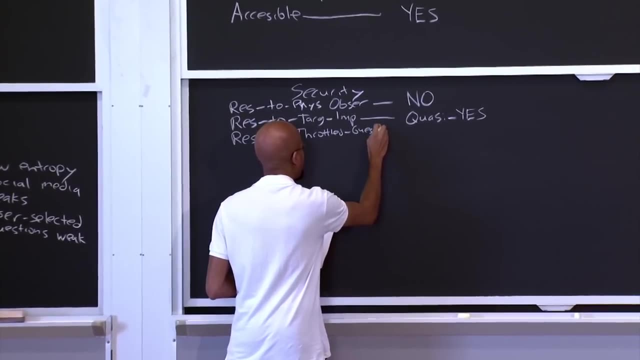 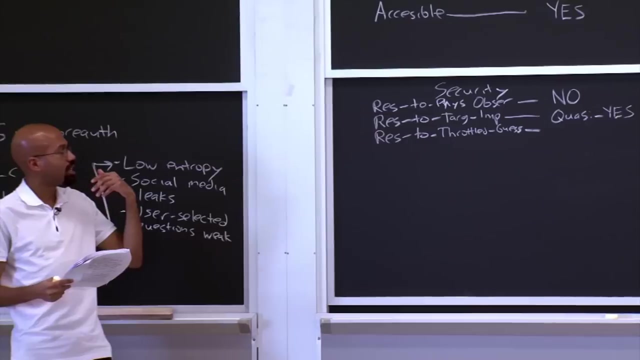 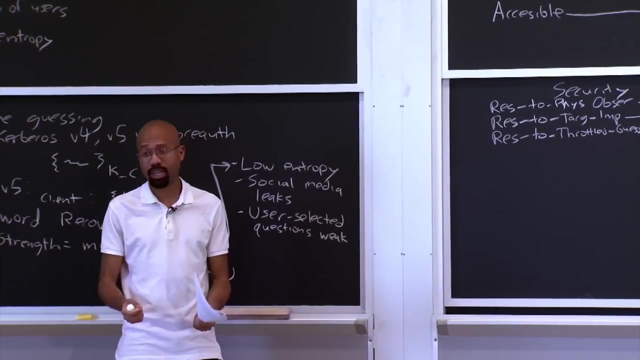 questions in many cases, All right. so then we have two categories that involve guessing. So the first one is resilient to throttled guessing, And so what this means is If the attacker cannot issue guesses at line rate because, for example, the server uses anti-hammering mechanisms, 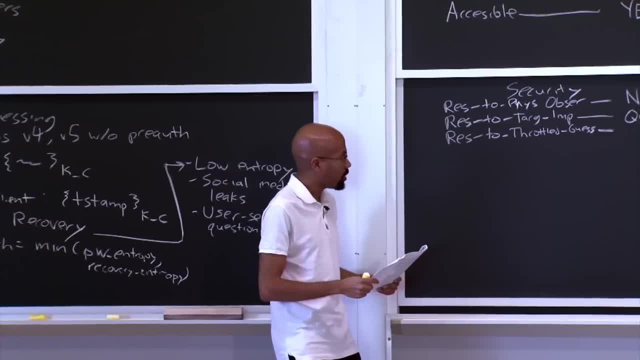 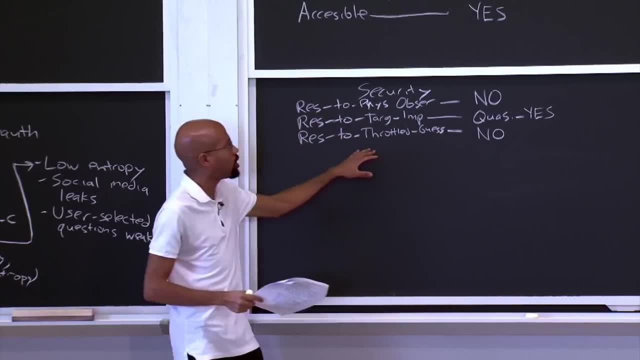 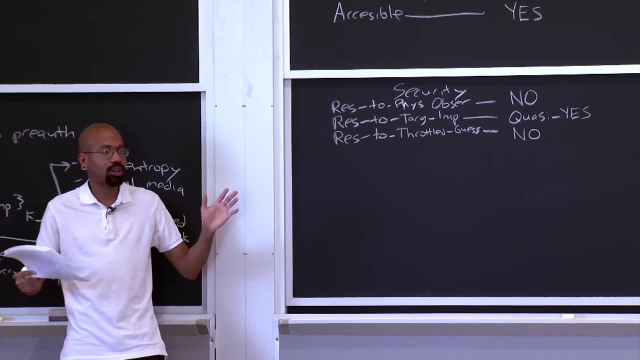 is the scheme safe against the attacker? And so here they say no. And so the reason why they say no is because in practice, passwords not only have sort of low inherent entropy, because they're not that long, but also they have that skewed distribution. 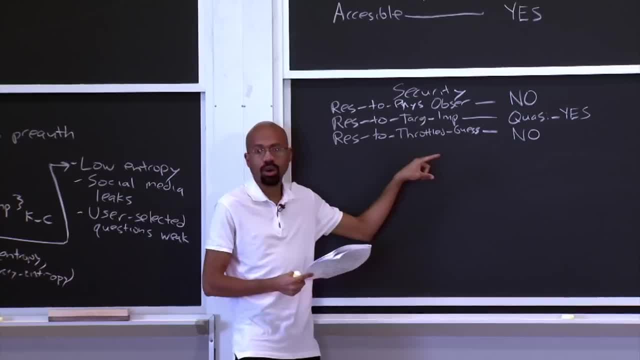 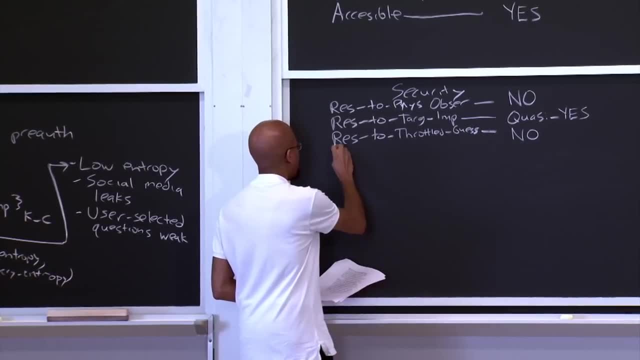 And so what that means is that even if the attacker is throttled in some way, typically the attacker can still make good forward progress and crack a lot of people's passwords. So they define another guessing property which is resistant to unthrottled guessing. 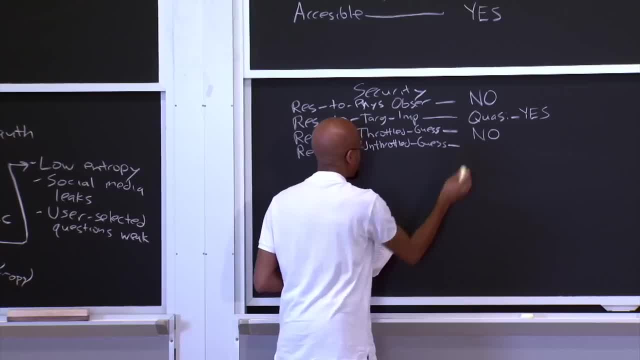 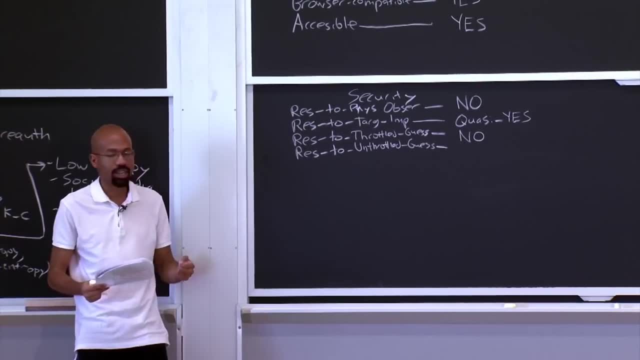 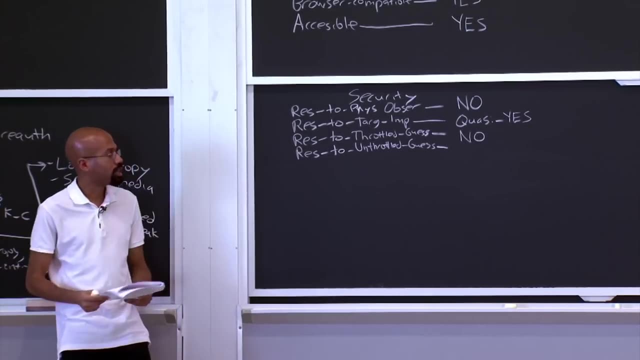 And so this is basically saying: Suppose that the attacker can issue these authentication forgery requests as quickly as he or she wants. So in other words, the attacker is only limited by the speed of their hardware. So is the authentication scheme resilient to that type? 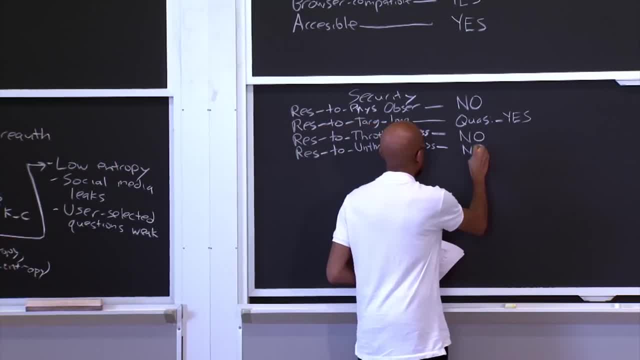 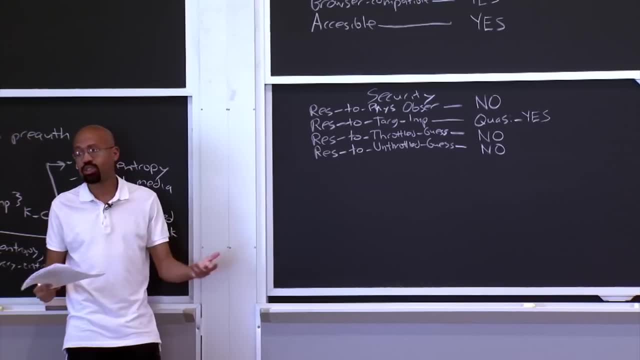 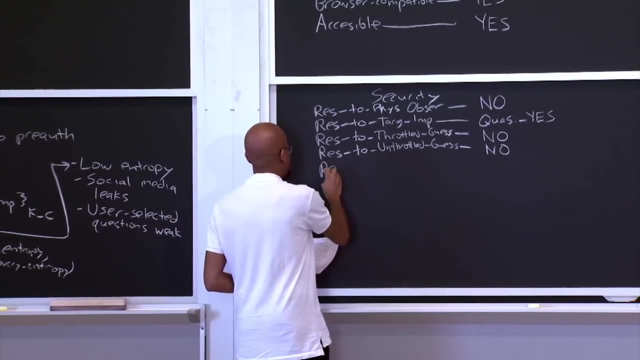 of attack, And here this answer is also no, for the same reason that the answer was no up here. So basically, passwords have a very small entropy space and they come from the skewed distribution. So that's all pretty straightforward. One interesting one is resiliency. 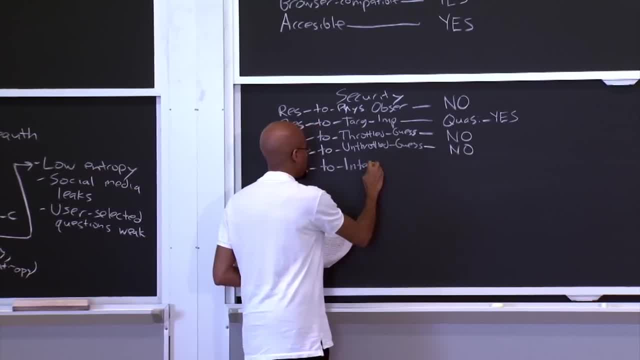 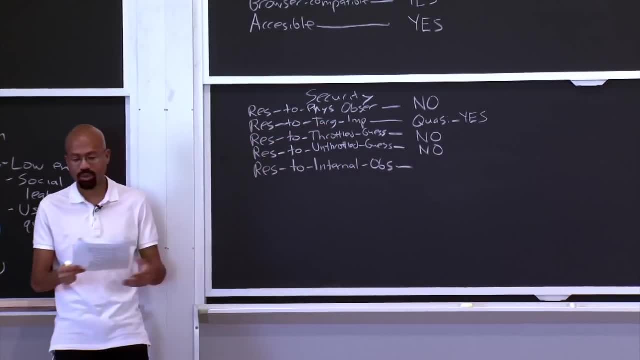 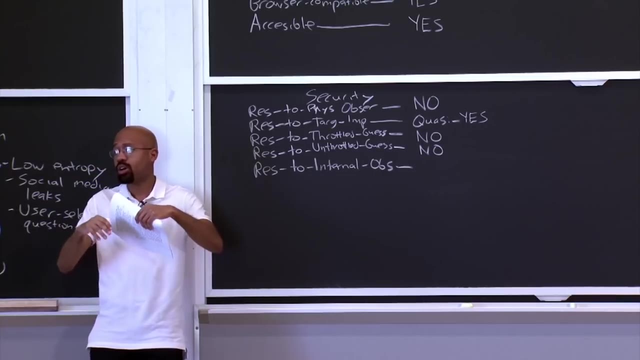 to internal observation. So this means that the attacker cannot impersonate a user by intercepting that user's input, For example by installing a keystroke logger on the keyboard that the user is using and using that logger to steal key presses. This also means, for example, that there's 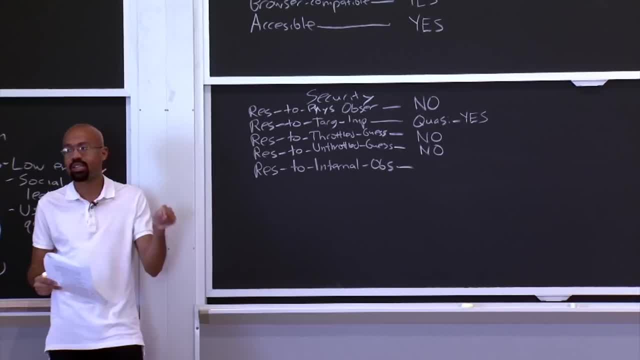 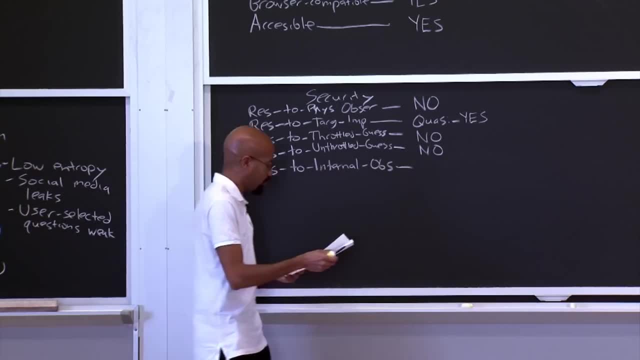 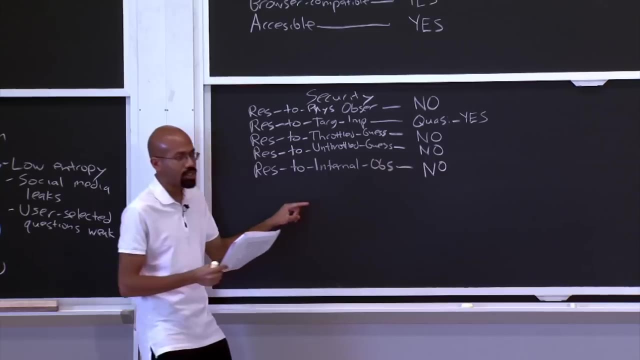 no way for a network attacker, who's observing the things that the client's sending over the wire, to use that knowledge of the network traffic to later impersonate the user. And so here they say: passwords do not have this scheme. And they essentially say it's because passwords. 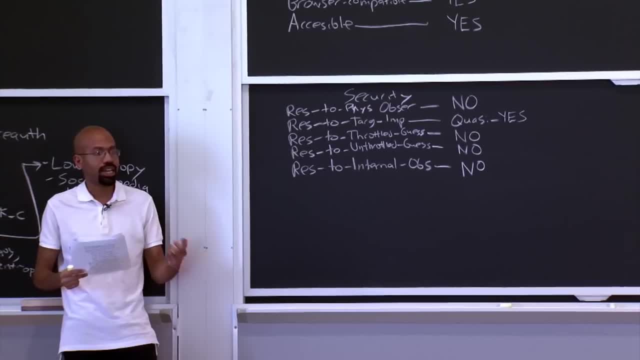 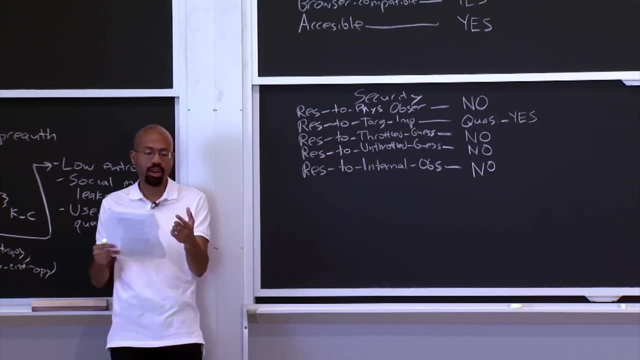 are static tokens. They don't change And typically static tokens are vulnerable to replay, right? So if somehow, for example, an attacker installs a keystroke logger and gets your password, then basically the attacker can use that password until it's either expired or revoked or something like that. 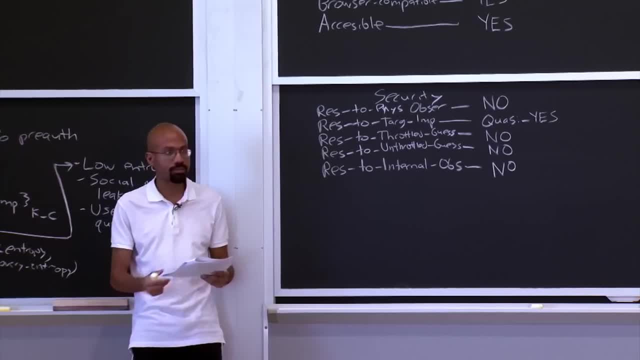 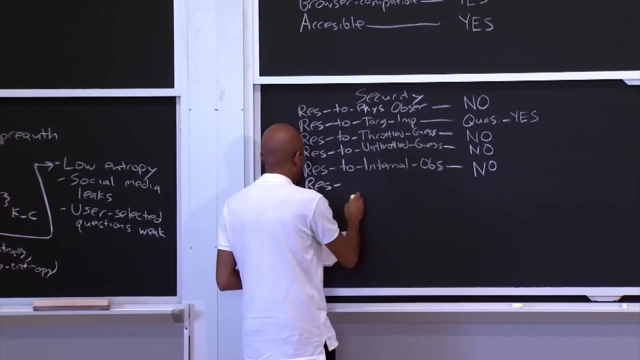 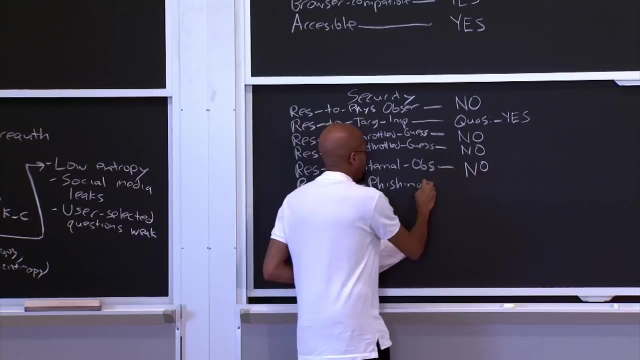 It can just replay it again and again to that authenticating server on the other side. So here passwords actually fail that test. Another thing that we've talked about a little bit in this class: phishing. So resilience to phishing is another Security metric. 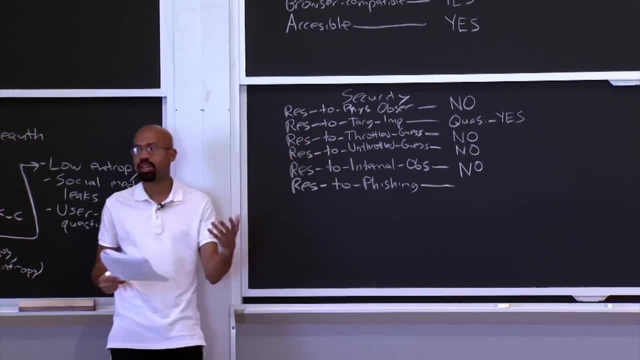 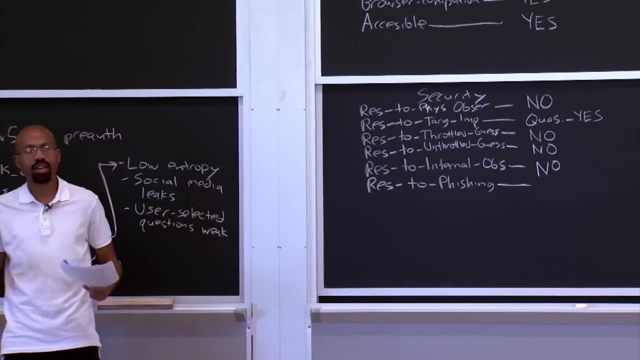 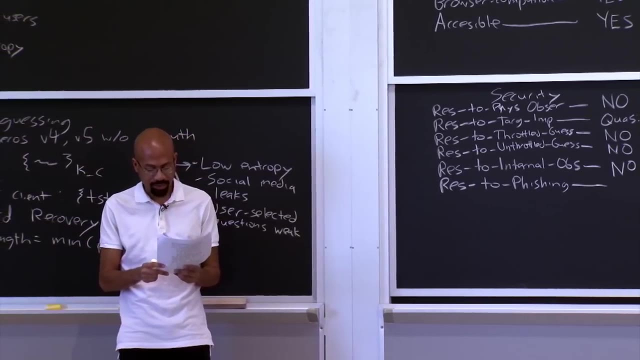 And the basic idea here is that if the attacker can simulate a valid service, for example by attacking the DNS infrastructure or something like that, then the attacker cannot collect credentials from the user that the attacker can then use to pretend to be the user later on. 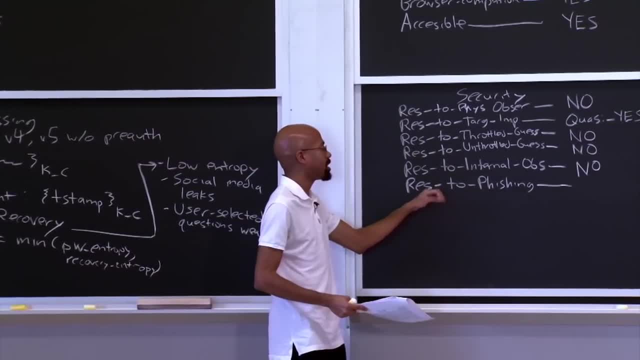 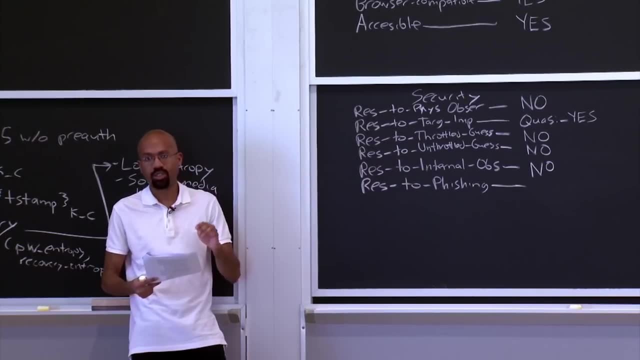 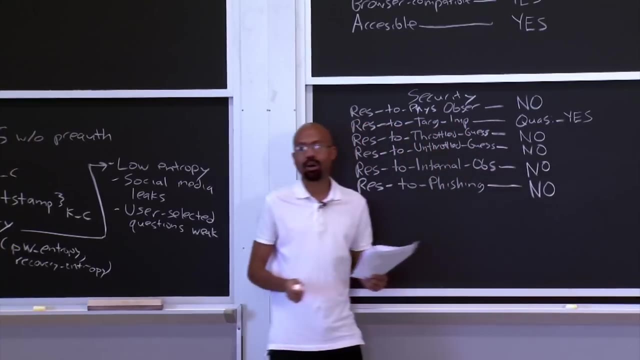 And so this, basically, is supposed to penalize sites that do not strongly tell the user: hey, I'm this particular service, so you can feel confident to give me your credentials. And so here passwords fail just because phishing sites are very, very popular. 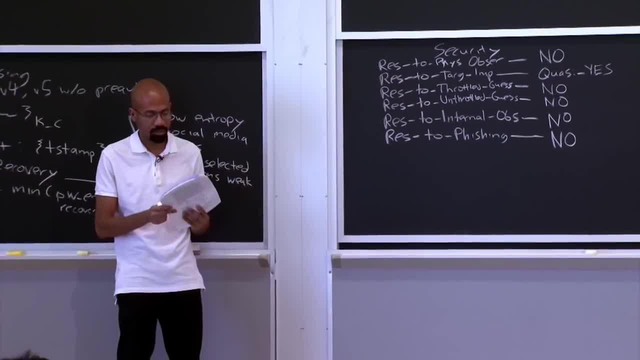 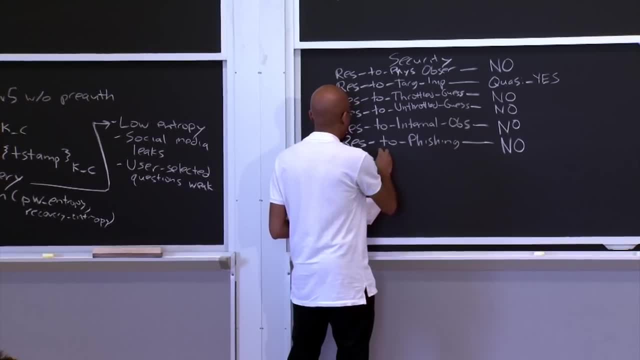 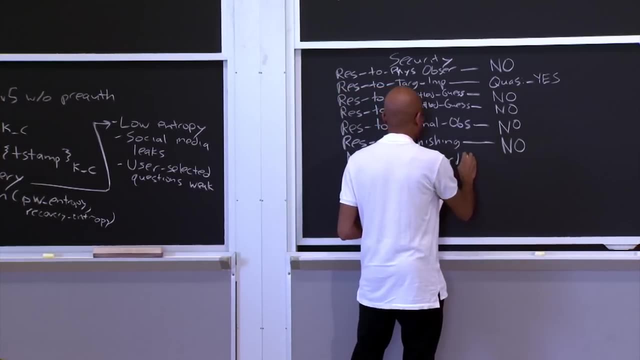 So passwords don't really intrinsically provide any protection against that. Now the next two are particularly interesting in the context of a large-scale distributed system. So no trusted third party. This essentially means that Other than the client and the server, 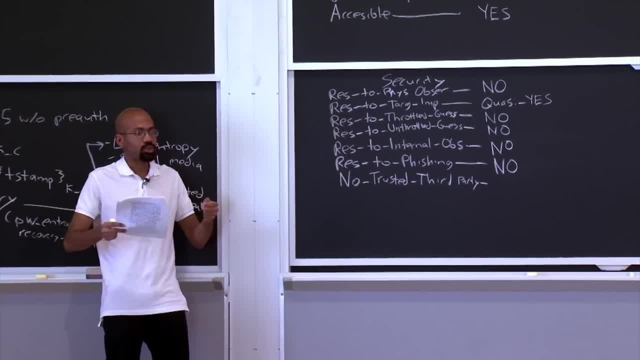 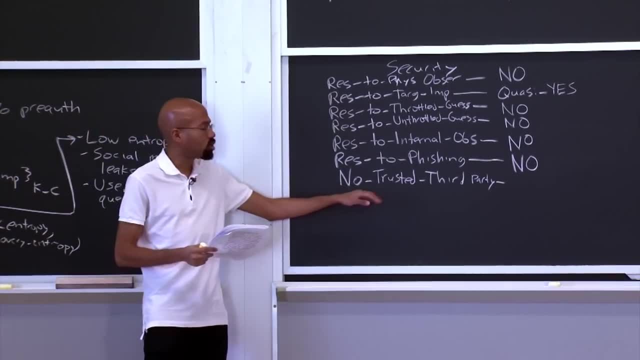 there's no one else in the system that is involved in the authentication protocol, And so that means that there's no third party who, if that third party were compromised, the entire integrity of the security scheme might fall apart, And so this is actually an interesting property. 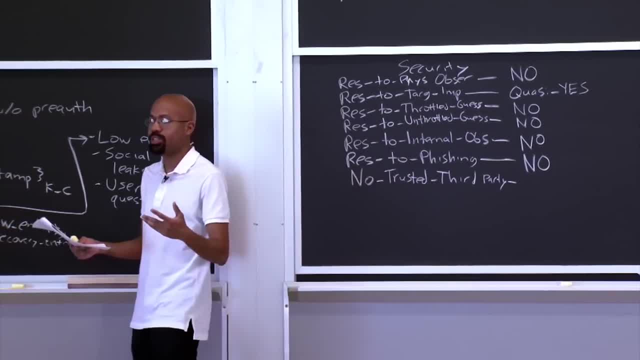 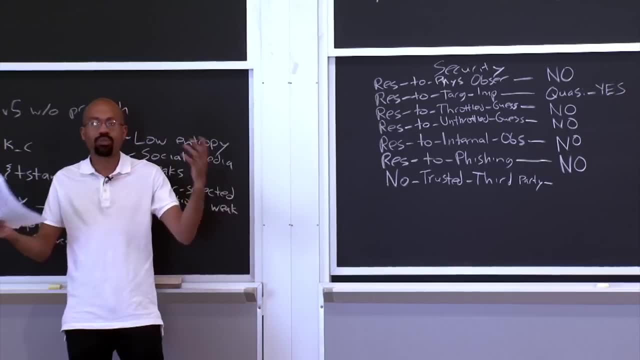 to look at, because a lot of authentication problems would go away if we could just store all of our authentication information in one place. We just store it in one place. It's very simple. We don't have to remember a lot of stuff on the client. 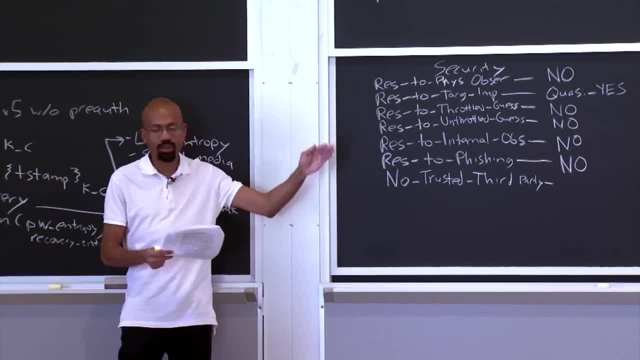 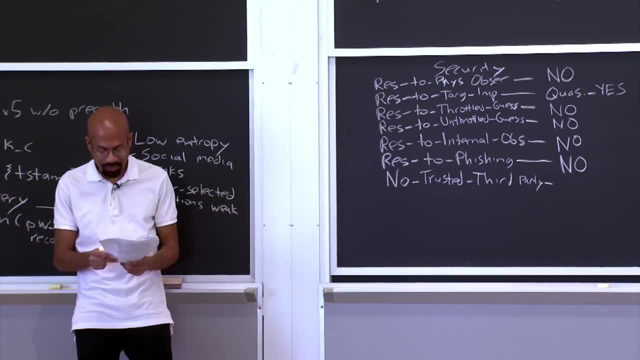 We just say, whatever service you want to use, you always go to this one third party, And that third party will always be able to sort of authenticate you and then allow you to go in your merry way. Now, of course, third parties are. 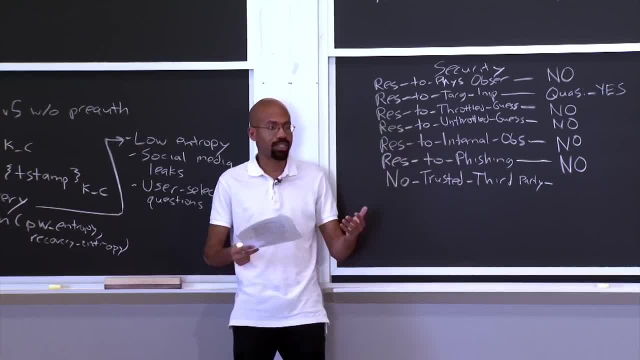 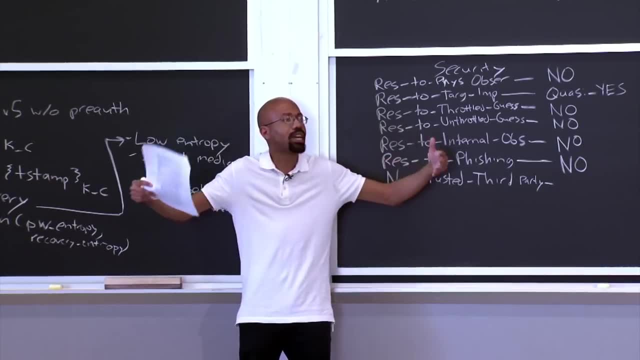 problematic from the perspective of robustness, Because if you do have one of these global third parties that everybody trusts, if that third party gets subverted, then perhaps the integrity of all the sites that use that third party to authenticate all those sites are potentially in danger. 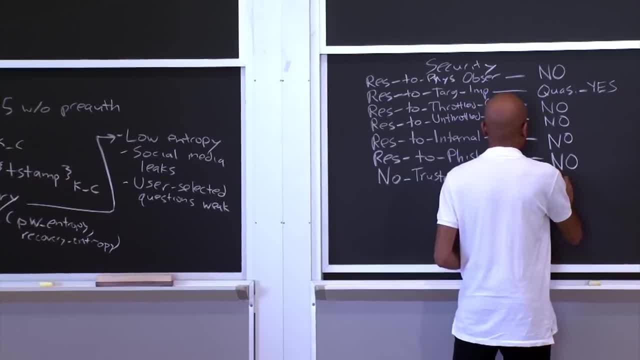 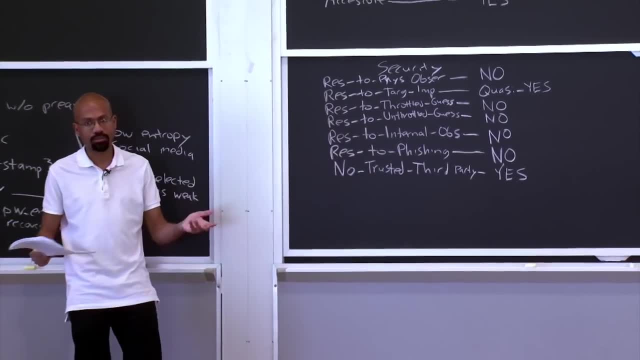 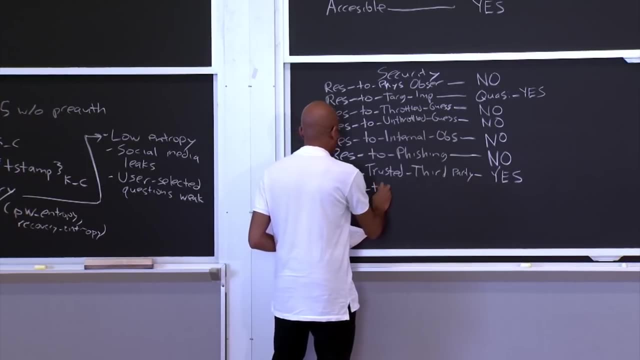 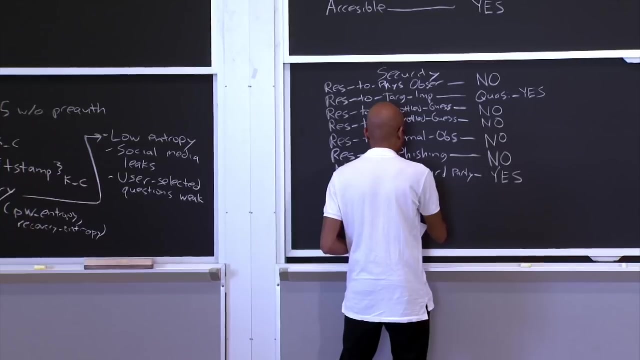 OK, Thank you. So they say that passwords do not have a trusted third party because each user is forced to have a separate password for each site. A related property is resilient to leaks from other verifiers, And by verifiers they just refer to these services. 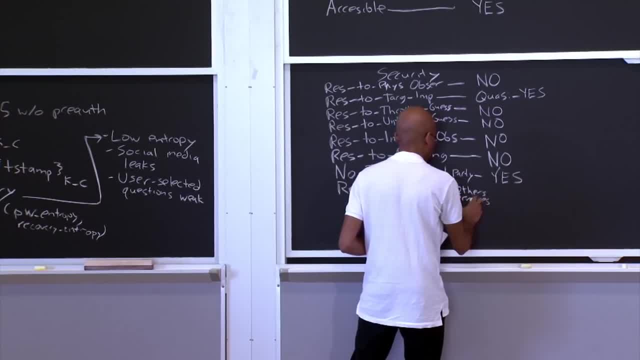 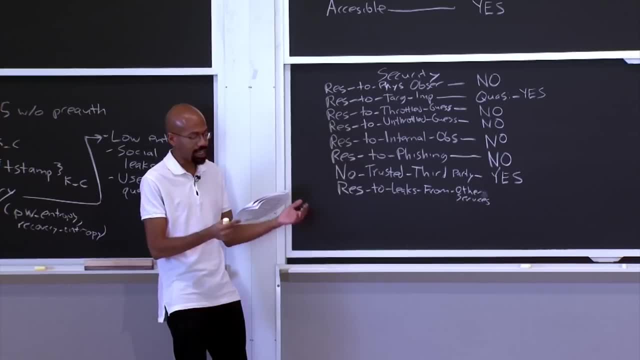 And by verifiers they just refer to these services that you're authenticating to, And so the author just defined this as nothing that a service could possibly leak can help an attacker impersonate the user to another service, So this basically penalizes schemes. 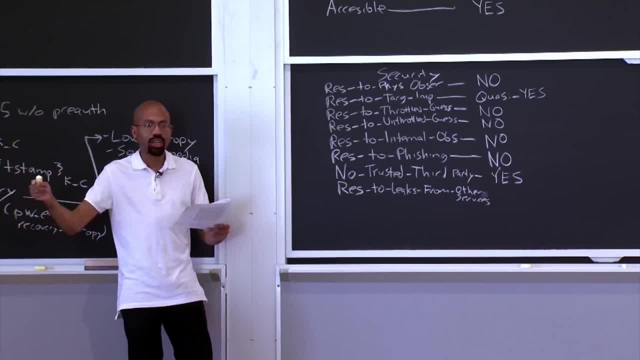 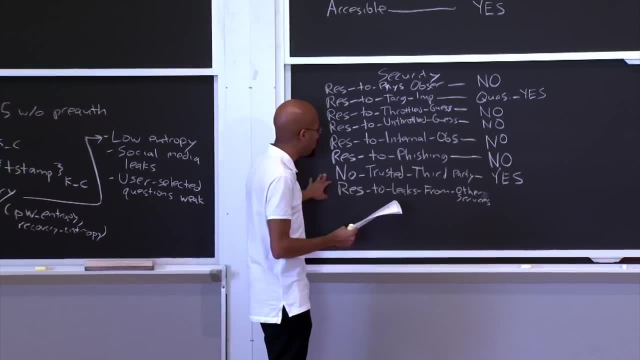 where fraud or malice or incompetence at one particular service will then possibly result in leakage of your credentials at some other service, And so this property is actually related to the no trusted third party scheme metric, Because if you don't want to authenticate, 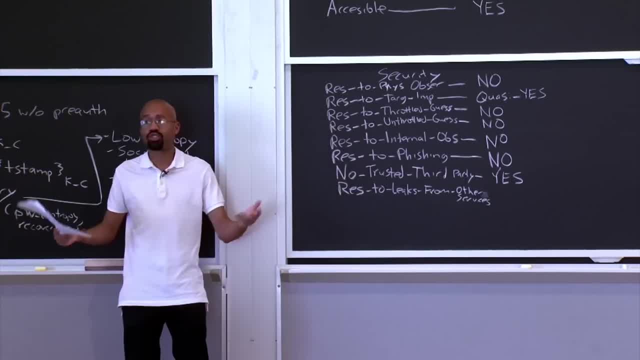 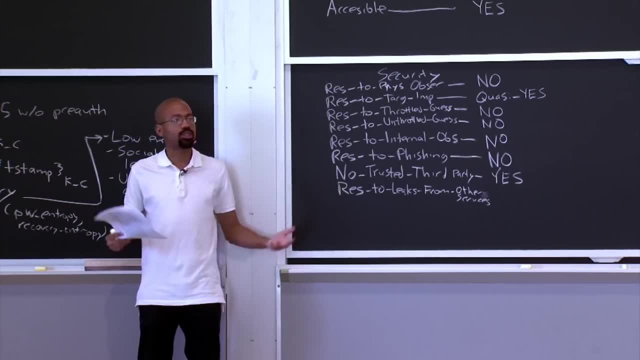 you don't want to trust the third party, then automatically you start thinking we want some type of distributed authentication system. But the problem with that then is that you may end up with a situation where the overall security of the scheme is dependent on the security of the weakest link. 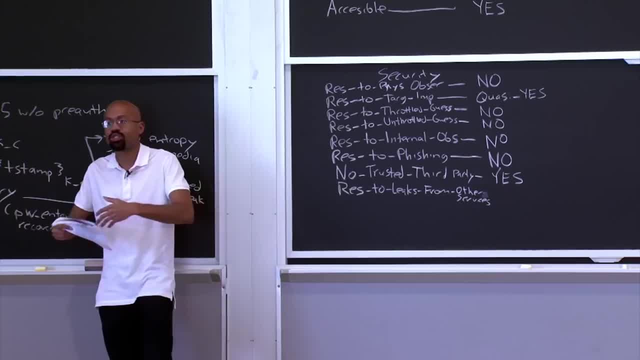 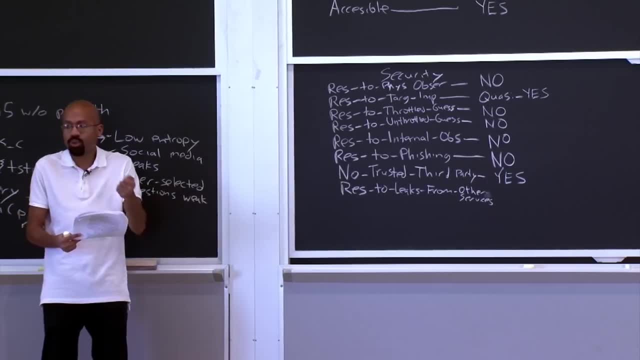 So think once again, like HTTPS, like the certificate authorities. In certain sense that's the distributed authentication system, But the problem is that if one CA gets subverted, then that means that person can issue fraudulent certificates for a bunch of different parties. 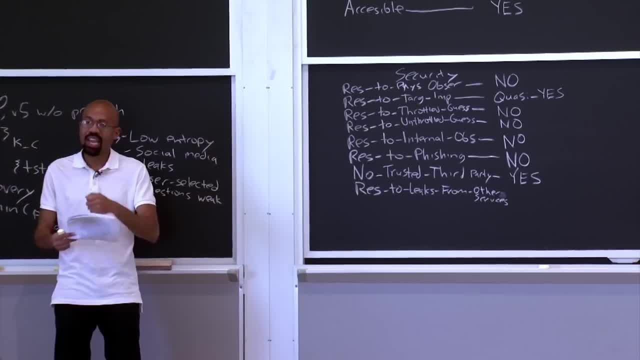 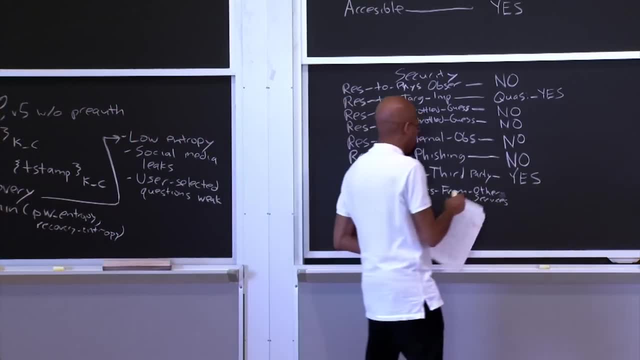 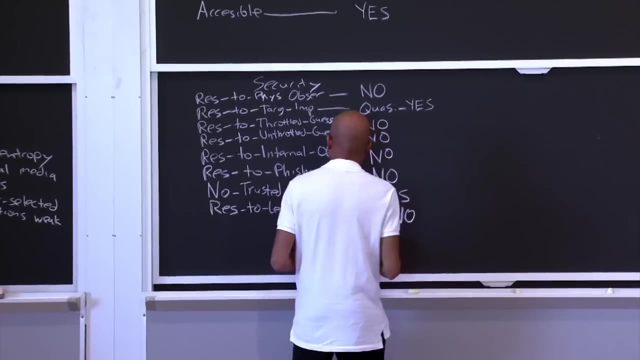 And so if you, if you, if the world ever makes a mistake and gives CA power to someone who's untrustworthy, then potentially the whole thing can fall apart. And so the authors say here that this is a no for passwords. So they say that because people often reuse passwords. 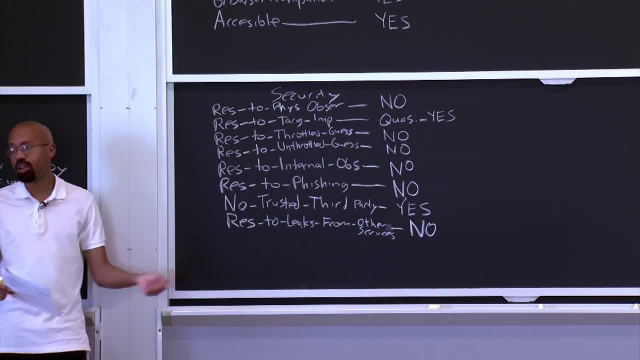 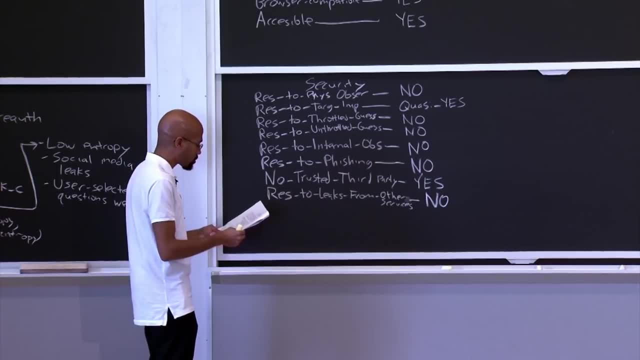 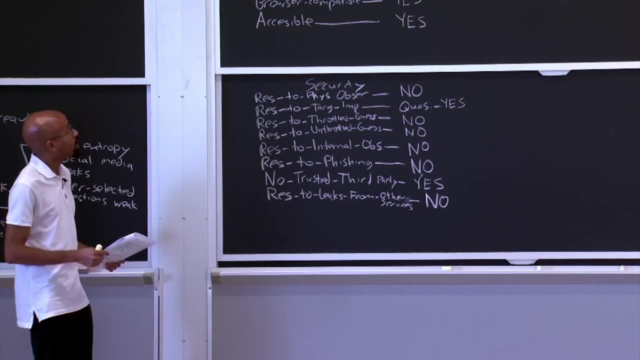 across the same site. if, let's say, my Gmail password's stolen, then maybe that means that my Facebook password has been stolen too. So the authors give a no there for passwords. So this is just an overview of some of the more important categories that the authors look at. 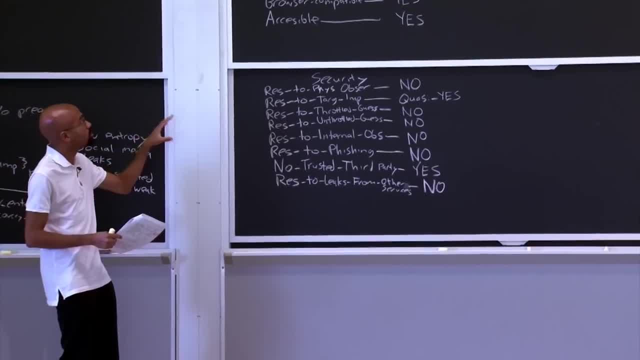 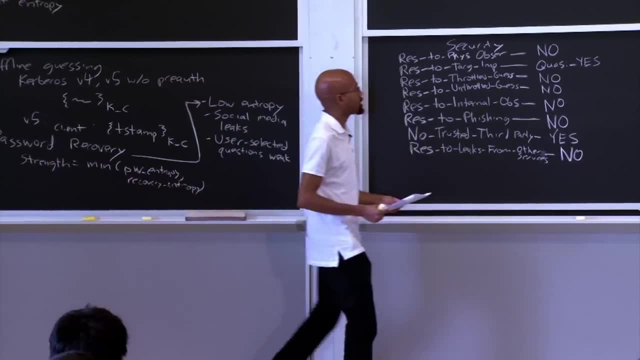 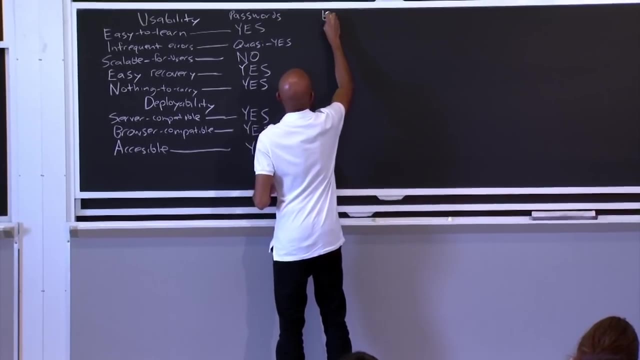 And so these things are only useful when you compare them to the scores that some other system might have gotten. So one interesting system to compare against is biometrics. So biometrics At first glance seem like a super cool thing to do, right? 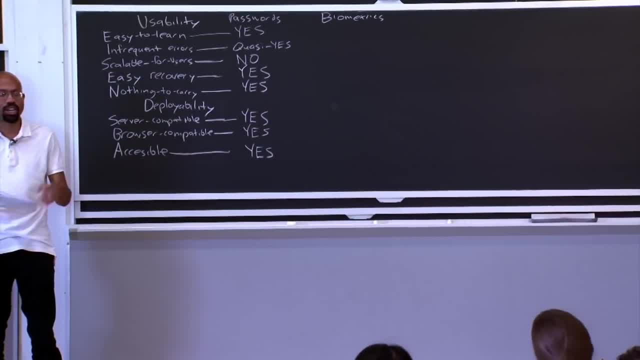 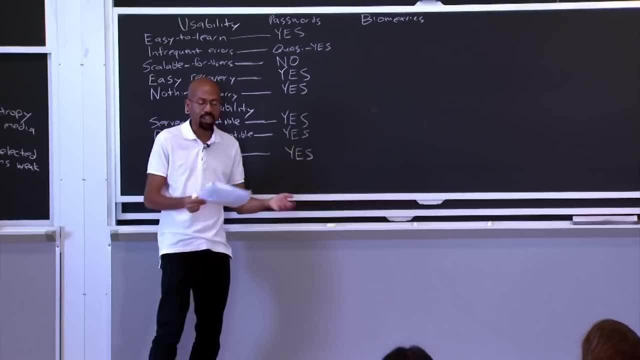 And so, in fact, a lot of times when you go watch science fiction movies, everybody's looking at iris scanners and putting their fingers in some type of palm reader or things like that. It seems very futuristic, right? So basically, biometrics leverage the unique aspects. 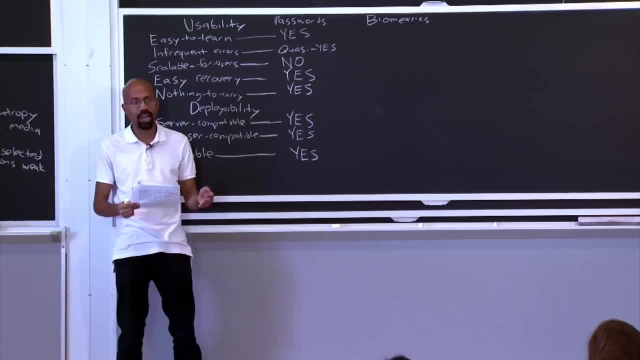 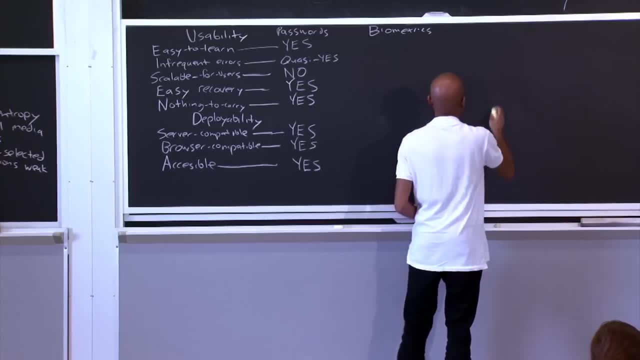 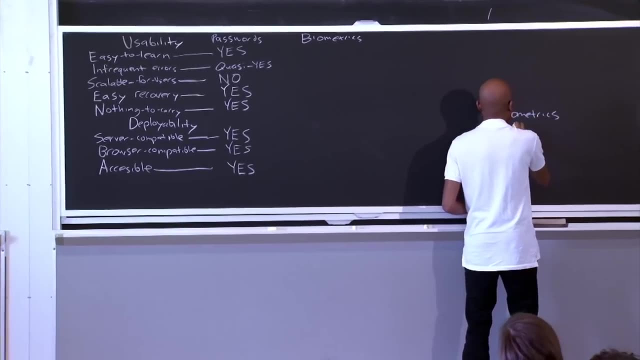 of someone's body or the way that they gesture or things like that to authenticate the person, And so one thing that might be interesting to think about is: how big is the key space? Actually, I'll put this over here, So the key space is actually not as big. 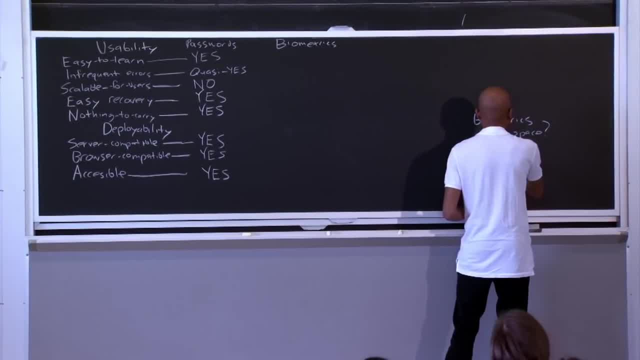 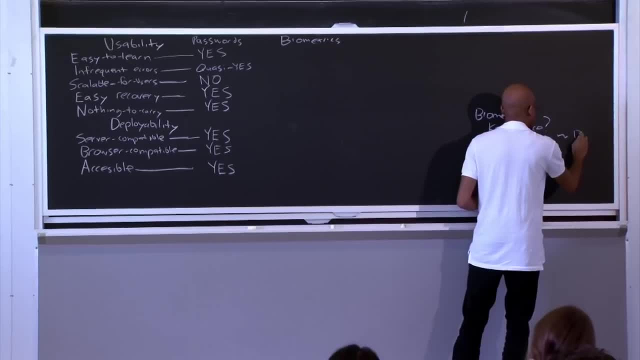 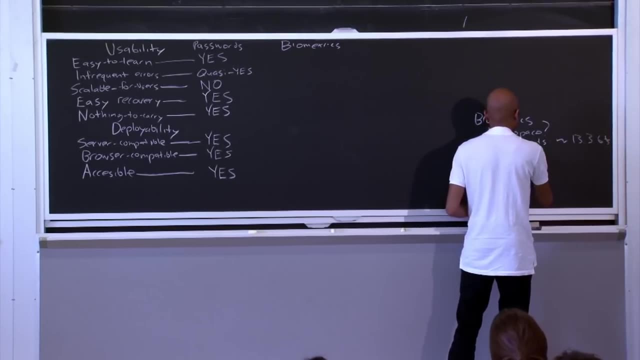 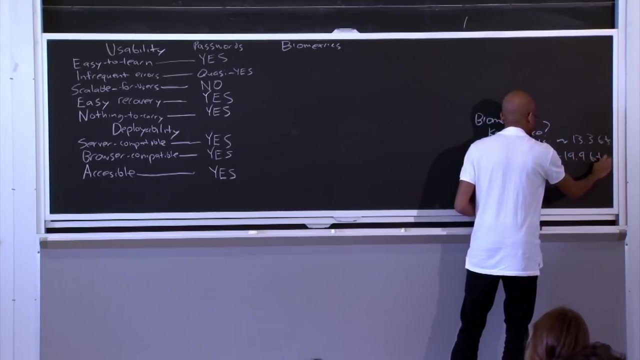 as you might think that it would be. So, for example, for fingerprints, the key space is roughly 13 bits. If you look at iris scanning, the amount of entropy is roughly 20 bits, And if you look at voice recognition, then you'll see that the amount of entropy 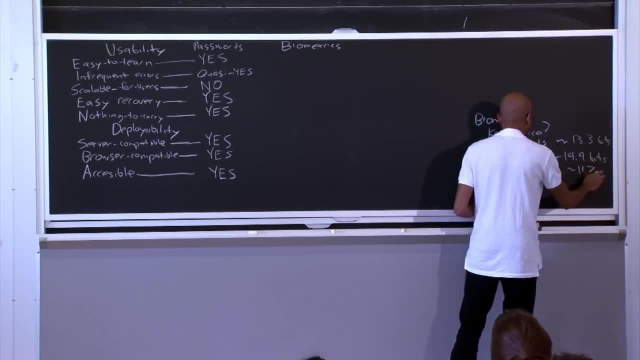 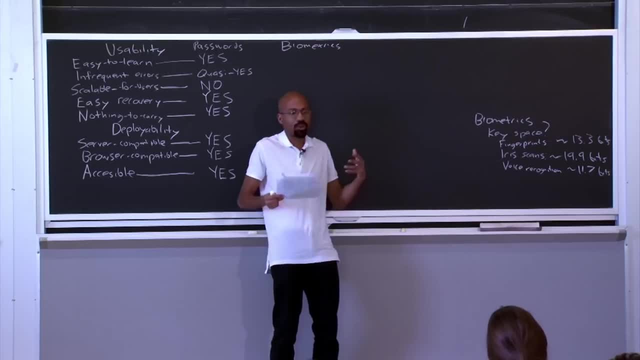 is roughly about 12 bits, And so this seems perhaps a little bit concerning, in as much as we have all these hopes that biometrics are from the future and they're going to really help us, But when we look at how much entropy they have, 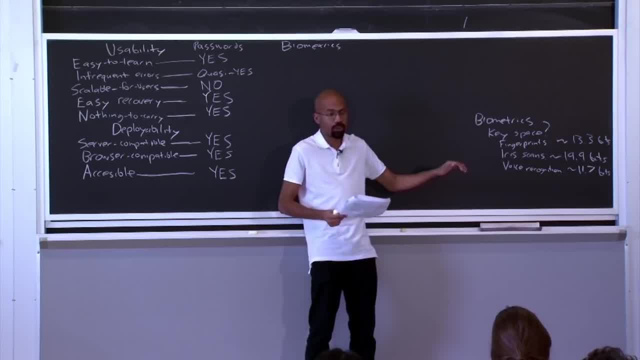 they actually are not that much better than passwords. Actually, they're roughly equivalent Because, if you remember, passwords have roughly 10 to 20 bits of entropy. So that's a little bit disturbing. But whatever, we'll continue and we'll eventually. 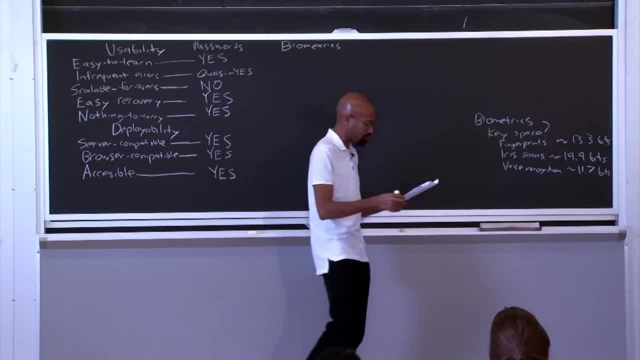 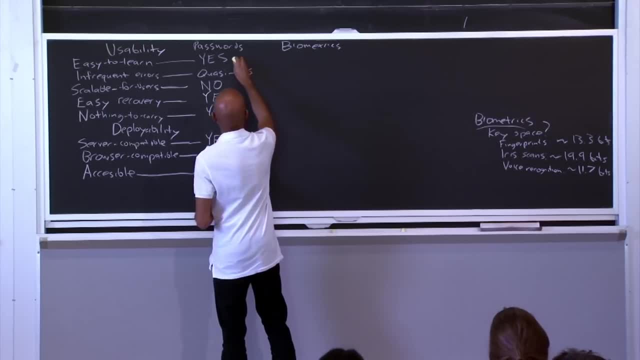 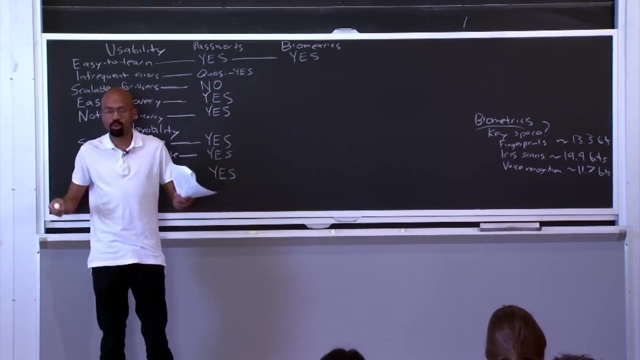 see how biometrics stack up versus passwords, And so how do they stack up? So, according to the authors, biometrics are easy to learn, And that's because presumably, you know how to move your body around or look at things in an iris scanner. 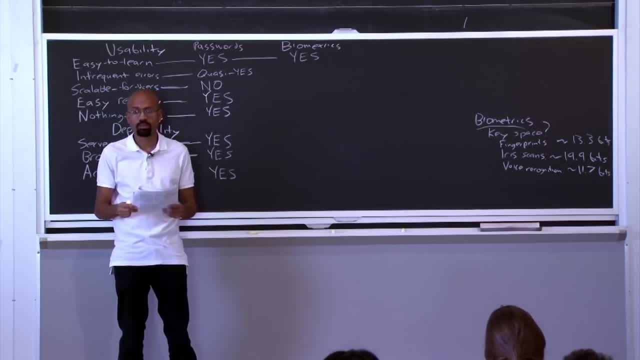 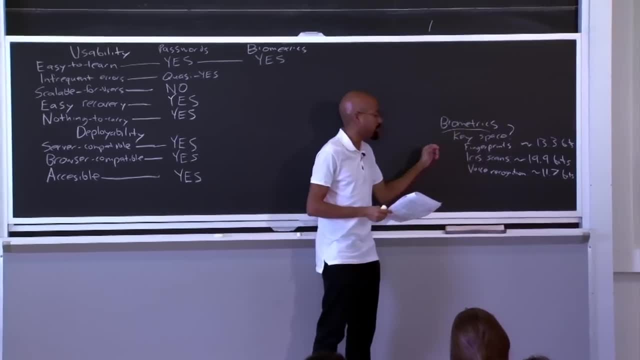 OK question. So are those numbers from the documentation? No, They're just technology- scanning things- or are they just a fundamental part of your sequence? So I believe that they are. well, let's put it like this. So I think that current hardware 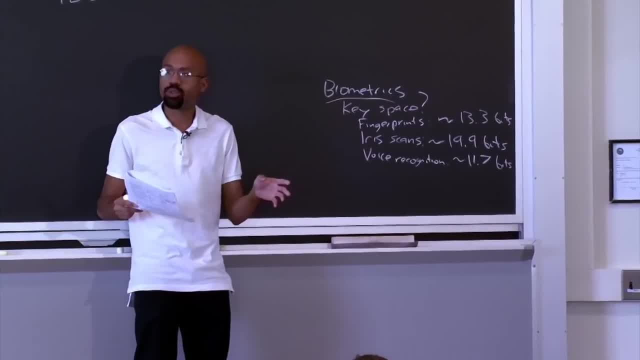 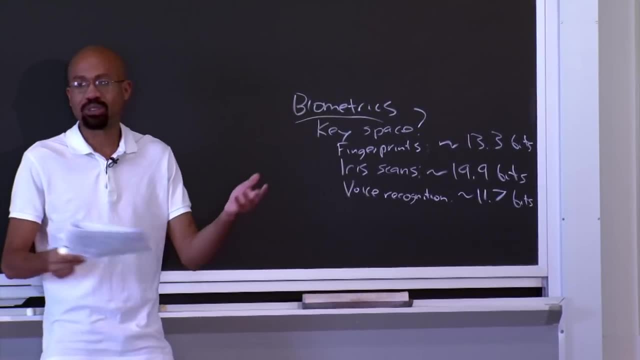 like current authentication, hardware gives you these limits here. I think that if you had higher resolution biometric scanners, you could potentially get better. I mean, presumably there's some lower limit that's guaranteed by the uniqueness of your DNA or things like that. 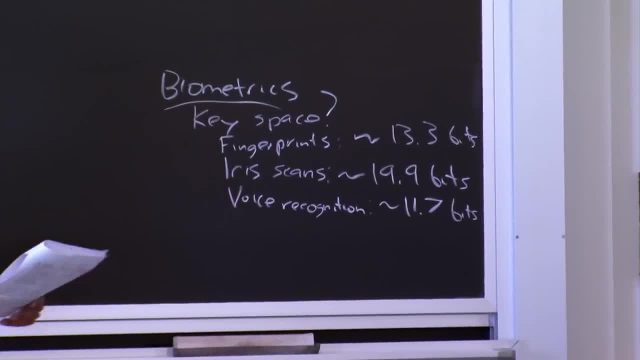 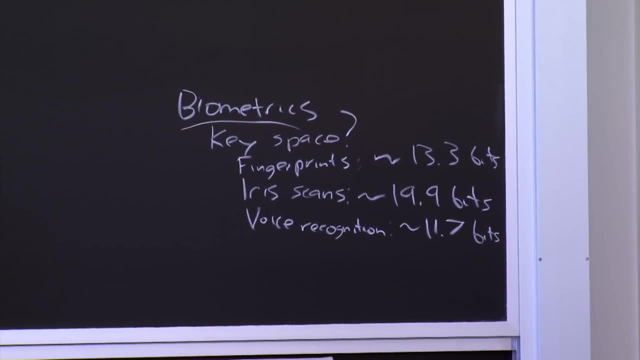 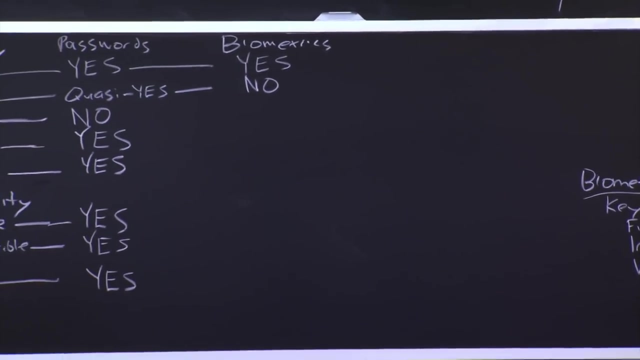 But yeah, I think these are not fundamental limits. So yeah, Authors say that biometrics are easy to learn because it's pretty easy to use these biometric scanners. What's interesting is that biometrics have frequent errors And that's actually a bit problematic. if any of you 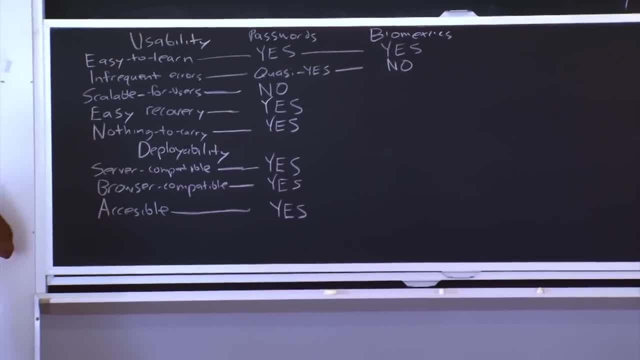 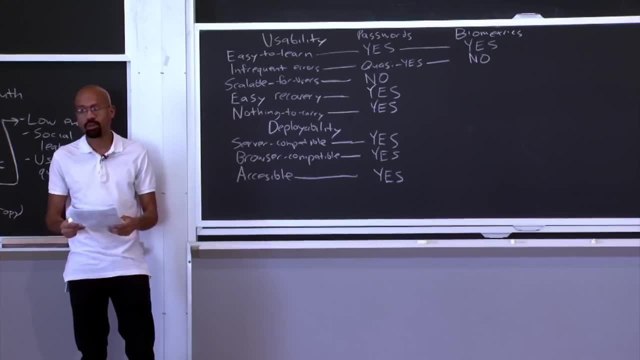 have ever tried to use these things. So, for example, like vocal recognition, So if you have a cold or your voice is a little bit hoarse because you've been yelling at a concert all day, or whatever, these things actually fail fairly regularly. 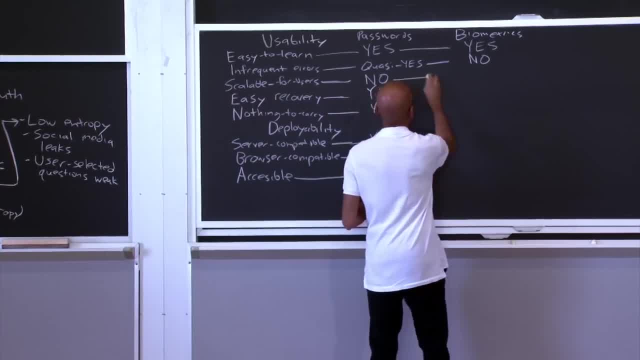 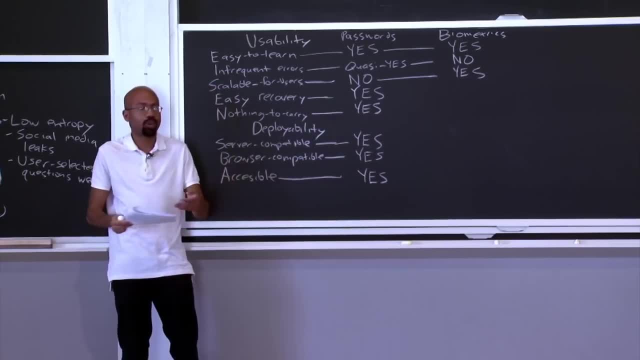 So biometric scores- a no on this. Scalable for users. So this is a yes Because basically you just bring yourself to whatever service you want to authenticate to And then you can just sort of authenticate like magic. So that's a very nice property. 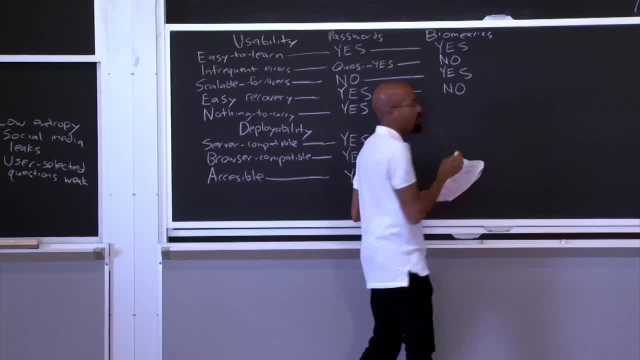 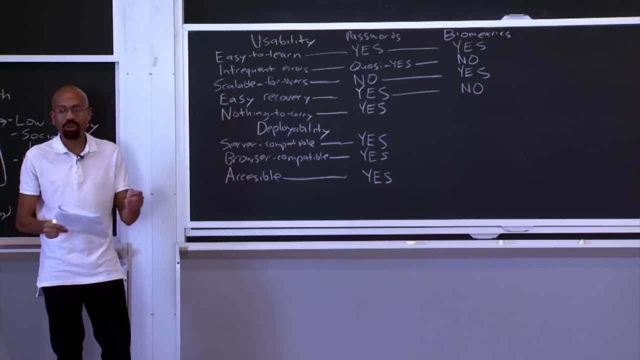 With respect to ease of recovery. so this is a no, And this is actually one of the big problems with biometrics. So let's say somebody somehow manages to steal your iris scan, for example. That person can replay that arbitrarily, Like you can't get new eyes. 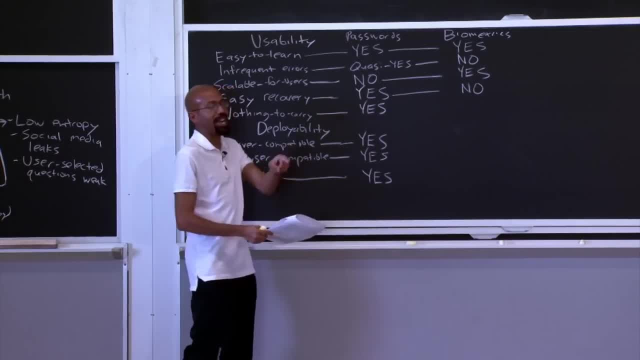 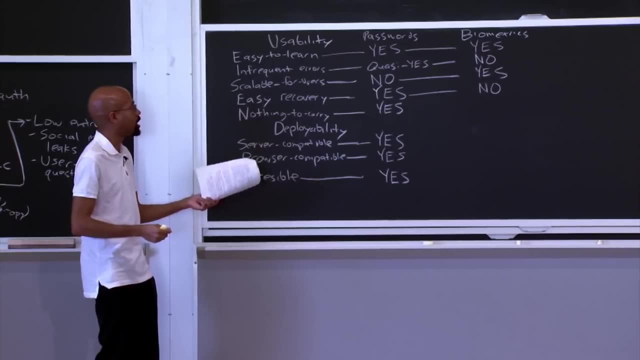 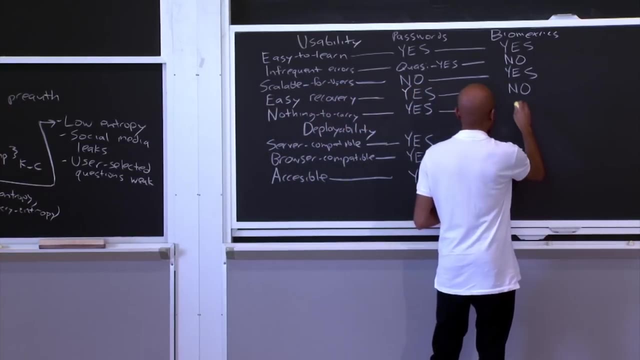 So that's not yet Exactly. That's right, Not with that attitude. yeah. So yeah, until getting new eyes is something Amazoncom will sell easy. recovery is actually a pretty big problem here, And then for the nothing to carry, biometrics wins. 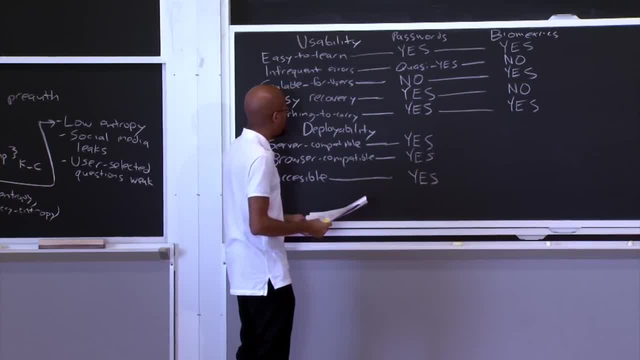 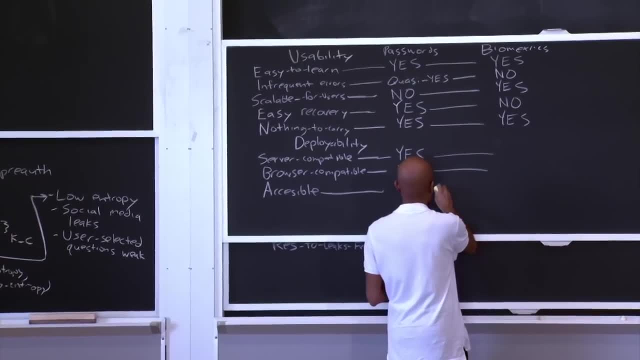 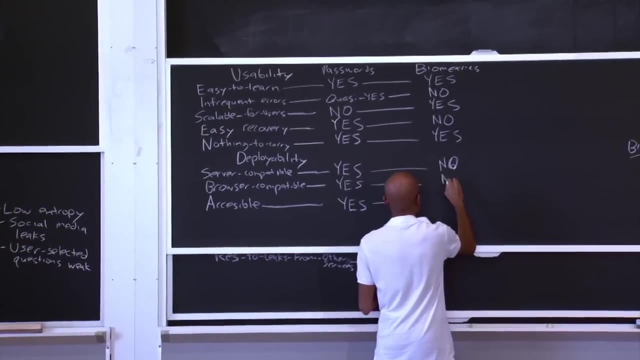 Because you just carry all this stuff with you automatically. So then what about deployability? So for deployability, this is actually not a big win for biometrics. So it is not server compatible. It is not browser compatible because browsers don't have some native API for taking an iris scan or things. 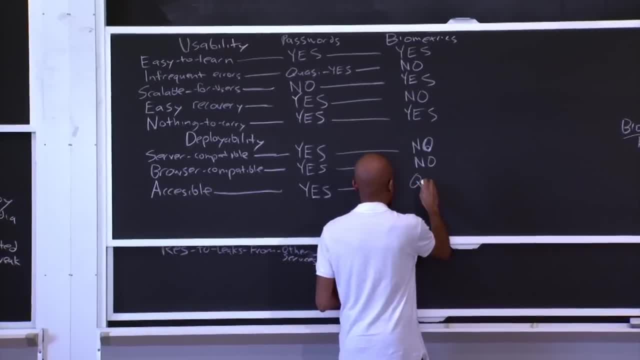 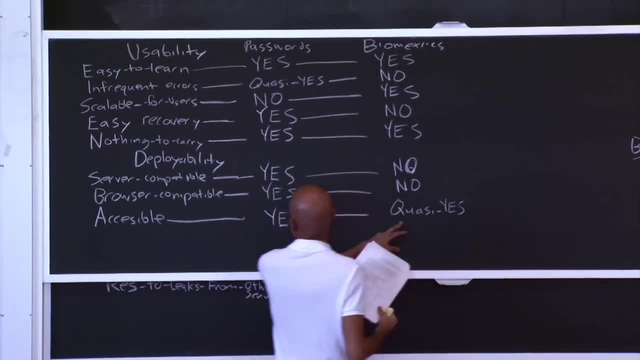 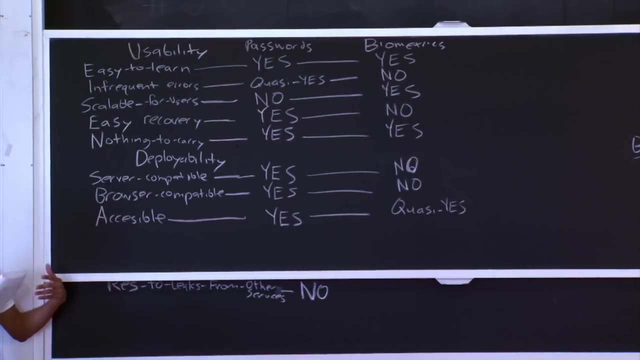 like that In terms of accessibility, the authors say this is a quasi-yes And I think they say quasi-yes because they say that because biometrics are error prone to enter, then this kind of makes it difficult even for sort of regularly able people to use. 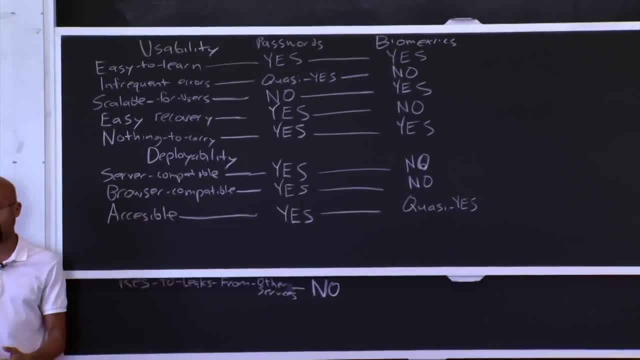 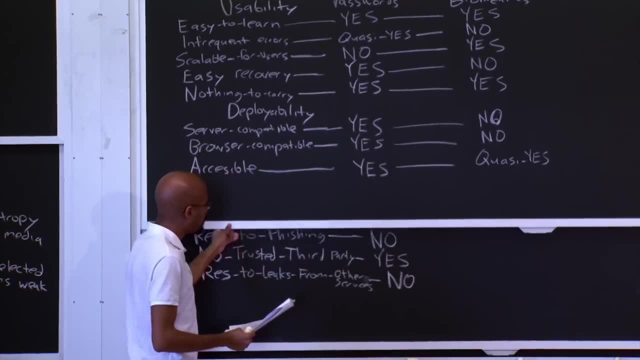 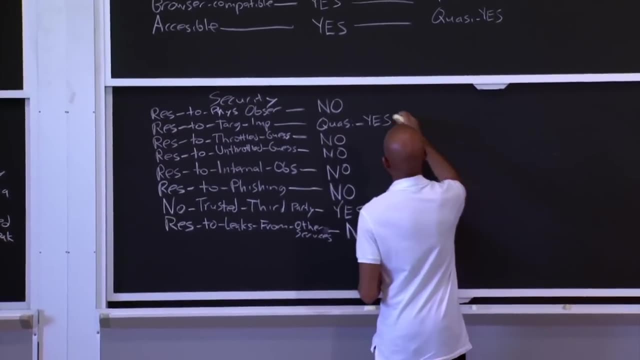 And then if you have some physical impediment, it makes it even more difficult to use some of these schemes. So that's a little sad. So biometrics don't quite seem deployable. So what about on security? So are they resilient to physical observation? 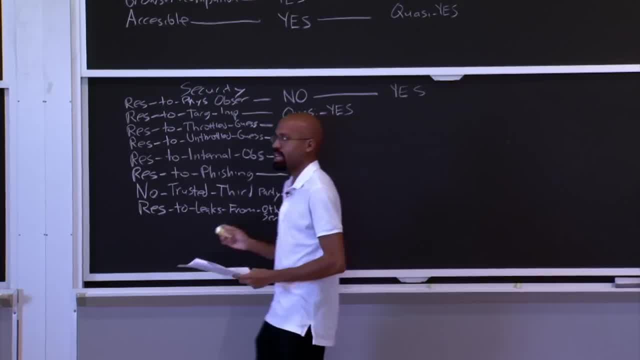 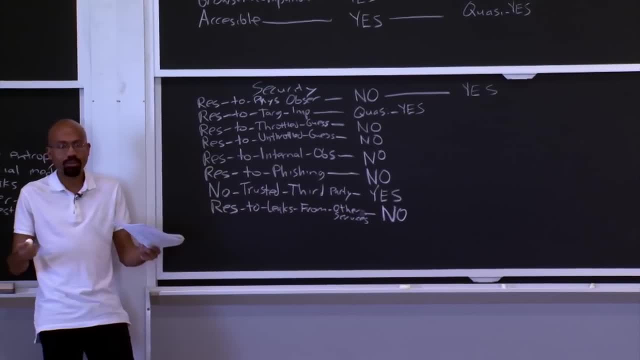 So here we will say yes, in the sense that if someone observes you're using an iris scan, for example, or someone observes you using a fingerprint reader, presumably that does not then give them the ability to impersonate you. Maybe voice recognition is a little bit different. 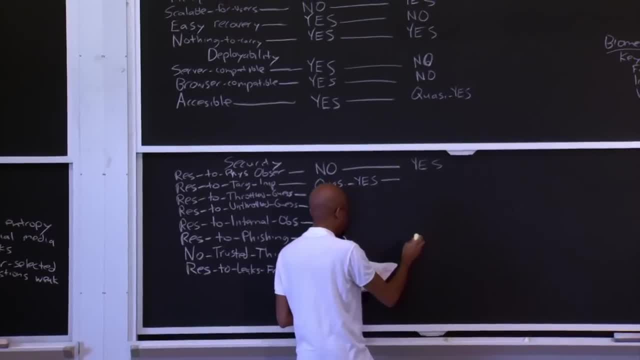 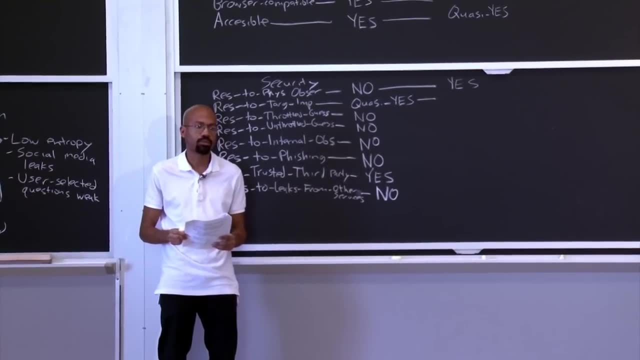 But we'll just say that we'll be charitable and we'll say yes here. But isn't that very weird, Because they're actually weaker than that. You don't even need to be observed while you authenticate. You can just be observed in real life. 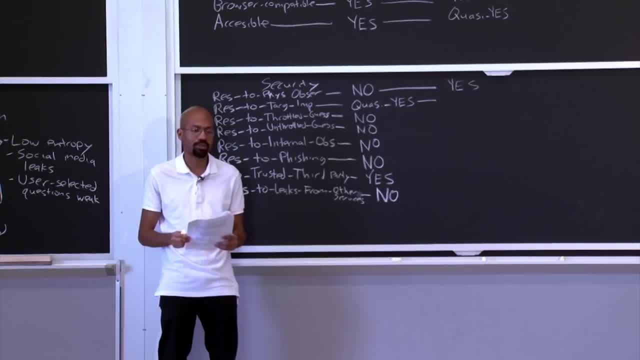 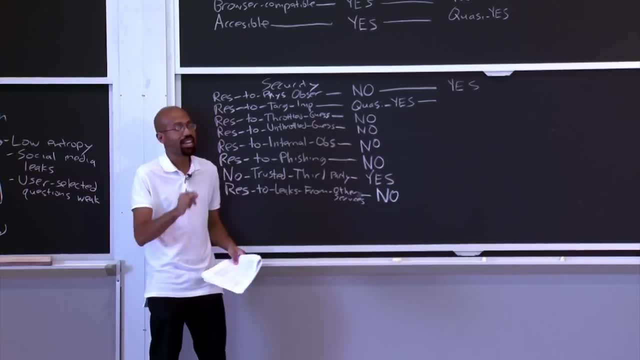 Like, if I take a very good high resolution picture of your iris or I look at your milk glass, I can get your fingerprint. That's right. That's right. Never leave a milk glass around this guy. Yeah, so that's actually a very valid point. 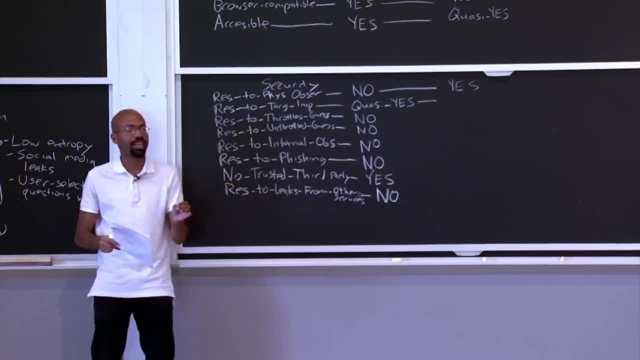 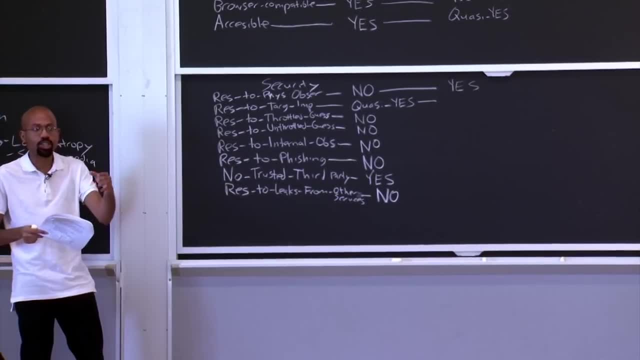 And so with a lot of these ratings. this is why I think the authors go to such pains to say: look, we don't want to assign weights to these things. And they say: we have this methodology whereby it's like if we were doing this. 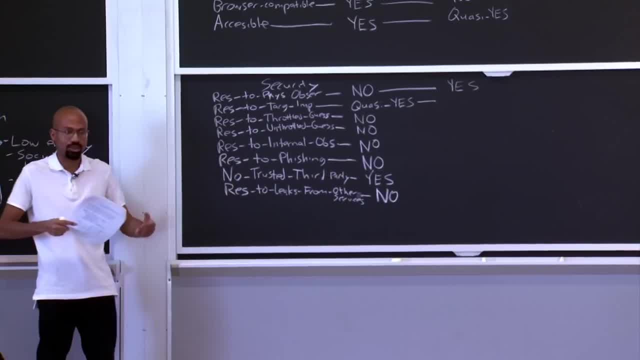 you would come up with a rating, Then I would sort of cross-validate it: Does it make sense with me, And so on and so forth. But you're right that there's a lot of wiggle room and stuff like this, And this is one reason why I think. 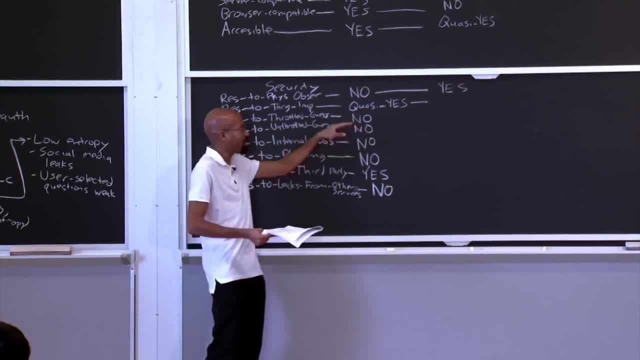 some of these quasi-ratings are even more funny than they should normally be Because intrinsically we're sitting around, we're sort of debating what does it mean to physically observe someone, for example? So yeah, you've got to take all this stuff. 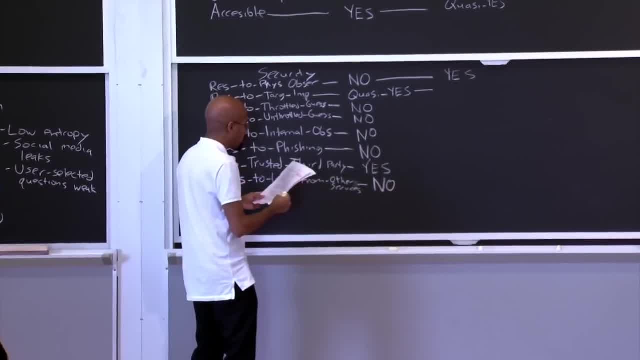 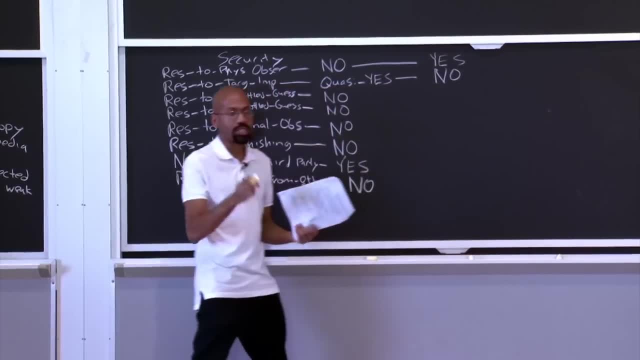 with a grain of salt. All right, so resistant to targeted impersonation. So here they say no, And this is actually for the reasons that you were just discussing. So they say that if I want to particularly impersonate you, I will go find your milk glass. I. 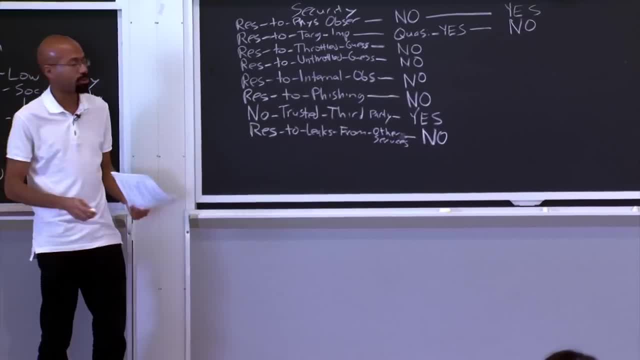 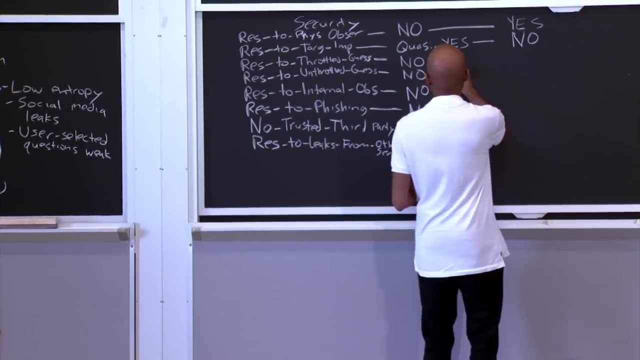 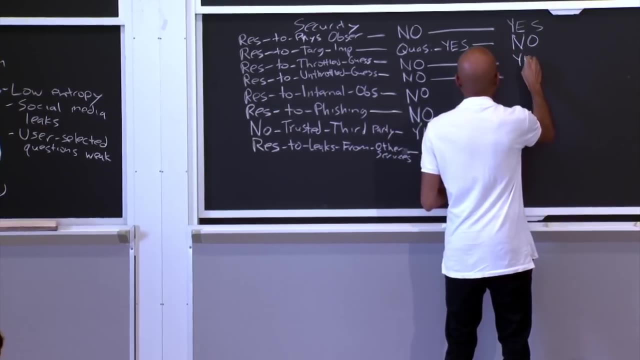 will take off your fingerprints with tape and then take it back to the crime lab and then do whatever criminals do. So they say no here for targeted impersonation. Now, with respect to the guessing metrics, so this is about interesting. So they say that biometrics are resilient to throttle guessing. 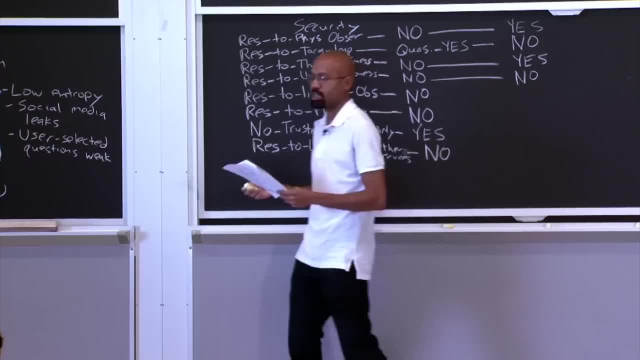 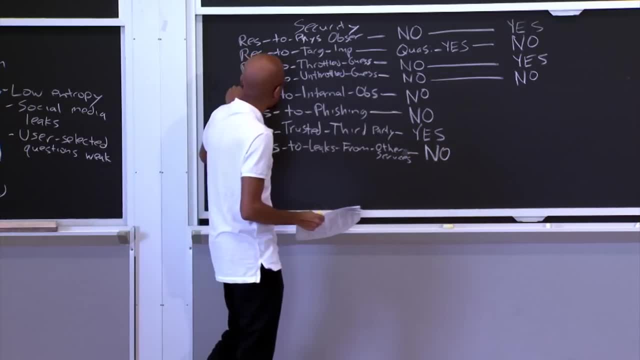 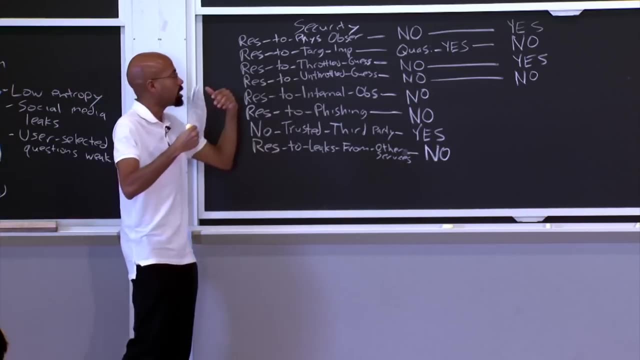 but they are not resistant to unthrottle guessing. The reason they say this is because let's look at this one first. So if the attacker, basically, is not thwarted by these anti-hammering defenses and can just sort of issue guesses, 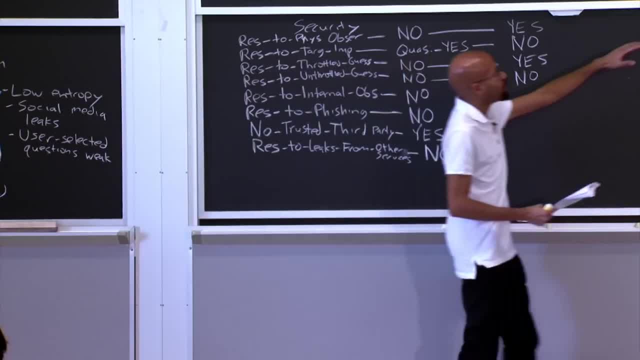 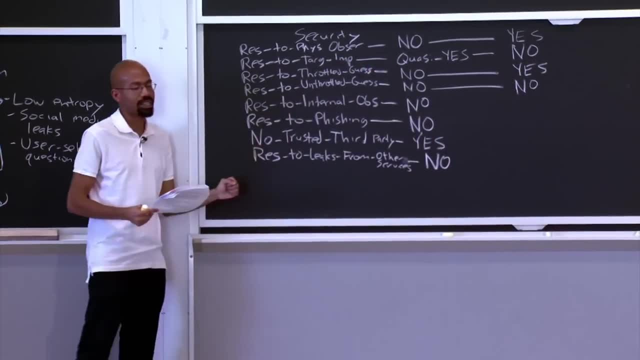 as quickly as he or she wants, then remember that the entropy space for these biometrics is actually not that large. So if you have someone who can do unthrottled guessing, we say no. biometrics are actually fairly weak. However, the authors say that they. 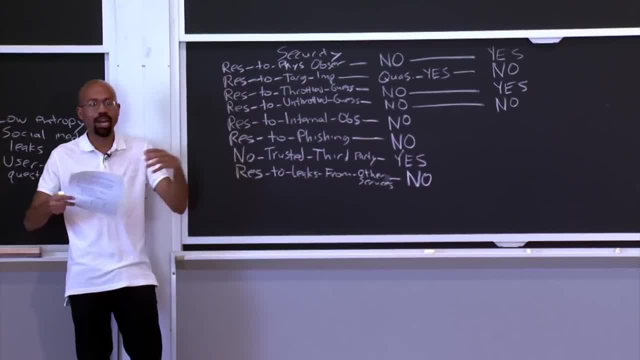 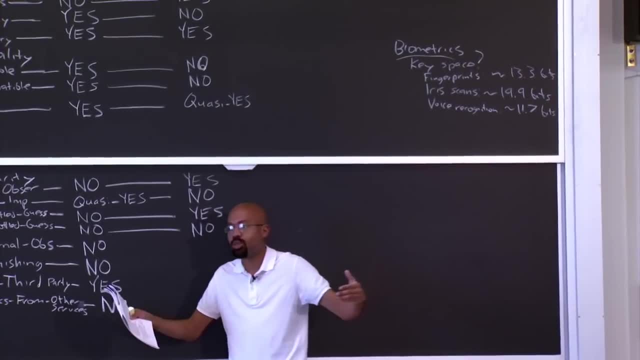 are resistant to throttle guessing, And the reason for that is because biometrics, even though they have sort of an intrinsically small entropy space, they're actually more randomly distributed within that entropy space, if that makes sense, And that's different than passwords. 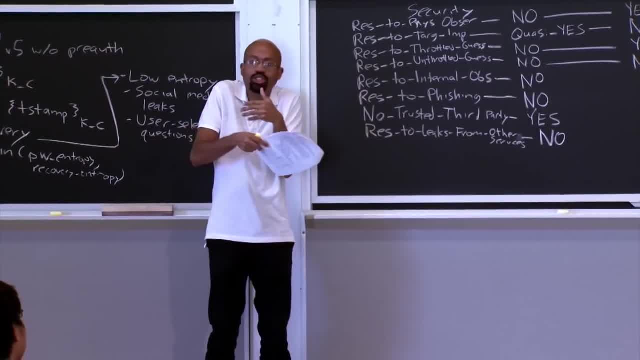 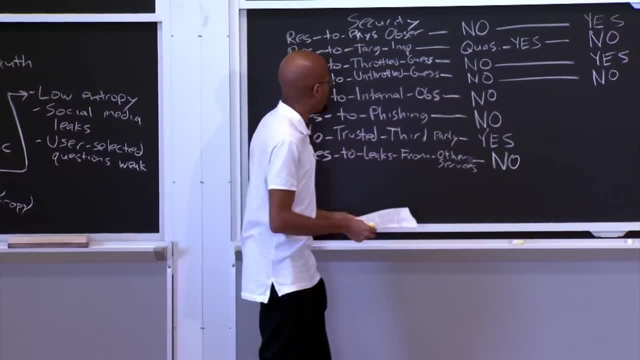 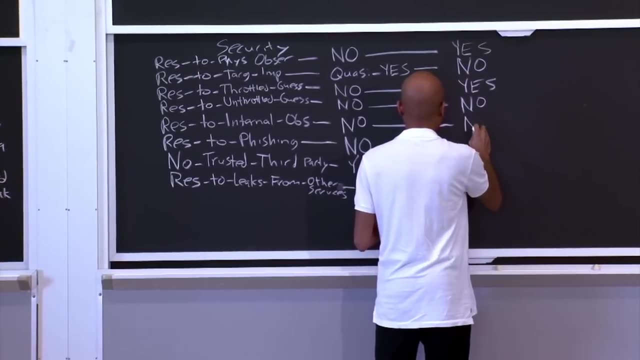 because passwords both have a small entropy space, but they're also clustered within some region of the entropy space, which makes things even worse. So does that all make sense? Yeah, OK, And then resilient to internal observation? here they say no. 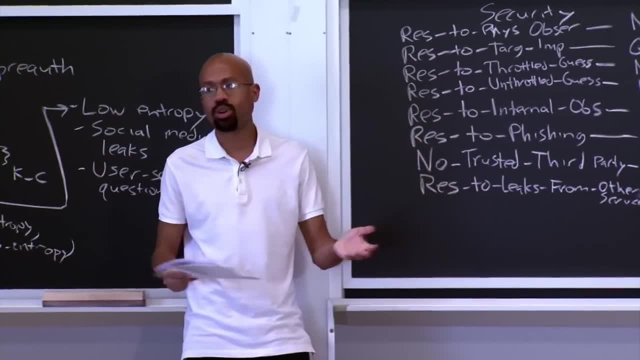 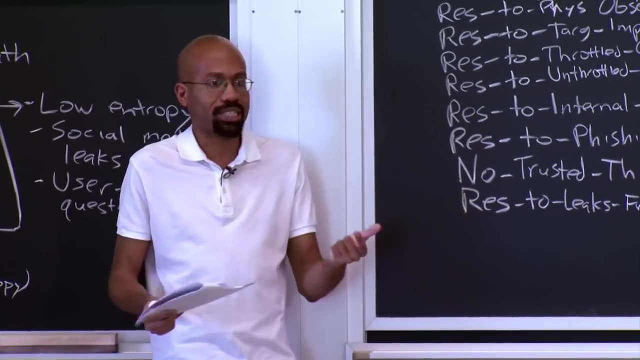 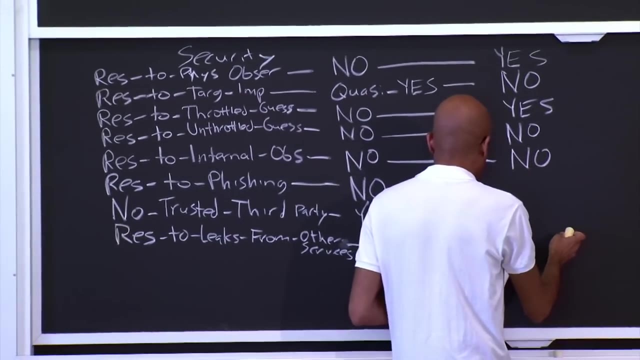 And that's because if someone manages, for example, to corrupt your fingerprint reader or whatever, and somehow gets access to your fingerprint, your fingerprint token, that is essentially a static secret which can be sort of replayed arbitrarily. Resistance to phishing: here they say no. 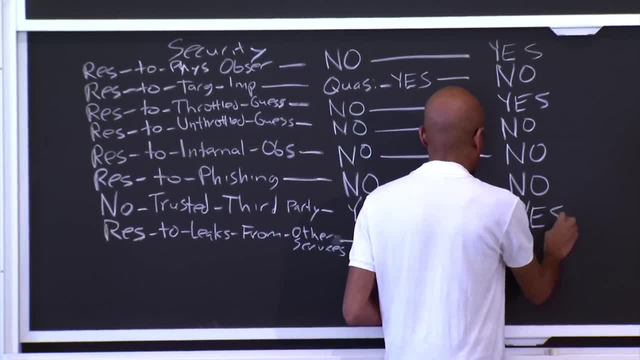 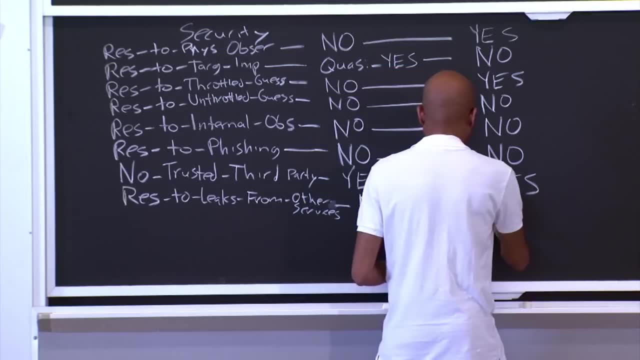 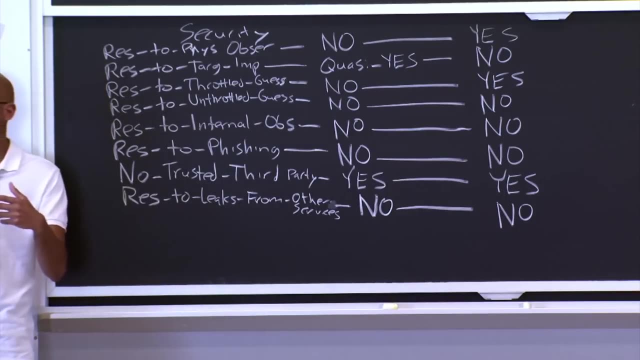 No trusted third party. so that's a yes. And then this one's actually interesting. So the resilience to leaks from other servers? here they say no, And this is very similar to why I think my passwords are not resilient to this, Because once again, your biometrics are a static token. 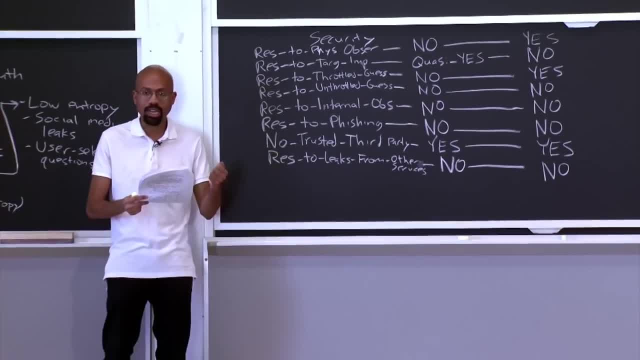 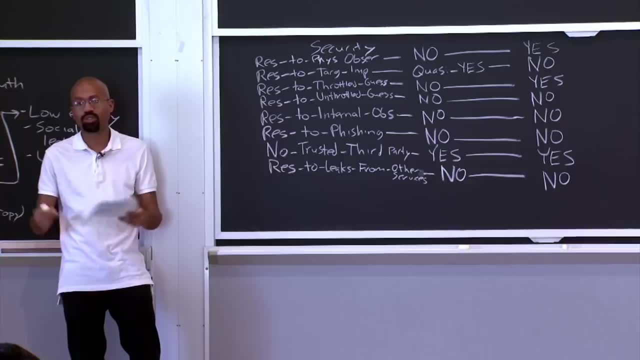 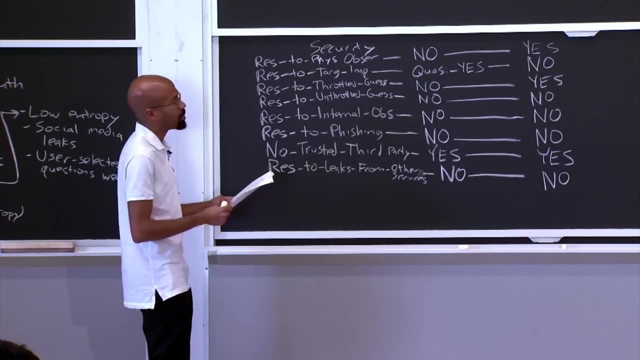 So if I use my iris scan to authenticate to amazoncom and then amazoncom leaks that iris scan data, then someone can now impersonate me at Facebook or something like that- some other service that uses that data. All right, so what does this mean? 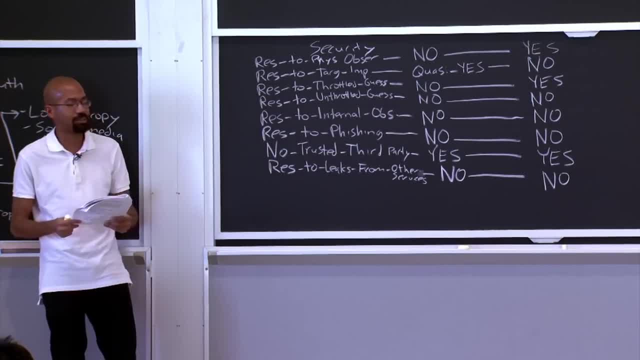 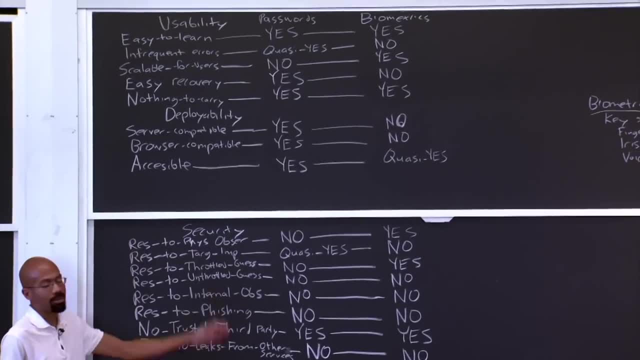 We have these two columns filled with nos and yeses and quasi yeses and stuff like that. So one way you could interpret this- this is just one way- is we could say: all right, what if we were to sum up all of these values here? 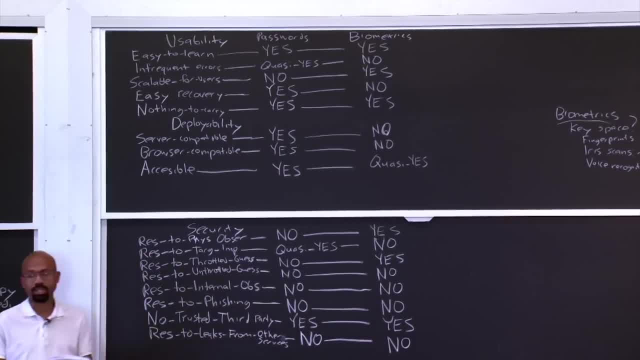 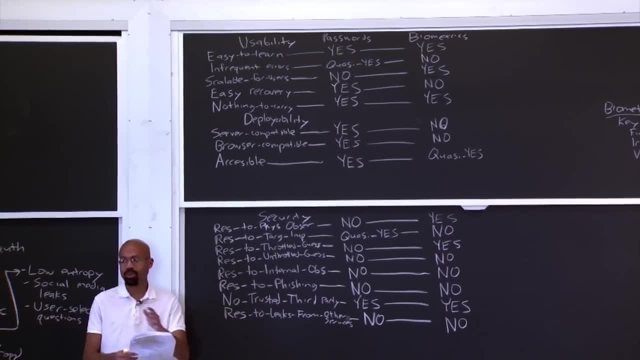 So let's say for each: yes, we actually gave a scheme. let's say one point. Let's say for each: no, we gave it zero points. And then let's say for each quasi yes, we give it 0.5 points. 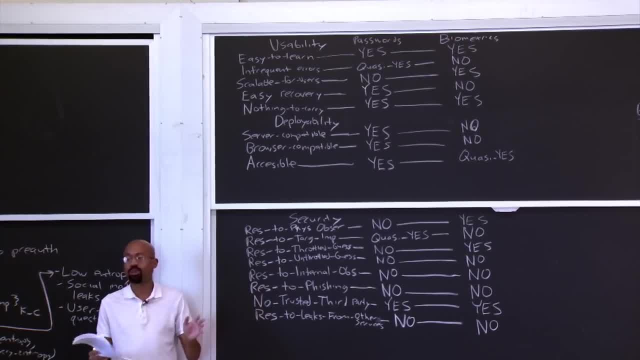 Just to be clear, this is not totally arbitrary, it is almost totally arbitrary. But this is sort of part of the interesting exercise of trying to understand what this paper is trying to tell us. So let's say that we have that scheme. Yes, equals 1.. 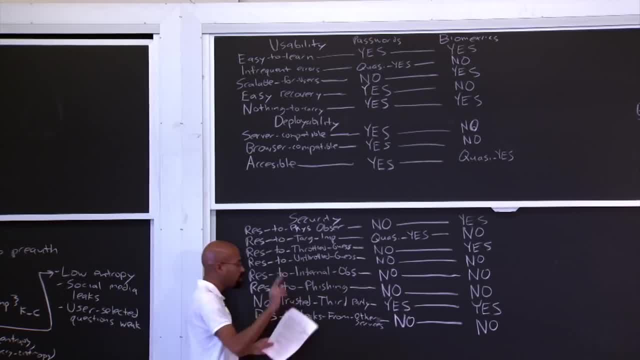 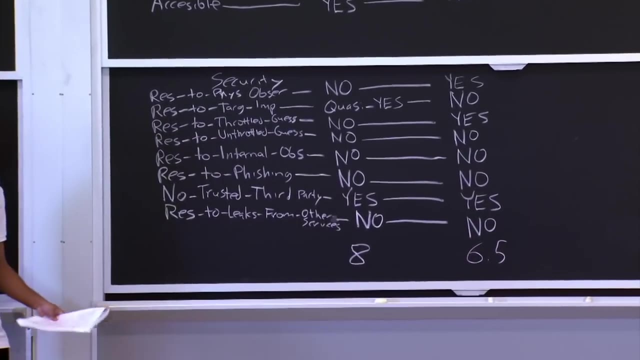 No equals 0. And then quasi yes is 0.5.. So what do the scores end up looking like? So we end up seeing that passwords get an 8. And we see that biometrics get a 6.5.. OK, so we now have two numbers. 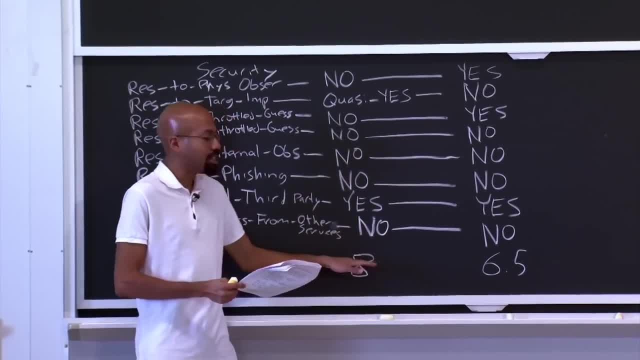 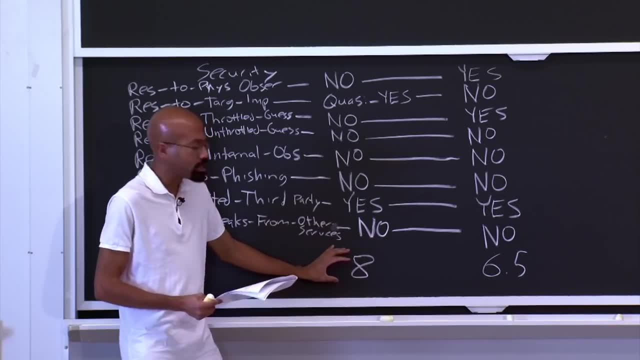 So what does this mean? Well, I think these numbers are very interesting. I feel like I've invented a new type of number which is like a qualitative number. So what does this mean? Well, as the authors go to pains to express. 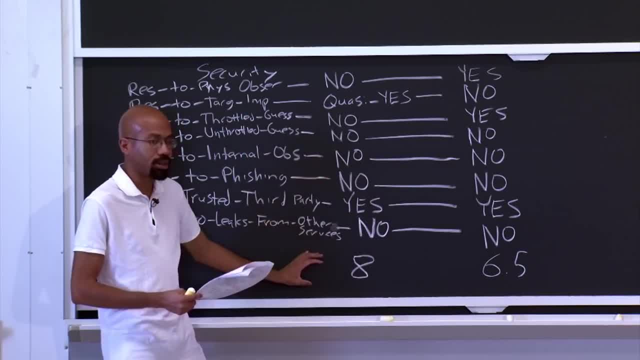 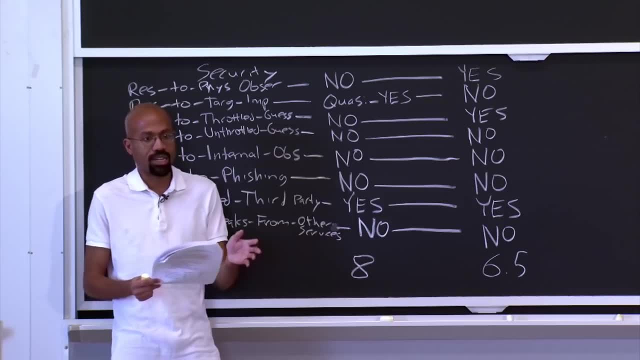 they actually don't want to assign weights, They don't actually want to do this comparison. But the reason why I think this is useful at least, is because you can at least see that it's not like biometrics blow passwords away. It's not like they're just so much better. 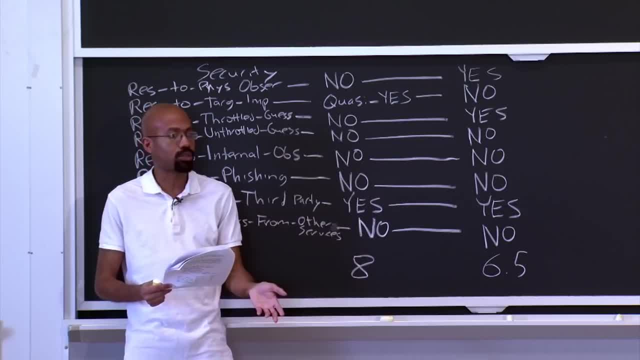 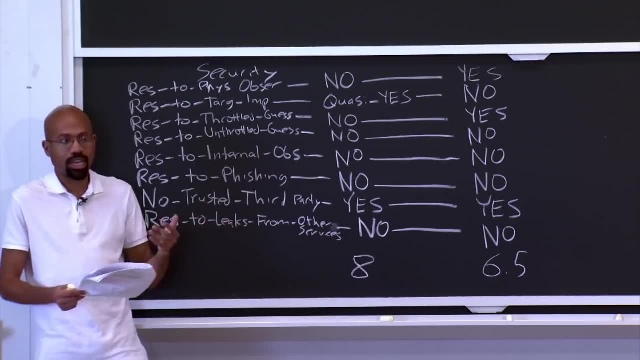 that obviously we should move towards biometrics instead of using passwords. And that's really the point of that big table the authors give in the paper. That's in fact why they don't give numbers. They just want to say: if you blur your eyes, 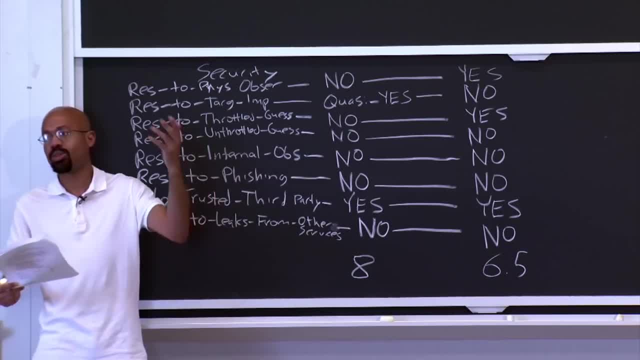 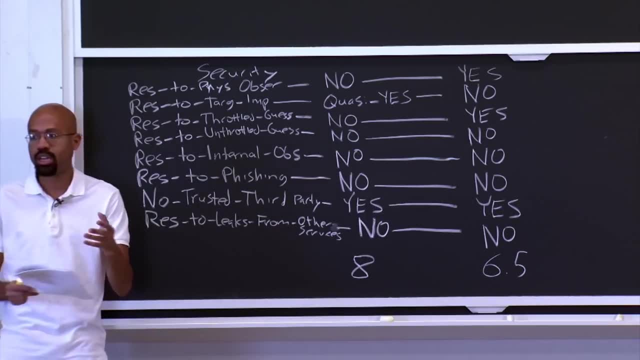 and you look at this table, you'll see that passwords are good And some things, And other things are good and better things, And then you have all these so on and so forth. So, ultimately, what it comes down to is in your particular security situation. 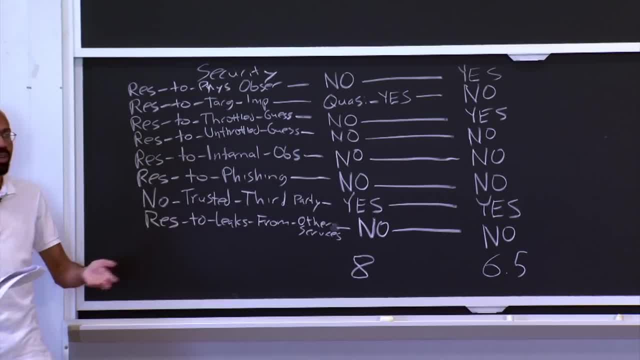 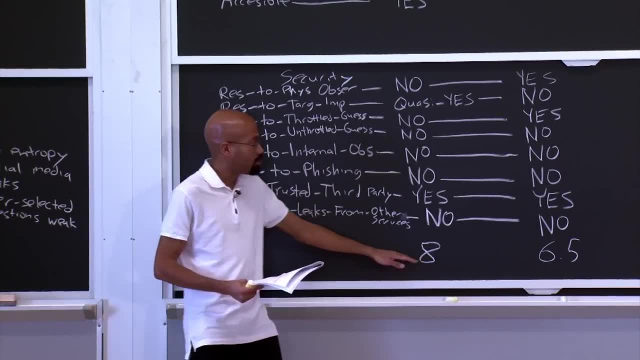 which one of these factors do you care about the most, And which ones are you willing to sort of sacrifice? So, once again, this score. you shouldn't take this too literally, But this is just saying: well, both of these things have strengths. 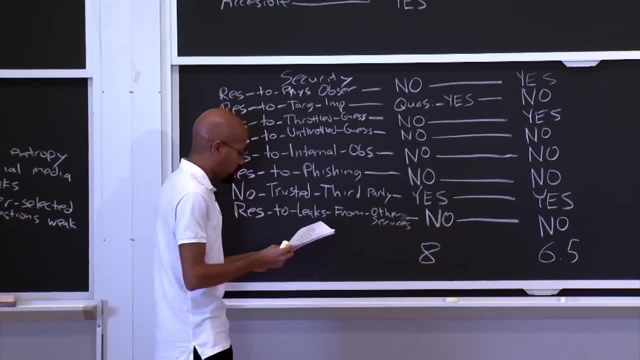 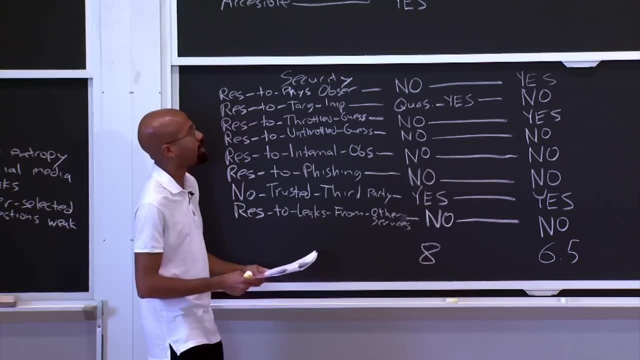 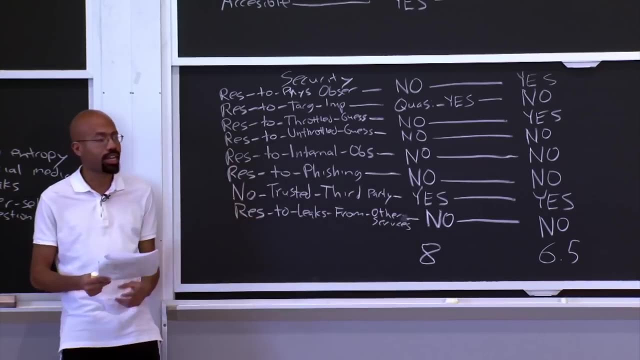 Both of these things have weaknesses, All right. so basically, we went to this table, We did this exercise And we figured out that it's very difficult to say that one authentication scheme is totally dominant over another authentication scheme. So you might think, all right, well, maybe we. 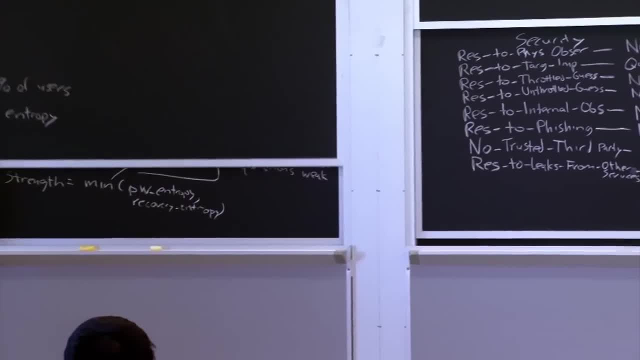 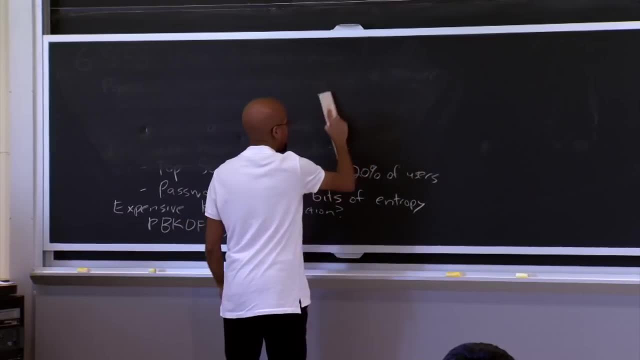 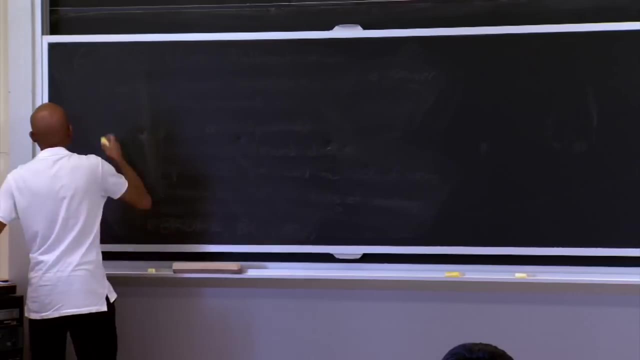 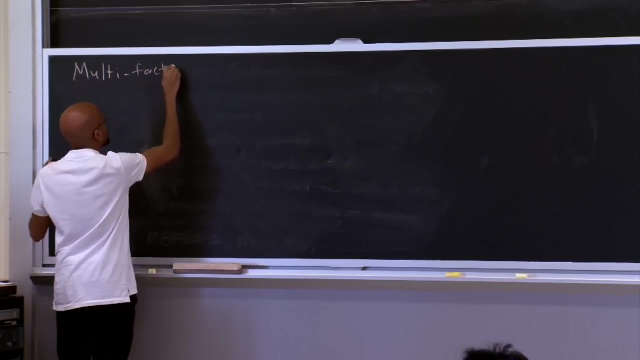 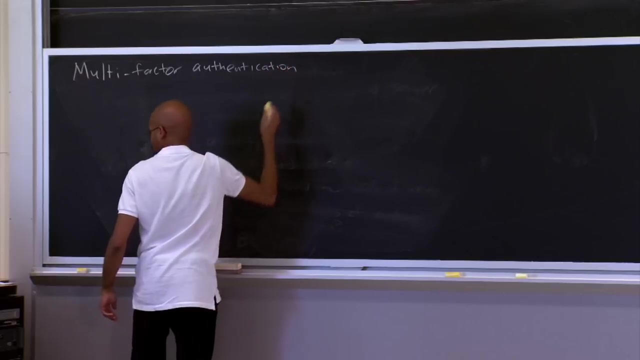 can sort of have the best of these sort of ambiguous worlds by somehow combining multiple authentication schemes, And that is what is done in systems that use multi-factor authentication, And so the idea here is that you want to use defense in depth. So the basic idea is that you want 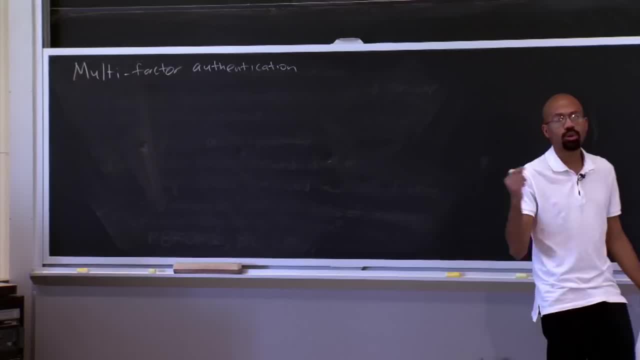 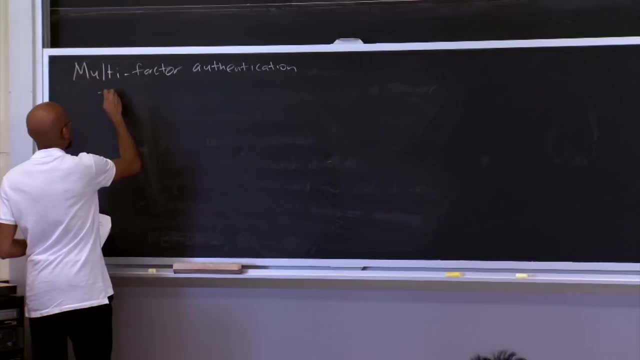 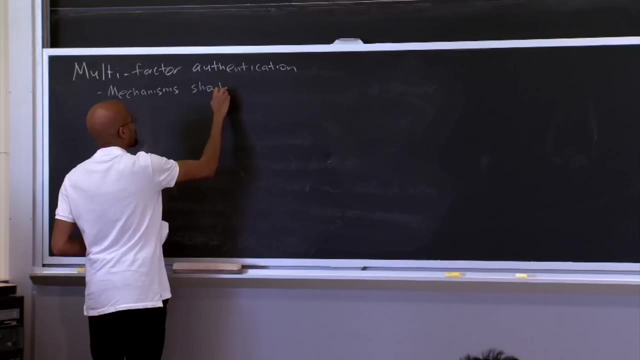 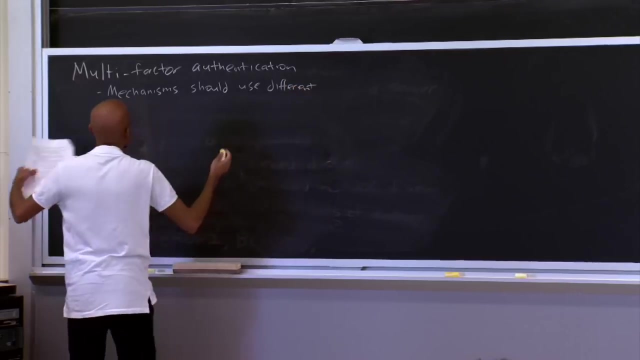 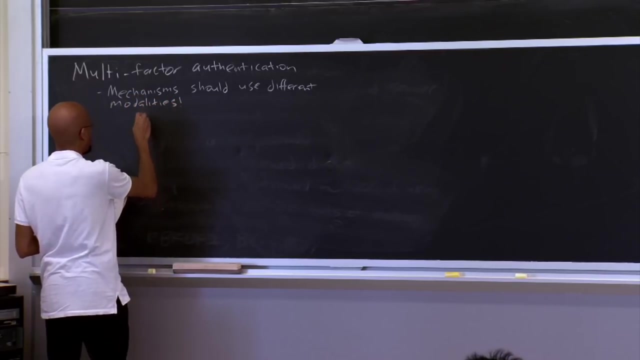 to require users to authenticate themselves with two or more different authentication mechanisms, And the key is that each one of these mechanisms should use different modalities, And by different modalities I mean they should leverage different sort of ways of authenticating. So, for example, one of those mechanisms. 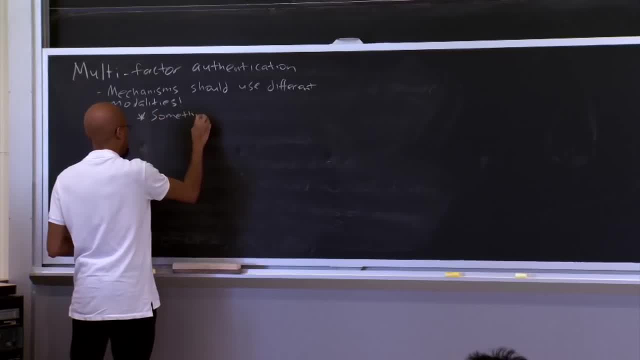 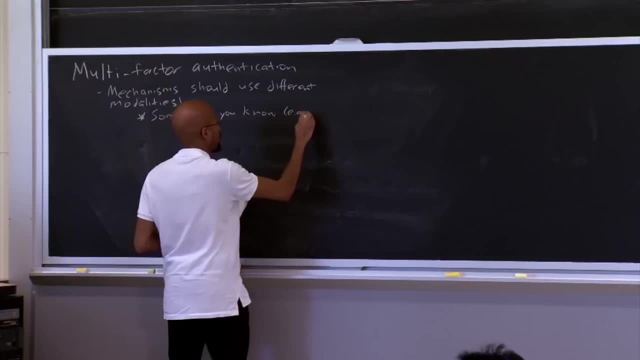 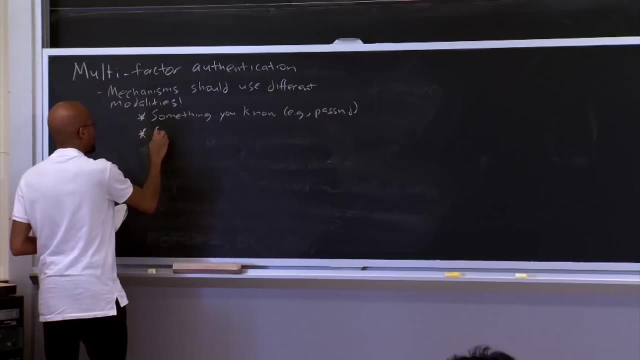 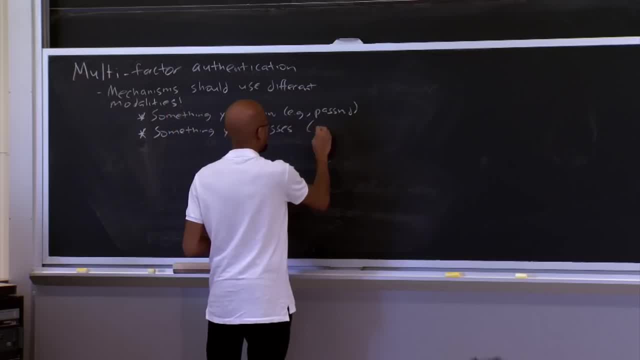 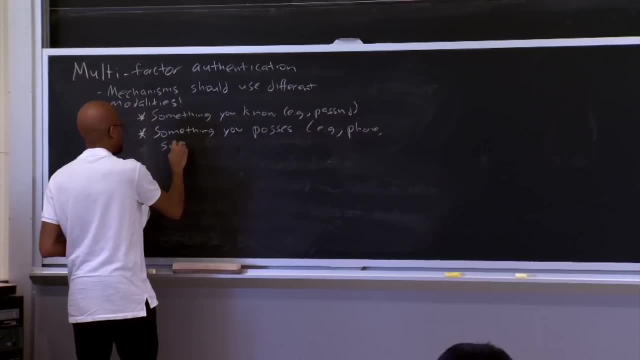 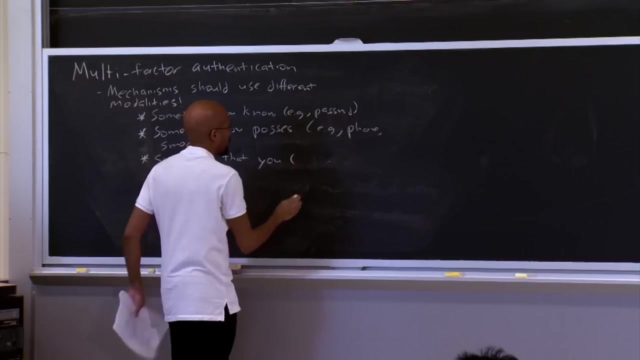 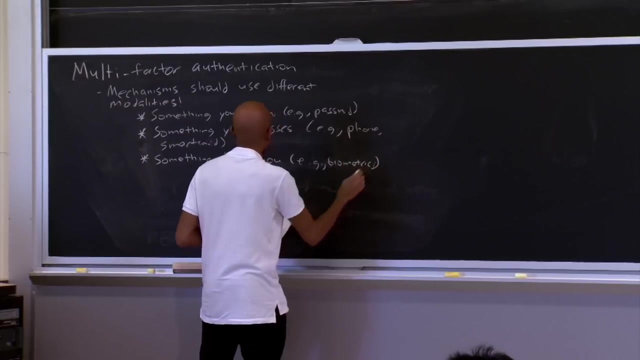 And so an example of this might be a cell phone, maybe a smart card, something like this, And then maybe another modality will leverage something that you are, And so this is, for example, what's done by biometrics, And so the idea behind this multi-factor authentication. 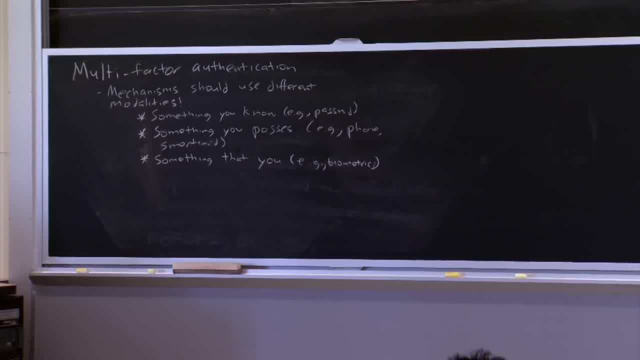 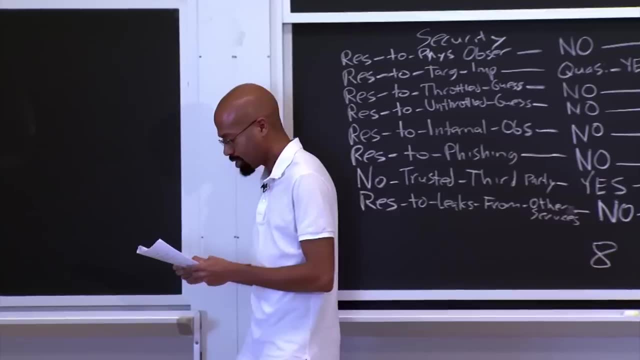 is that when you use schemes like this, an attacker has to sort of steal or subvert multiple things to be able to successfully impersonate you. So, for example, the attacker might be able to guess your password, but maybe the attacker can't steal your cell phone, for instance. 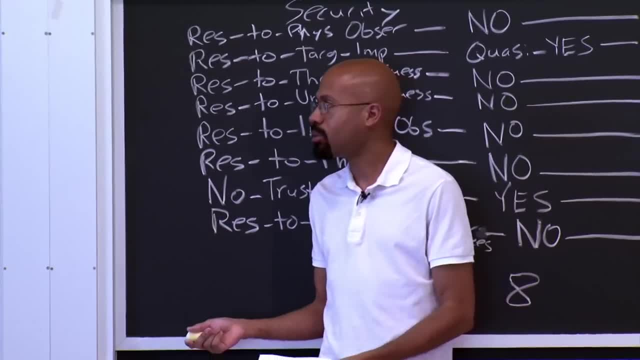 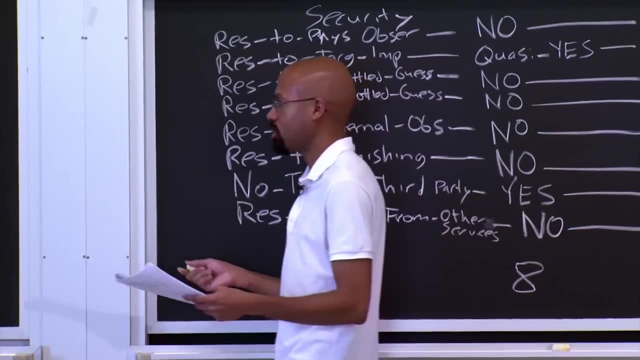 And so there's a couple different examples of this. Maybe the most common one is Google's two-factor authentication for things like Gmail, for example. So you have a password, but then when Google detects that you're using, let's say, Gmail from a machine it doesn't know about. 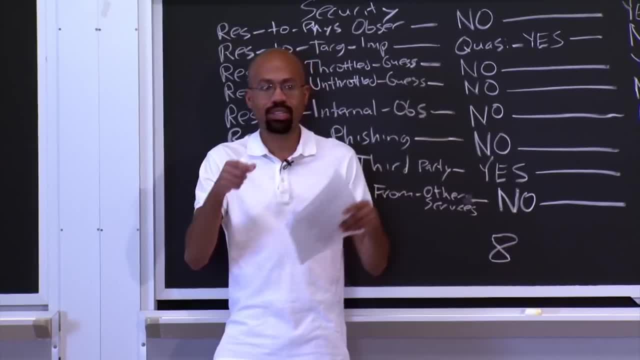 it's going to send you a text message and have some little code in there, And then you have to type in that code as well and Google says, OK. well, presumably you weren't so clueless that you got your password stolen. 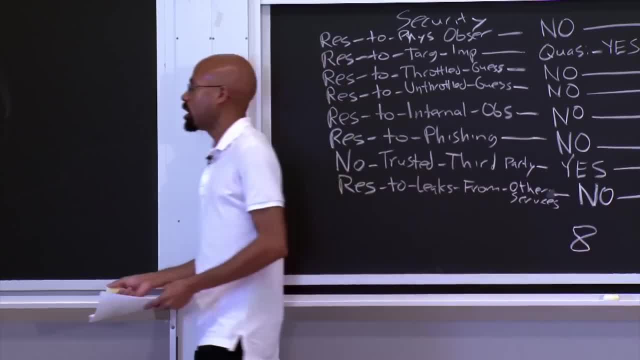 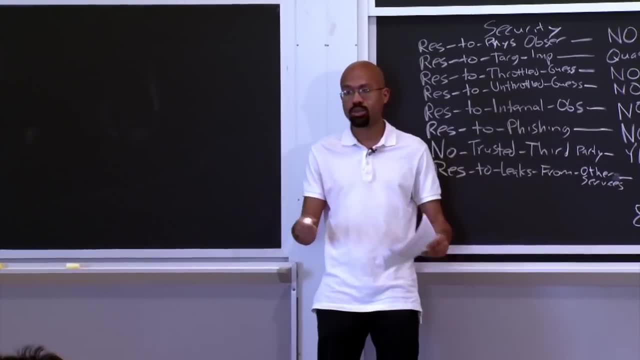 and someone stole your cell phone. If that happened to you, you deserve to get hacked. Google's a good example of this. AWS actually has this, too- Amazon Web Services- So you can actually use two-factor authentication to control your VMs or things like that. 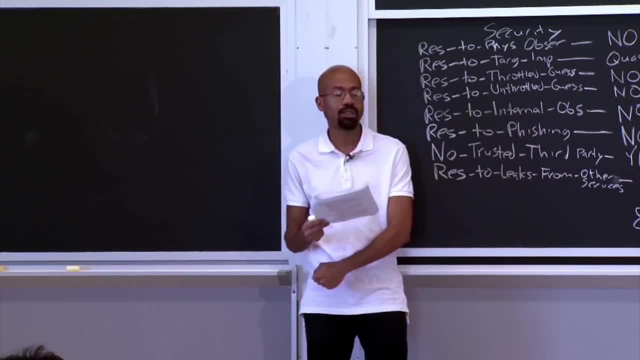 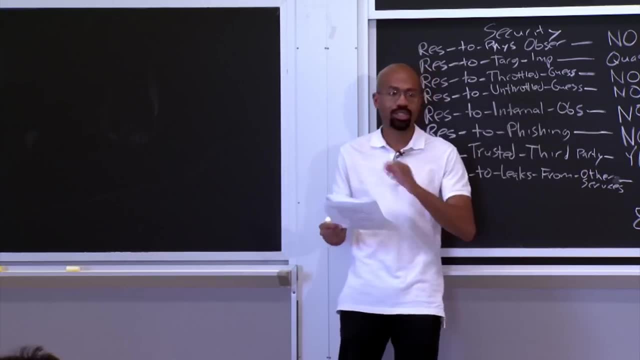 And they have an option to use a smartphone app for the second thing. in addition to the password, They also allow you to use a custom security dongle. that's dedicated hardware that just allows you to sort of do this two-factor authentication. So this all seems very nice. 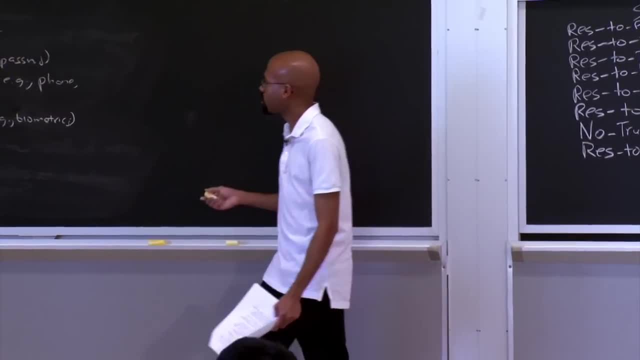 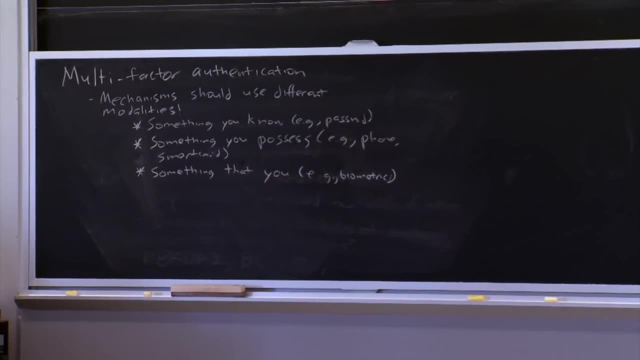 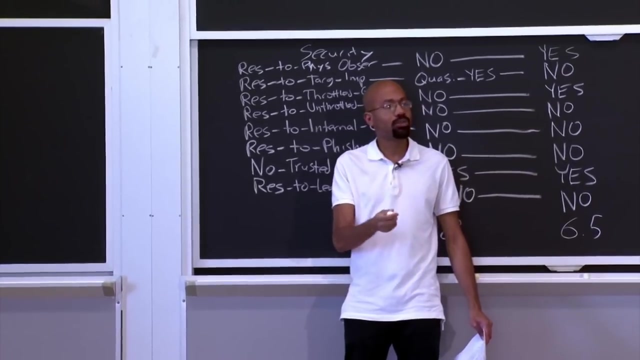 One sort of sad thing, though, is that I didn't put an S on it. How do you spell possess? This is embarrassing, Let's just move on from there. So one thing that is a little bit sad about this stuff is that there are actually empirical studies that show that if you give users 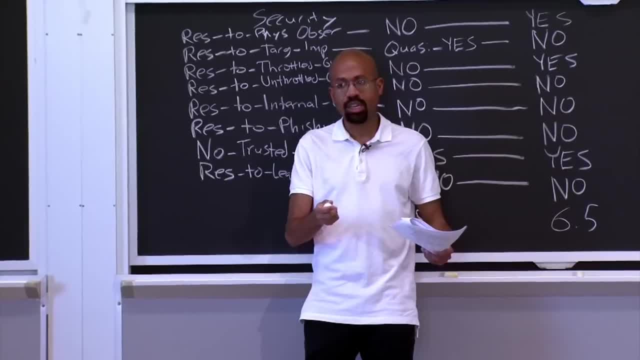 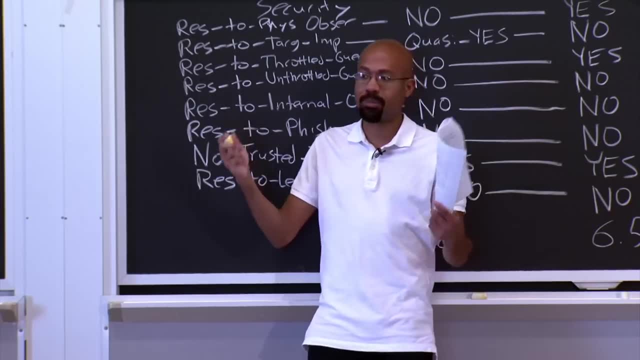 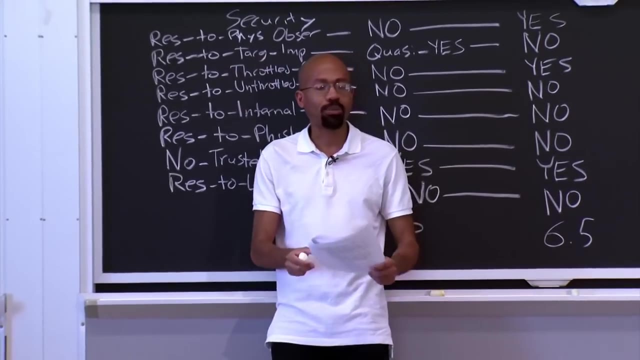 a second means of authentication besides passwords, then they will typically pick weaker passwords, Because they then get more confidence that they now have these two things. So why not just make my password, Mr Rogers, and then just be done with it? So there's interesting sort of models that security researchers have about how people 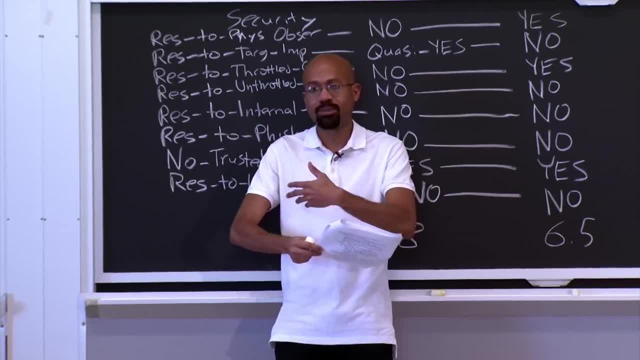 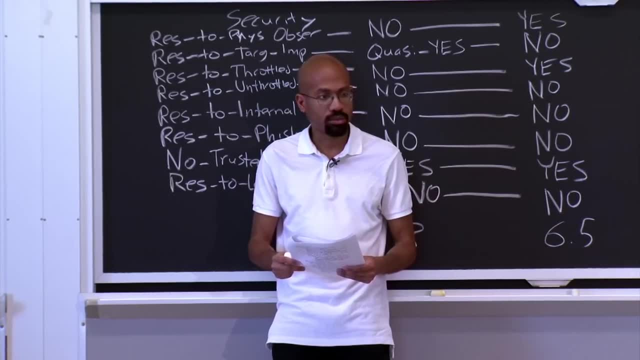 sort of evaluate risk. So it's interesting. So the more protections you give them, sometimes the weaker they will use other protections. I always felt like that was the ATM idea that you have a credit card and they're like: so that means you're pinned. 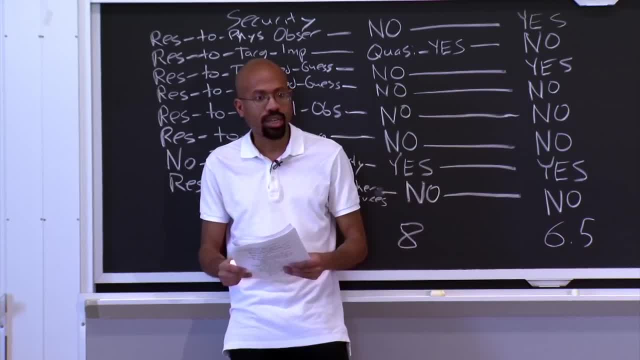 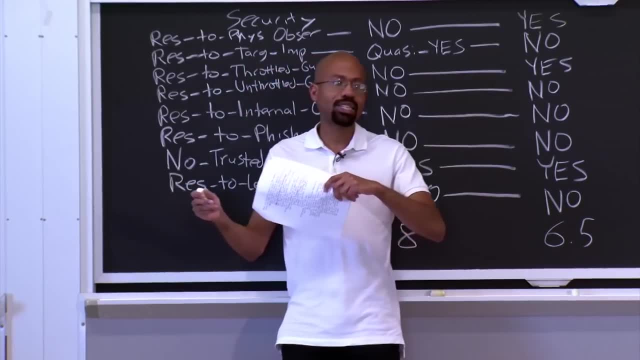 It can be four numbers, which is totally not guessable by anyone, right? Yeah, I mean credit cards are very interesting Because, yeah, They allow you to have these four digit pins, But then, behind the scenes, they have these enormous fraud prevention. 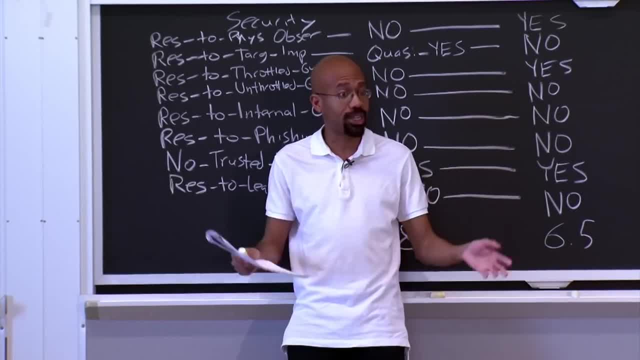 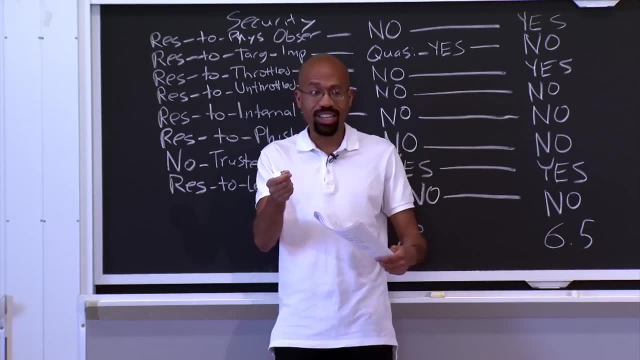 sort of setups that are actually extremely interesting, like the machine learning they do and stuff like that. I mean, I don't know if you've ever been in the situation where you go overseas, for example, and you try to use your card. 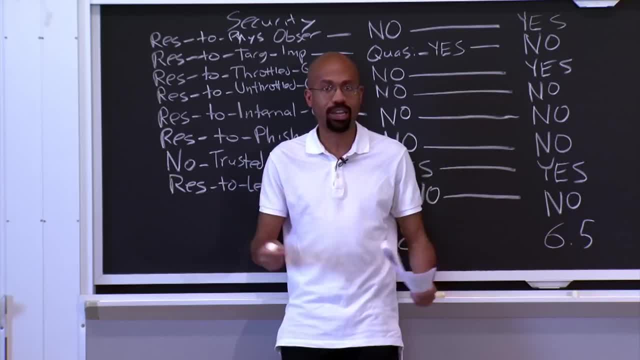 Like sometimes, at first I thought I was getting like, I thought it was like Liam Nielsen. on the other end, Like someone will call me, it's like: are you using your ATM card? I'm like: yes, yes, I am using my ATM card. 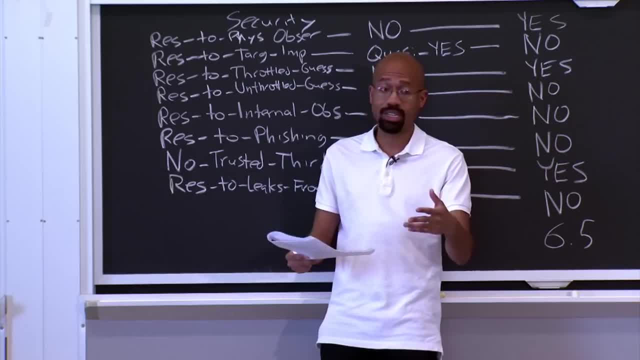 What's going on And it's like the bank right, And so that's a very easy thing for them to detect. Yeah Right, You're actually using your ATM card internationally. But sometimes, like I've actually had that happen to me- 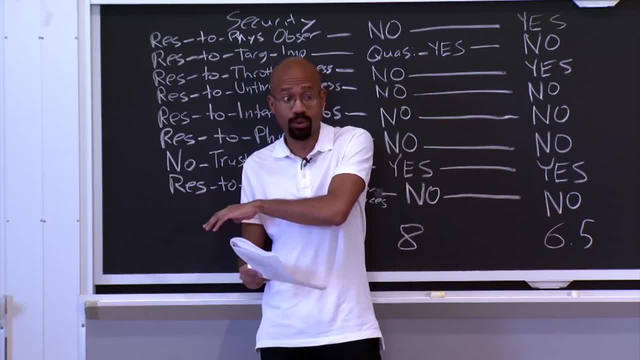 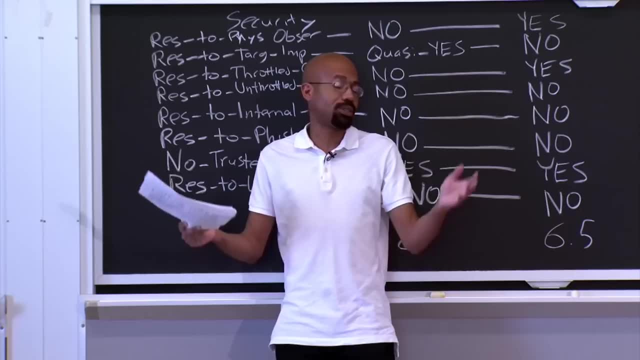 where I went to a website like an e-commerce site that I hadn't been to before And, for whatever reason, they thought it was outside my profile Right, So maybe whatever. I usually buy science fiction books And then all of a sudden I buy a My Little Pony book. 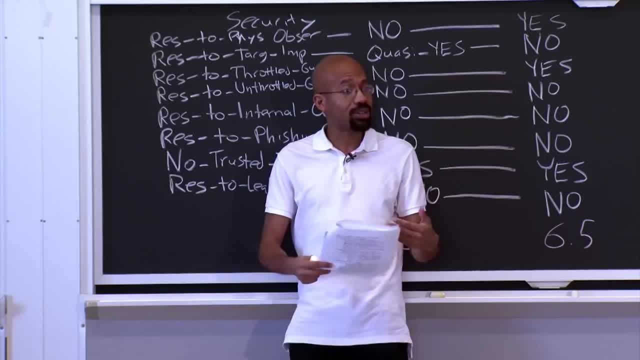 And then they know they'll call me or they send me an email And they're like: if you don't get back to us in 30 minutes, we're going to put a lock on your card. And so I think the reason that credit card companies do that is because they really feel this tension between wanting people to use credit cards, because that's how they make money, versus not wanting criminals to use the credit cards. That's how they lose money. So they have decided to err on the side of putting a lot of security on the back end infrastructure. 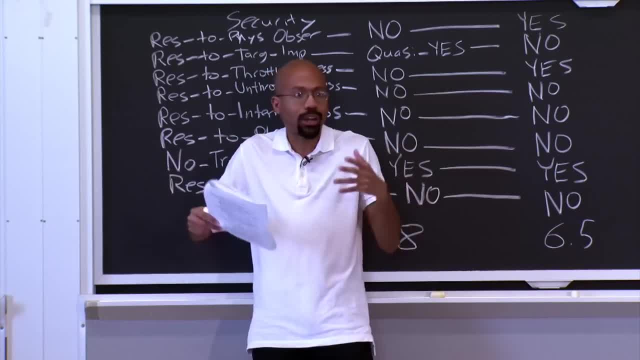 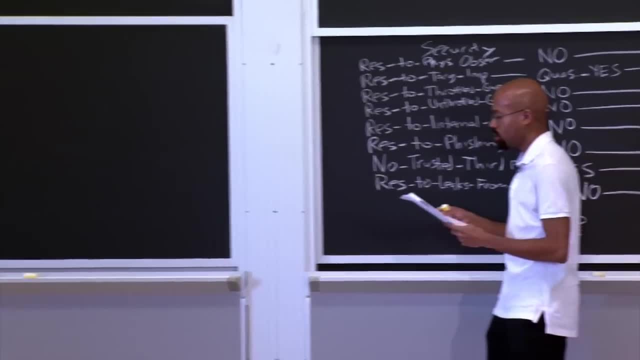 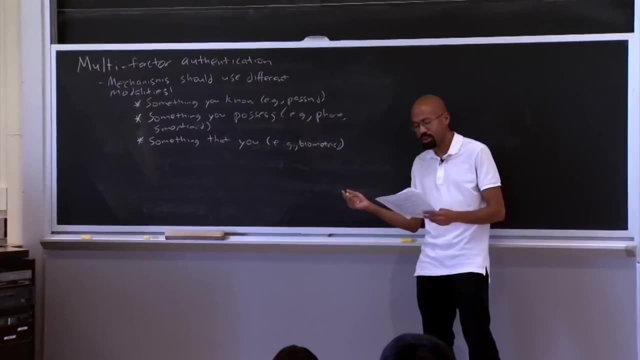 doing the machine learning and stuff like that to analyze fraud-like patterns? Any other questions? OK, So, yeah, So in the homework. the homework question basically asks you to think about what are some of the potential factors you might want to consider when you're thinking about authentication schemes. 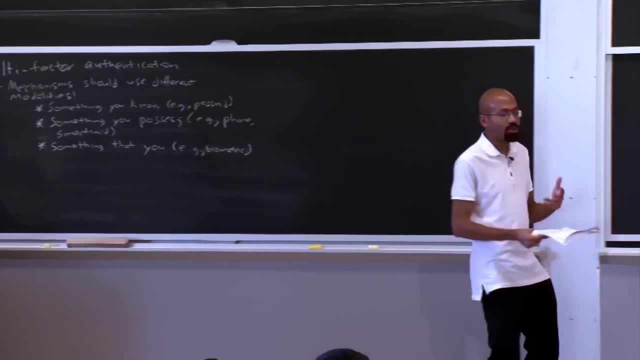 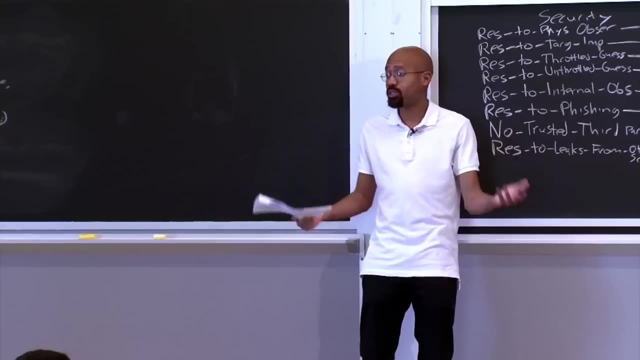 in a bunch of different scenarios, And I mean at a high level. there's no sort of right or wrong answer to the homework question. It's very much like this discussion here. You sort of look at a bunch of things that you could be concerned about. 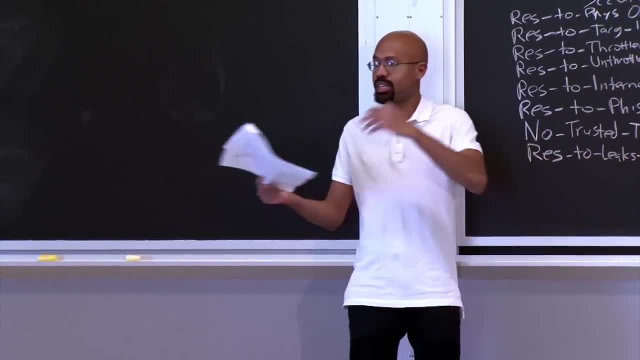 And then you decide, OK, well, in this scenario, I care more about this. In this scenario, I care more about this. So, for example, one of the questions was about logging into a public library And I said, look, Athena machine. 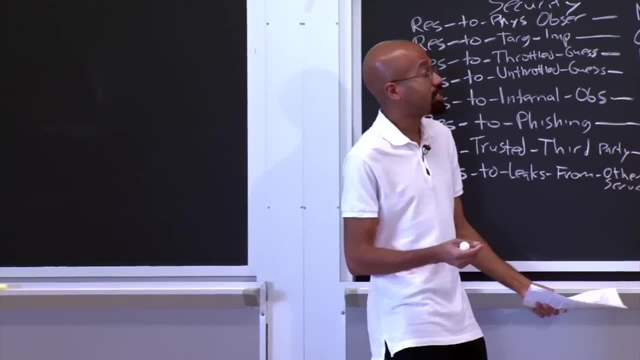 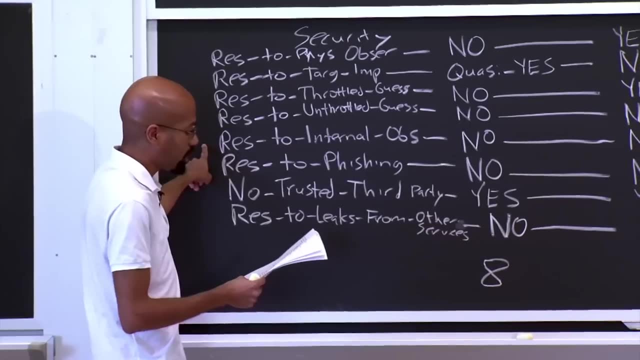 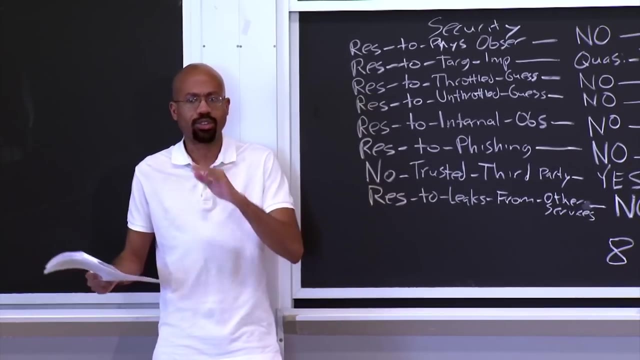 what might you want to care about there? Well, maybe one thing that you might care about, but that might be difficult to protect against, is sort of resistance to internal observation, Because maybe there's a lot of malware possibly on those machines. I mean, who knows what these undergrads are doing? 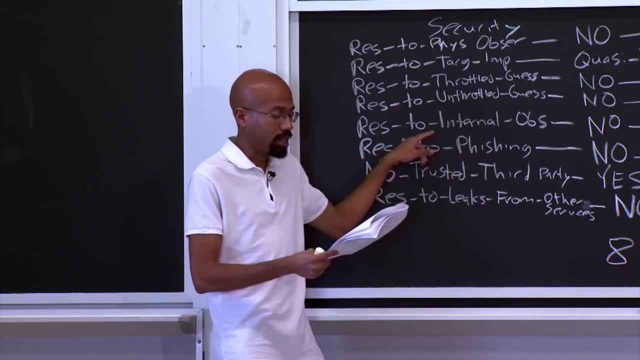 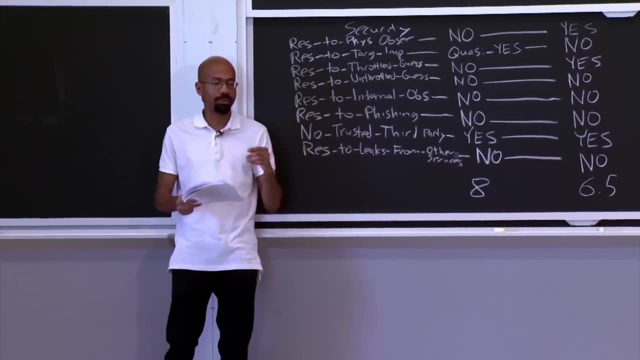 So maybe it's difficult to protect against that. Maybe you have to punt on that. Another thing you might think about is: with respect to that, maybe that means that biometrics isn't a great idea. So a lot of times, biometrics, you really 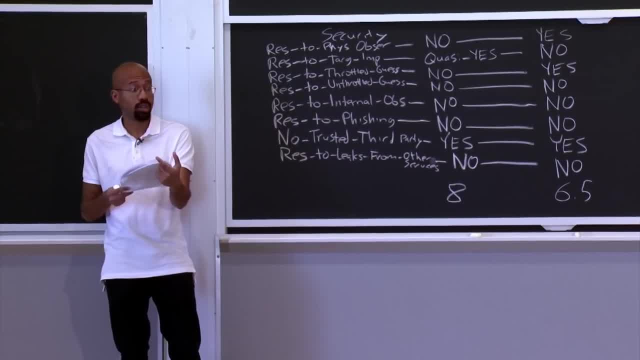 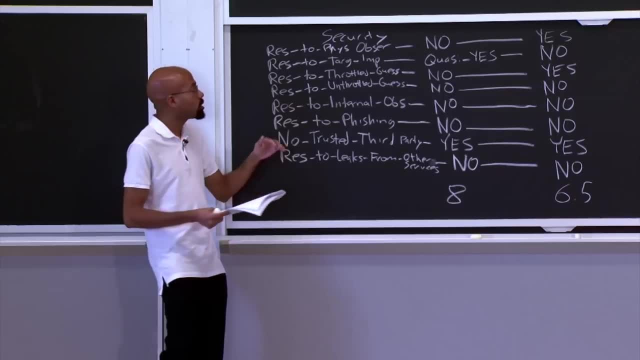 want to have that biometric reader be something that you trust Because, once again, it's very difficult to replace your iris scan. It's very difficult to replace your fingerprints. So if you think that you're in a situation where you can't guarantee this property, then maybe biometrics. 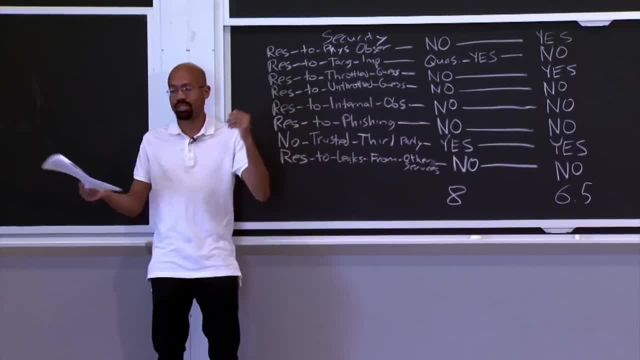 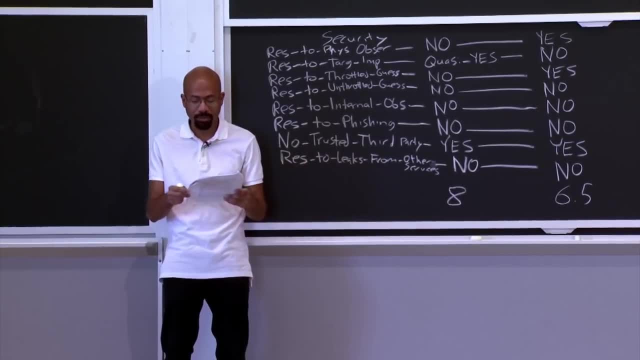 is a bad idea, Because the penalty for losing someone's fingerprint data is actually pretty bad. Now, that person will always be on the no fly list Because their fingerprints are always considered to be terrible. So you know, getting back to sort of the ATM example, 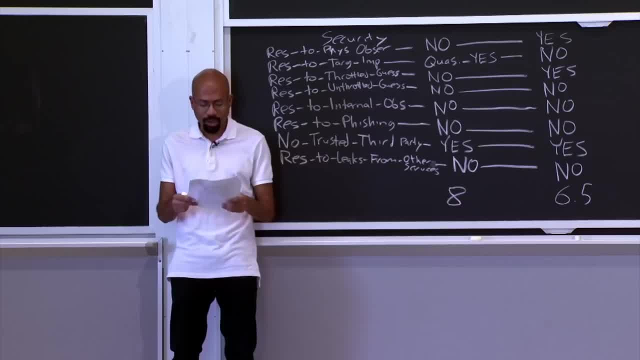 So what kinds of things might you care about there? Well, there it's a little bit of a different threat model, I think. So to the banks, you know, ATM security actually matters a lot. So, for example, one thing they want is resistance. 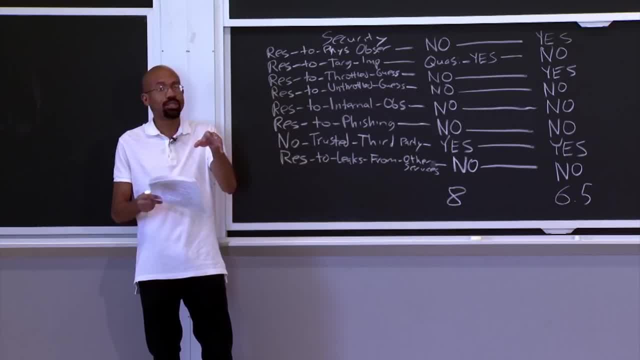 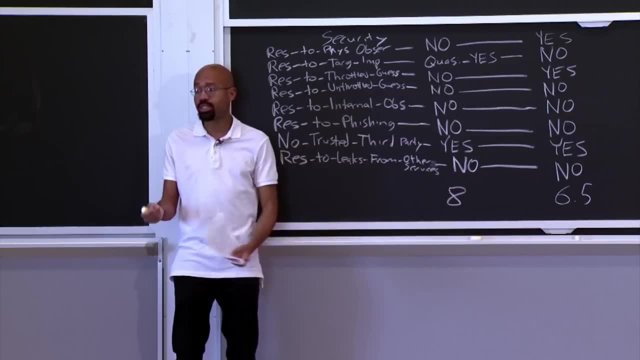 to physical observation. So this is the idea: if I see you somehow interacting with the ATM machine, I shouldn't be able to use that and then somehow impersonate you. And they also want this resiliency to theft too. The idea like if I lose my card. 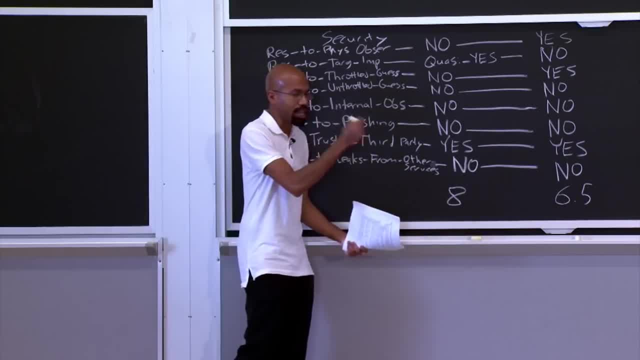 then it shouldn't be the case that someone can just take my card And then use it And then somehow impersonate you And then use it to buy things on my behalf. And that gets back to our previous discussion. The credit card companies have decided. to say: we're going to actually implement a lot of the heavyweight security stuff on our side in exchange for making it easier for you to spend money and then forget to pay your fees, and then we get more money that way. But they do definitely care about those things. 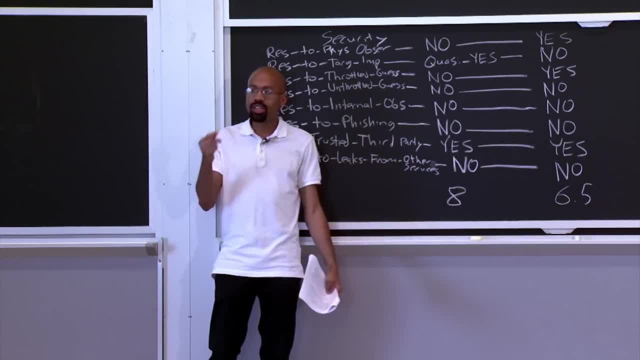 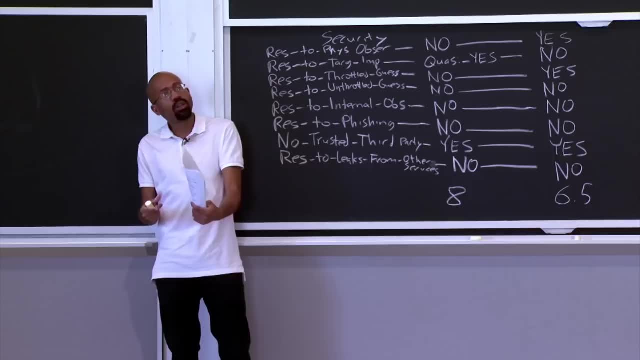 One thing you might think about once again, going back to biometrics, is: does the bank trust ATMs, Like does it actually trust those physical terminals? So on the one hand, you might think yes, because presumably the banks either built them. 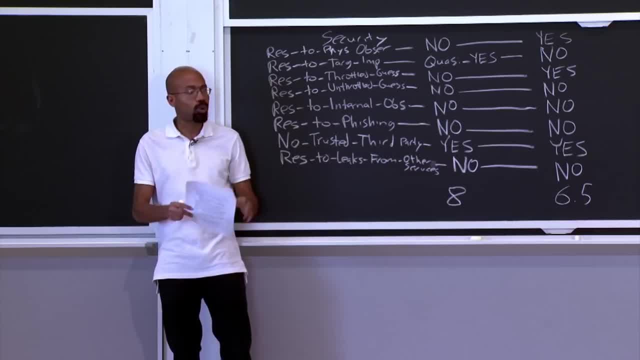 or they trust who built them, But on the other hand, once those things get out in the wild, only Zeus knows what's going on, And in fact it's a pretty popular scam in a lot of countries to have fake ATMs. 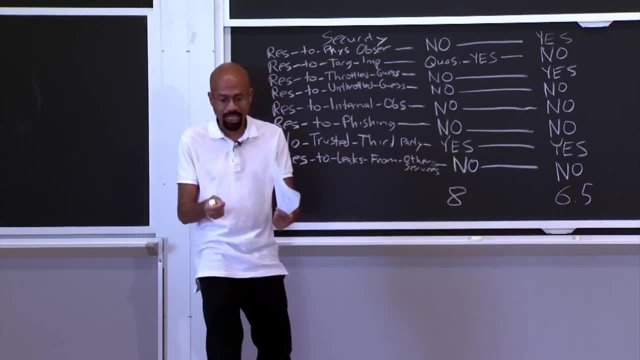 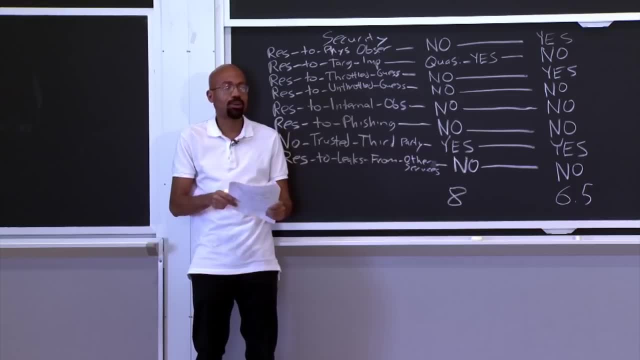 or to have shell ATMs. You go into a country, you go into the ATM, you put your card in there and either there's a relay attack or it actually doesn't ever talk to the bank back in at all. It just has a reader which steals your pen. 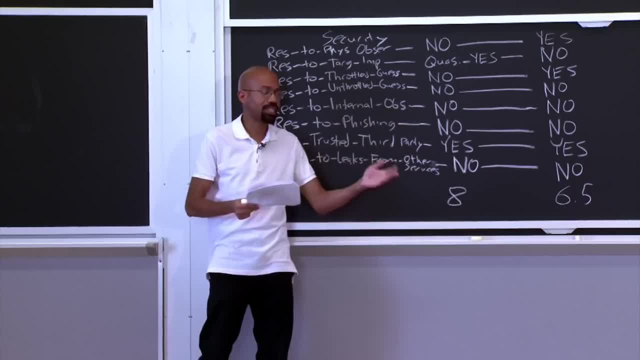 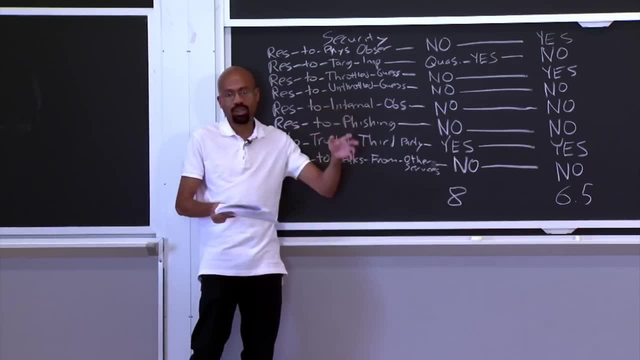 So maybe, in fact, the banks don't trust those end terminals, And if that's the case, once again, maybe biometrics are not a good idea, even though you'd think that that seems like a good idea. I can only withdraw money if my biosignature matches. 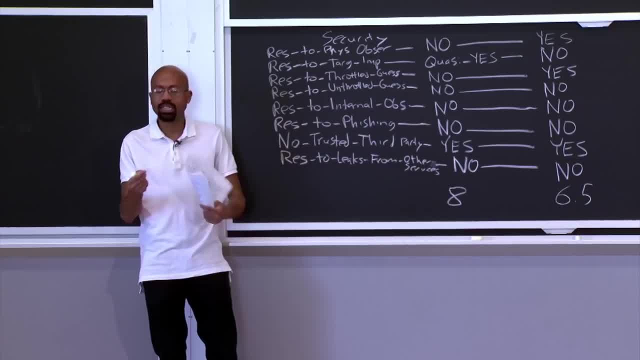 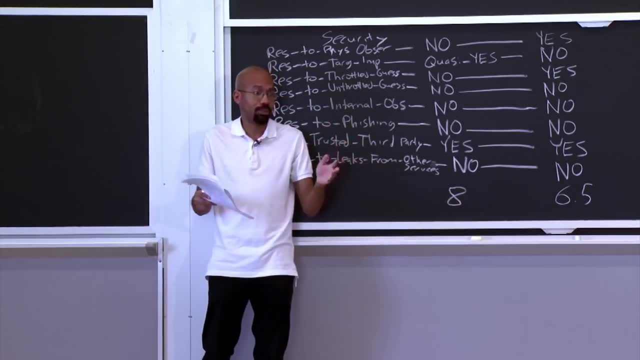 And another interesting thing to think about is maybe there should be in the ATM case two different levels of security, based on whether I want to just read the state of my account or whether I want to maybe write- And by write I mean actually spend some money. 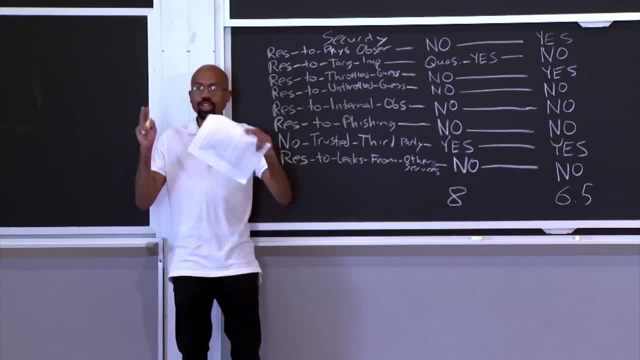 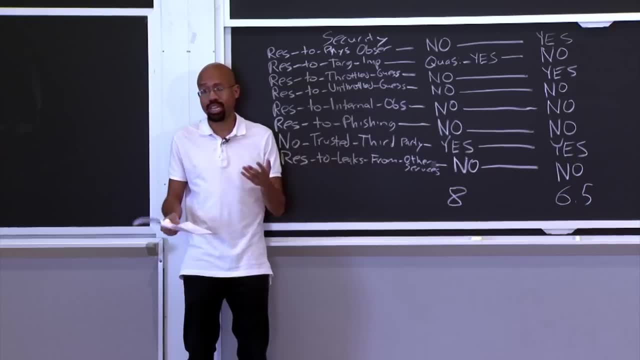 So maybe it makes sense, if I just want to check how much money I have, maybe just the password or just the pen is good enough for that, But then maybe, if I want to actually withdraw some money, maybe we use some two-factor authentication scheme. 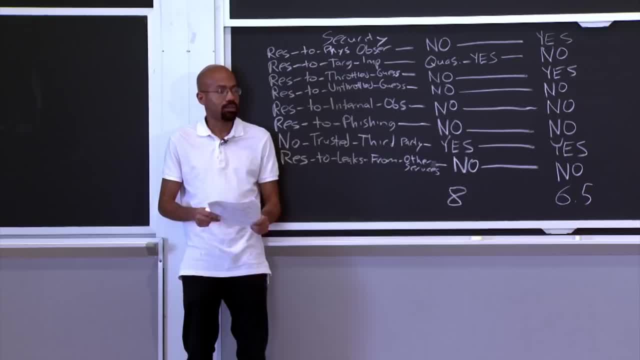 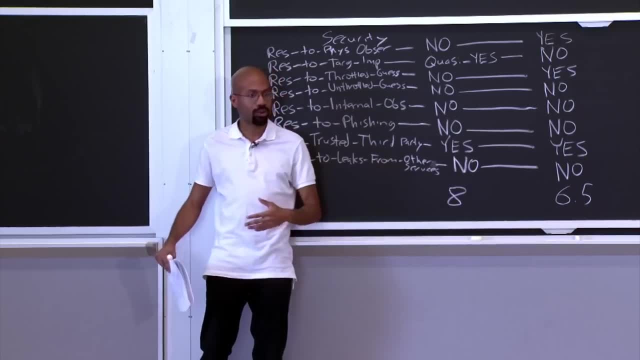 Maybe something gets sent to my phone or maybe something like that. I know once again, in the overseas scenario, if you're somewhere where you don't necessarily trust that terminal, it can be nice to have that two-factor authentication protecting your transactions. 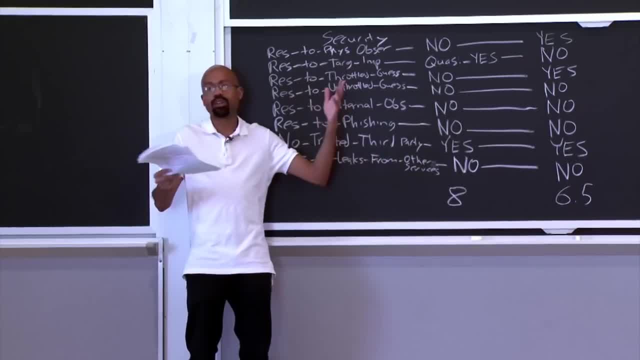 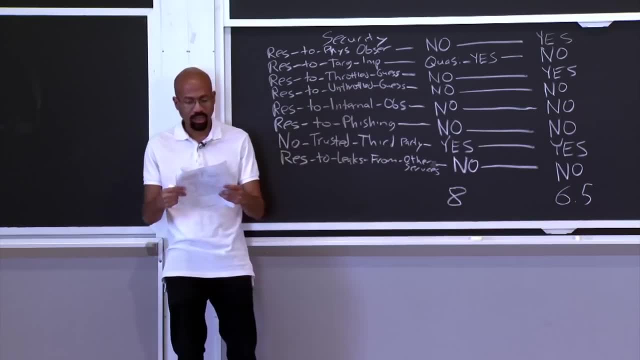 Because maybe you don't care if the criminal reads that you have some x number of dollars in the account, but you don't want them to actually change that either which way. All right. so what's interesting is that you get to the end of this paper. 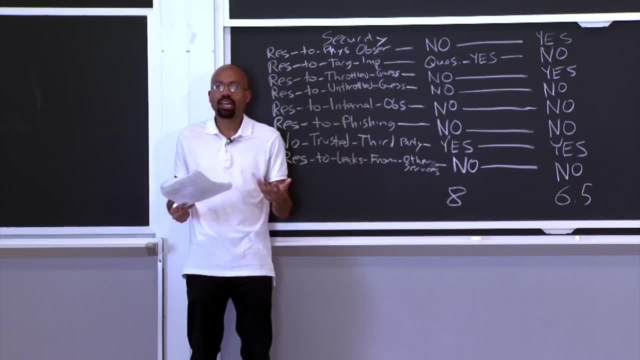 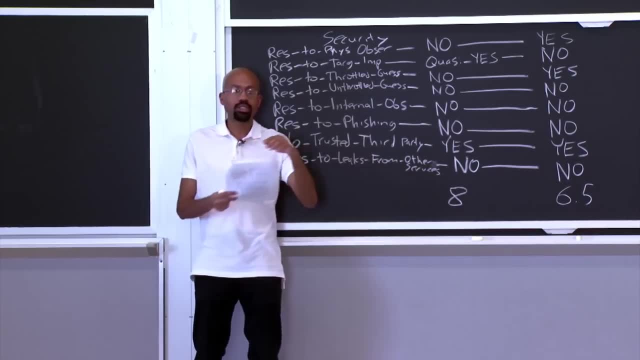 and in a sense it's kind of like watching Inception. You're kind of like I feel both happy and sad. That was a weird ending, Because on the one hand it says: well, here's this nice framework for evaluating stuff. 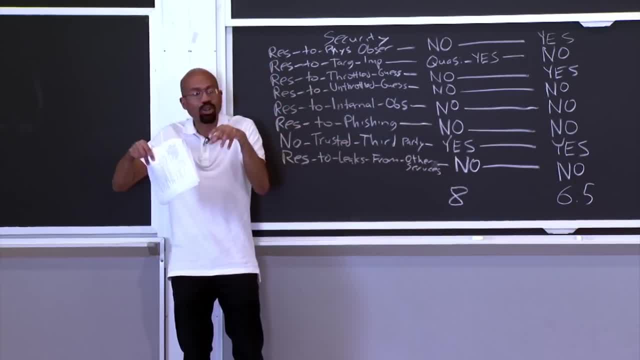 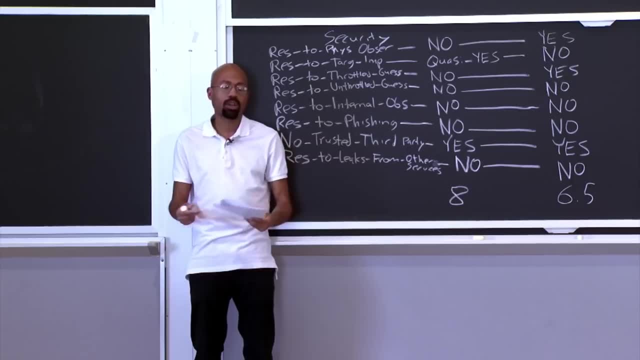 As it turns out, these schemes, they don't nicely cluster in terms of here's everything that is better and here's everything that is worse, And so the conclusion, I think, of the paper is that, well, this is authentic. 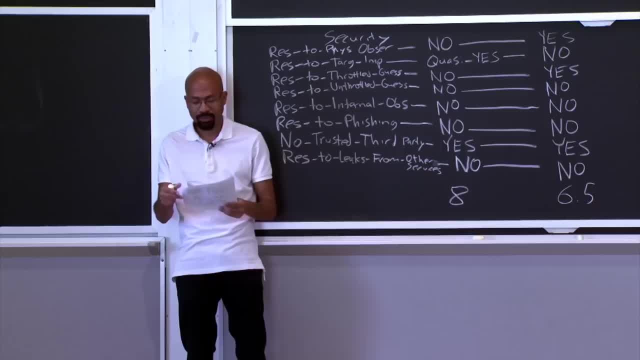 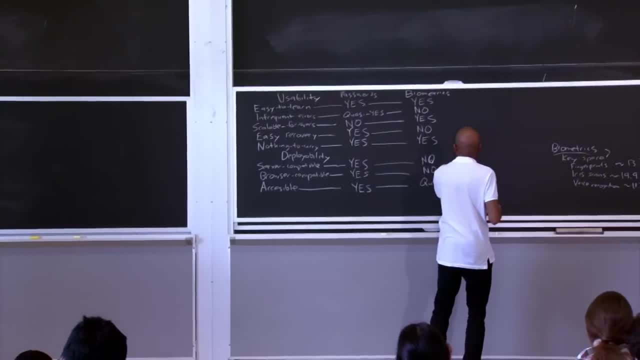 The communication scheme that you should use is actually highly dependent on your particular situation, And so I think one great example of that is this thing: They don't mention this in the short version of the paper, but they mention this in the longer version of the tech. 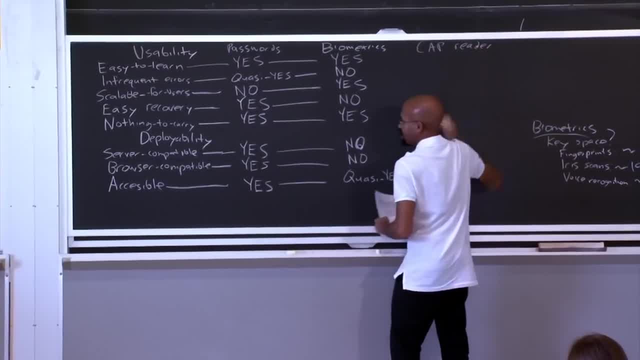 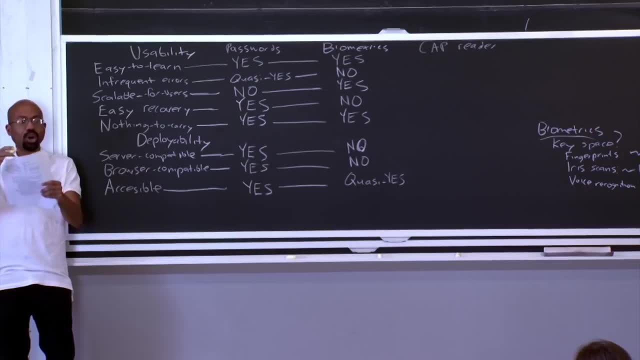 report. It's this thing called the CAP reader, And the reason I thought that was interesting is because if you look in the short version of the report, it says there was only one thing: that got total dominance on the security questions. That just went all the way through. 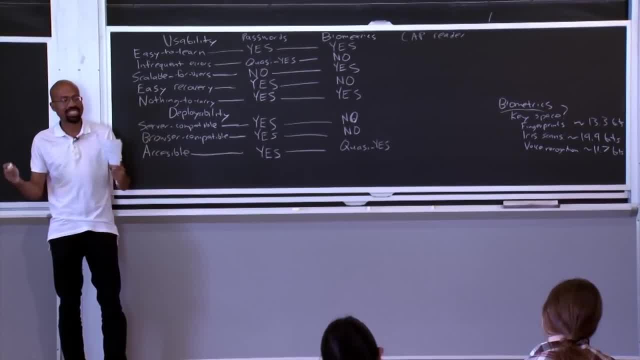 and it was like: yes, yes, yes, it's the CAP reader. We don't talk about it in this short paper. I was like: ah, So I went over. I read the longer version. So what is the CAP reader? 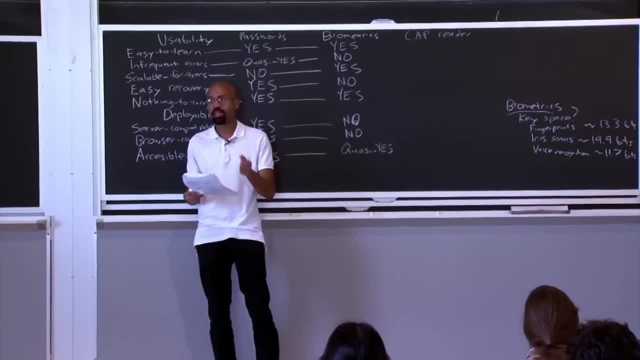 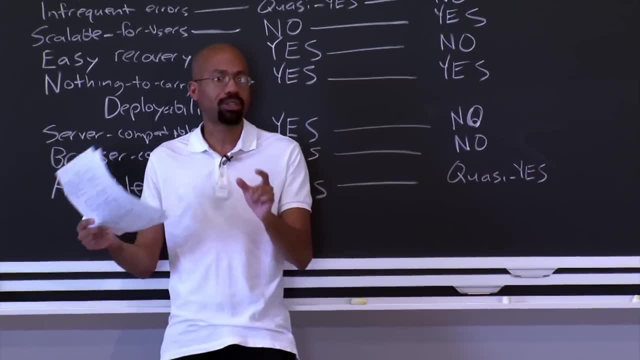 So basically, it's a way to basically protect online credit card transactions And it looks like a little handheld calculator basically. And so you take this CAP reader and let's say you want to go pay for something online. You take your card, you put it in there. 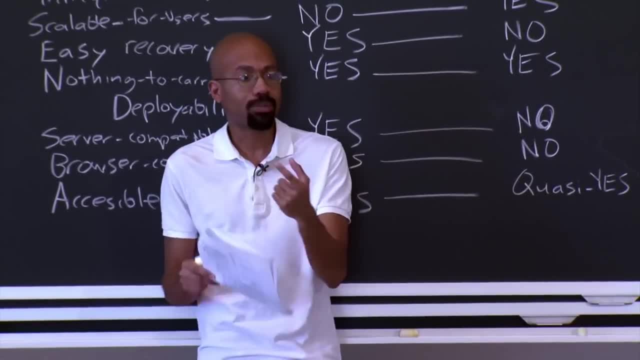 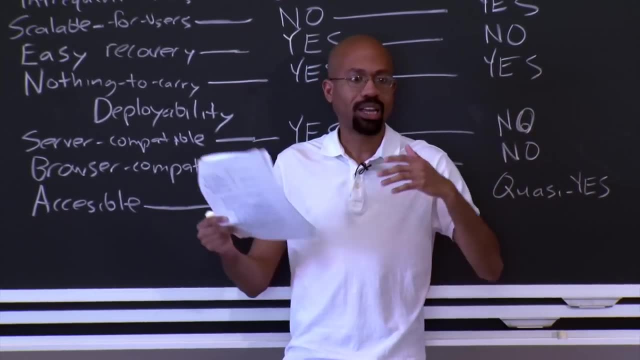 and then you enter your PIN into that CAP reader. Now note that because that CAP reader comes from MasterCard, abstractly speaking, and because it can't be, you know, updated with stuff that the user installs, MasterCard trusts that CAP reader to not have malware. 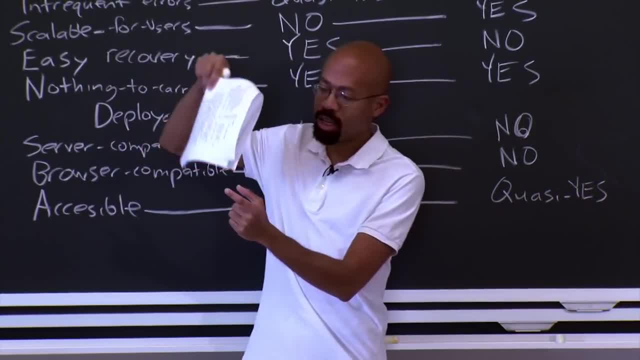 So that avoids the problem of key loggers and stuff like that. So you put your card in there, you enter the PIN to this trusted terminal and it's basically going to output some eight-digit code, And that's the code that you actually. 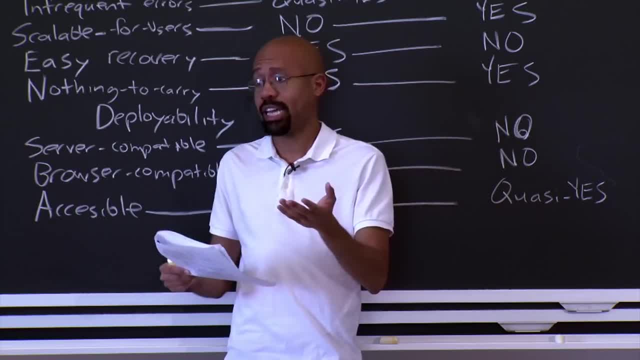 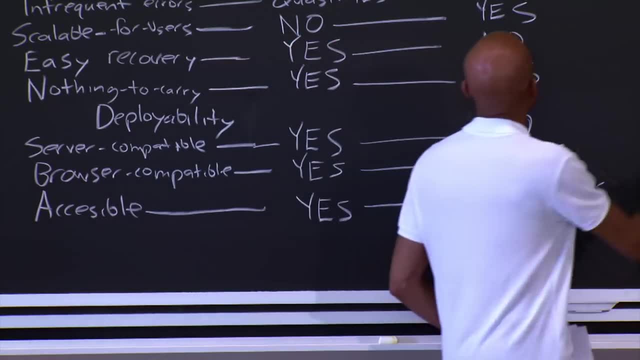 use to tell the web service: hey, I am who I say I am with respect to this particular card here. So that's sort of the physical setup of how you use it. So what does that longer version of the paper say about the CAP reader? 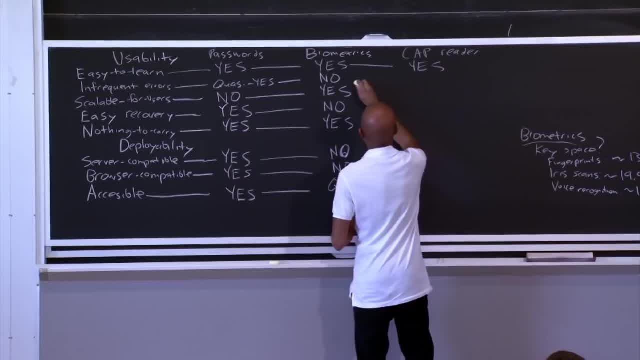 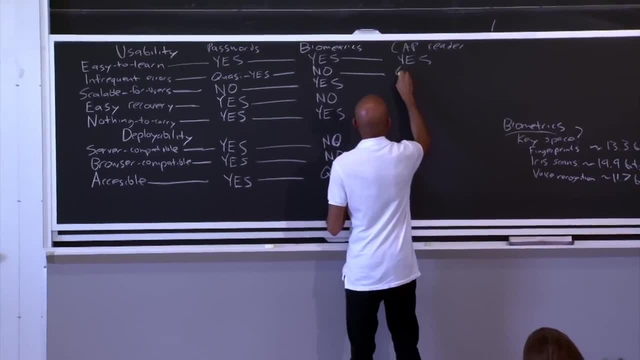 So they say it's pretty easy to learn because you just stick your card in there, enter your PIN, kind of like you would do it in ATM. That all works fine. For infrequent errors they say quasi-yes for the same reason that they say quasi-yes for passwords. 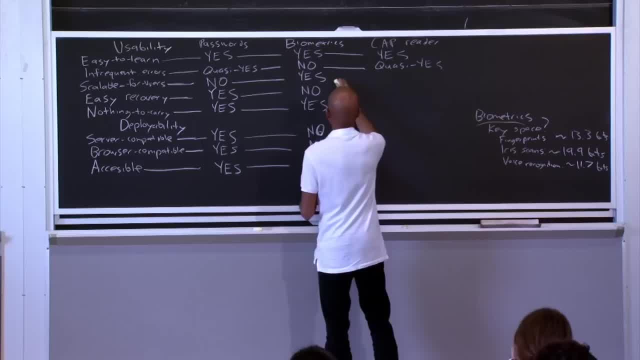 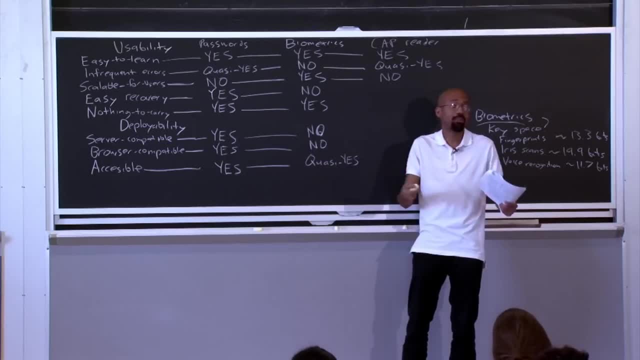 Because entering your PIN, sometimes you might make a mistake or something like that. It is not scalable for users because you basically have to have a separate credit card, a separate PIN, maybe even a separate CAP reader for each site that you go to. 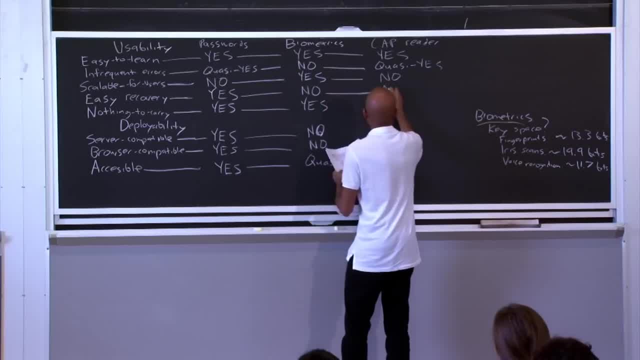 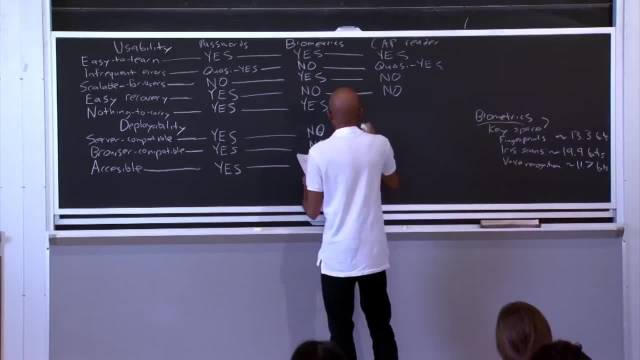 So it says no for scalability. Easy recovery is no right. How do you replace a lost CAP reader? How do you get a new card? That's kind of a pain And it also fails nothing to carry because you've got to carry your card in the CAP reader. 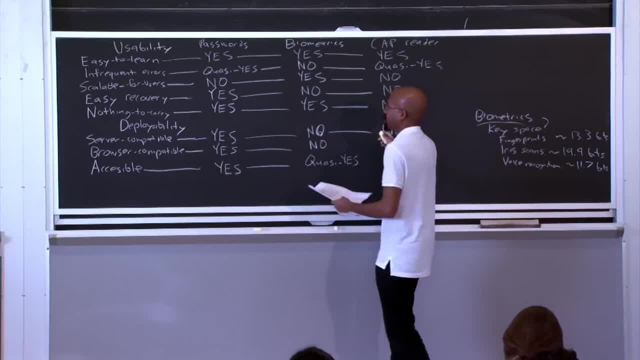 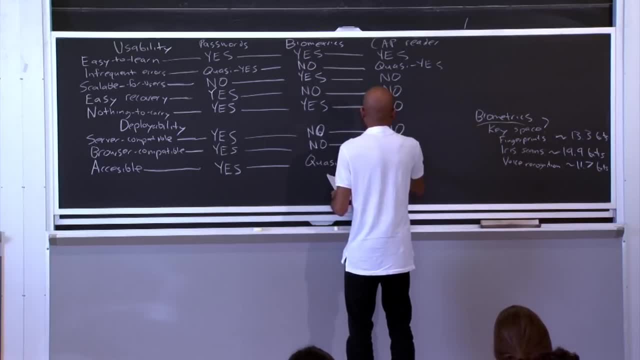 So this is not server compatible, because the site has to know how to use this special CAP reader protocol before it can proceed. It is browser compatible, though, because you're just using standard HTML CSS JavaScript to interact with the back end. 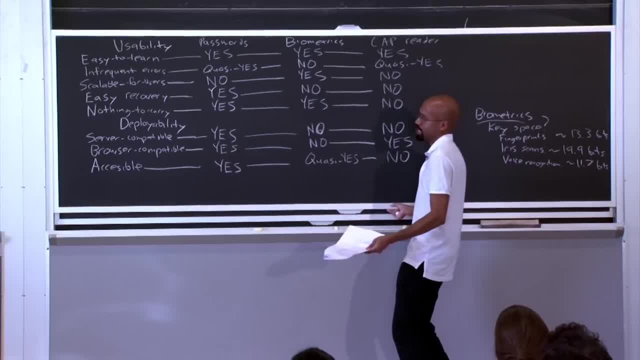 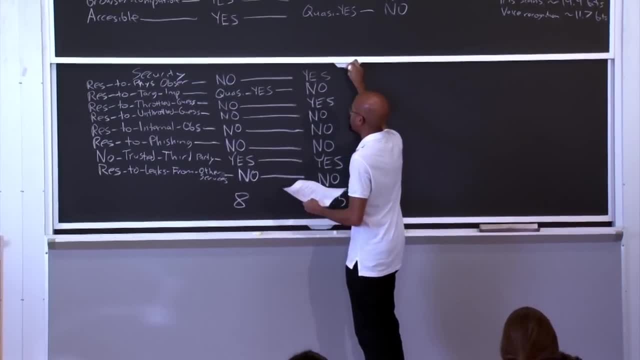 And the authors say no, it's not accessible because blind people can't easily read that eight-digit code that's put out by the CAP reader. So what happens next? So, for the security questions, though, this thing just dominates, right. 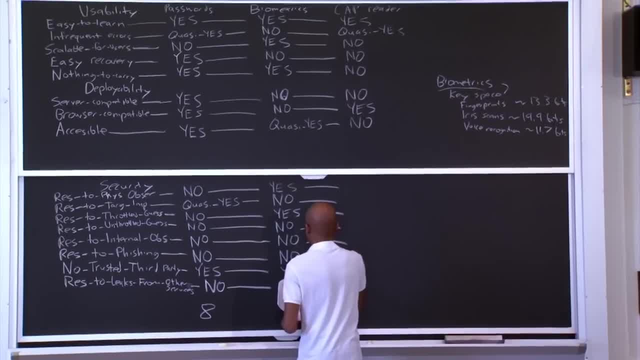 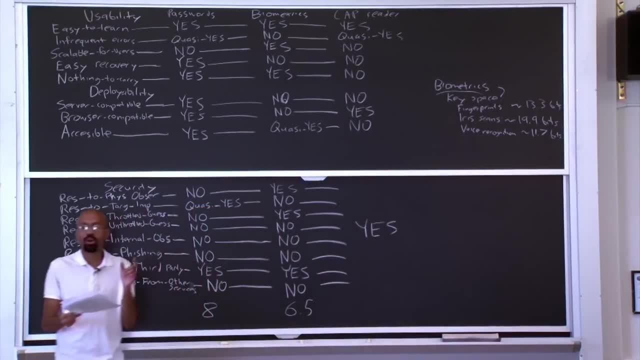 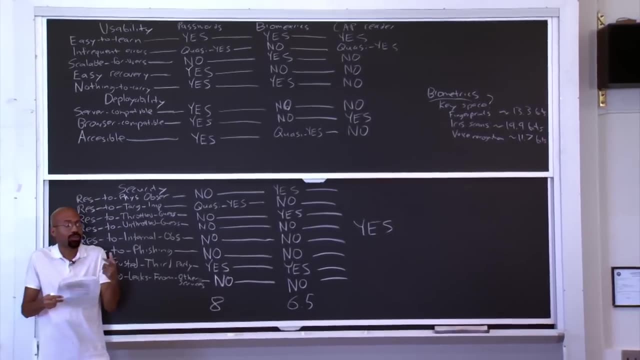 So for every single one of these, it's a yes right. So, in particular, these eight-digit codes that are output by the CAP reader. they're one-time codes, So every time you have an online transaction, it'll spit out this unique thing that will never be used again. 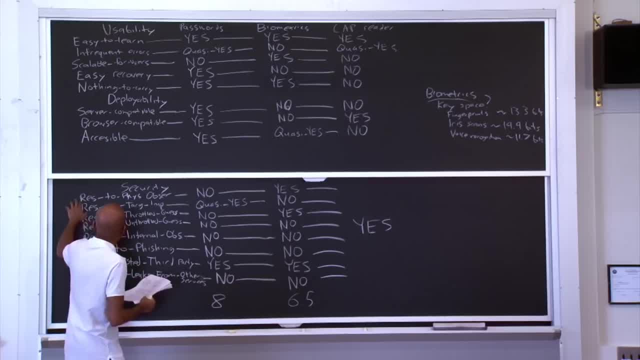 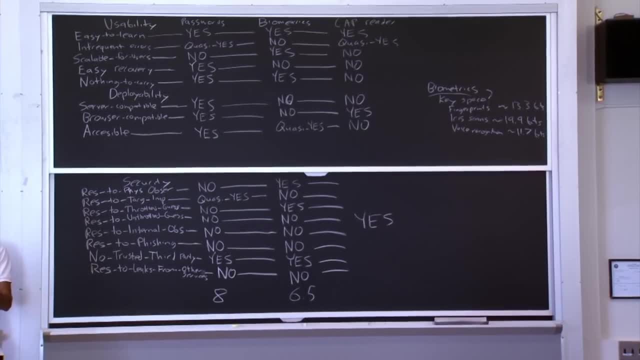 So what's nice about that is that means, for example, that it's resistant to physical observation, Because if I see you generate a particular eight-digit code, I can't use that again. It's not a static token like a password. 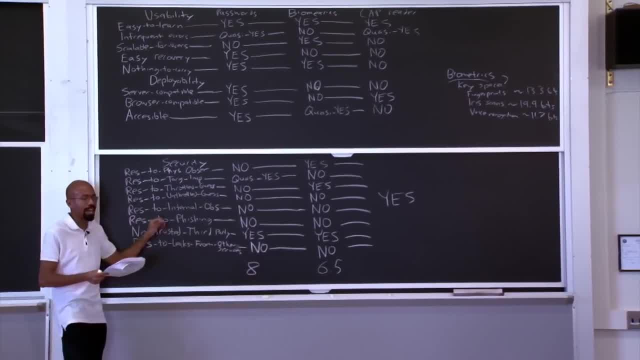 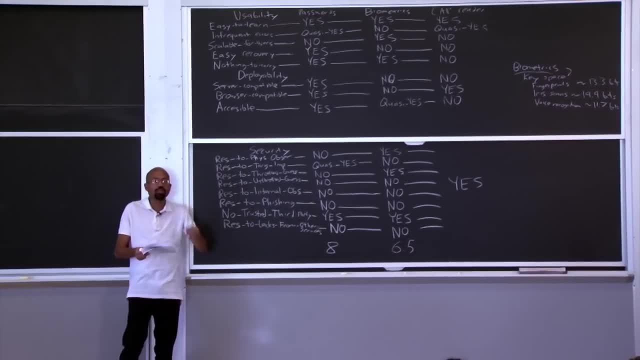 Similarly, it's resistant to throttled and unthrottled guesses, because these things just get thrown away, Right? So even if I leak one of these things to you, you can't then use it to impersonate me. Why is it resistant to leaks of that eight-digit code? 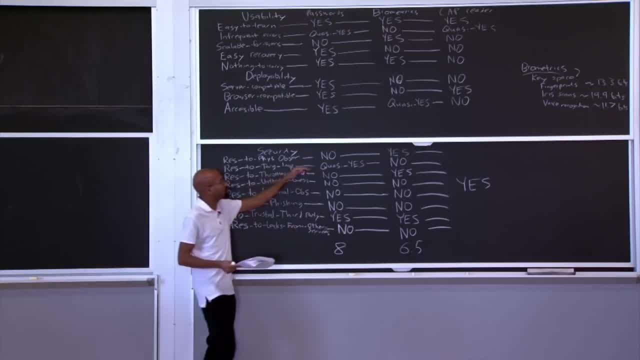 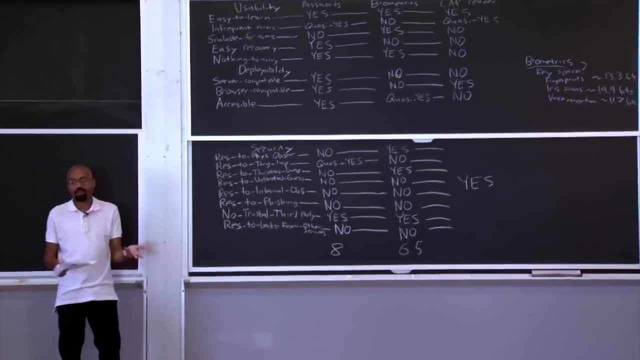 from other services. It's a one-time thing once again, So the CAP reader just runs the table on all these security properties. And yet people don't use CAP readers in practice, right? They're not a super popular thing, And so why does that happen? 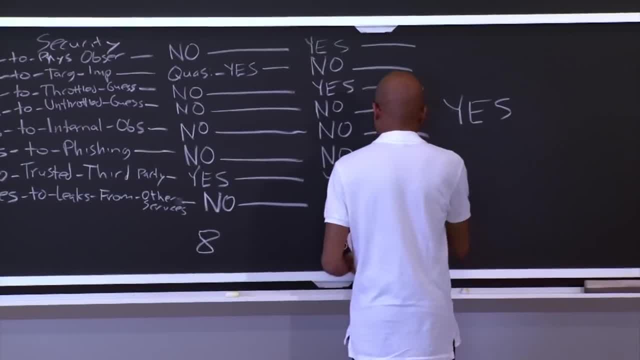 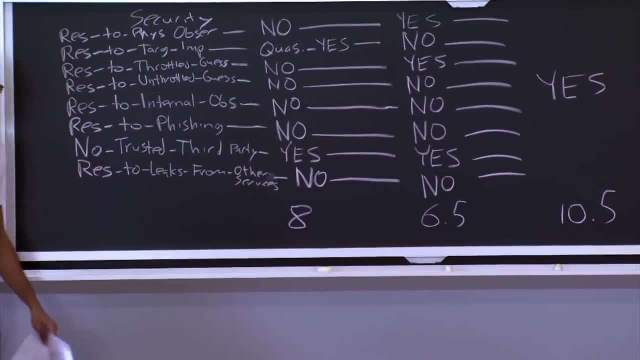 Well, once again, and in fact one thing, I forgot. So if we're looking at my little sort of qualitative number score, so CAP readers get a 10.5.. And so this seems great, particularly because it runs the table on all these things here. 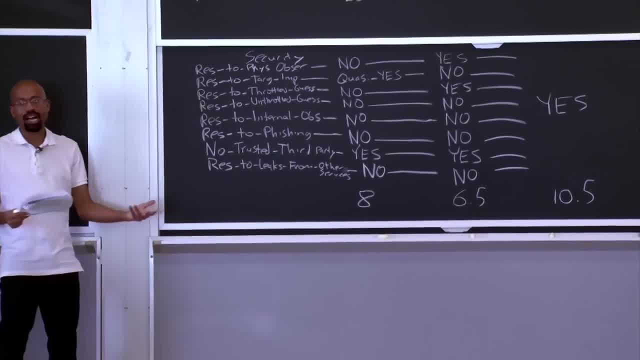 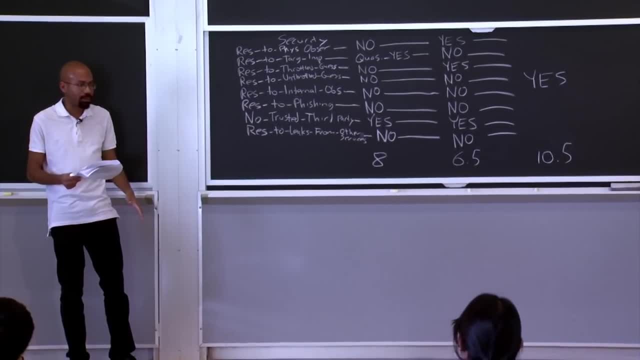 But once again, why don't we use these things? Well, because in most people's lives there's a bad trade-off here between the security and then the usability and deployability. People don't want to carry on CAP readers, People don't want to go through this whole protocol of I. 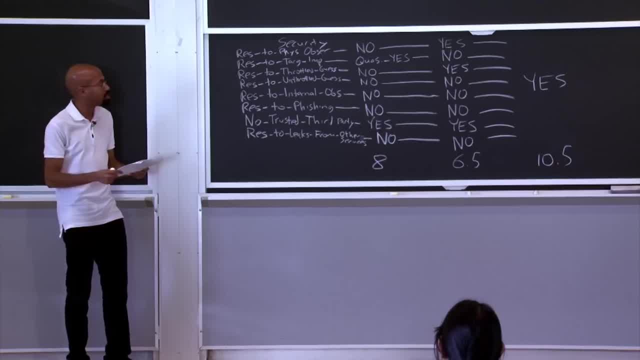 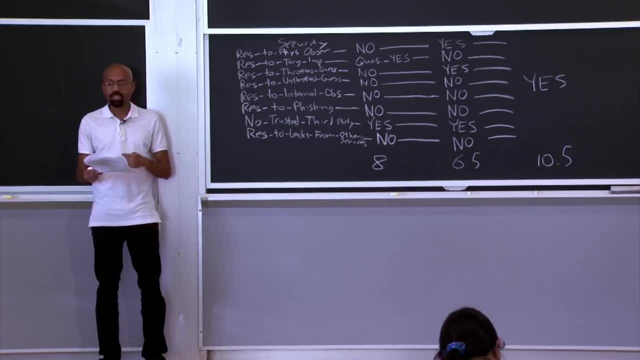 got to put the thing in here and then get this digit and then sort of put this digit into the website. And so what this means is that, in practice, deployability and usability are oftentimes more important than security, Because developers don't want to go. to the cost of integrating these new mechanisms into their services. Users don't want to have to learn how to use these things, And if users are given any freedom whatsoever to choose the security of their scheme, they will often pick small passwords or weak pins.